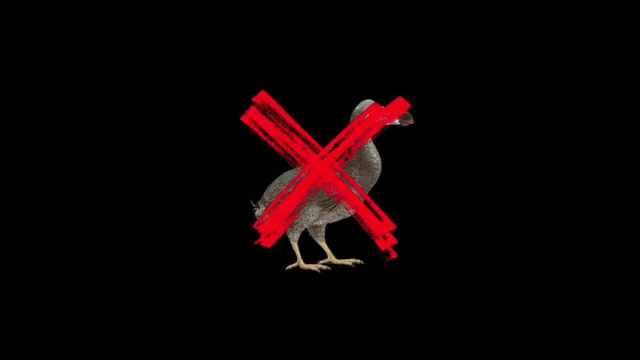 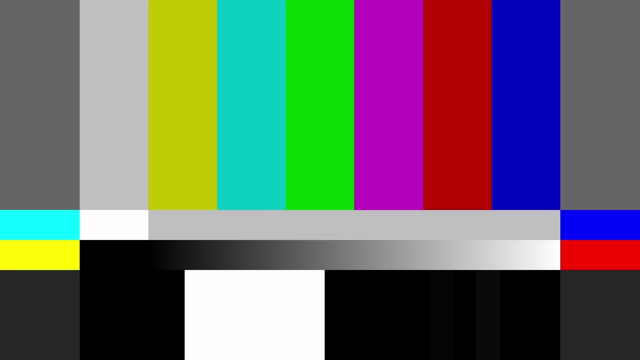 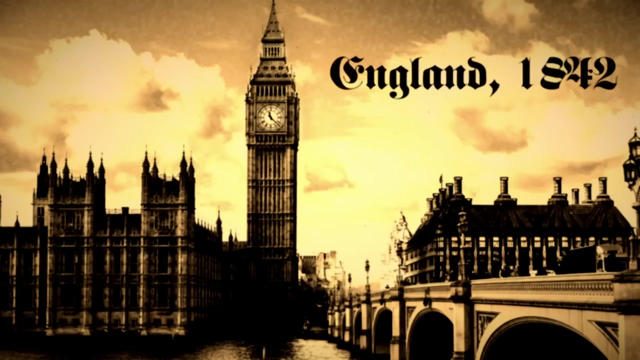 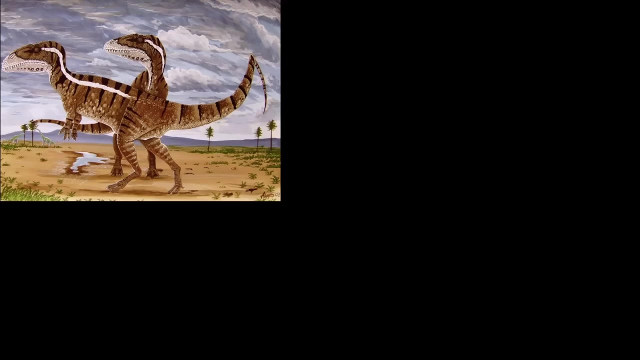 Dead as a Dodo. Hmm, Hey, so does anyone remember England, 1842, when naturalist Sir Richard Owen was studying giant fossils of long-extinct reptiles? He noticed that three specimens- Megalosaurus, Iguanodon and Hylaeosaurus- shared several. 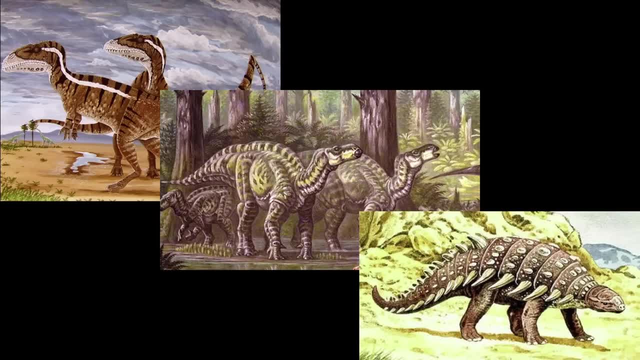 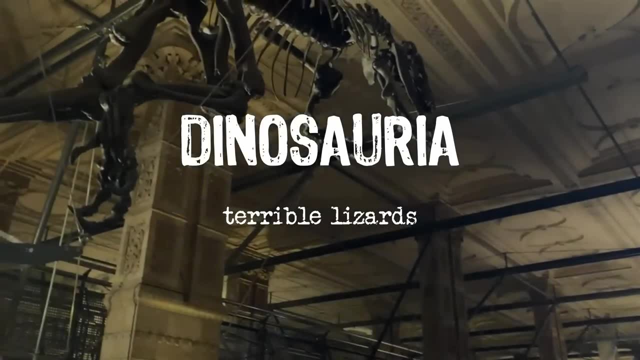 distinctive traits. He proposed that species with these traits be grouped into a new scientific classification – Dinosauria, Greek for terrible lizards, And everything was fine and dandy and everyone was having a great time defining dinosaurs by physical qualities until some guy called Charles Darwin turned up and said: 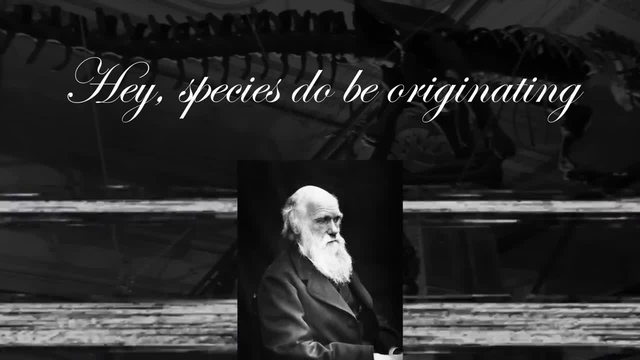 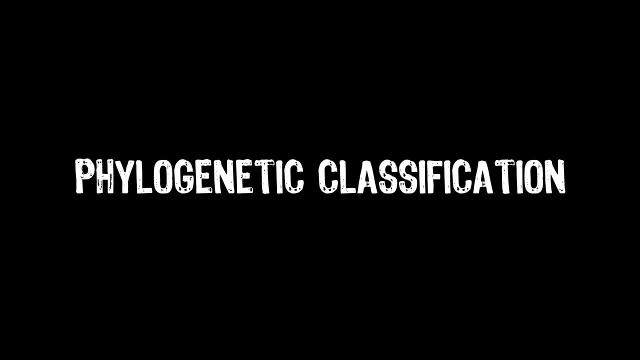 Hey, species do be originating. And then, once they realised things evolved, the naturalists threw out their old textbooks and invented this new thing called phylogenetic classification. In phylogenetic classification we imagine a big family tree of all species ever. 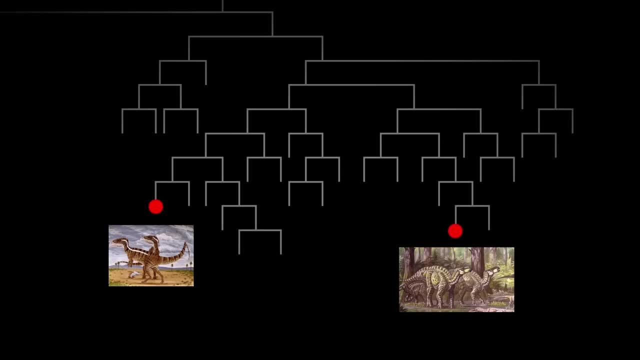 Somewhere here we'll find, say, Megalosaurus and Iguanodon, And we define dinosaurs as Well. if we climb up the tree far enough from each of these species, we'll find a species that's an ancestor to both of them. 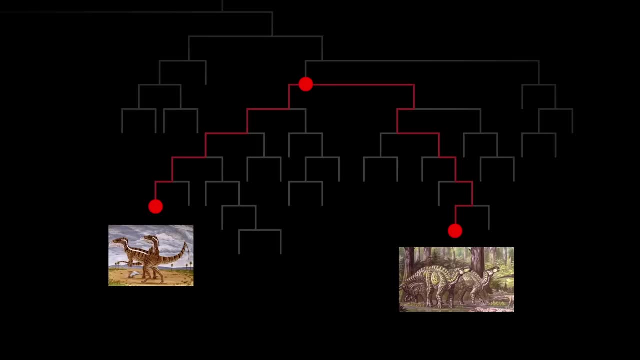 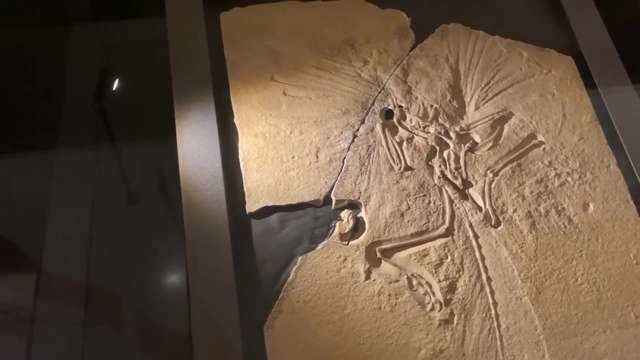 We take the latest possible such ancestor to be the first dinosaur, with dinosaurs as a whole, comprising everything that animal ultimately gave rise to. And that's great right- A definition of dinosaurs based on their very evolution. But somewhere along the line, scientists discovered that birds share many traits with 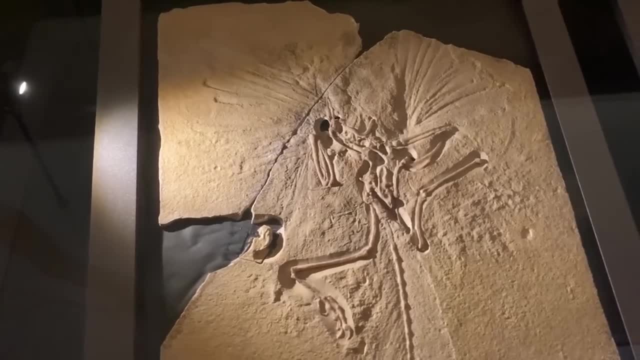 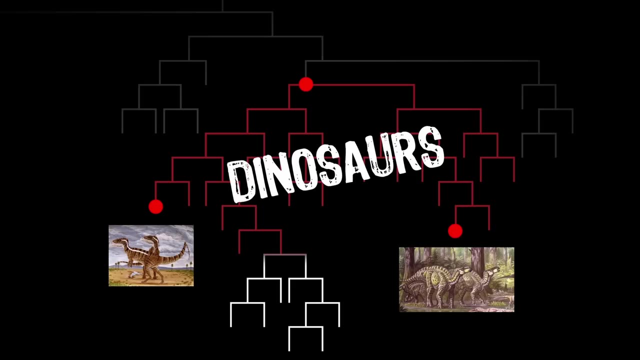 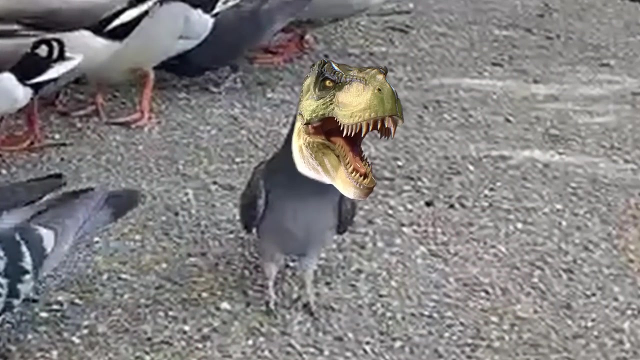 certain groups of dinosaurs And therefore must have evolved from them. In other words, the entire bird family tree fits here And according to phylogenetic classification, we have an inescapable conclusion: Not only did birds descend from dinosaurs, they ARE dinosaurs. 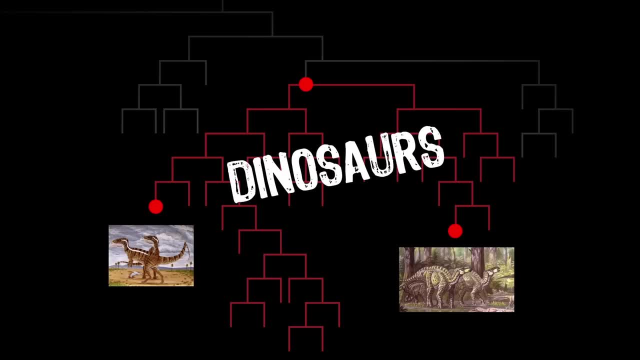 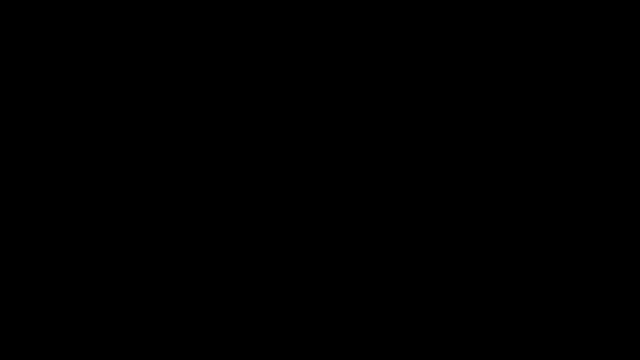 Or rather they were, until scientists decided birds evolved from something else and they took the whole bird family tree out again. But then they put it back And to make sure they never made the same mistake again, they redefined dinosaurs to be all animals descended from the last common ancestor, a triceratops and a sparrow. 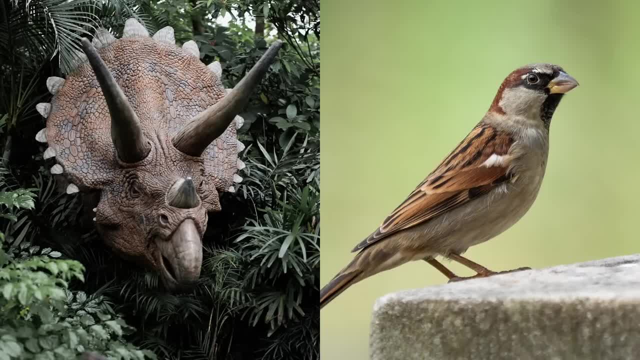 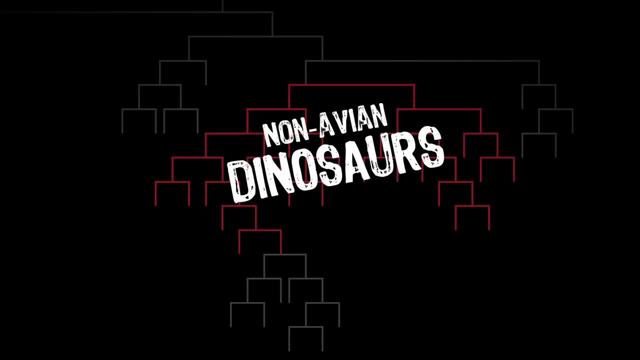 Yes, the very definition of terrible lizard now depends on the sparrow. If you want to talk about dinosaurs except birds, the scientific term is non-avian dinosaurs, And these are indeed extinct. so the question should actually have been: what killed the? 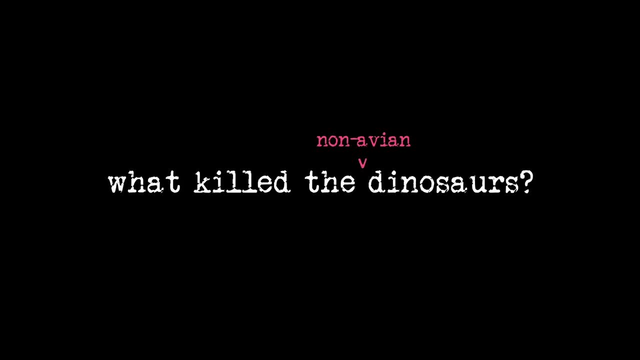 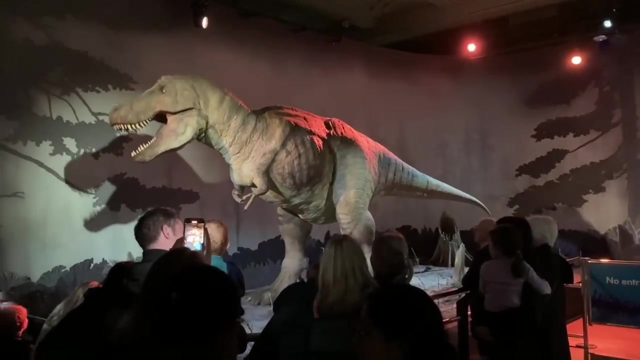 non-avian dinosaurs. Right, That was an awfully long detour. just to explain a clarification everybody probably assumed anyway, Despite being severely simplified, it was confusing and entirely un-conducive, to say. an engaging video intro, But isn't that kind of interesting? 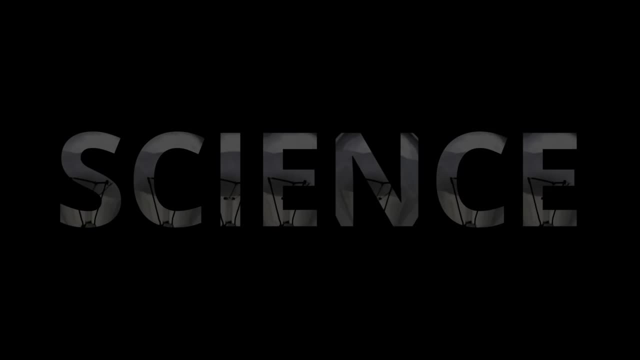 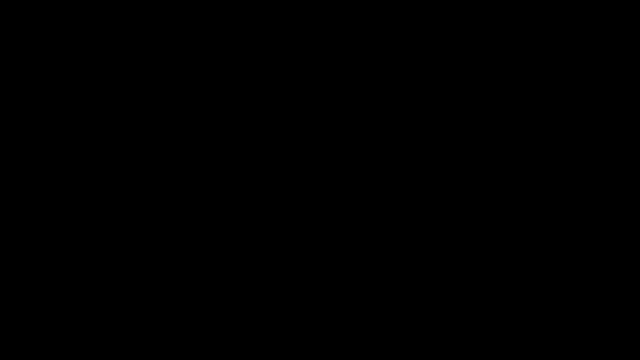 Given you've just clicked on a video about dinosaurs, I'm going to go out on a limb and suggest you might be someone who likes science. But how much is science? How much have you really thought about how that science is communicated? Is it really as simple as scientists do? the science and the public hears about it. 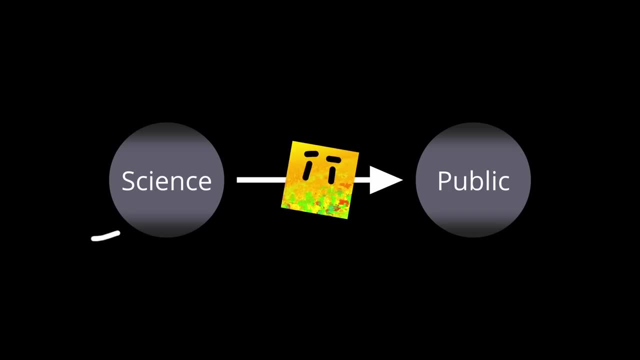 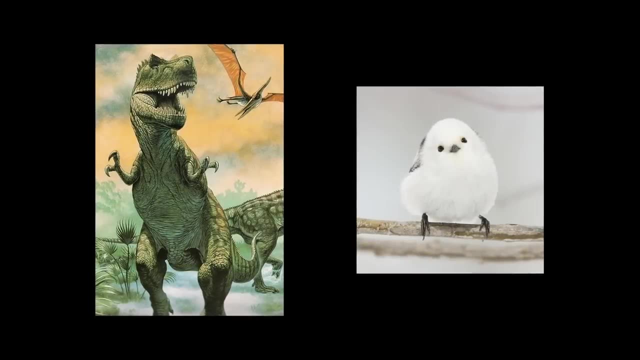 And no, I'm not just talking about the existence of a crooked journalist in between. Turns out, the whole thing is a fair bit more wibbly-wobbly-timey-wimey than that. We've already seen how public and scientific views of dinosaurs can end up in wildly different 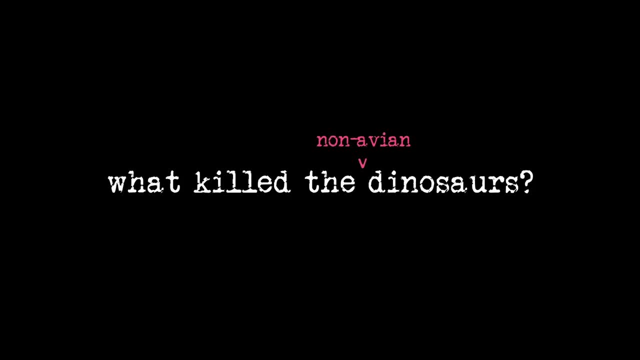 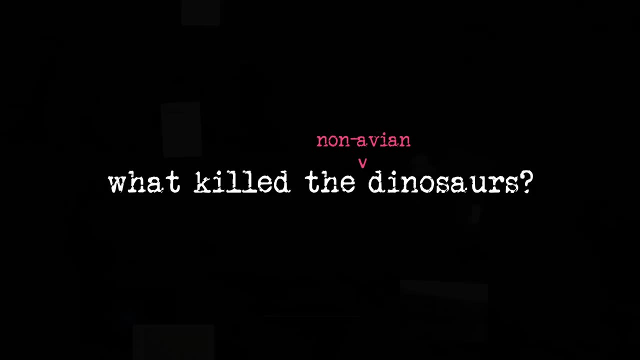 terrain- and no case study exemplifies this- quite like the mass extinction that spelled their doom. Behind this question- A question your mind most likely had a say in, So how much have you thought about how that science is communicated And what's the most snappy answer for the moment I asked it lies one of the longest. 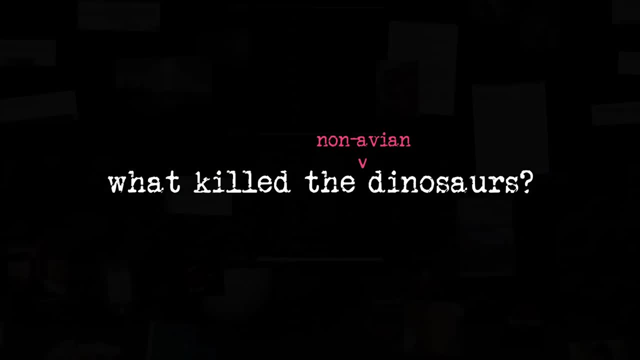 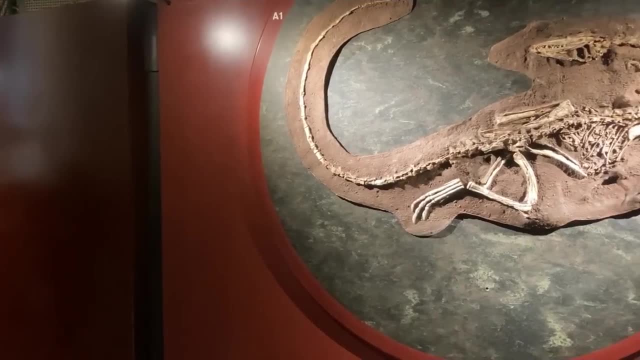 and most vicious feuds in all of science, And one inseparably tied to its own perception in popular media. Inspired by a book that illuminated the debate, as it happened, I've embarked on a mission to understand the dinosaurs' extinction and its place in society. 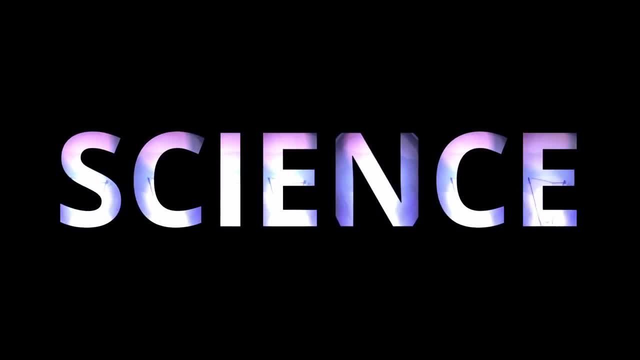 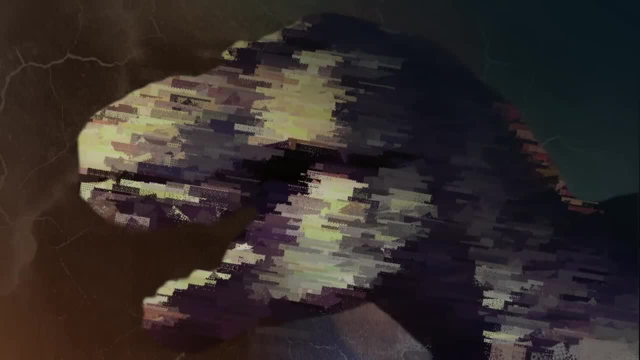 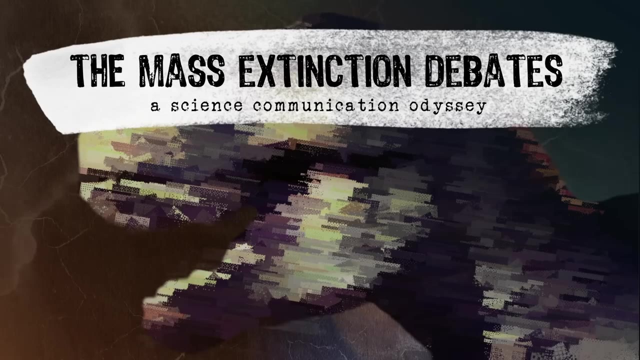 What happened? How do they know? How do you know? And what does it all mean for science as a whole? So if that counts as an engaging video intro, please join me for this excessively deep dive into the Mass Extinction Debates: a science communication odyssey. 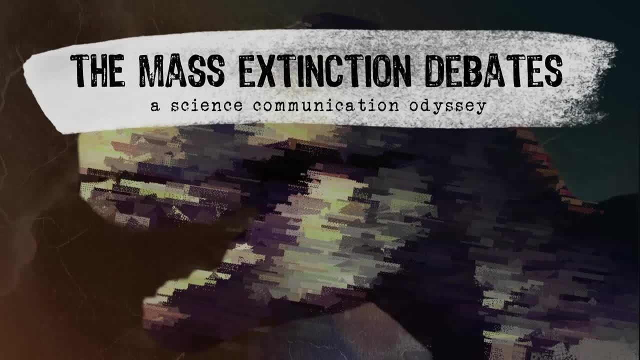 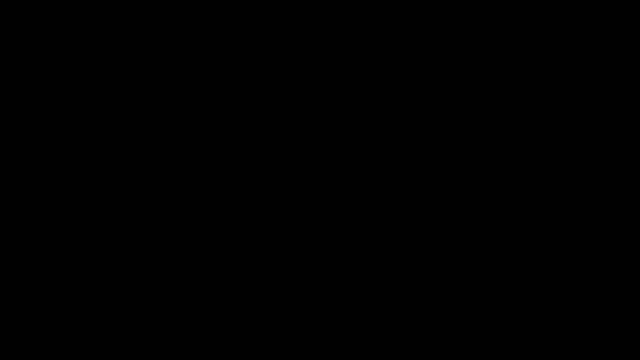 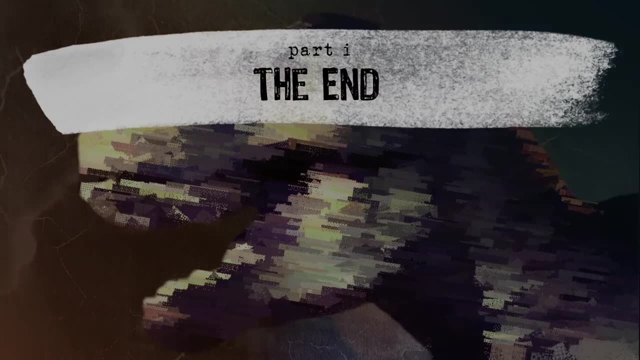 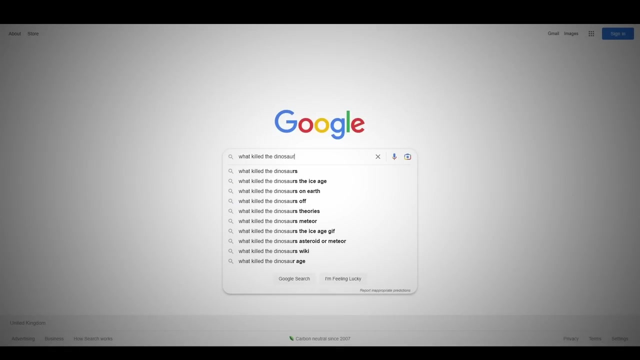 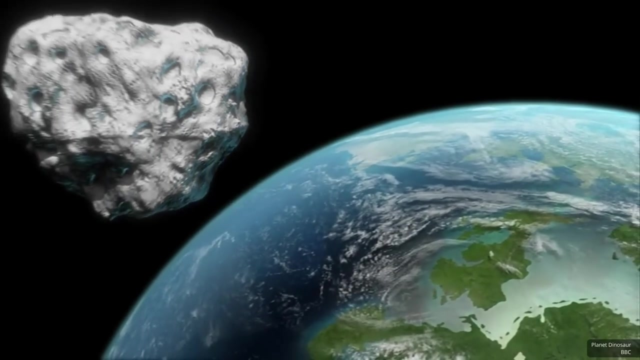 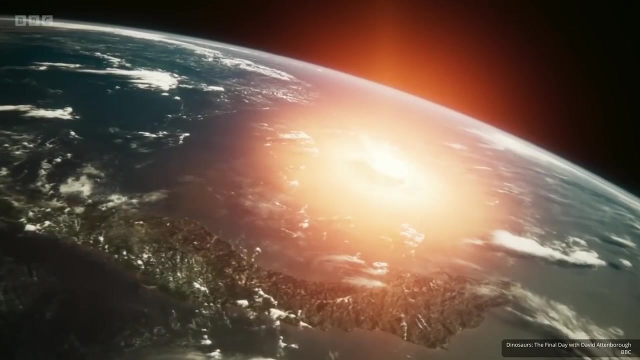 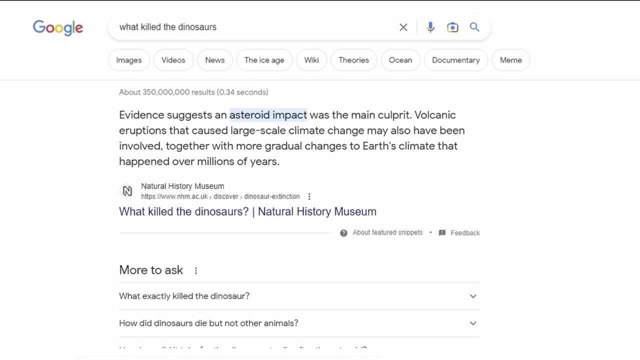 Part One, The End. Well, Google, the ultimate barometer of civilisation, has clearly made its mind up, And never one to miss the chance to copy Google. so has Bing. Your mind, too, probably sprang straight for a big space rock. 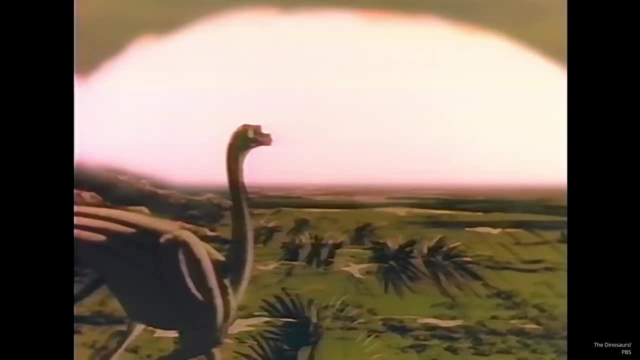 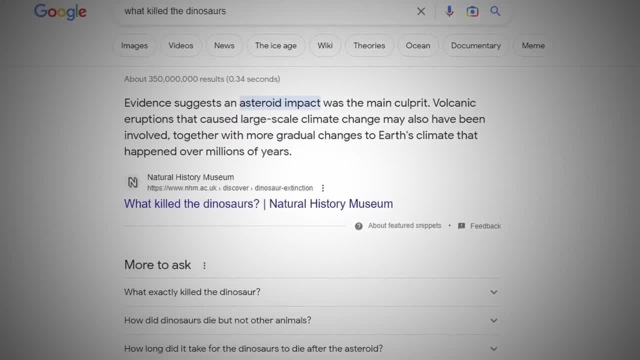 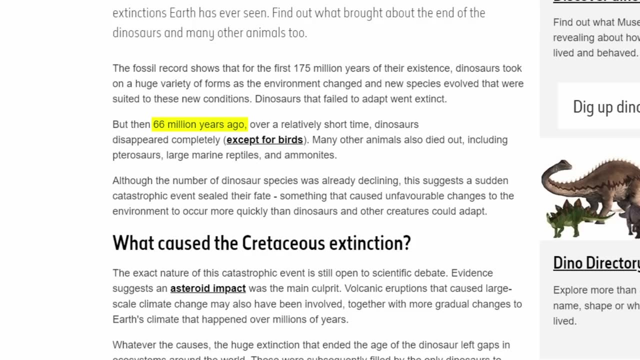 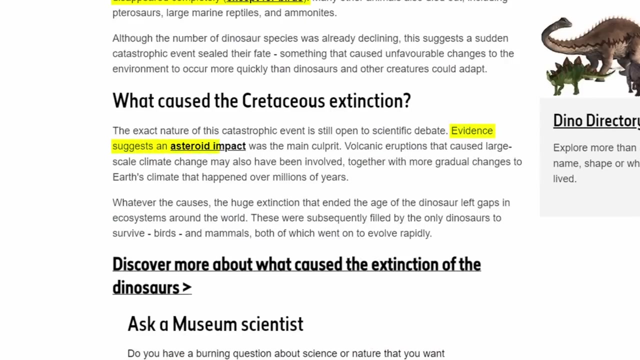 first thought you had. Google's confident verdict comes from the website for London's Natural History Museum, which covers the basics pretty succinctly. Sixty-six million years ago, over a relatively short time, dinosaurs disappeared completely, except for birds. Evidence suggests an asteroid impact was the main culprit. 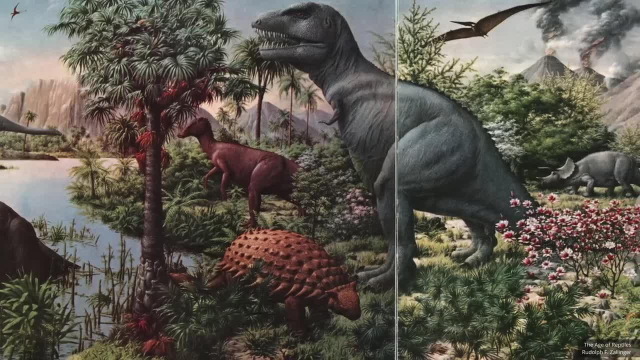 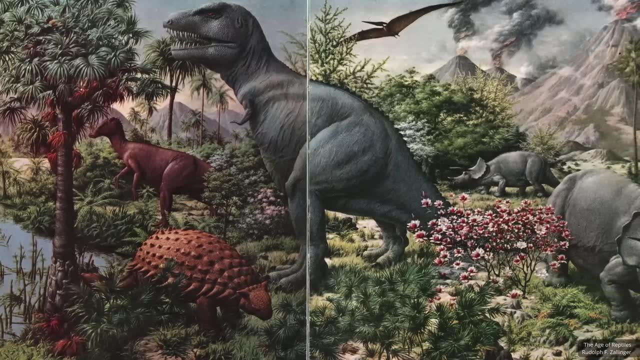 Obviously, not all dinosaurs disappeared at once. Most lived and died naturally, and there were plenty of smaller extinctions- plenty of smaller extinctions during their time on Earth. But this extinction marks the eradication of all non-avian dinosaurs, the boundary between the age of reptiles and the age of mammals. 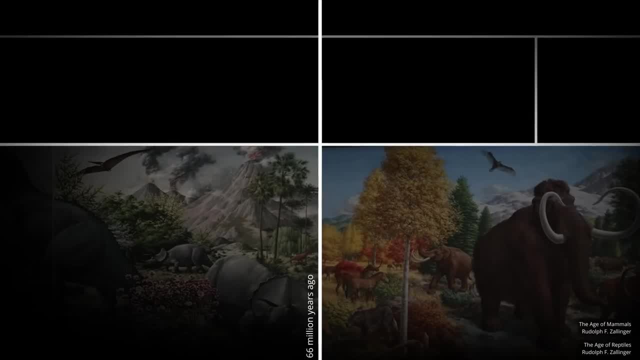 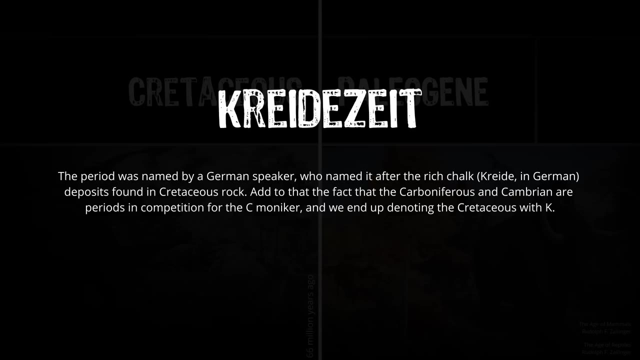 The periods of geological history at this divide are called the Cretaceous and Paleogene. Other sources might use Cretaceous Tertiary instead of Cretaceous Paleogene tertiary being a now outdated term for the post-dinosaur world, So using the German word for Cretaceous, it's complicated. we call this event the KPG or KT. 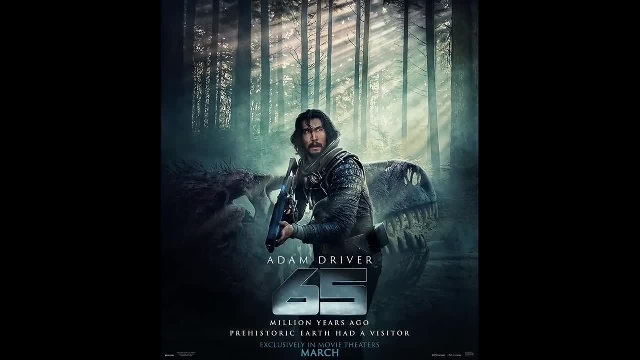 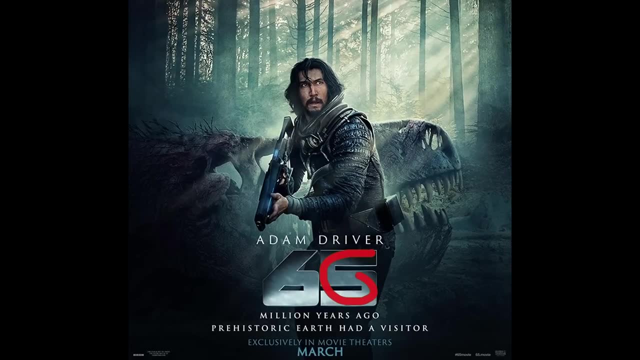 extinction You might be more familiar with 65 million years ago, as the KPG extinction date. This used to be the consensus, but modern rock-tating technology has fine-tuned our estimate a little further back. I, for one, have a distinct memory of most dinosaur media suddenly. 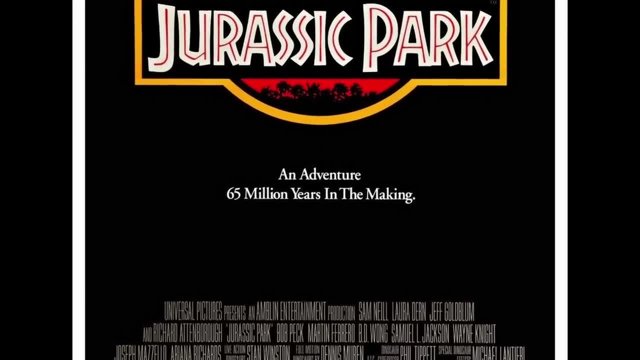 and without explanation, shifting from 65 to 66, and my brain's logical assumption at the time was that we'd somehow have to go back in time to the time of the extinction, of the KPG or KT extinction. So, using the German word for Cretaceous, it's complicated- we call this event the KPG or KT extinction. So, using the German word for Cretaceous, it's complicated- we call this event the KPG or KT extinction. So, using the German word for Cretaceous, it's complicated- we call this event the KPG or KT extinction. 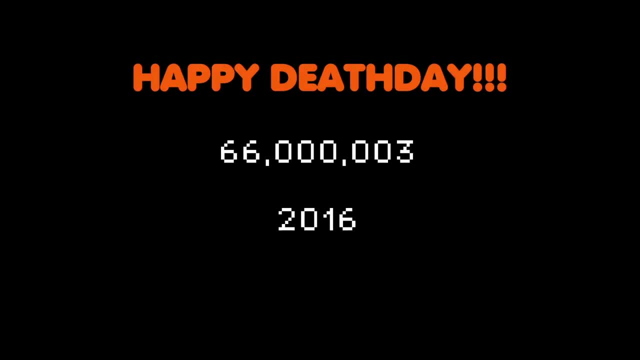 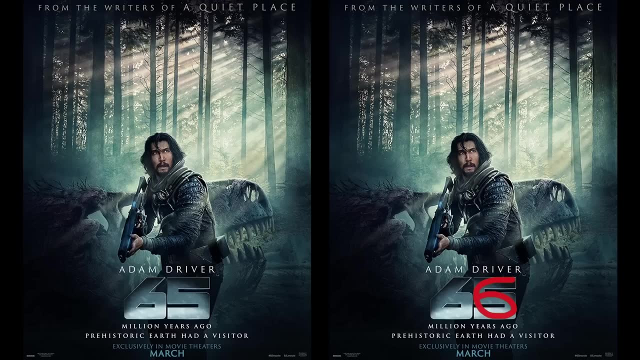 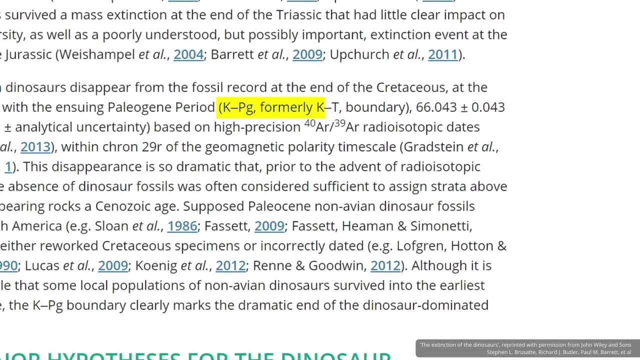 Ticked over, As if we knew the anniversary to the exact year. Even in deciding between two consecutive numbers, we've uncovered another divide between dinosaurs and public perception of dinosaurs. One number is iconic, inseparable from the extinct reptile's very notion. The other is what the science actually suggests. 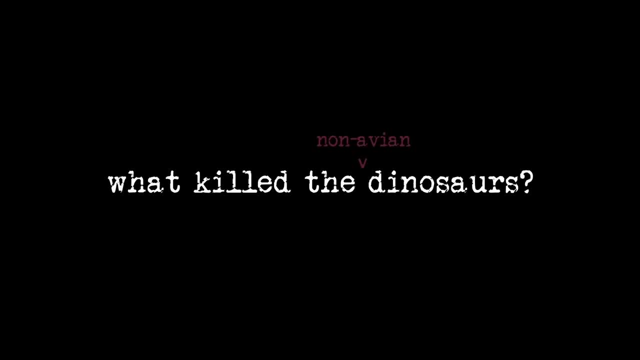 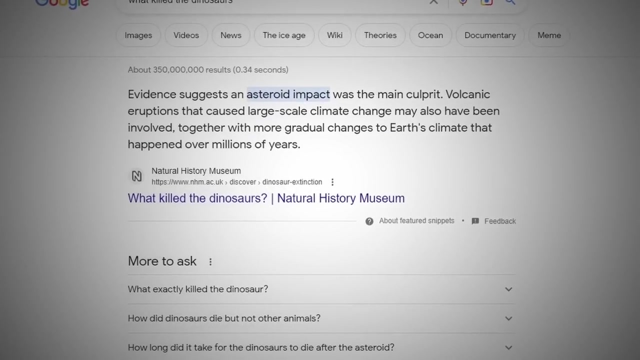 So not only do public consensus and scientific consensus disagree on what was killed, they can't get the when straight either. What chance then is there for the HAW, Since Google has crowned the Natural History Museum the arbiter of KPG extinction truth? 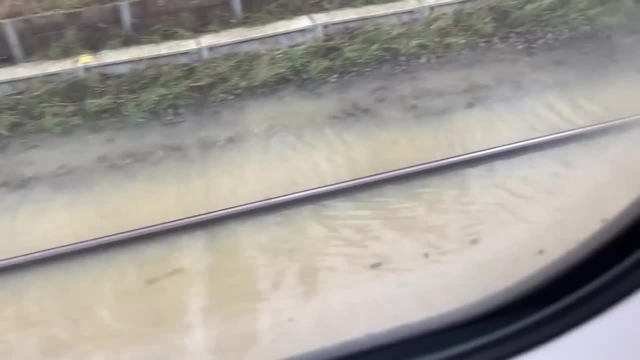 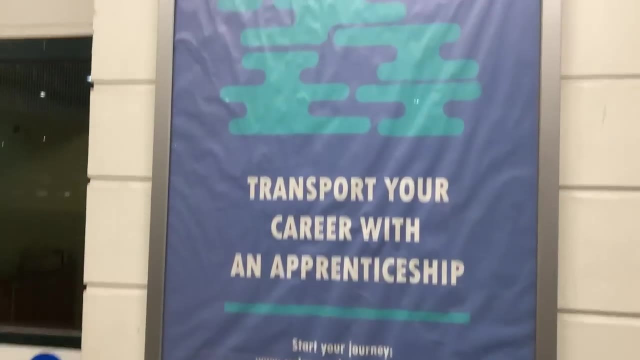 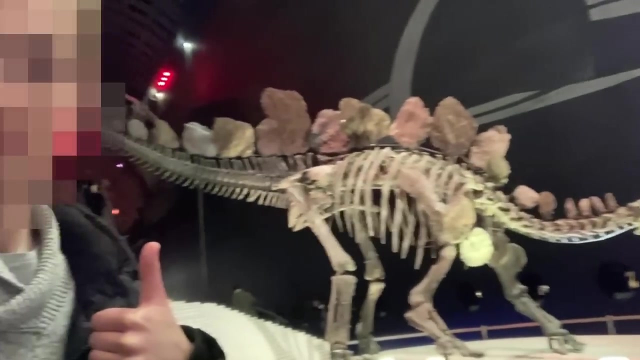 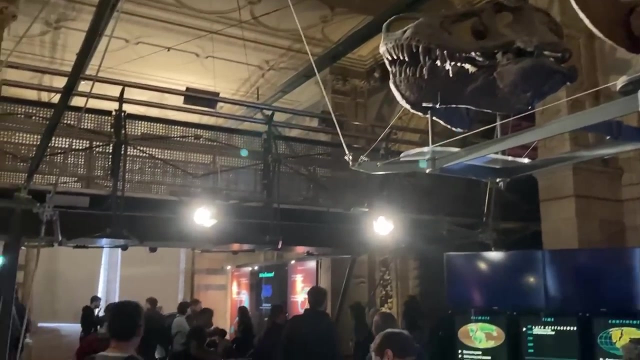 I thought I might as well pay it a visit. I had to survive flooded railways, redirected trains and consequently Swindon, But I did in fact make it. as this highly incriminating footage shows, For nearly 150 years the Natural History Museum has stood as a shining dinosaurian beacon. 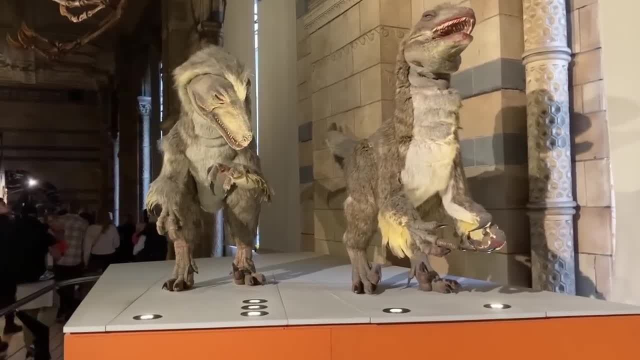 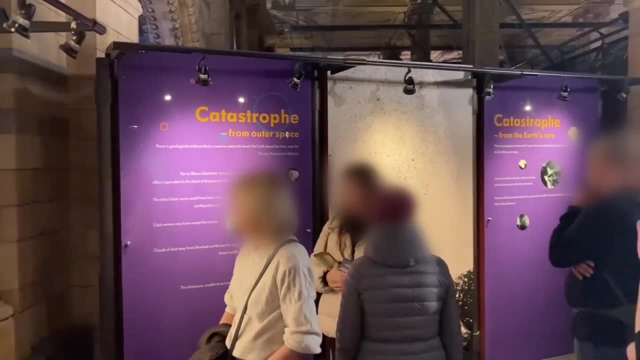 the British public's first port of call for learning about giants of the past. Given its natural science pedigree, which we'll return to later, how does it present the dinosaurs extinction Zooming in on these displays? I was too timid to ask people to move. 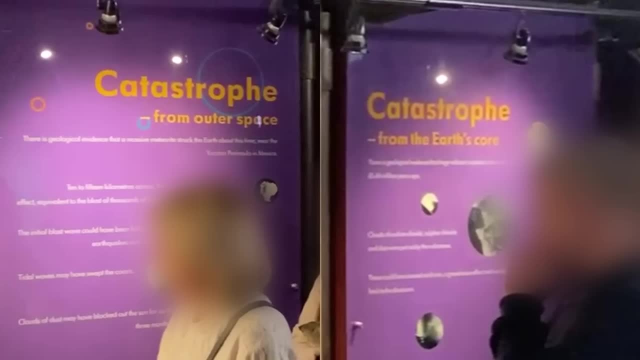 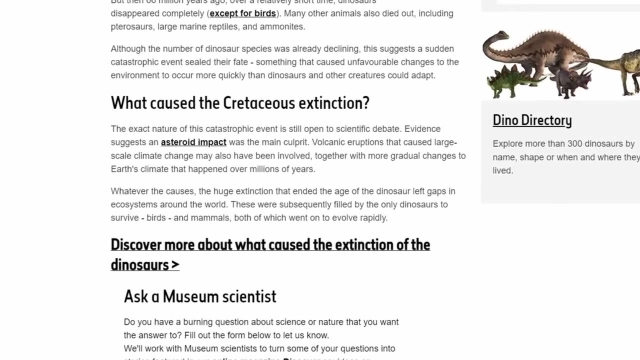 we find the dinosaur exhibit gives two primary theories behind the KPG event: Asteroid impact and intense volcanism. Asteroid impact and intense volcanism: Indeed, the full answer on the museum's website goes into more depth. Evidence suggests an asteroid impact was the main culprit. 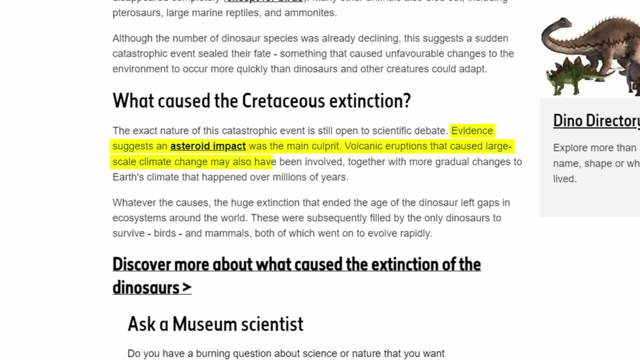 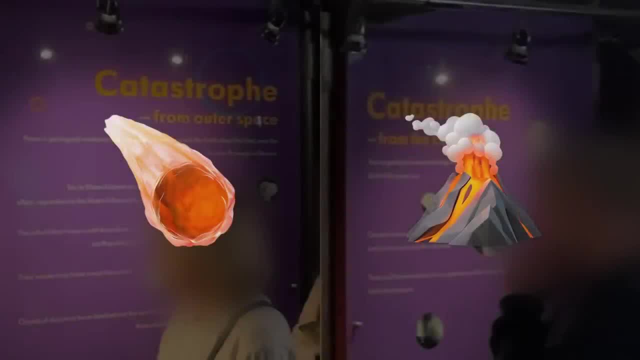 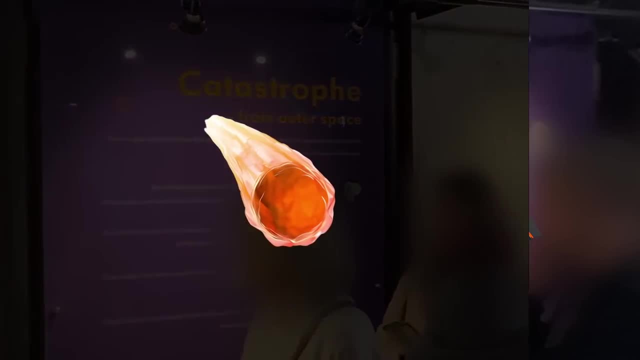 Volcanic eruptions that caused large-scale climate change may also have been involved, together with more gradual changes to the Earth's climates that happened over millions of years. Beyond the museum's summaries, what do these two theories actually say in detail? Everything so far has given asteroid-first billing, so let's start there. 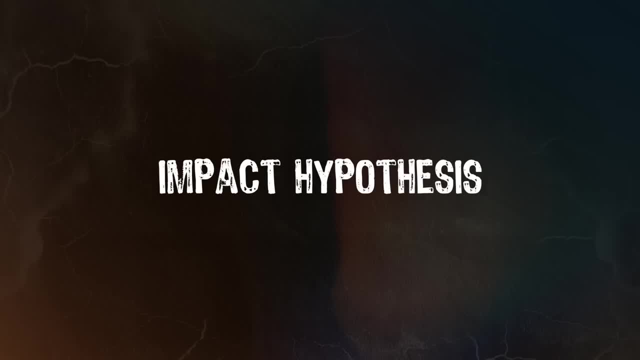 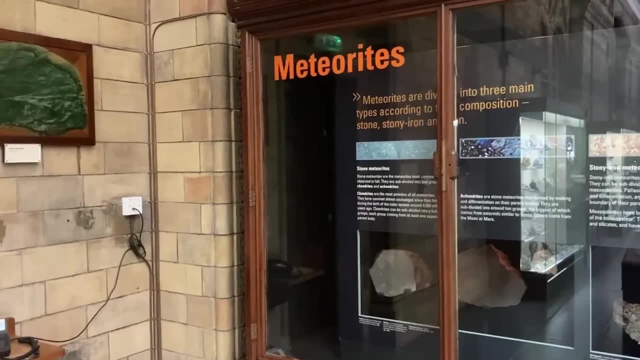 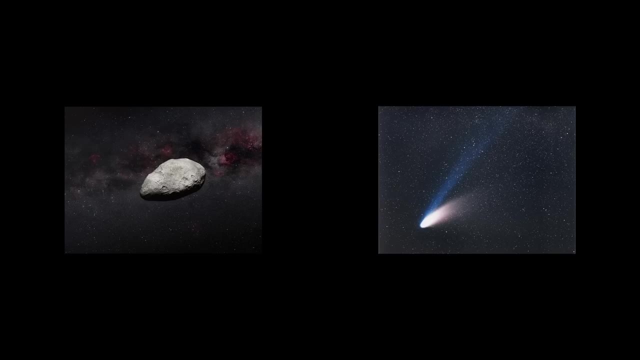 What is the impact hypothesis? In the deep reaches of the solar system there are asteroids. I mean comets Or meteorites. Okay, Asteroids are small astronomical bodies made of rock. Comets are made of ice and dust and often have bright tails. 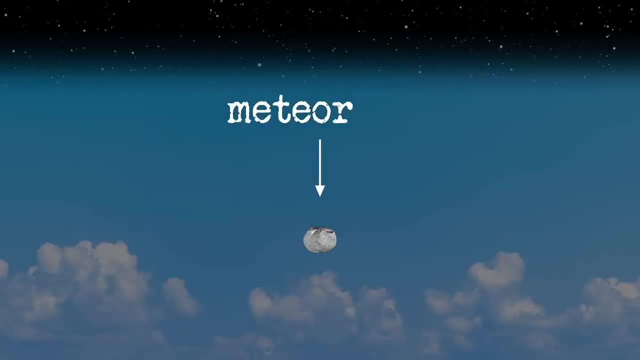 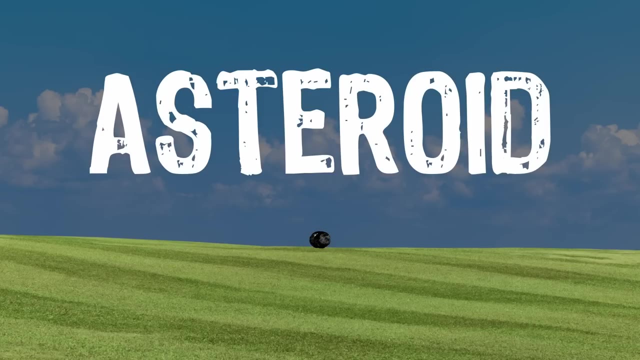 Meteoroids are small pieces of ether which become meteors upon entering the Earth's atmosphere and meteorites upon hitting the ground. For the sake of brevity, I'm just going to say asteroid, to cover all of these from now on. 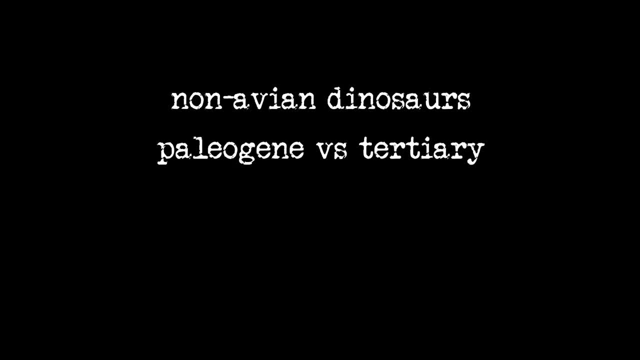 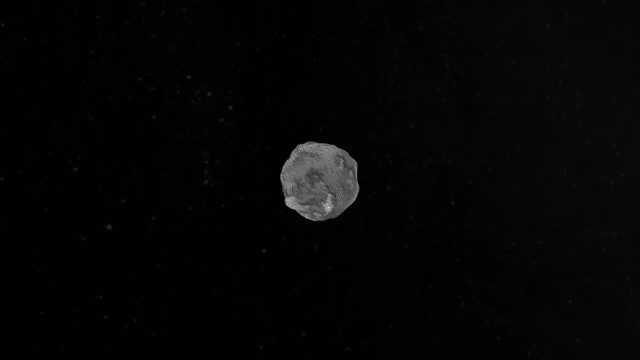 You know what? we've already had: the non-avian thing, paleogene vs tertiary, 65 vs 66, and now this, I'm just going to start a counter. The impact hypothesis posits that 66 million years ago, an asteroid hit the Earth. 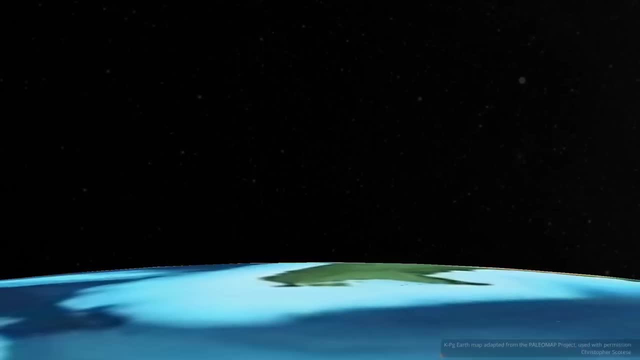 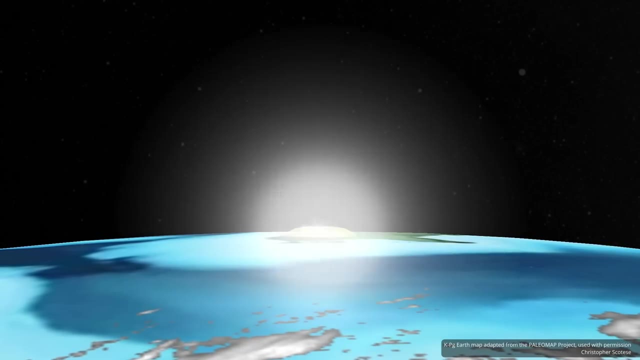 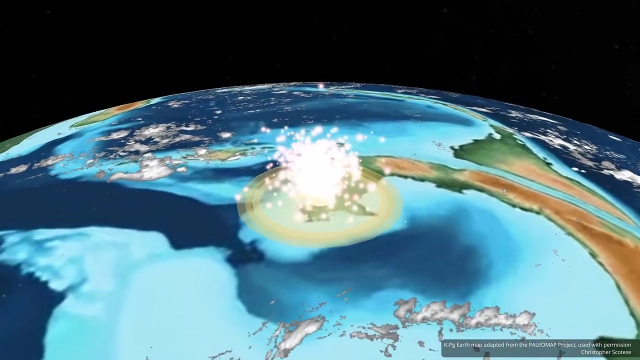 It was around 10 kilometres in diameter, roughly the size of Mount Everest, and travelled fast enough to slice through the atmosphere in seconds. Imagine a mountain travelling a hundred times the speed of sound And imagine the sheer amount of energy its collision would release. 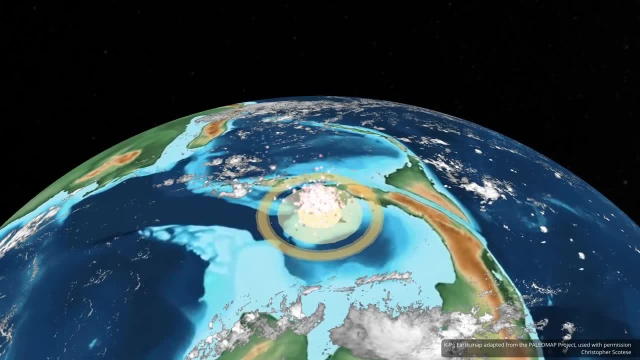 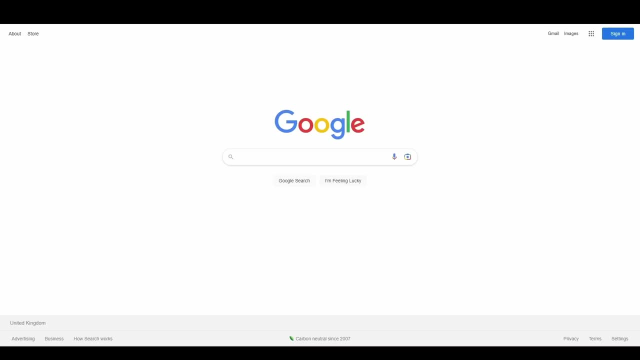 All that energy was taken out on what would become the Yucatan Peninsula in Southern Mexico, Perhaps near the future site of a town called Chicxulub. Chicxulub has become so synonymous with the KPG-Impactor that googling Chicxulub causes this to happen–. WEEEEEEEEEEE, BUSH, BUSH. I am easily amused. Everything nearby was instantly vaporised. This might well have been the largest momentary energy release on Earth for billions of years, and nothing within hundreds, perhaps thousands, of kilometres was surviving that. And that's just stage one. 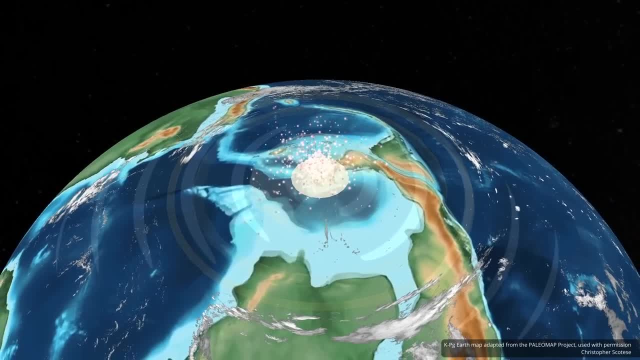 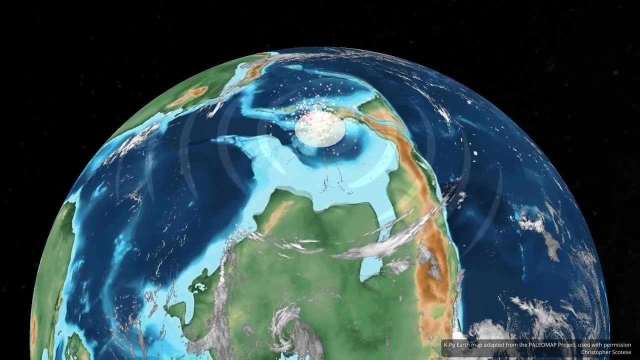 Stage two is the shockwave. As the fireball faded, immense distortion of the Earth's crust caught up and pushed the radius of destruction further still. Earthquakes thousands of times stronger than any in human memory shook the whole continent. Meanwhile, the impact ejector 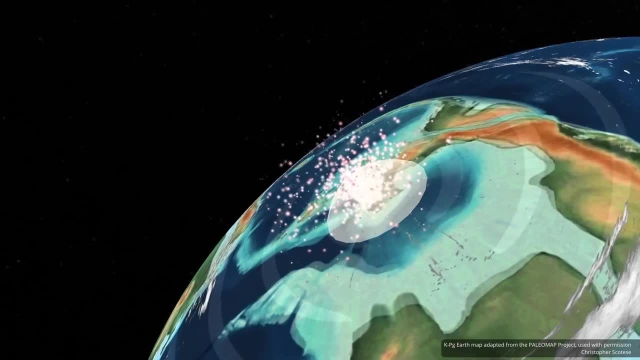 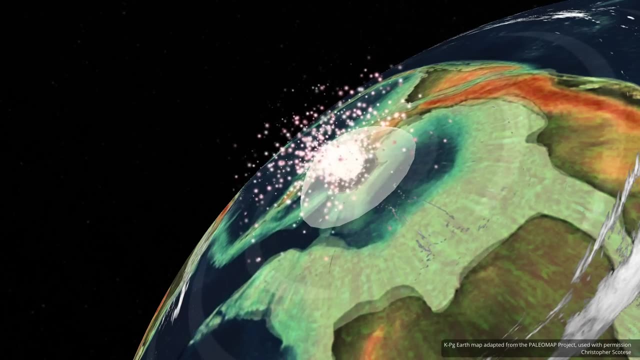 everything thrown up by the fireball arced its way out and back into the atmosphere. Even for those not in the path of the largest chunks of airborne Mexico, the number and velocity of the small chunks superheated the atmosphere, Stifling heat and forest fires. 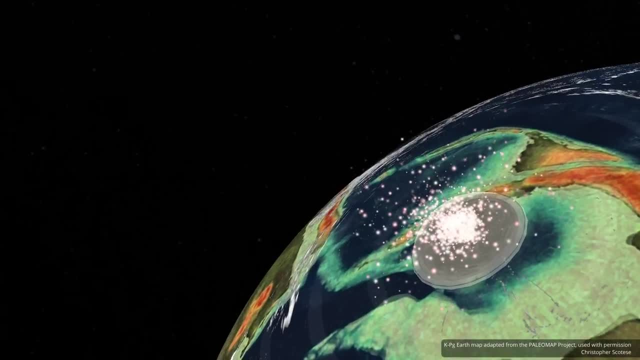 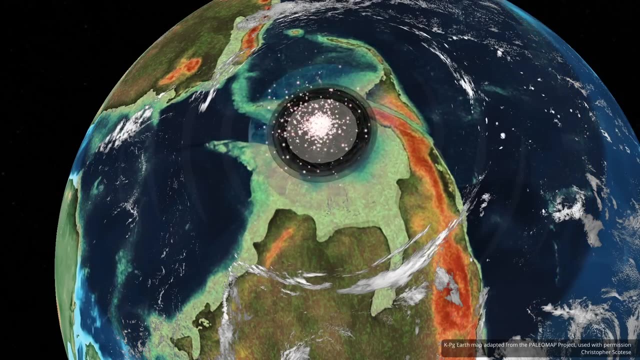 spread across the hemisphere And as half the world went up in smoke. the final stage of immediate death arrived as a tsunami driving churned seafloor and charred debris in the mainland around the Gulf of Mexico. But, contrary to popular belief, 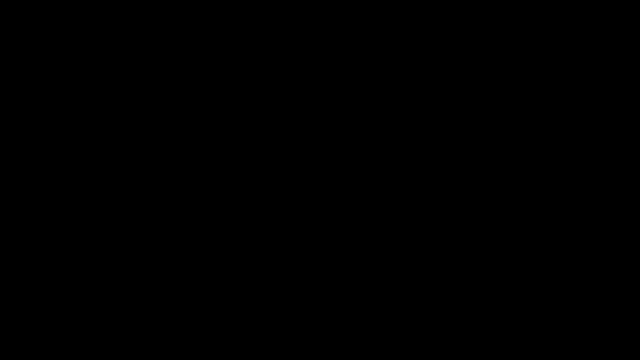 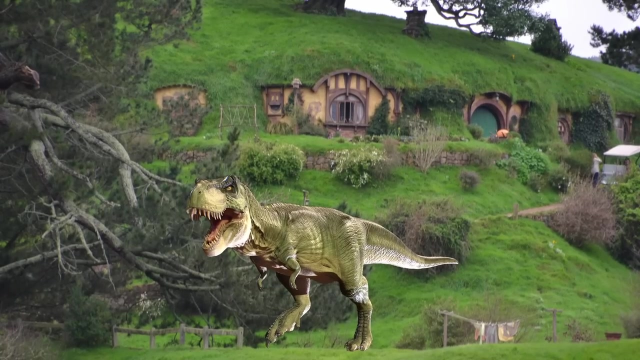 this alone wasn't enough to end the age of dinosaurs. Say, you're a dinosaur in New Zealand, You've experienced at most a slight rumble and everything's pretty peachy. You shrug and go back to normal dinosaur things for a while and then you notice it's getting dark. You look down at 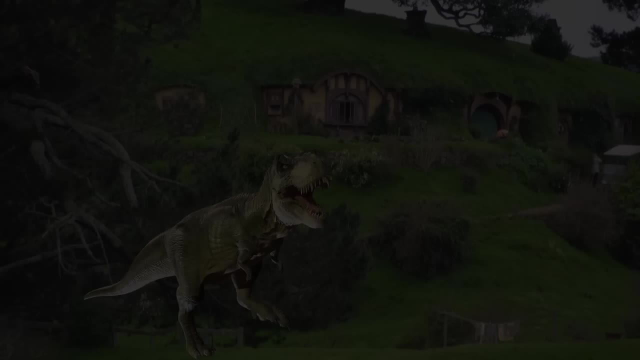 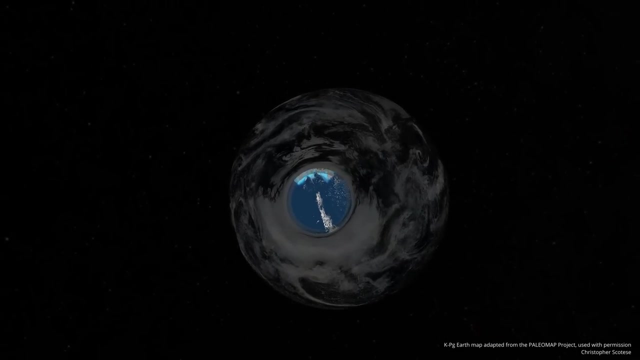 your dinosaur watch and it's only like 3pm and then you look up and you realise a shroud of ash is slowly encircling the entire planet. The real killer in the impact scenario is not the quick, merciful apocalypse in North. 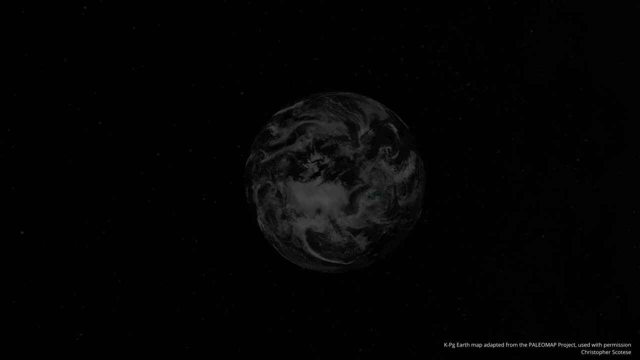 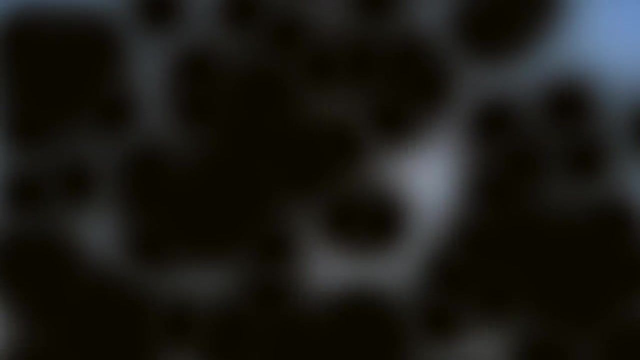 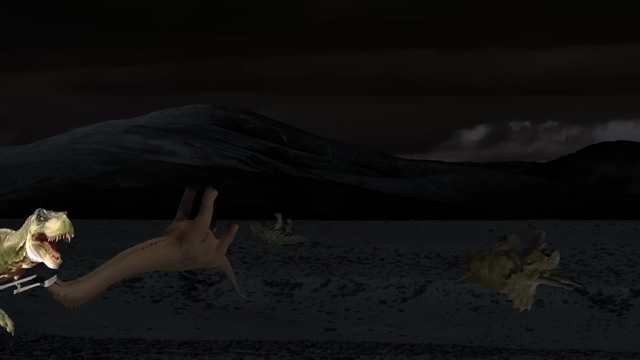 America. It is the slow, chilling grip of worldwide starvation. Impact ejecta infests the upper atmosphere, blocking sunlight for perhaps decades. Temperatures plummet, Photosynthesis shuts down At first. the carnivores are in heaven. on earth, The herbivores have all starved and 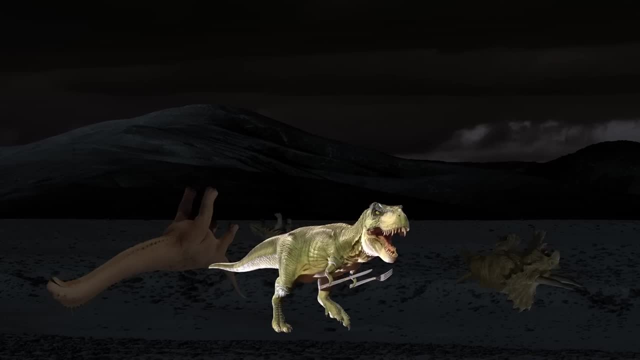 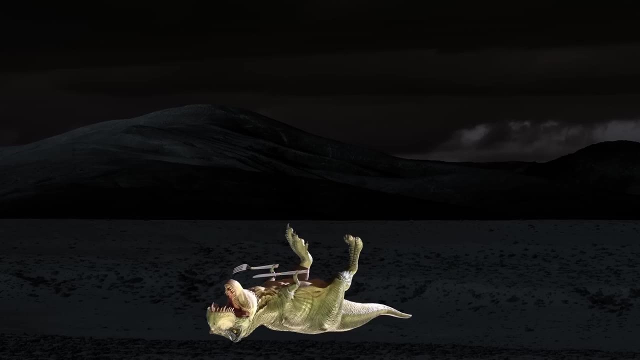 lie strewn across a barren landscape, Easy pickings, But without sunlight to fuel the food chain. this bounty is an illusion. The carnivores too will soon perish. And even after so much death, the ordeal still had one last hurrah. 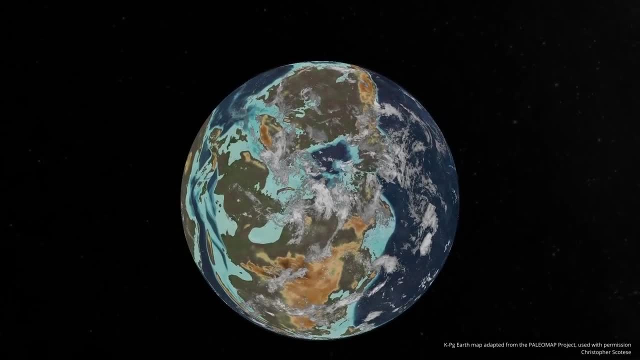 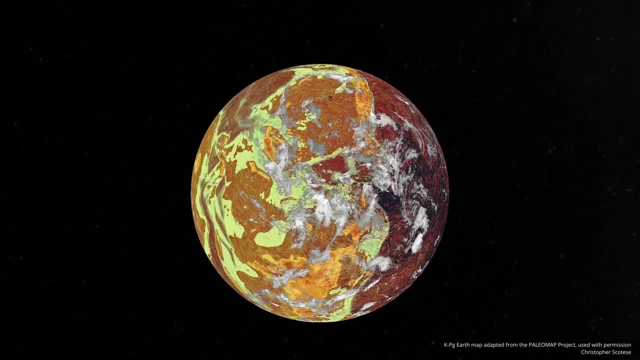 Once the ash had fallen to earth, other atmospheric poisons took over. Carbon dioxide shoveled upwards in vast quantities from the shattered limestone of the gulf's seafloor, sent temperatures careering in the other direction via the greenhouse effect. By the Intermediate Value Theorem, there was a 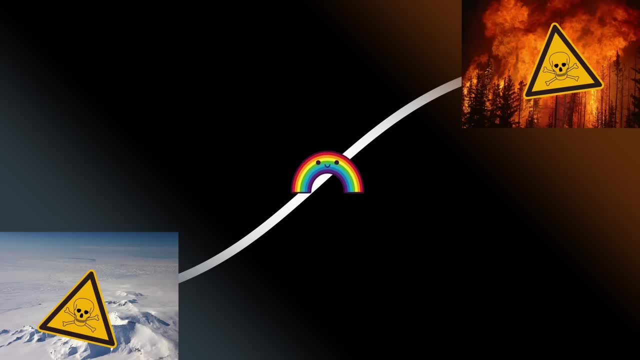 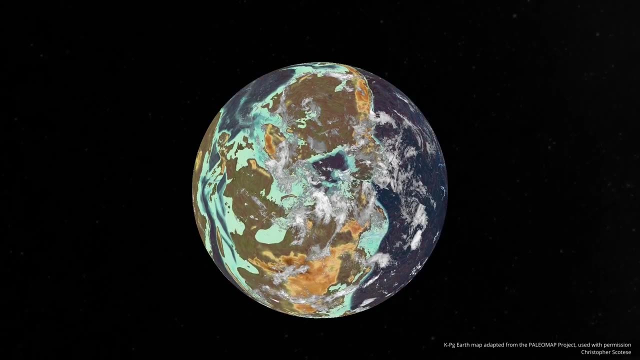 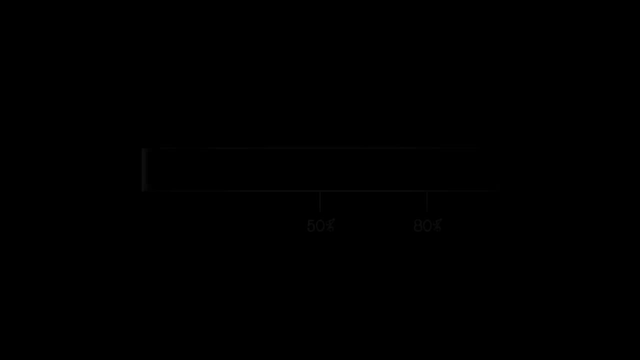 brief moment of pleasant temperatures somewhere in there. You know silver linings. This heating was the final pulse As the CO2 filtered out of the atmosphere. at last, the survivors found themselves in a new and very different era in earth's history. All told, somewhere between 50 and 80% of all animal species on earth went extinct. But this number obscures the true devastation because it only considers species that were 100% eradicated. In terms of individual lives, the figure is much higher. 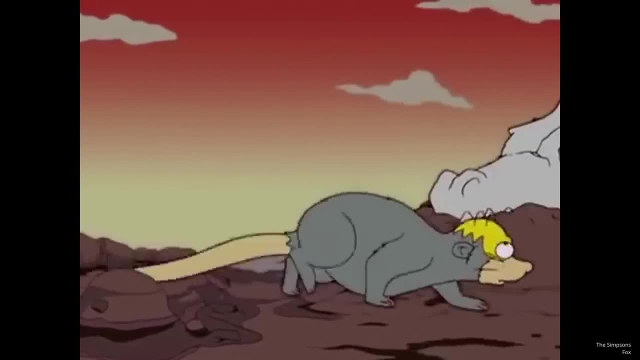 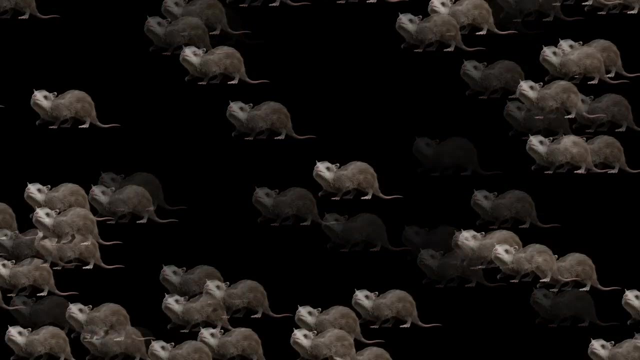 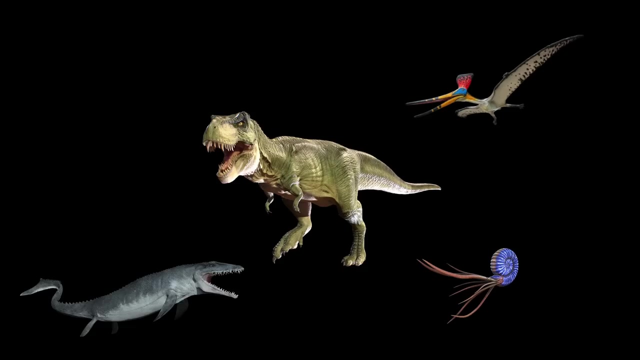 The popular view of hardy mammals crawling free of their dinosaur oppressors is inaccurate, because mammals also suffered heavy losses. The difference is, at least a few did survive All non-avian dinosaurs, all pterosaurs, all marine reptiles, all ammonites and a whole. 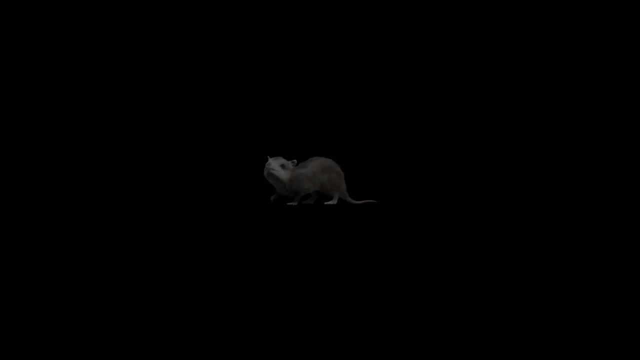 load of other stuff did go extinct. The survivors were mostly small, With efficient metabolisms, generalist diets or safe hiding places. Even then, plenty of species with these traits died off too, so maybe a lot of it came down to luck. 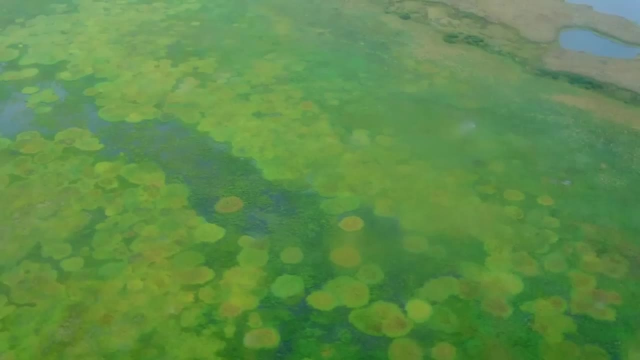 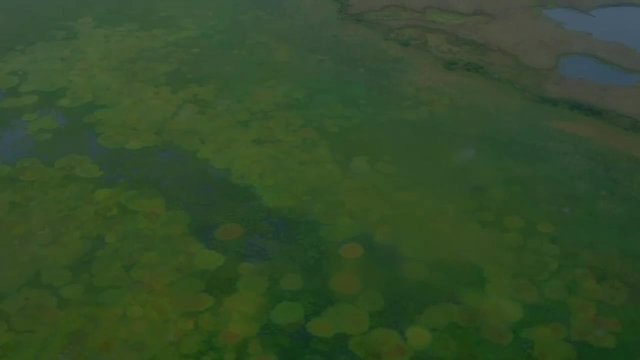 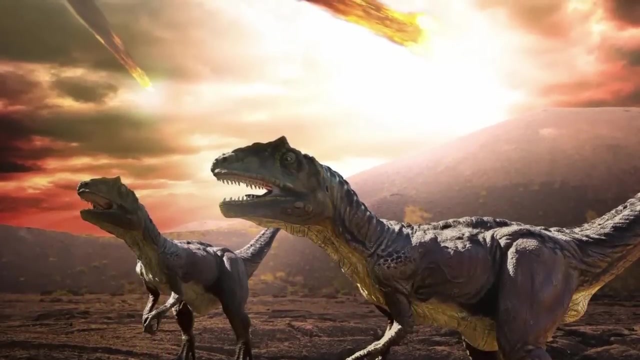 Land plants made it through thanks to their secret weapon seeds and, amazingly, a few species of oceanic photosynthesizers scraped through the darkness Just enough to rebuild food chains in the world to come. Only then were the effects of earth's chance encounter with a big space rock so many years 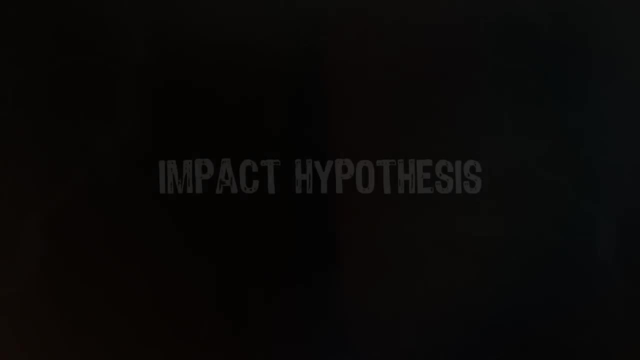 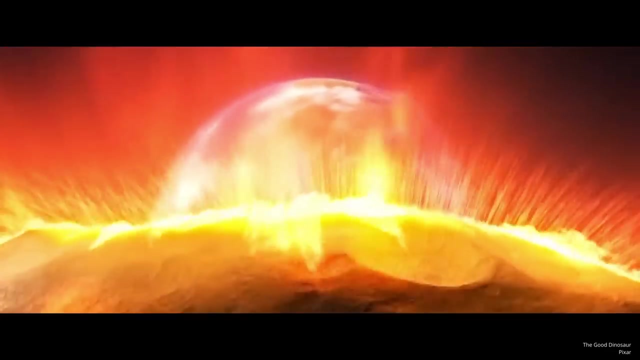 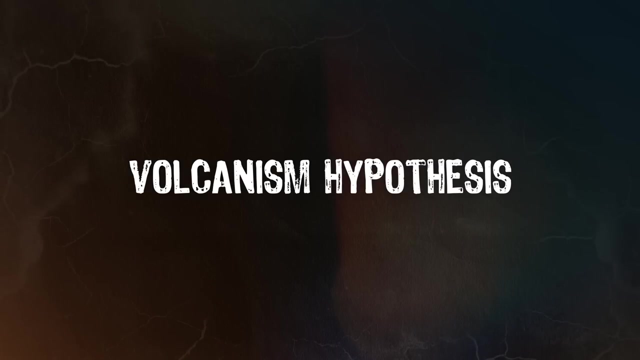 earlier forgotten. The impact hypothesis paints a high-resolution picture of an intense descent into hell, spurred by a single day, A single catastrophic event that so easily could have never happened. The volcanism hypothesis is less sudden, but no less hellish. 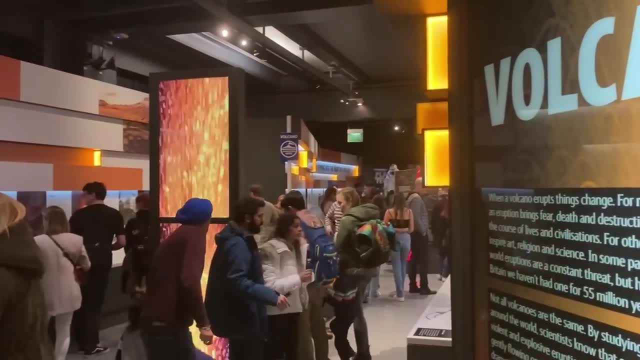 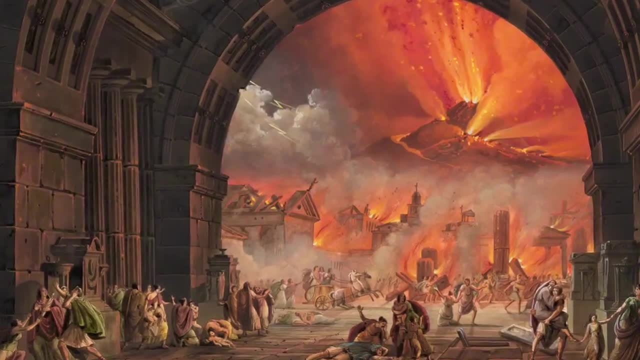 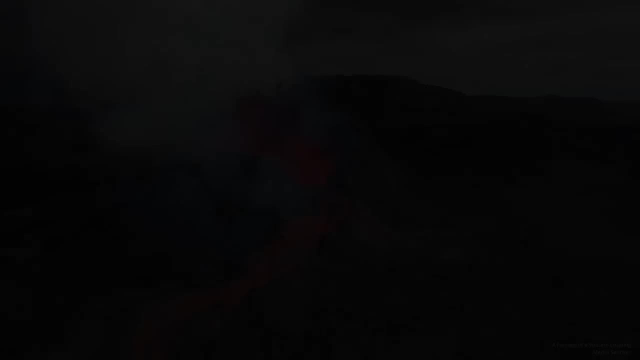 Unlike asteroids, volcanoes have been a known entity throughout history. Awesome destructive potential fuelled by upwellings of molten rock, pressure building in underground cavities until the very end The top explodes with sufficient power to level cities. Yet KPG volcanism relies not on these abrupt eruptions, but a different type entirely. 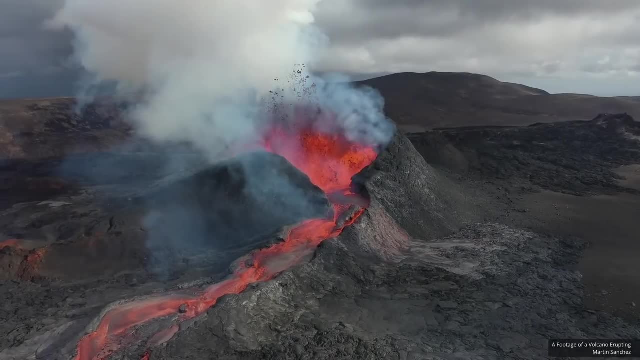 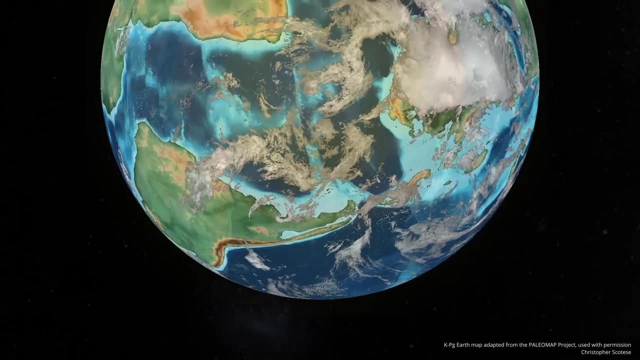 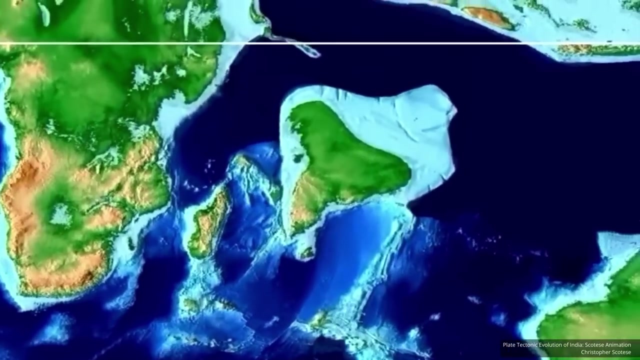 A slower, subtler foe with the power to choke a planet. According to the volcanism hypothesis, a million years or so before the KPG boundary, the Earth's interior underwent a dramatic shift below the future Indian subcontinent. India at this time was an island speeding its way across the ocean, destined one day. 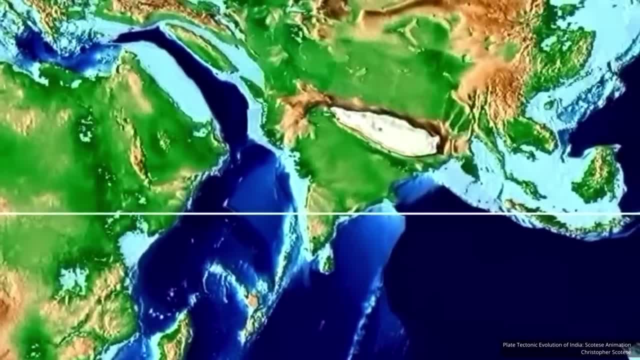 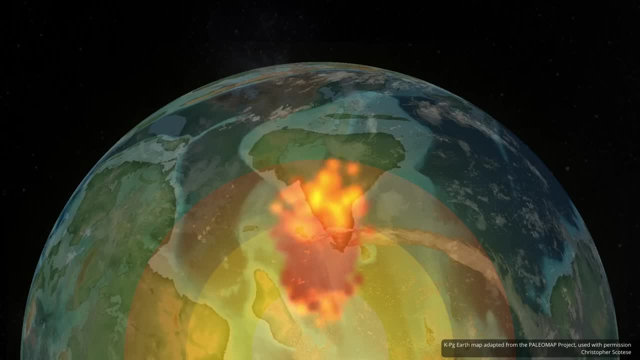 to crash into the rest of Asia and form the Himalayas. Underneath this island, a mantle plume was forming An enormous current of rock, bringing heat from the planet's core closer to the surface than usual. A similar thing is currently happening in Hawaii. The isolated island chain is believed to be fuelled by a thank-y-bly much smaller mantle plume. Volcanoes resulting from a mantle plume don't tend to be the explodey kind. They're more the constantly spewing out hot liquid like a salivating dragon kind. 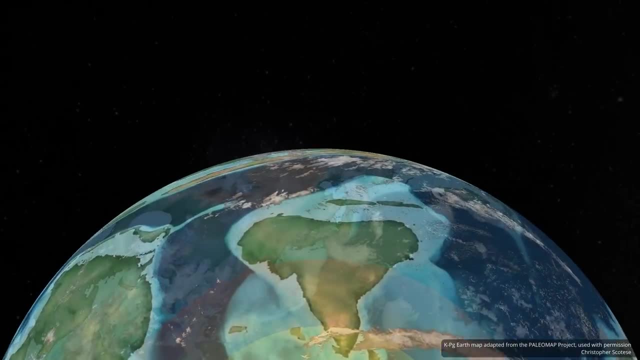 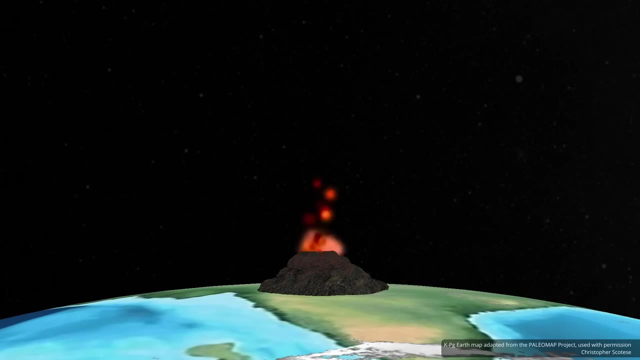 The lava is a constant constantly spewing out hot liquid like a salivating dragon kind. The lava is a constant constantly spewing out hot liquid like a salivating dragon kind, And on the scale of the K-Pg plume. this was bad news for the dinosaurs. 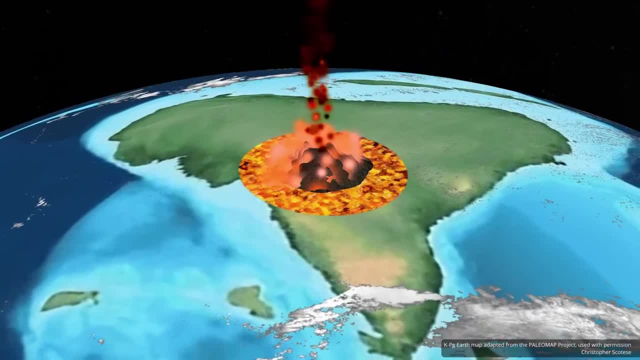 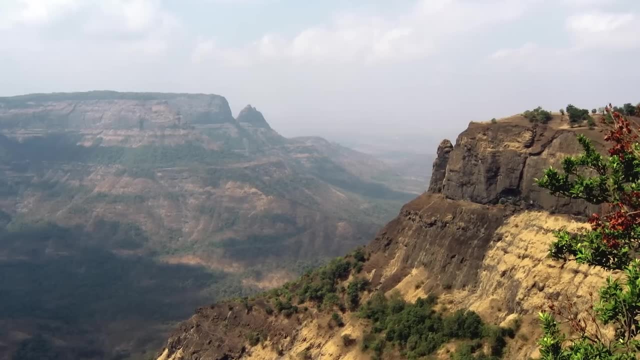 For perhaps hundreds of thousands of years, India became an ocean of lava. A million cubic miles of the stuff seeped inexorably through the crust. The solidified remnants of this flood basalt eruption are known as the Deccan Traps. 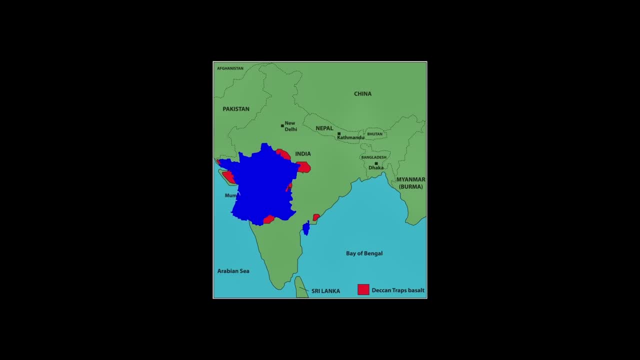 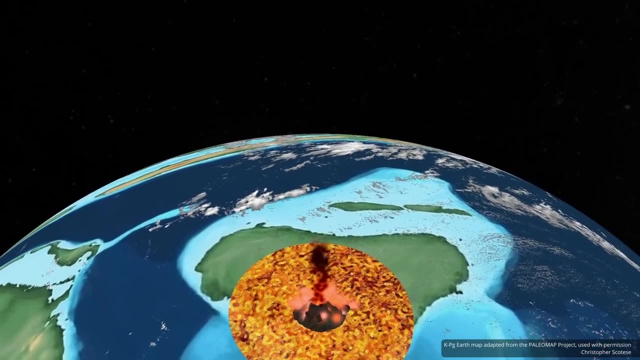 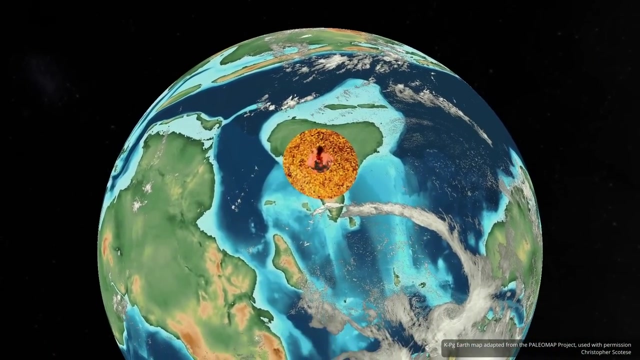 They're up to two miles deep and cover an area the size of France. But much as in the impact scenario, this localised destruction was far from the true apocalypse. Once again, it was atmospheric contamination that proved fatal. Two gases, sulphur dioxide and carbon dioxide, seeped from the fissures unyieldingly. 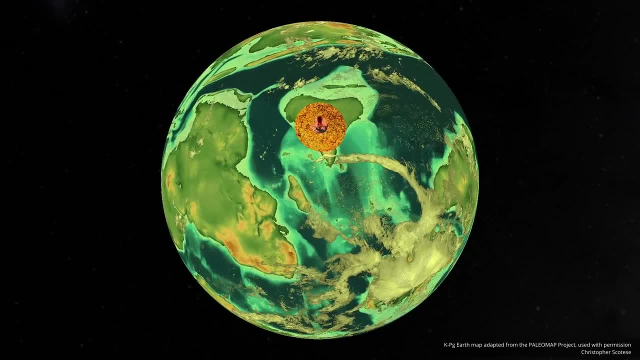 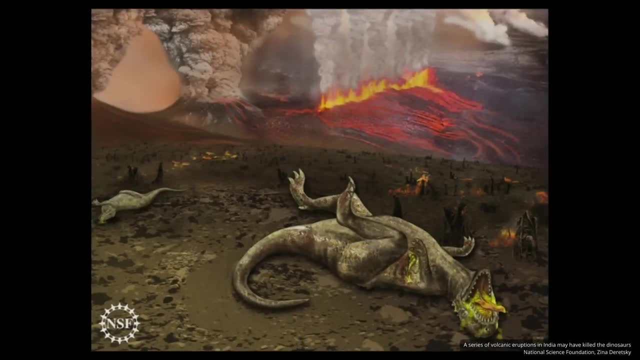 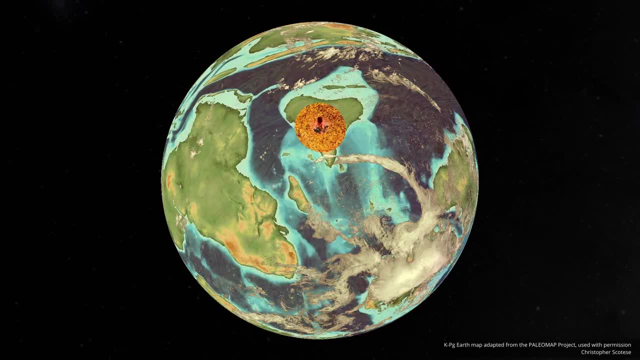 The lava was a constant, constantly spewing out hot liquid like a salivating dragon kind. The lava was a constant, constantly spewing out hot liquid like a salivating dragon kind, And once the sulphur dioxide had filtered out, carbon dioxide took over again driving. 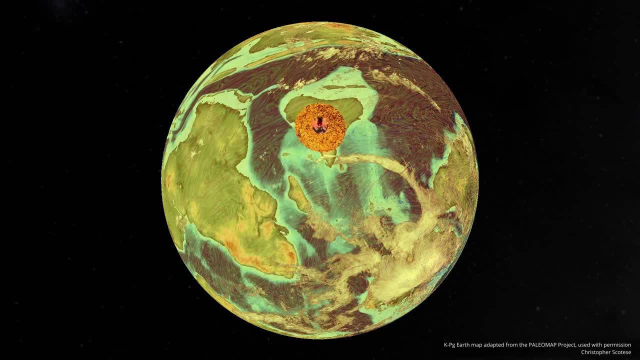 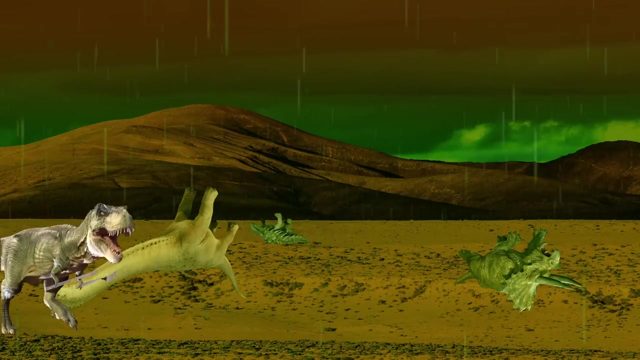 climate change in the other direction. Until the next massive eruption spewed out yet more sulphur. Each pulse in isolation had geophysical checks to counter it, But so many for so long proved too much for the Earth. This cycle of constant environmental chaos, wringing and strangling stressed ecosystems. 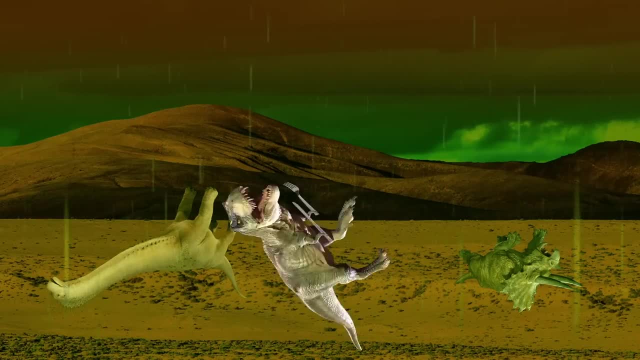 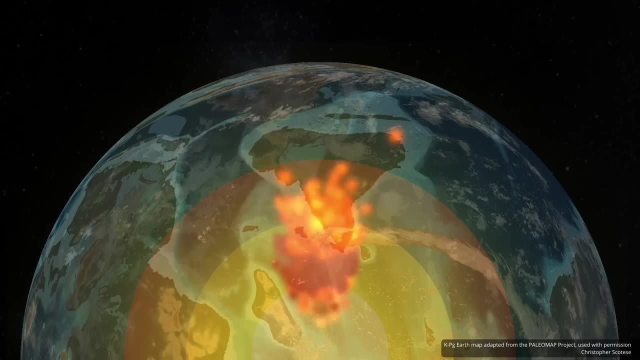 to breaking point. One by one, food chains cupped, collapsed, species went extinct and we end up with a total extinction profile that matches that of the impact hypothesis. Only the fortunate retreat of the mantle plume ended the event. After one last massive encore of fire and toxins at the KPG boundary, the volcanoes subsided And 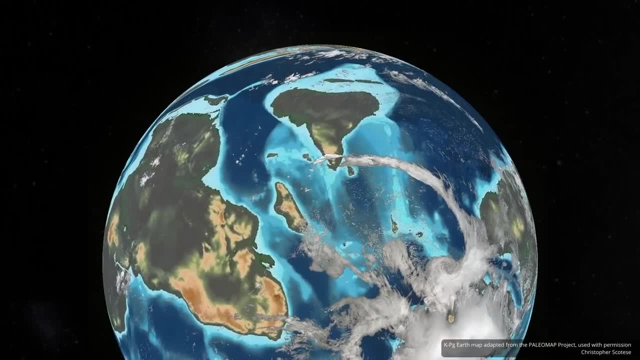 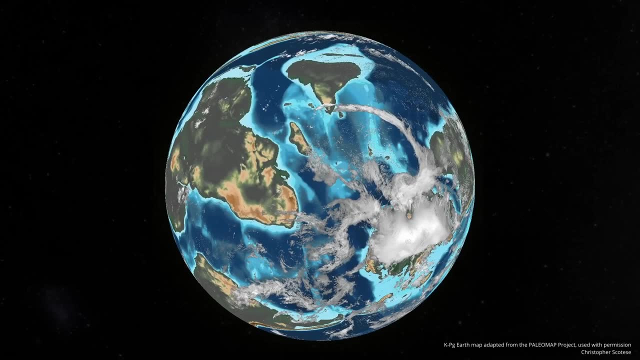 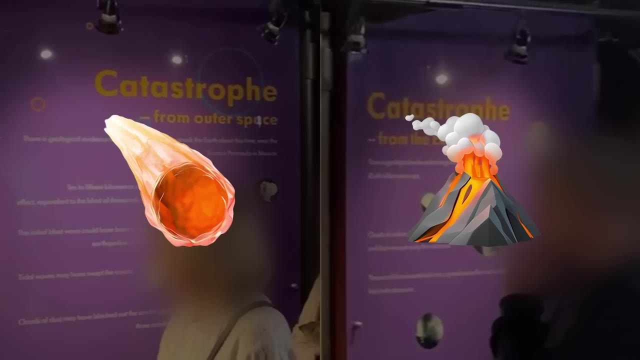 just as in that alternate history of asteroid-induced extinction, the dinosaurs were gone and the small, hardy, lucky survivors were left to repopulate a desolate planet. As we'll see later, these are far from the only theories behind the extinction of the dinosaurs. 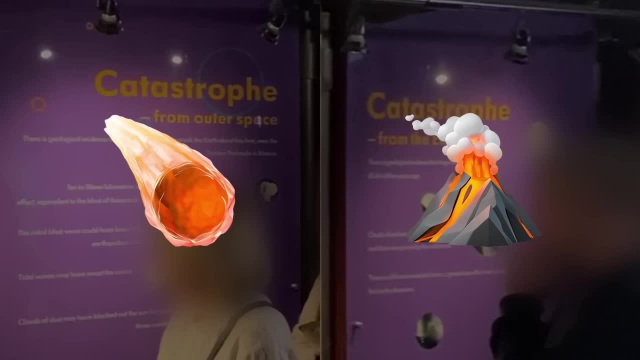 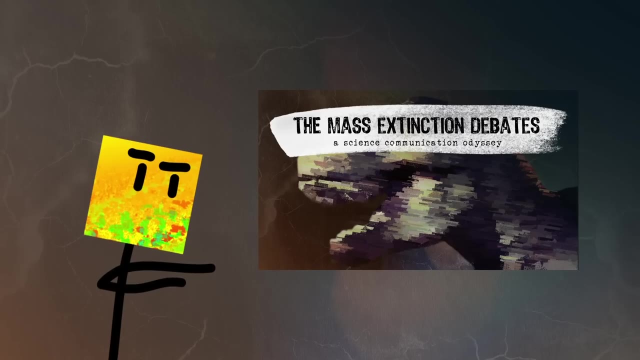 although they are the most significant to modern paleontology. But here's a tricky question Which, if any is correct- And by tricky I mean- requires most of the rest of this absurdly long video to answer. like seriously, thanks for being measured in geological time at this rate, The cliff notes. 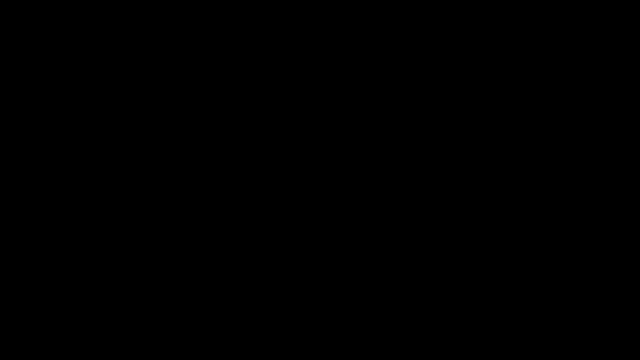 are as follows. There are three evidence-supported facts which all experts in relevant fields in 2023 agree on. The non-avian dinosaurs and many other species went extinct around 66 billion years ago. A large asteroid hit Chicxulub around 66 million years ago. The Deccan Traps erupted around 66. 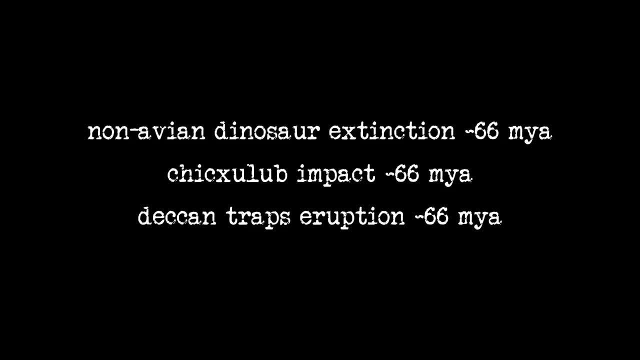 million years ago. To say anything beyond that, anything about the exact chains of events, how they're related or any other factors, strongly depends on who you ask and what counts as consensus. But if you ask me to make a judgement based on my own research, again big rabbit. 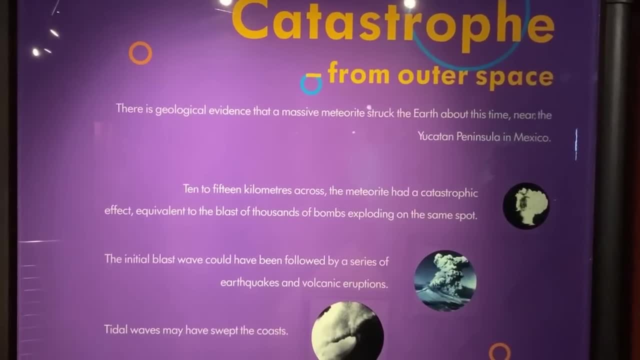 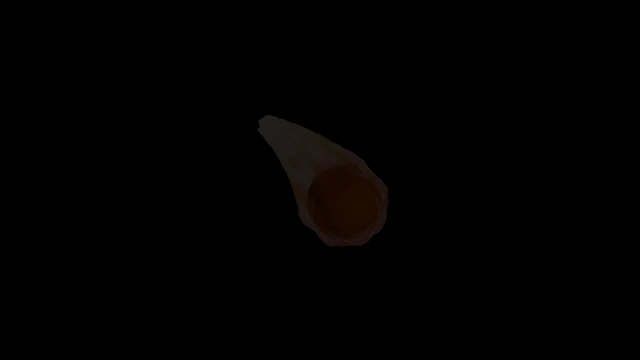 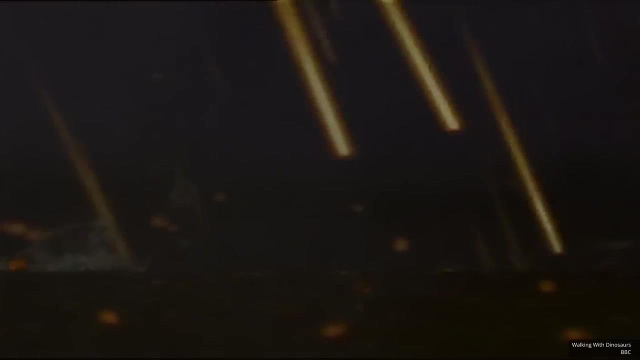 hole there. we'll return to you later. scientific consensus comes down on the side of the asteroid Death from space. it is. So if that's what the science thinks, how does that translate to what you think? What society as a whole thinks? Counter-intuitively, given our other issues with 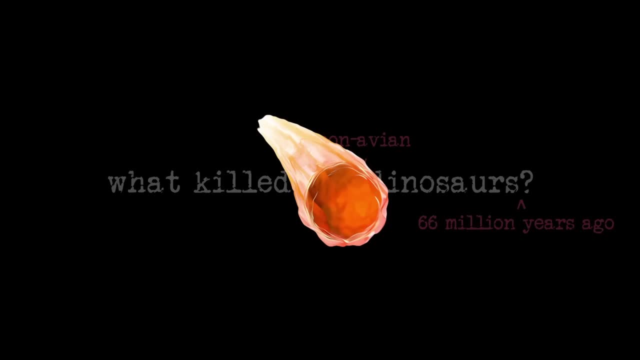 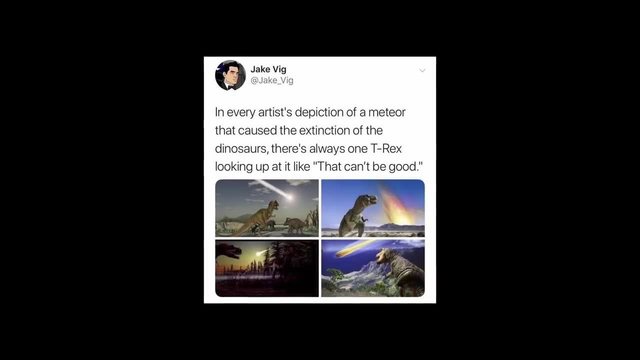 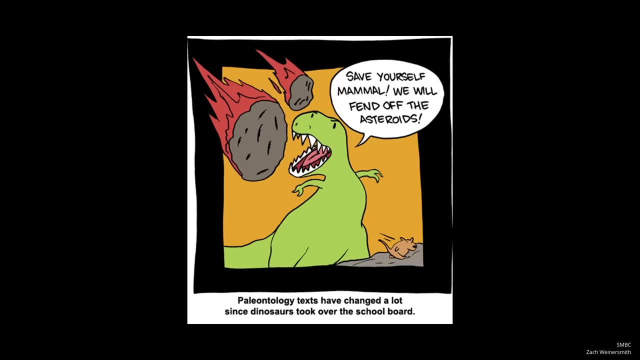 this question. it appears asteroid wins out. here too. Agreement, Incredible Science communication works. It's not hard to speculate that the impact hypothesis has become ingrained in our collective understanding of dinosaurs. Think dinosaurs, think asteroid. The idea has become rhetorical shorthand. 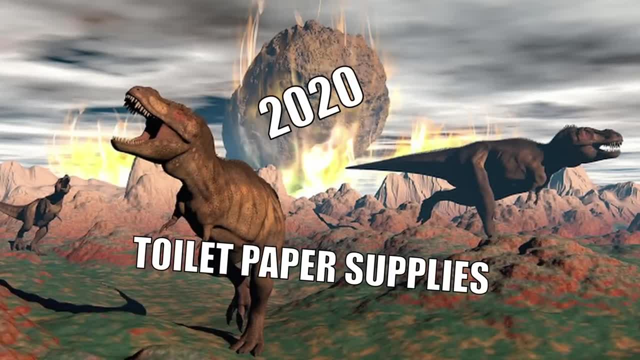 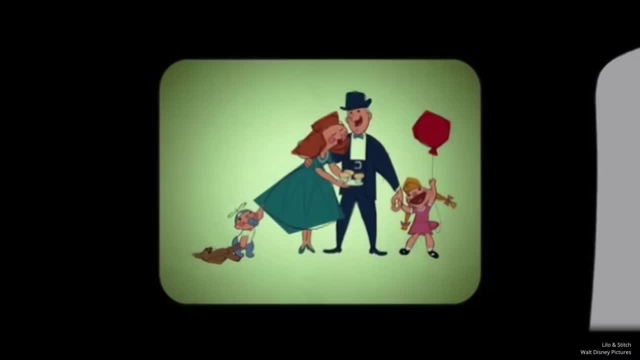 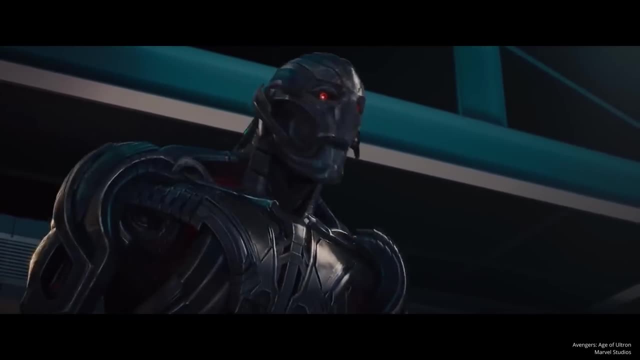 for a dominant paradigm, suddenly and without warning displaced by a dramatic event. But don't worry, I won't sink to that cliché anywhere in this video. Look at cinema, for instance. Films with zero connection to asteroids or dinosaurs present the event as fact or employ it as heavy-handed metaphor. 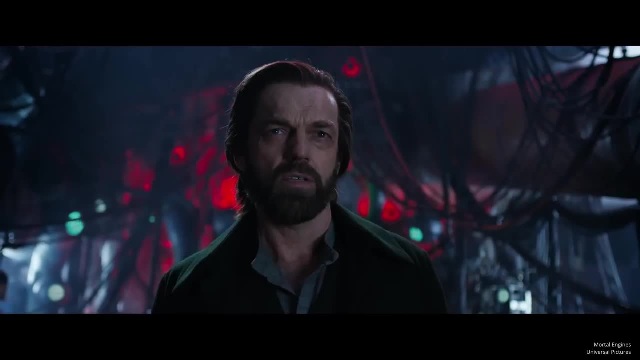 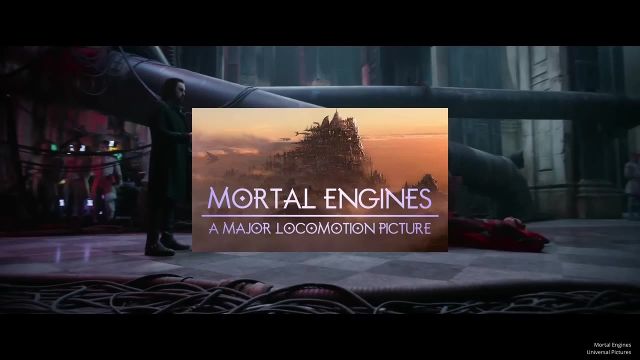 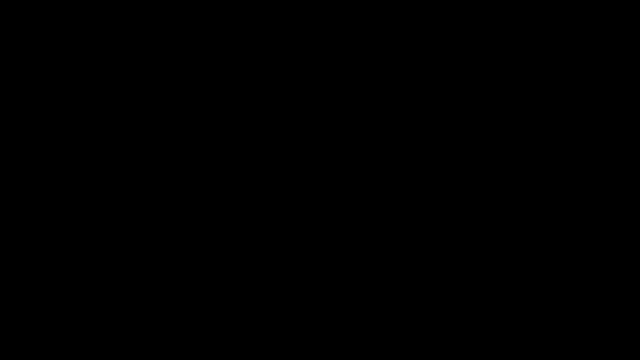 You're a relic of a dying age, A dinosaur. I'm the meteor. Can't believe I forgot the worst line of that film in my review. But are a few movie lines and unsubstantiated claims about public opinion really the best evidence? No, I needed data. While there's no shortage of reviews of expert opinion, 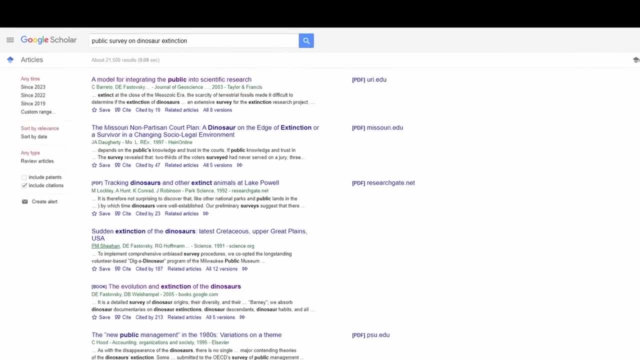 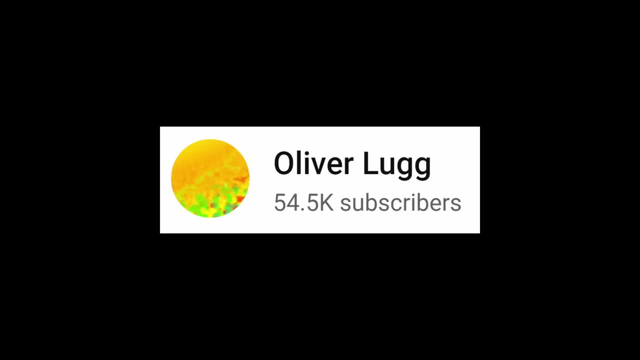 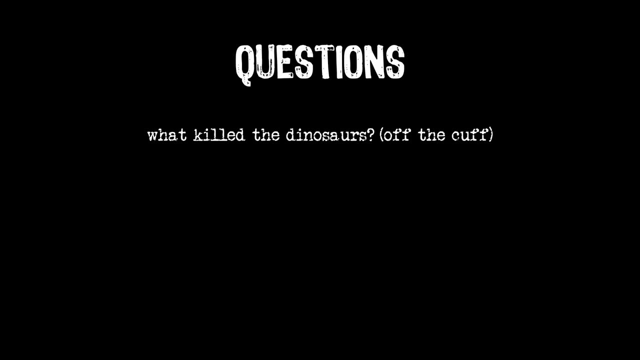 I found data lacking when it came to the public's beliefs about dinosaur extinction. Luckily, I happen to have my own segment of the public to exploit for research purposes. I put out a survey for my subscribers to see if that could gauge public consensus. Five simple questions. What killed the dinosaurs? Please answer off the top. 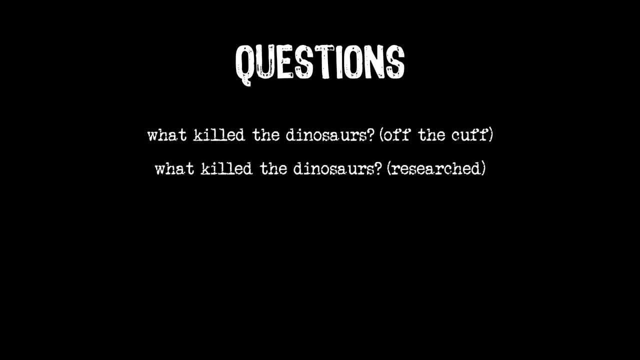 of your head? What killed the dinosaurs? Please research before answering. How old are you, Which country are you from And how interested and knowledgeable are you when it comes to dinosaurs and paleontology? It's important first to note the likely sampling bias here Given YouTube's. 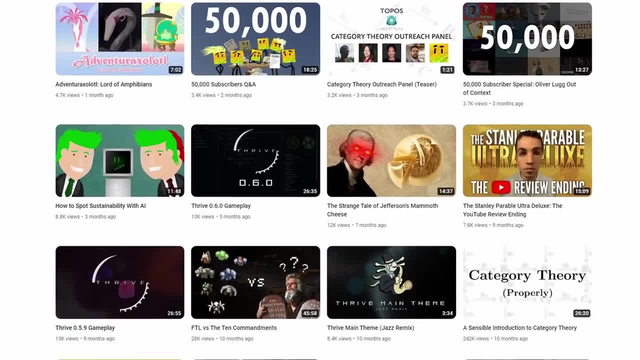 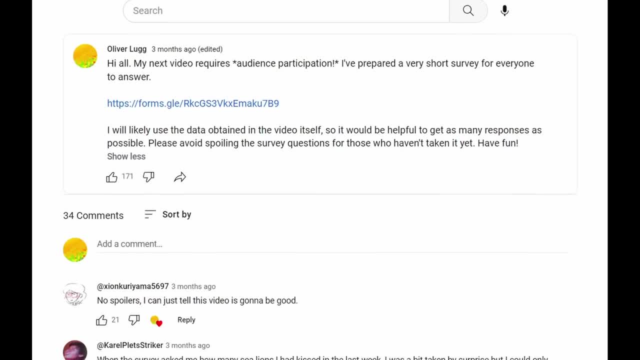 demographics and my channel's past and future. I don't think I'll be able to answer that question. I expected a bias towards respondents who are young and from English-speaking countries with above average interest in STEM fields, And despite attempts to hide the subject of 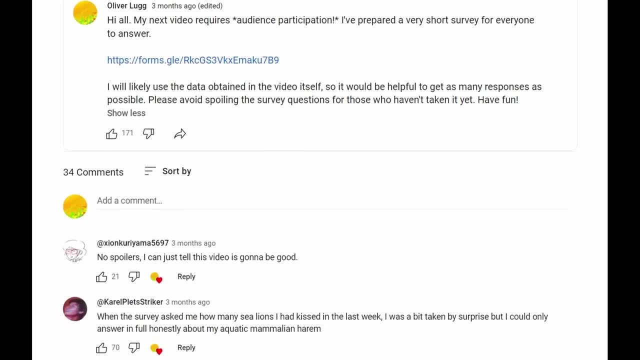 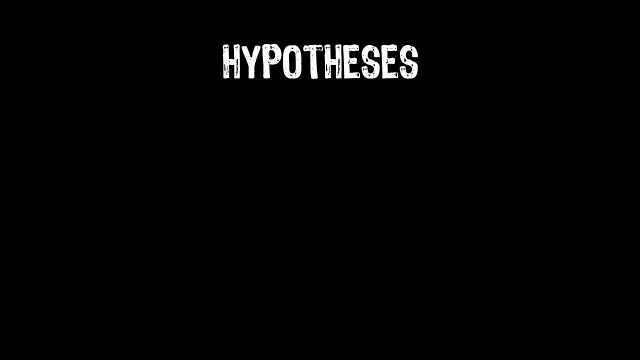 my survey. whenever posting it, I expected a fair degree of self-selection bias, both in terms of interest in answering random surveys and interest in dinosaurs. And while we're on the topic of doing research properly, I should note I made several hypotheses before conducting the survey. Off-the-cuff answers strongly favour asteroid as the single cause. 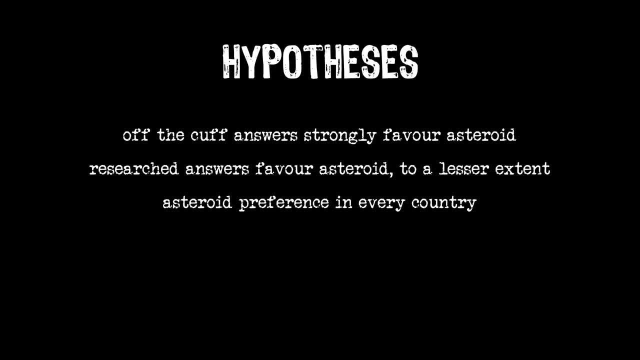 Researched answers favour asteroid, but to a lesser extent. Preference for asteroid is present across all countries. Preference for asteroid is present across all age groups, with a stronger effect in younger groups. Preference for asteroid is present across all interest levels with a stronger effect. 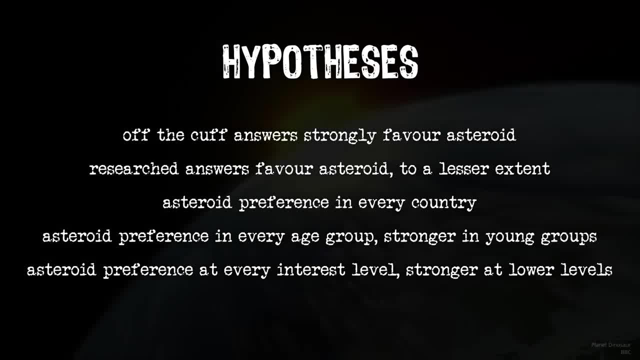 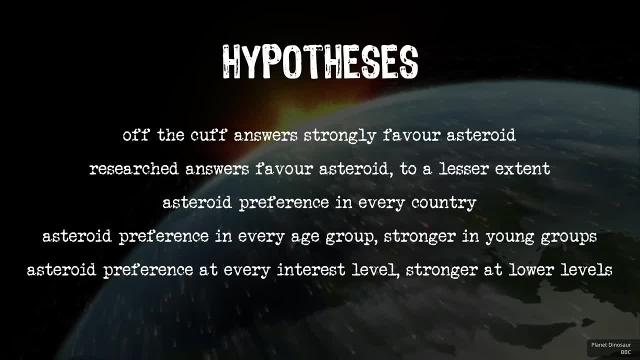 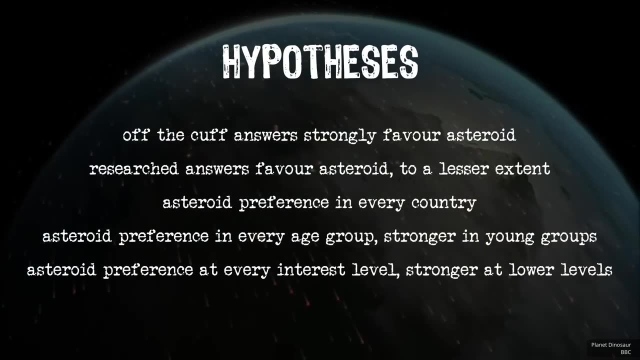 in those less interested. Essentially, I thought asteroid impact would be favoured as the single cause in any group, but that older groups, those with more expertise and those who had done research would show more recognition of the nuance. I hope that by the end of this video you'll understand why I singled out those parameters. 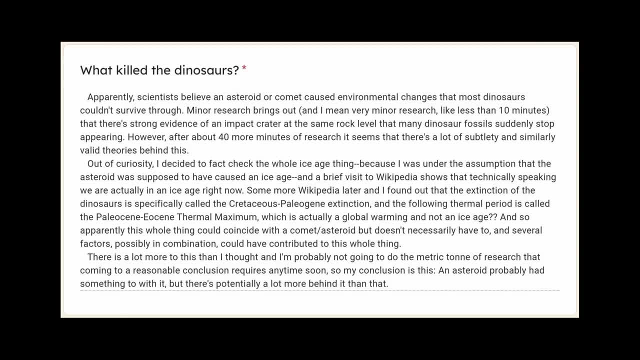 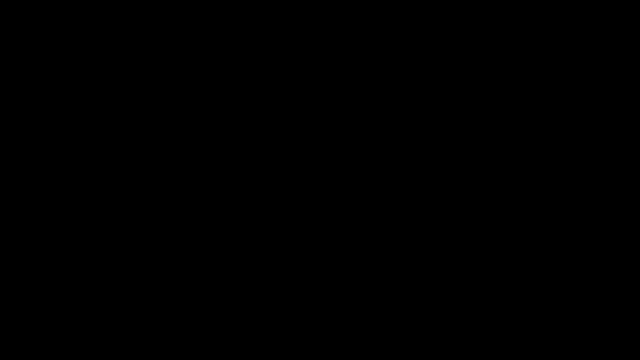 Classifying answers proved a bit of a nightmare. Giving people the freedom to write anything while necessary led to a lot of headaches, But I did come up with a system which I'll quickly run through for transparency. Obviously, the whole asteroid-comet-meteor. 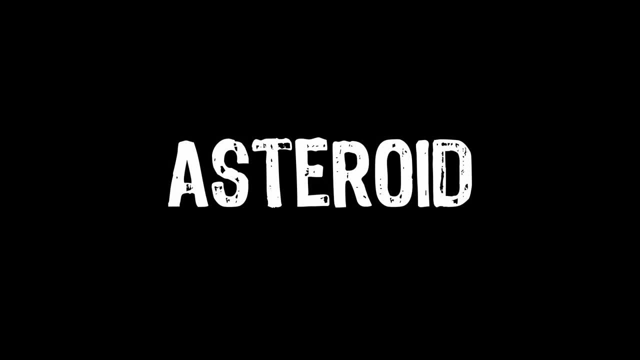 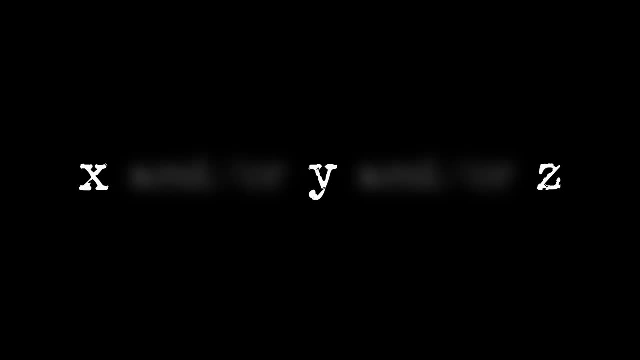 debacle got crushed into one answer and the same for some other things. If someone gave two or more factors with a clear causal link between them, I classified their answer according to their answer. So asteroid begets ash begets. starvation became asteroid. If I couldn't establish a causal link, I combined the listed factors using AND-OR. Note this didn't. 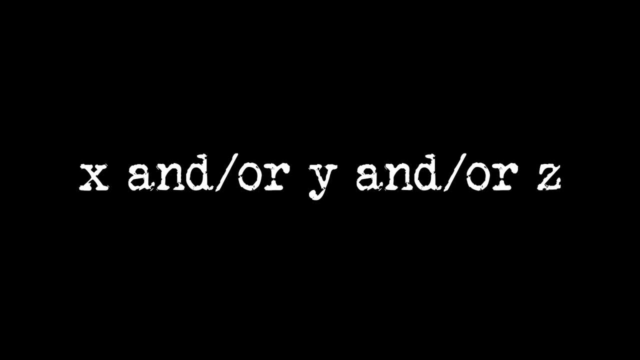 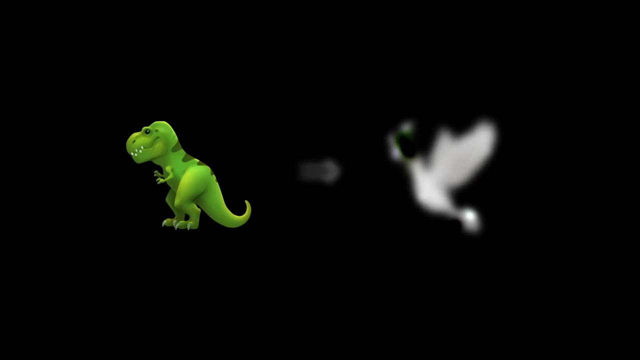 distinguish AND from OR, and it didn't express how prominent each factor was. in their answer, Answers which mused on a few things before settling on a conclusion, became that conclusion, and I specifically omitted mentions of evolving into birds, except where that was the only factor given, because I wanted to focus on the extinction and 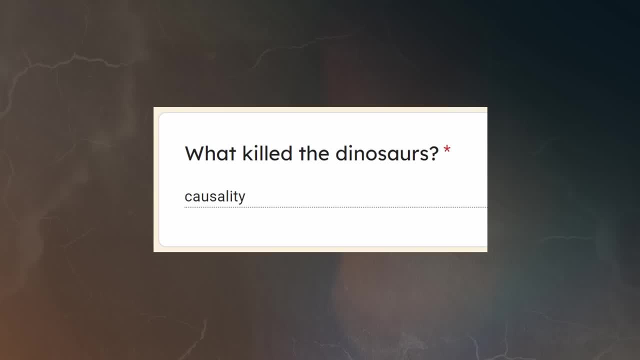 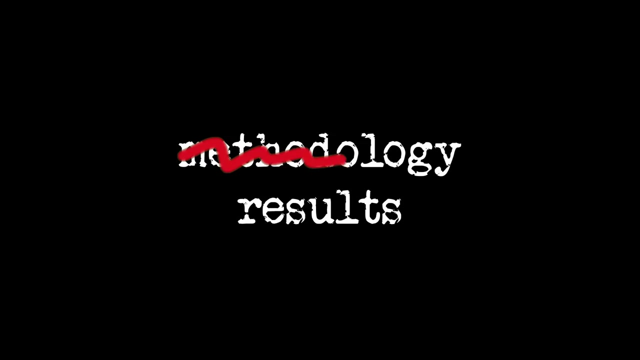 not the well actually aspect of the question. I also didn't filter out joke answers: A because it was often hard to tell the difference, and B because I wanted my proportions to reflect the entire sampled group. Still not sure if that was the best idea. That covers the methodology, so 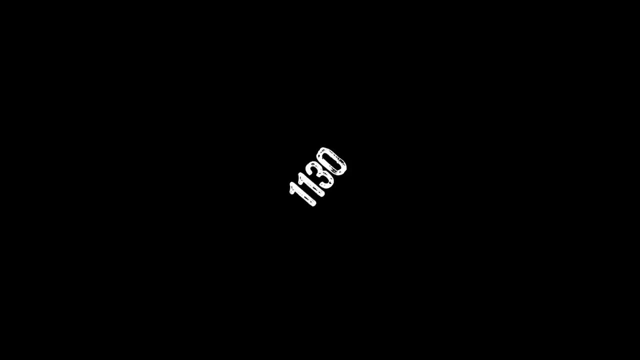 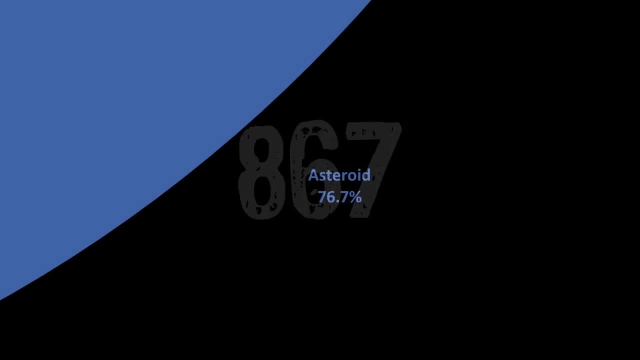 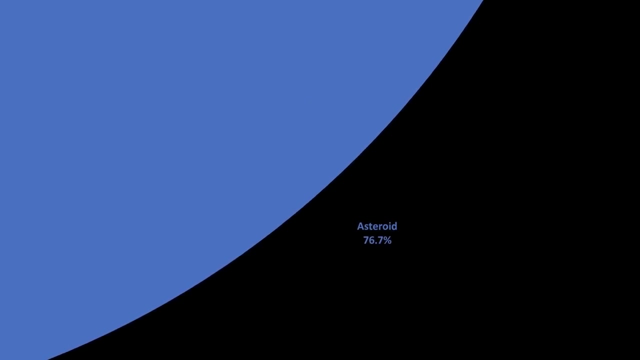 let's get to the exciting bit: The results. I received 1,130 responses Of these, 867, or 77% they're off-the-cuff source of Dino Doom. That's a strong majority, right? I was expecting higher. 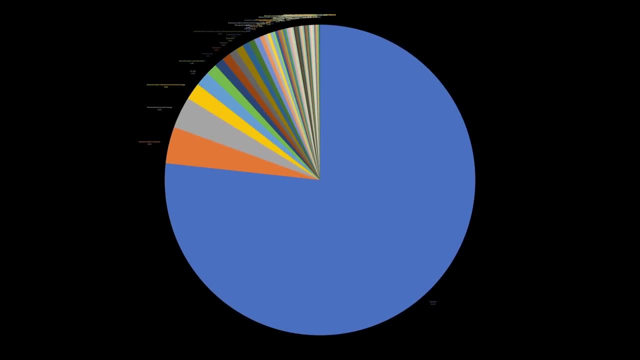 in all honesty, and I was surprised at the number of answers that mentioned neither asteroids nor volcanoes- It seems, like many scientists, I had overestimated the public's knowledge of my subject area. Unlike many scientists, I had underestimated the public's memory of the 1997 film Batman and 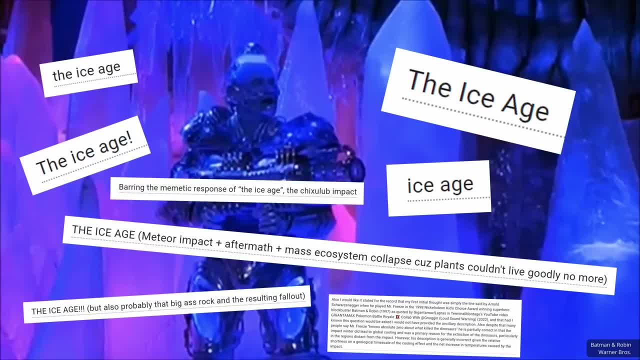 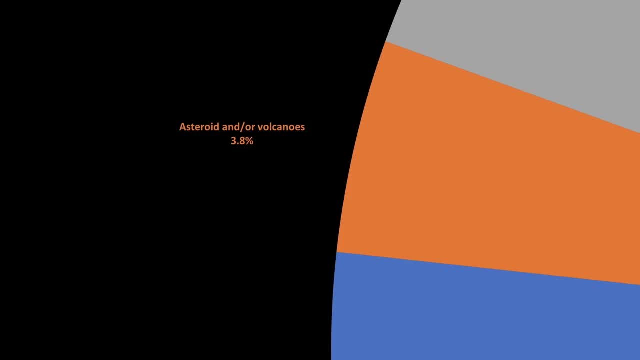 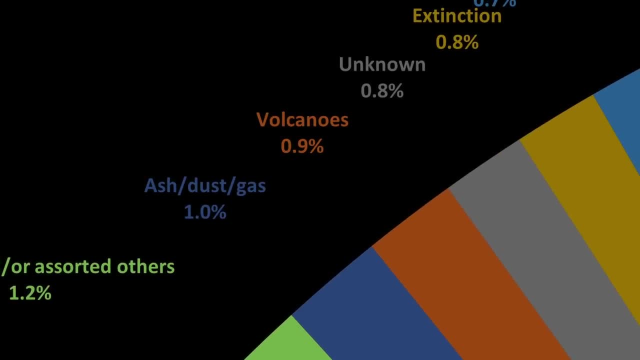 Robin, What killed the dinosaurs? The Ice Age, Second to asteroid, was asteroid, Asteroid and or volcanoes, with a pitiful 3.8%. Volcanoes on their own came way down in eighth with 0.9%, That's 10 people. For comparison, nine people said dinosaurs were killed by extinction. 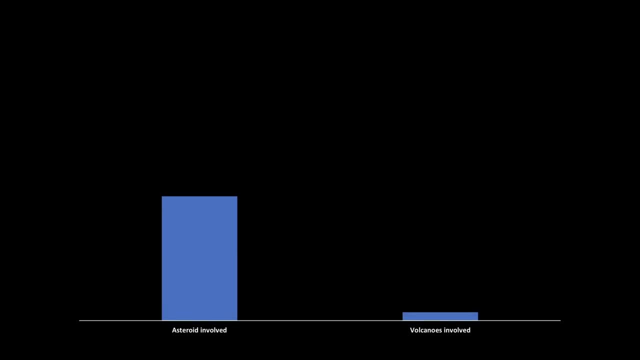 Just extinction. If you're concerned about the first-past-the-post approach here, don't worry. I've considered that. Responses mentioning asteroids as any factor came to 85% compared to 5.8%. Some improvement for volcanoes there, but yet more asteroid dominance. 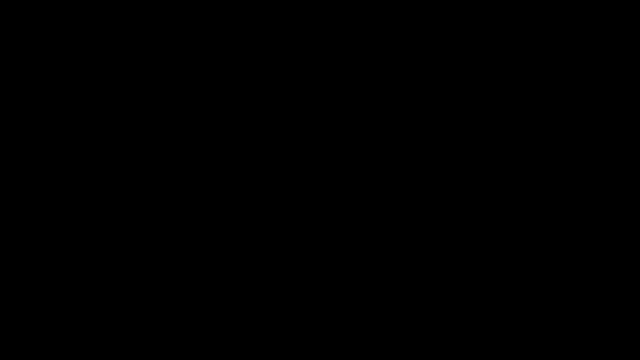 What, though, happens if you ask people to look something up before answering? Well, you get some people who've put hours into a properly sourced, well-written argument, and you also get: I've already done research, bro. I'm too busy for this shit. 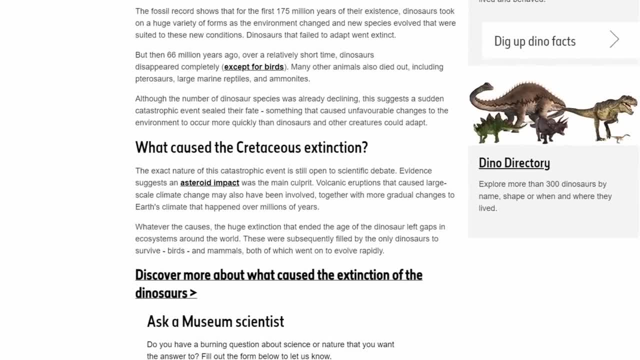 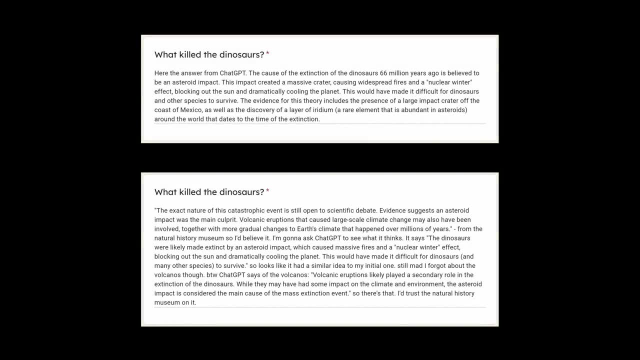 You get 21 people quoting the Natural History Museum verbatim, 13 of whom did so without credit and clearly thought I wouldn't recognise it, and you get TWO people asking Chat GPT, producing answers that only mention asteroids without extra prompting. 58% of respondents this time gave answers boiling down to asteroid. 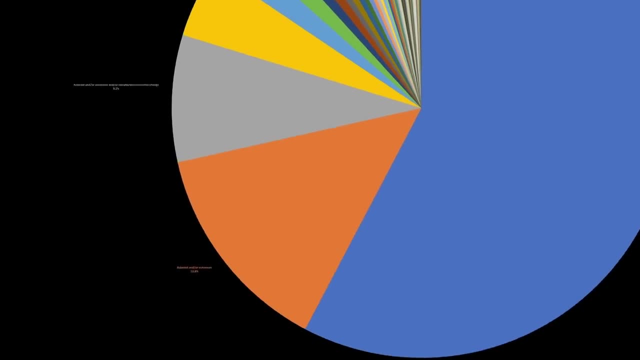 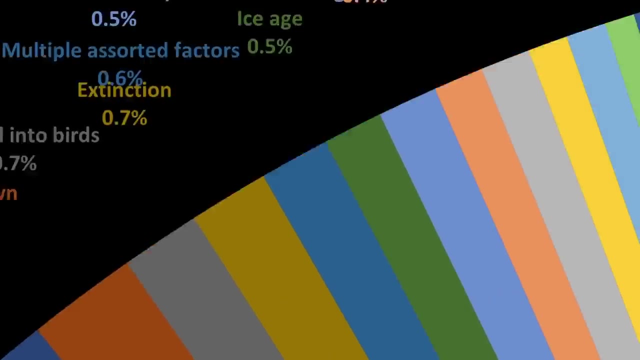 Still the majority, but a sizeable drop. Asteroid and or volcanoes remained in second, with an increased representation of 14% Volcanoes on their own lost support, dropping to 0.4%, Although in alternative data these two had 1%. 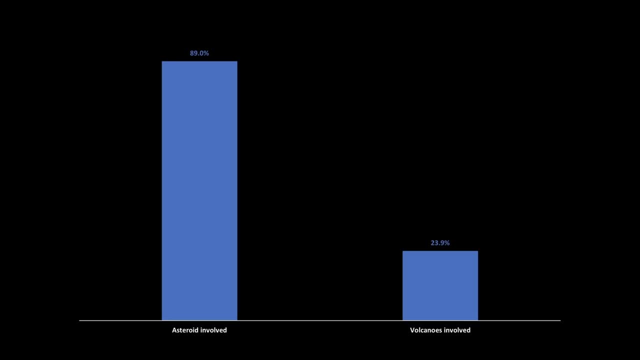 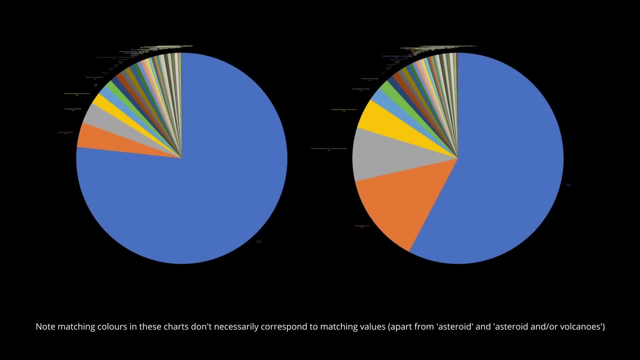 When asked about幹嘛- transitions between asteroids, they both answered the following ones: Alternative vote: world volcanoes did better. Asteroid share also increased. A quick interpretation of these results suggests research is likely to make people more aware of the volcanism theory, but not more likely to support it. They are, however, much more likely. 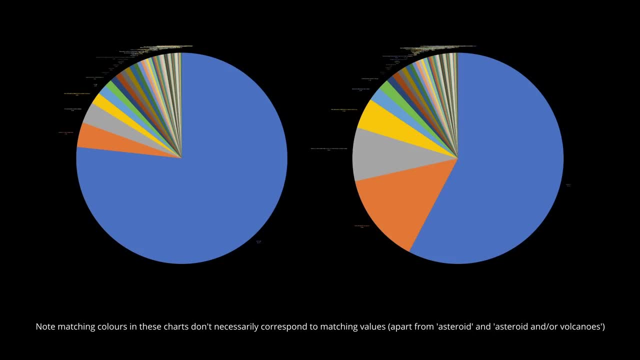 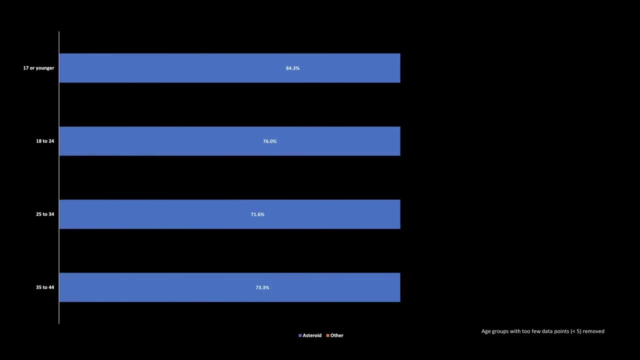 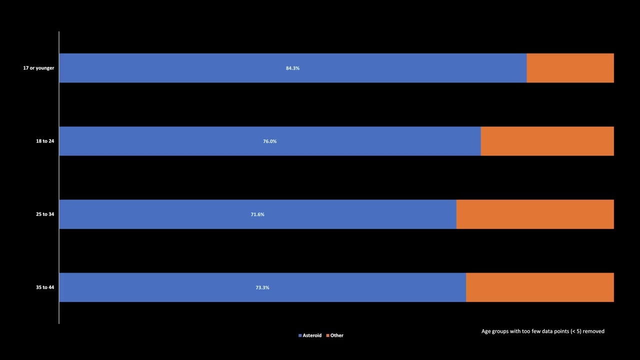 to support multiple or competing factors that include asteroids and volcanoes. Turning to age now This graph shows proportion of respondents who answered asteroid versus something else in the first question. Unfortunately, due to demographic problems, I had very few answers from older individuals, so I've excluded them. here We can see a slight 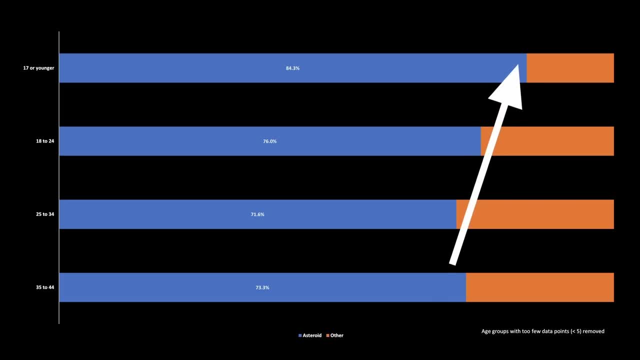 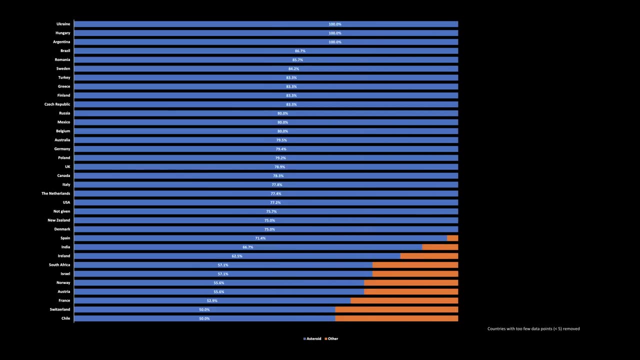 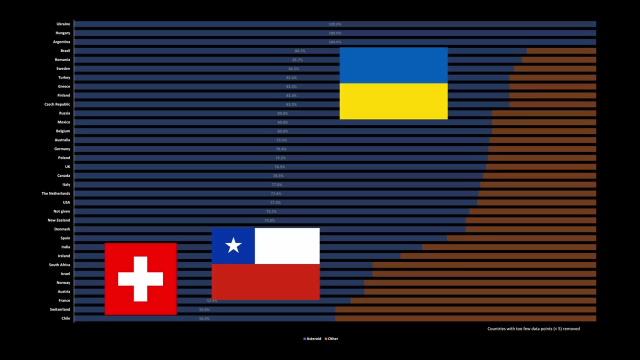 trend, Younger individuals were more likely to say asteroid. Geographically, it was almost an asteroid sweep. Excluding countries with small sample sizes, every country was 50% asteroid or higher, with Switzerland and Chile the most asteroid sceptic- Ukraine, Hungary and Argentina. 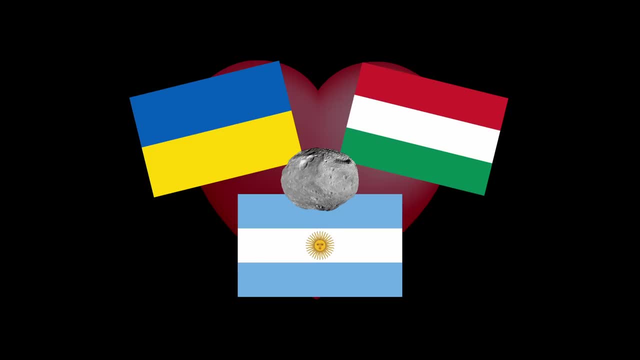 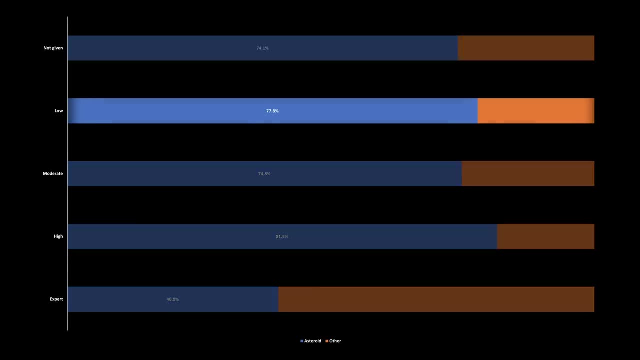 meanwhile, were 100% pro-asteroid. I have no idea what to do with this information. And finally, interest and expertise. I ended up creating groups with low, mediocre, high and expert levels of the two measures combined, according to my own judgement. 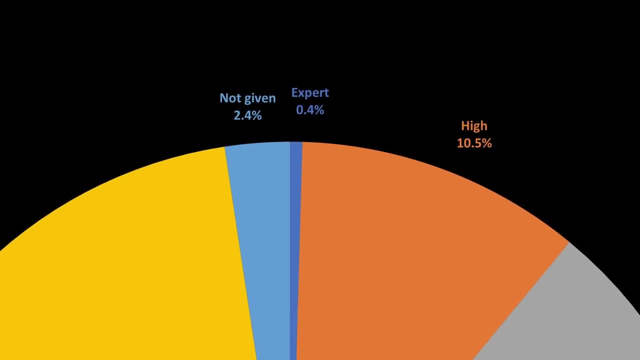 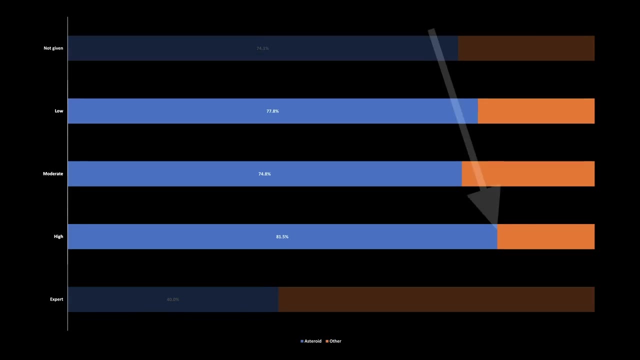 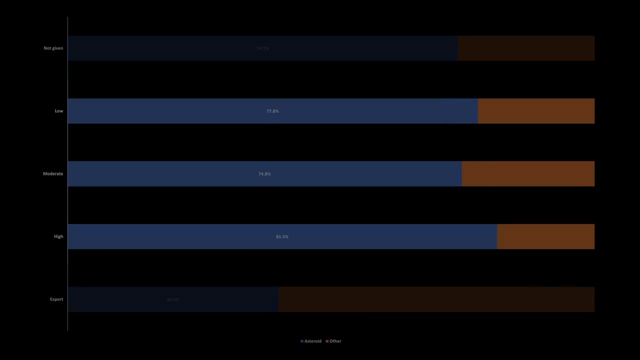 Note, though, I only received responses from 5 experts as identified by me, so take that category with a grain of salt. Excluding experts, the trend is in fact towards asteroid as interest grows. Again, I overestimated familiarity with the idea among low-interest groups. 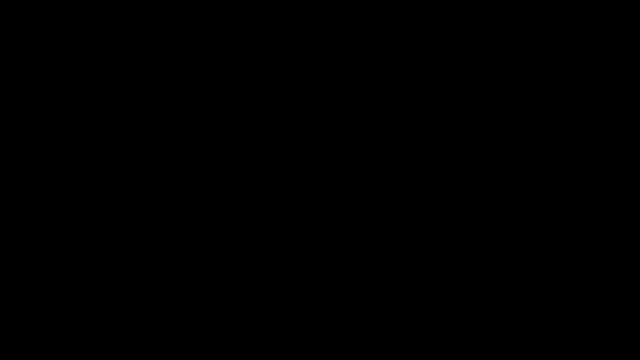 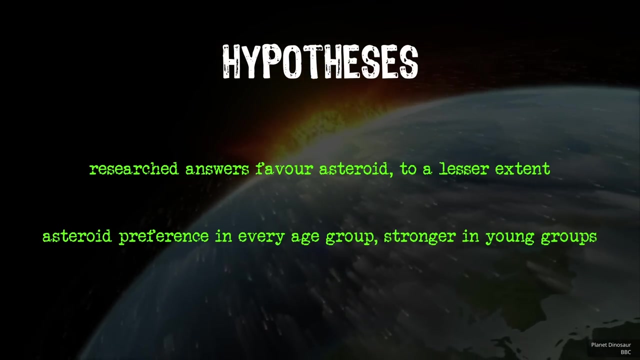 Oof, that was some data analysis, Prime YouTube content right there. Of my five hypotheses, I think it's fair to say I found strong evidence for two, reasonable evidence for two and uncertain evidence for one. Not bad going I can. therefore. 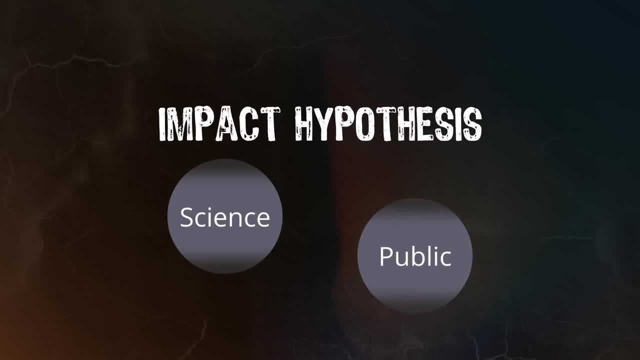 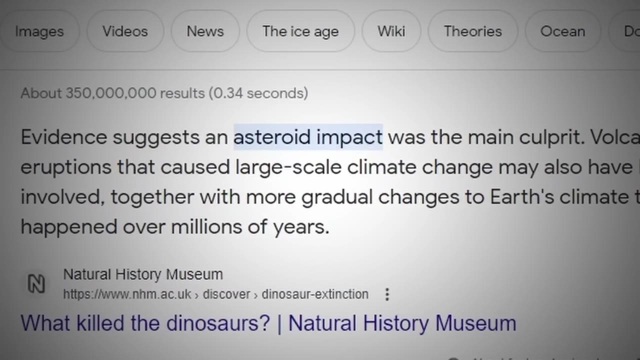 say, with a bit of confidence, what I had only speculated before. Public consensus across many ages, many countries and many knowledge levels supports the impact hypothesis. Whether representing scientists or the average Joe, Google is right: An asteroid impact killed the dinosaurs, But I wouldn't have made this video if it was that simple. 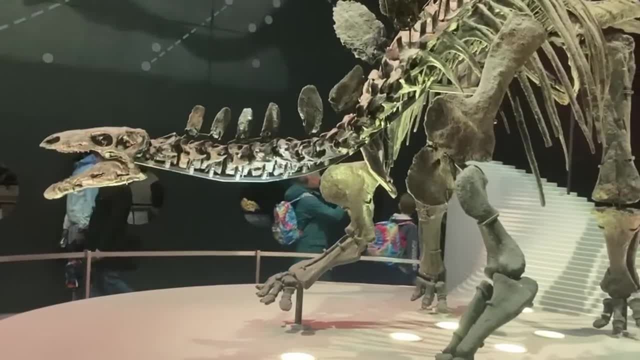 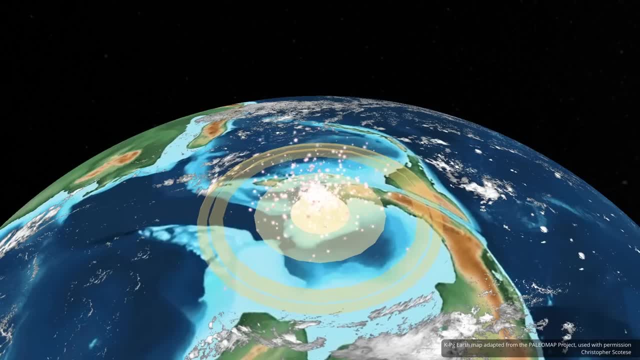 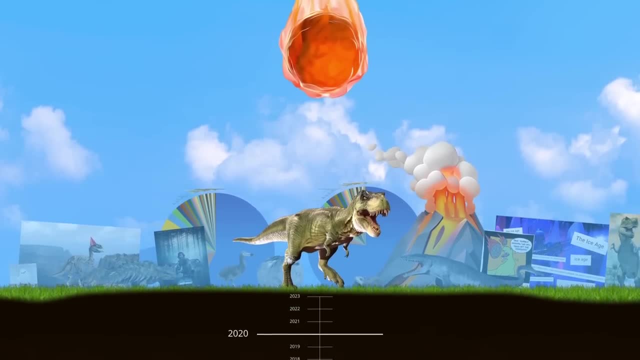 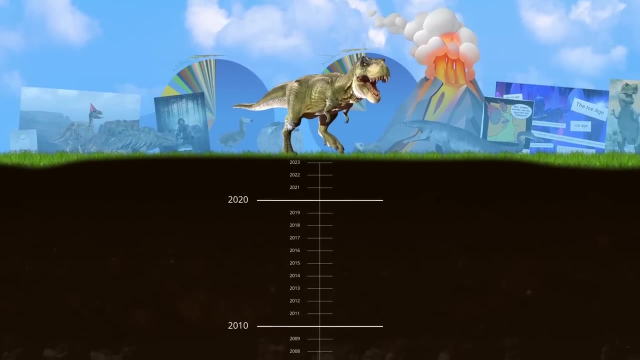 Without the richer understanding of how we got here and why it matters, A single layer piled atop countless unknown layers of the past. We have but scratched the surface, And if paleontology has taught us anything, it's that to go back to the beginning to understand the whole story and our place within. 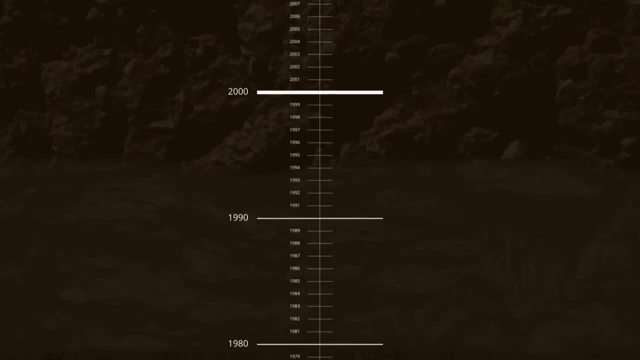 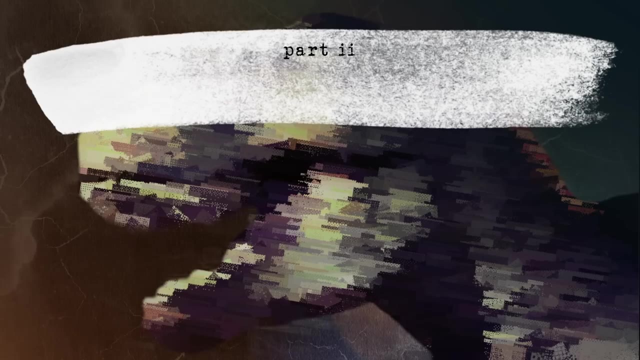 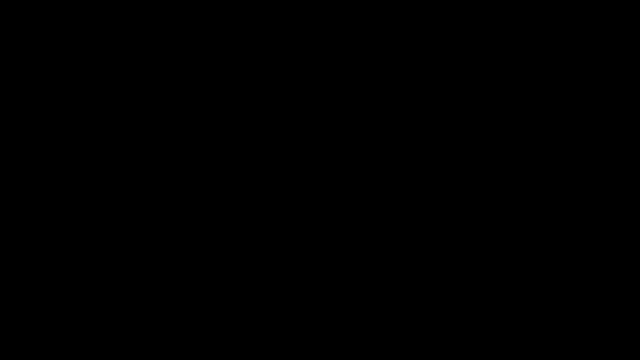 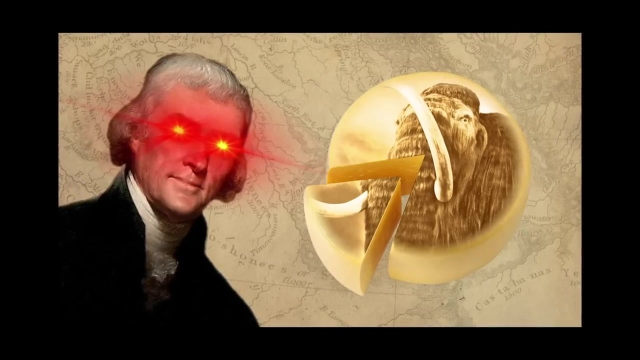 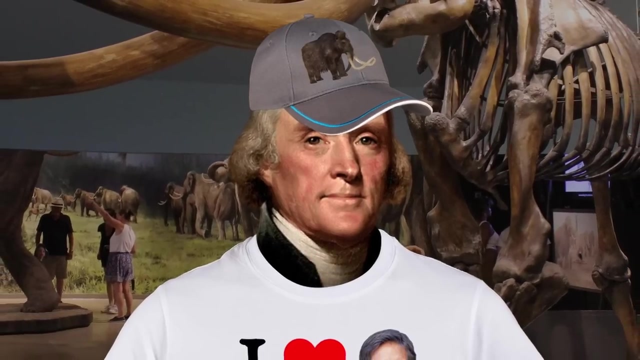 it. We need to dig. Part 2. The Record of the Rocks. Our story begins with mammoth cheese. For those new to the channel, I made a video a while back about Jefferson's mammoth cheese. You could go watch it if you like. In short, US President Thomas Jefferson became obsessed with 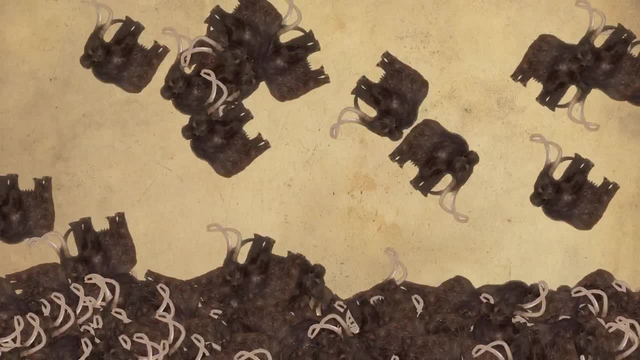 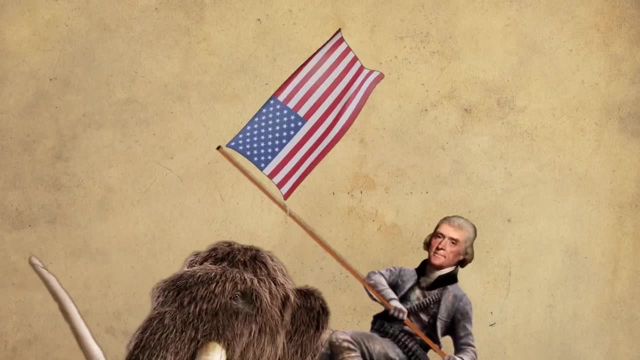 mammoths. after so many of their fossils turned up in his young country, Some guy gave him a giant cheese wheel. people called it the mammoth cheese. history was made. What's more, Jefferson's mammoth mania might have made most of America. He was convinced mammoths. 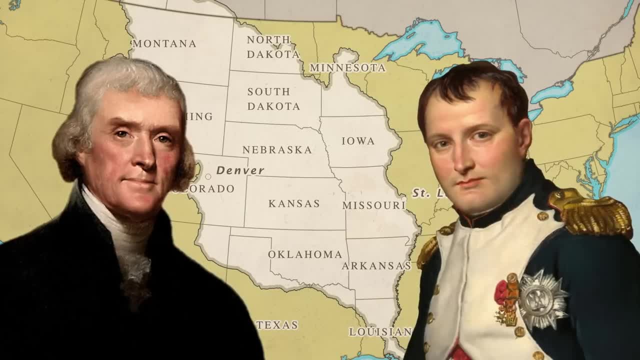 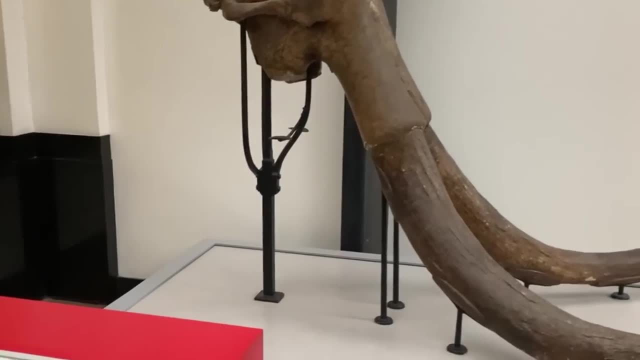 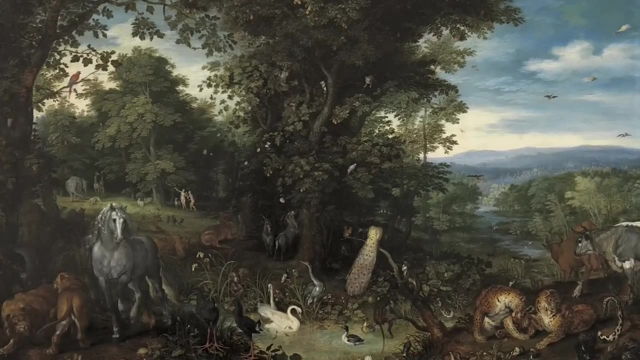 must still exist out West and purchased a large portion of the continent to find them. Implicit in this goal is Jefferson's rejection of extinction. He fully believed species cannot simply disappear. At the time, roughly 1800,, this was a common view. Theologically speaking, if God had created the 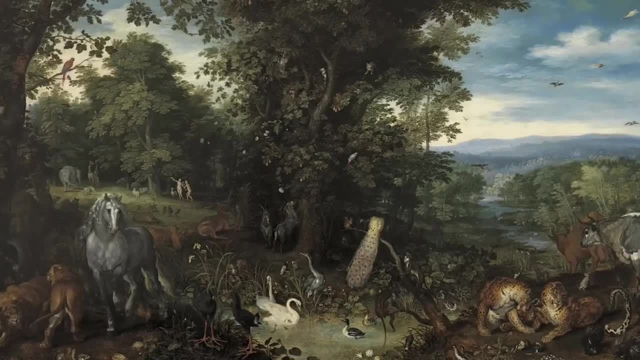 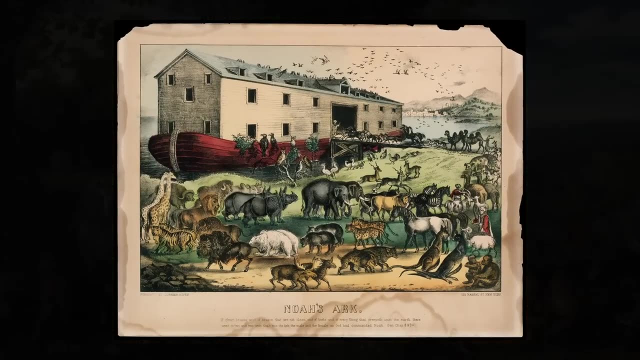 earth in its perfect form from the beginning. how could extinction possibly occur? That would imply a fault in creation itself. The one exception was the biblical flood Found a fossil that doesn't match any living creature. Easy flood did it, Noah just didn't like them. Indeed, this was the 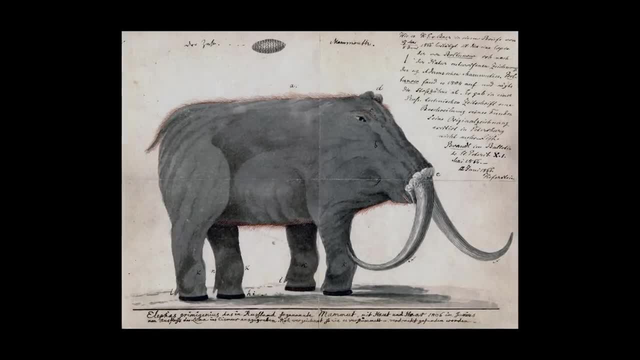 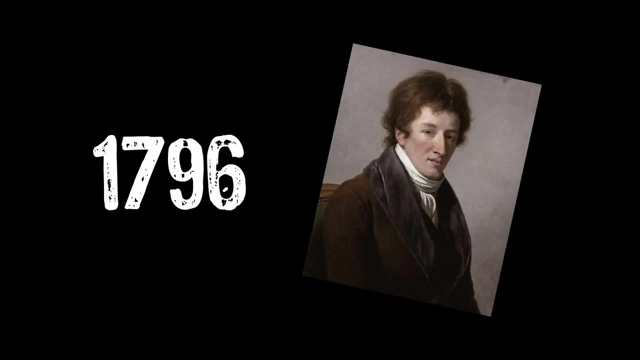 view on American mammoths back when they were first unearthed. But these same bones would soon bring extinction to light as a scientific concept. In 1796, French naturalist Georges Cuvier published a paper arguing that mammoths, which in many cases he reclassified as mastodons, 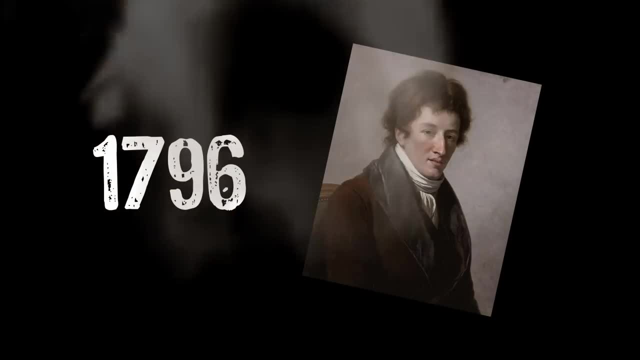 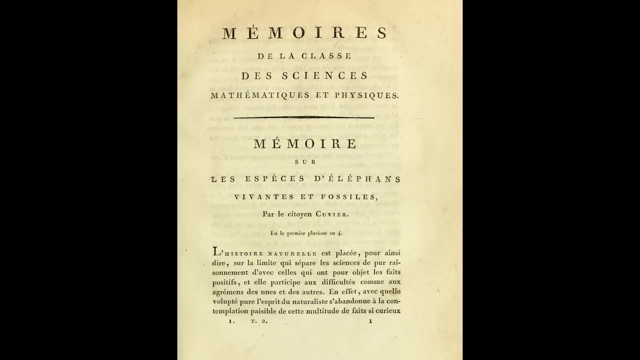 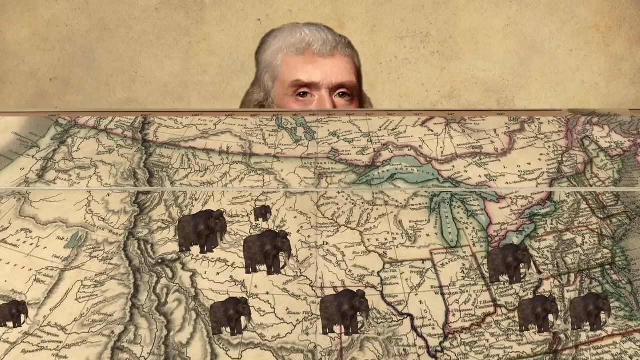 were extinct. They looked like elephants but they weren't, and they ruled dead. This paper is the first formal description of extinction, the first to provide a real deduction from real evidence. As Jefferson's continued pursuit of living mammoths shows, not everyone jumped on. 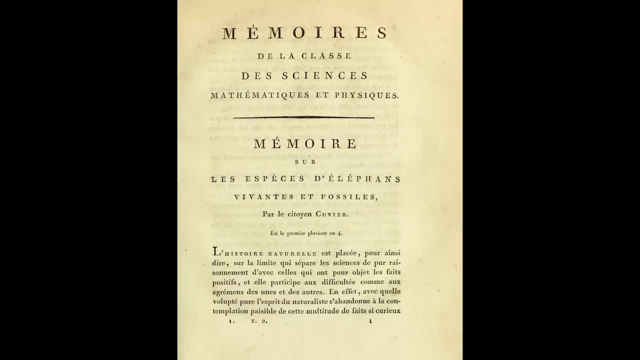 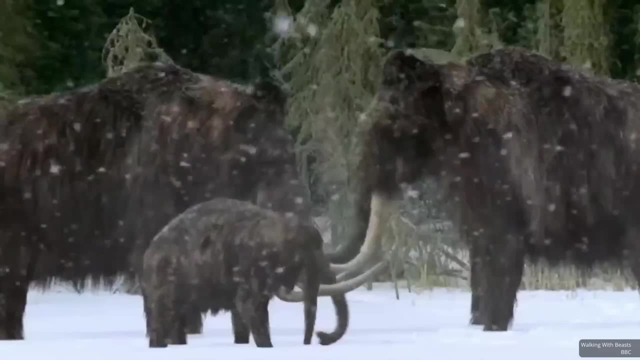 the extinction bandwagon, but the idea was accepted by many naturalists At the moment of its birth. extinction invoked a question that would bubble and seethe for the next two years: The question of how many mammoths would survive the next two years. 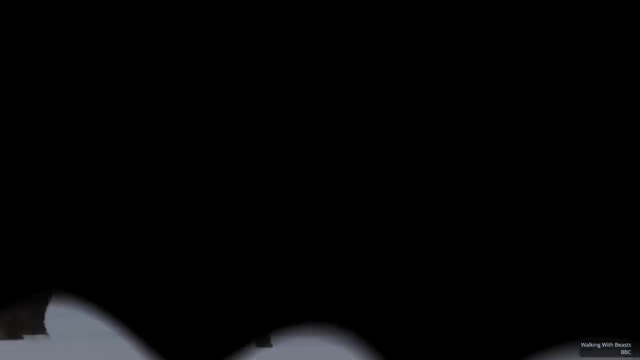 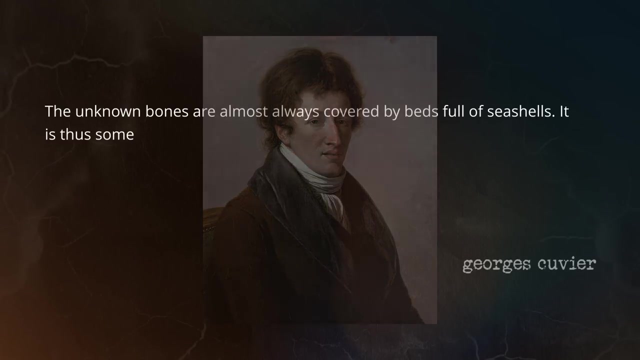 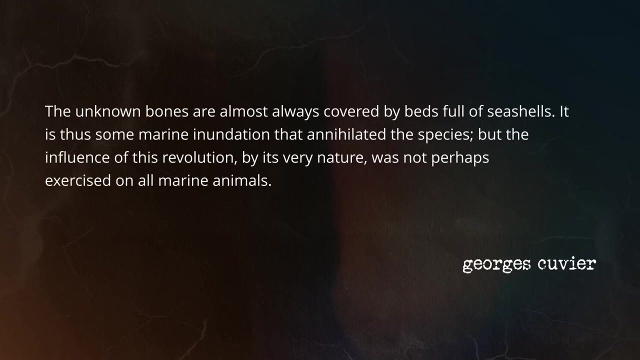 If species do disappear how? Cuvier's answer was a natural progression from the flood, He believed. great cataclysms- revolutions, in his words- regularly blanketed regions and wiped out populations. Many were oceanic deluges on a scale beyond human imagination. This philosophy, 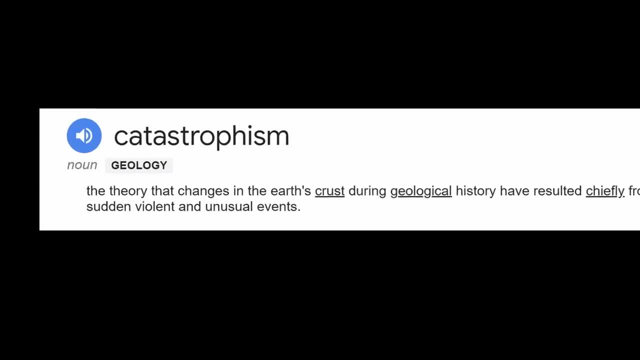 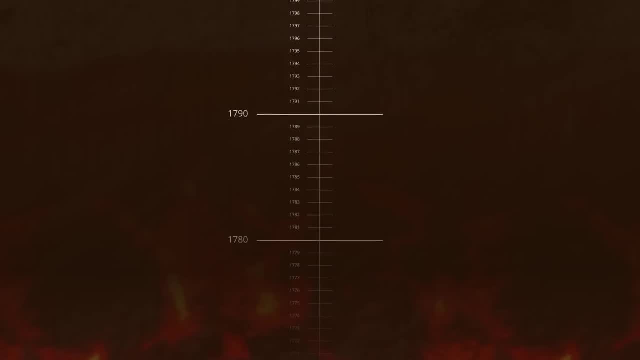 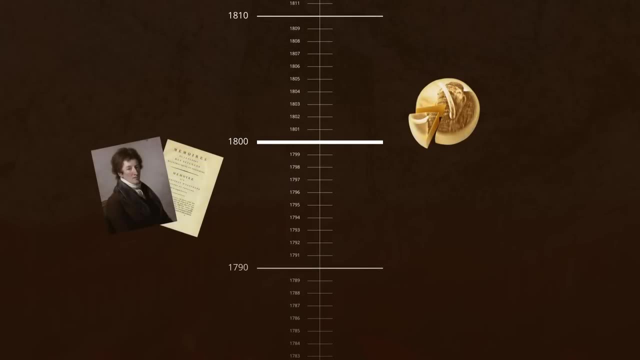 is known as catastrophism, the theory that changes to the earth were caused by sudden, violent and unusual events. Identifying changes to the earth in the first place, though, is tricky business, So before we understand those sudden, violent and unusual events, we need to take a step back. For me, in more ways than one. 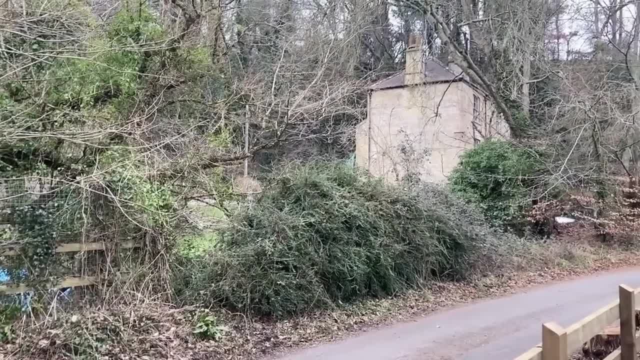 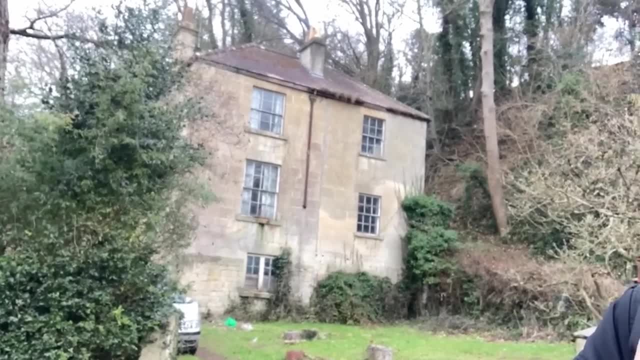 There's an unassuming house I used to walk past during wanderings through the outer reaches of the city of Bath where I went to university. Annoyingly, I only realised its significance after I left, so I had to make a day of it to get this footage. 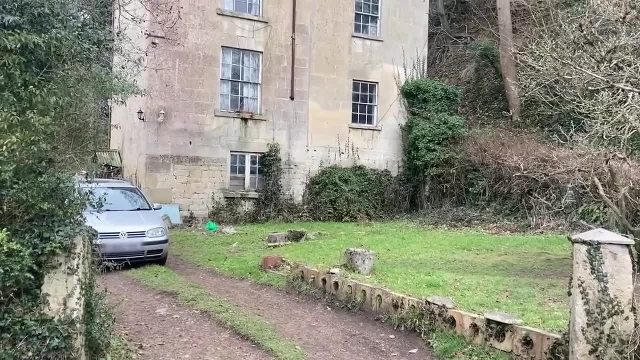 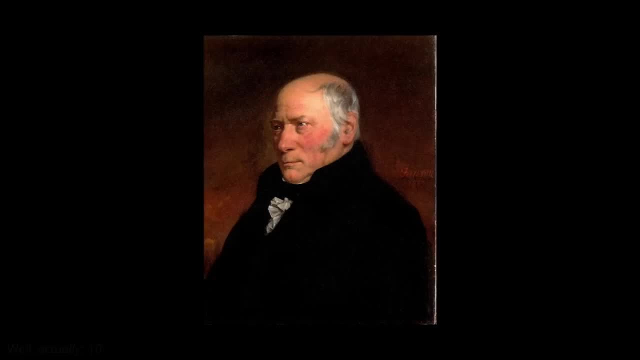 Ew, there are things back on my mind. Around 1800, this house- and yes, it was this house and not the one next to it, the black is on the wrong house- was home to a man named William Smith. Smith was a geological. 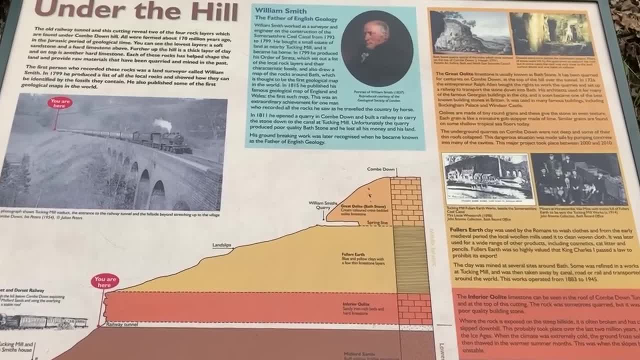 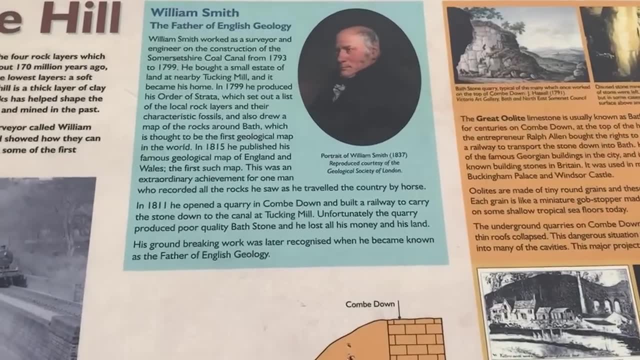 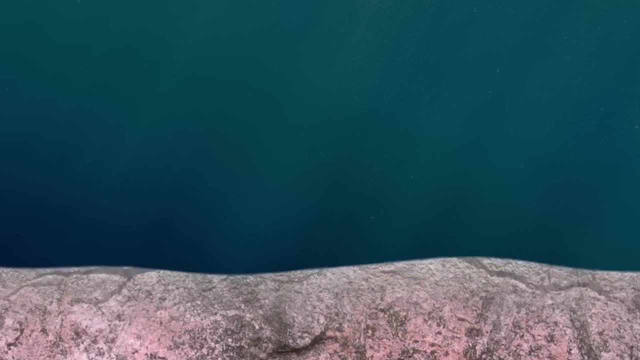 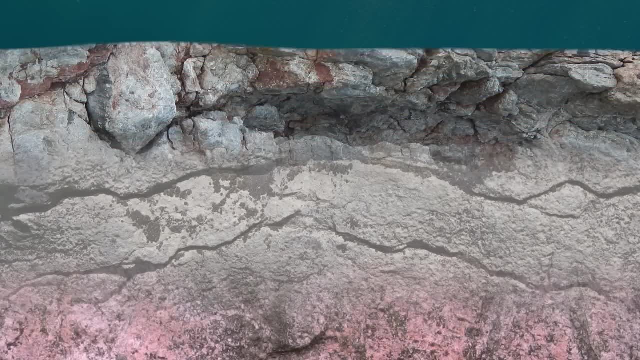 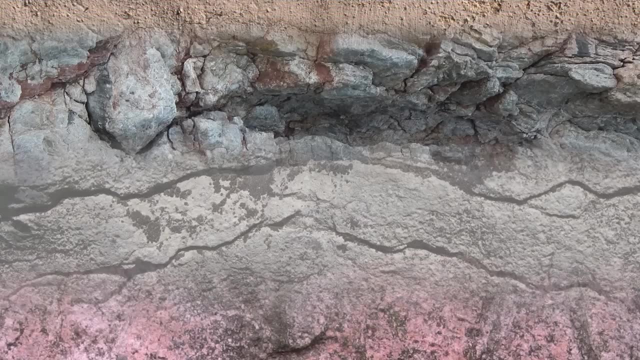 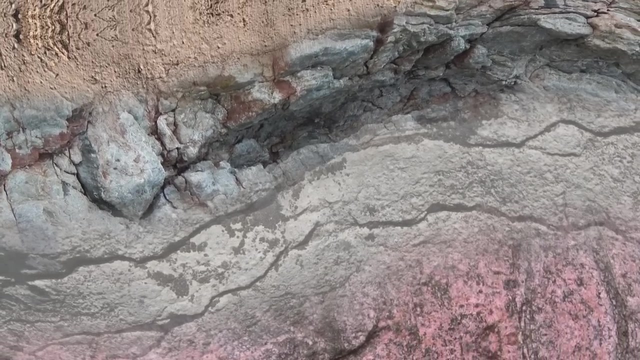 reveal how conditions changed, including contemporary fossils. In absence of other factors, you have a full timeline. getting older, the further down you dig. Sadly, there are many other factors. Any kind of squishing, rotating or other distortion renders the whole sequence useless. 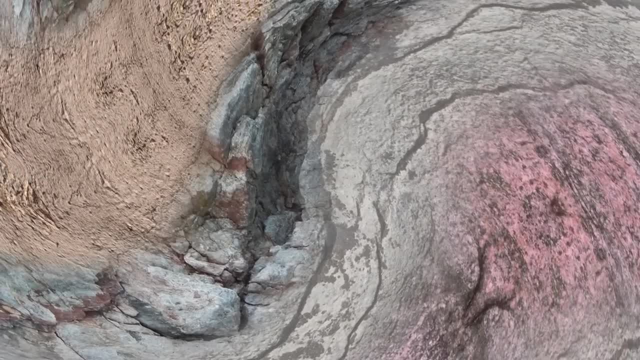 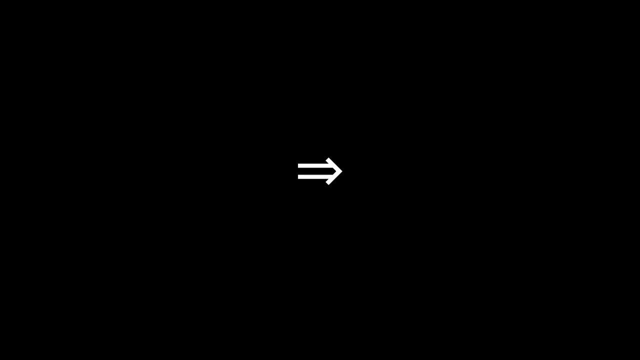 if the layers are unique enough- rock types, clay vs chalk and so on- you can piece together some kind of reconstruction. But much more likely, rock alone tells you very little. If you can't put the rocks in order, you can't put the fossils in order. Simple as that. 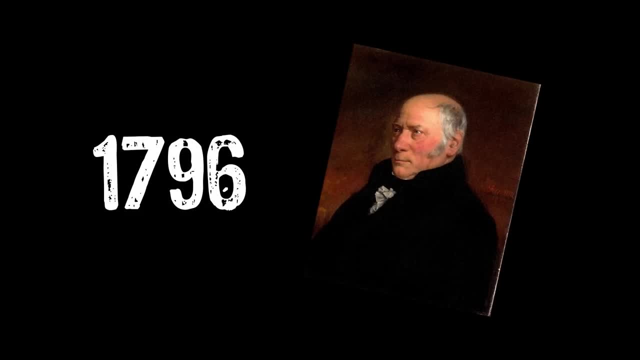 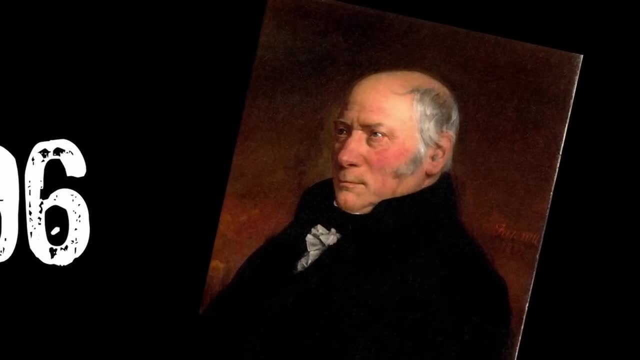 This was the problem Smith was pondering in Somerset, And it was in 1796, the same year as Cuvier's extinction proposal, that he had one of those epiphanies that really makes you stand back and appreciate the human mind. What if we turned it backwards? What if we could put? 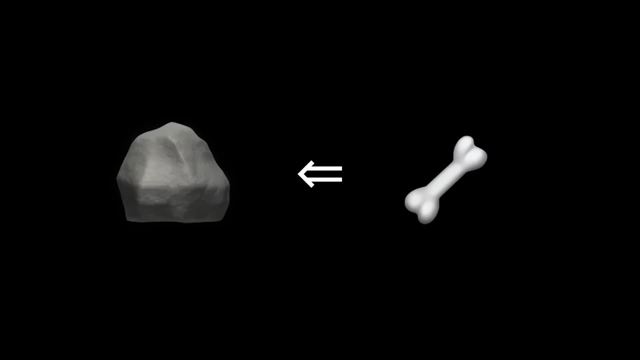 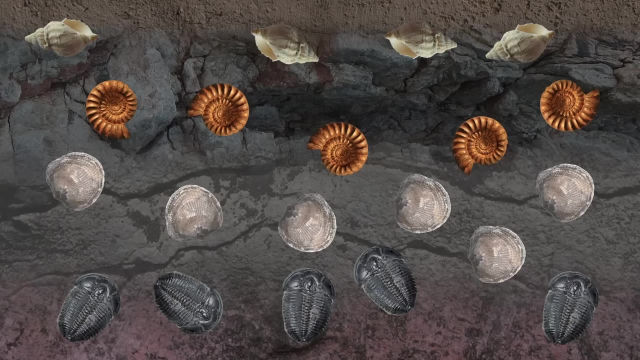 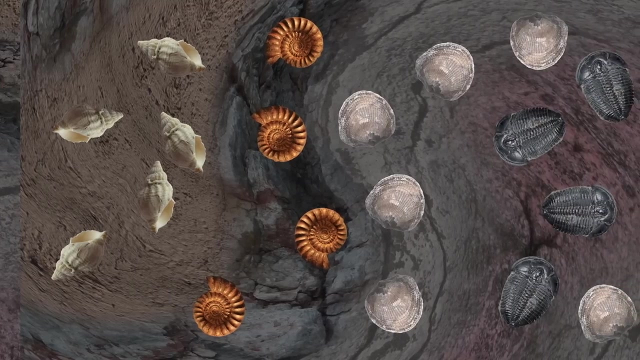 the rocks in order by putting the fossils in order. Take deposits with well-established, calm and regular sequences, often quite rare, find the characteristic fossils of each and use these to correlate against ages in chaotic deposits anywhere in the world, If the same fossil 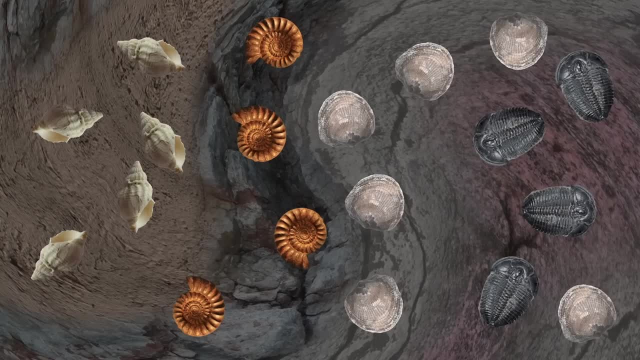 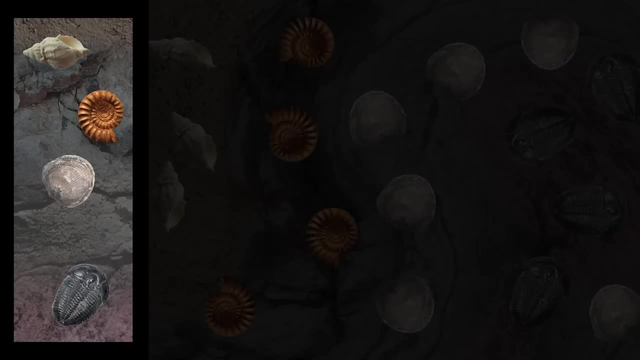 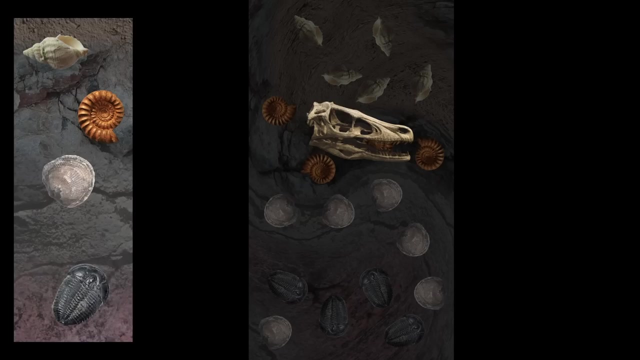 appears in two places but nowhere else. it's likely these together represent a distinct geological period. Using the order of correlating fossils in calm sequences, you can decipher the order of pretty much any sequence and date new fossils unique to irregular sequences that were until then. 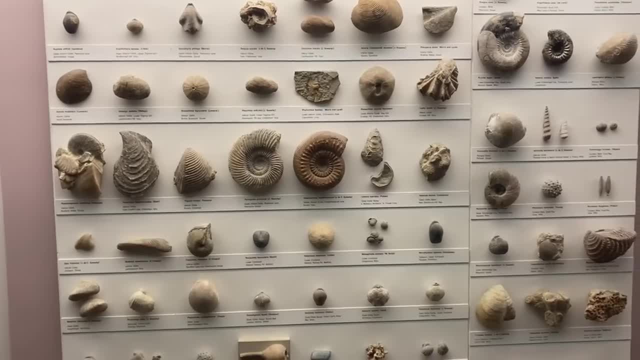 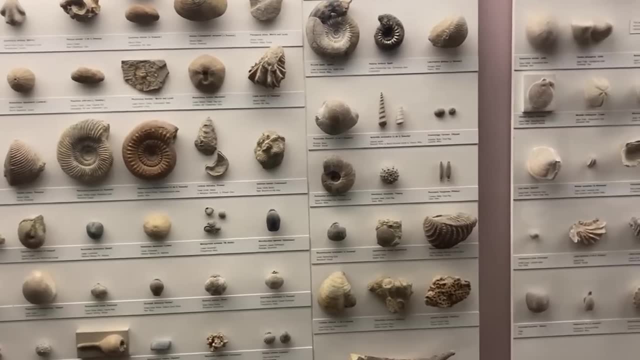 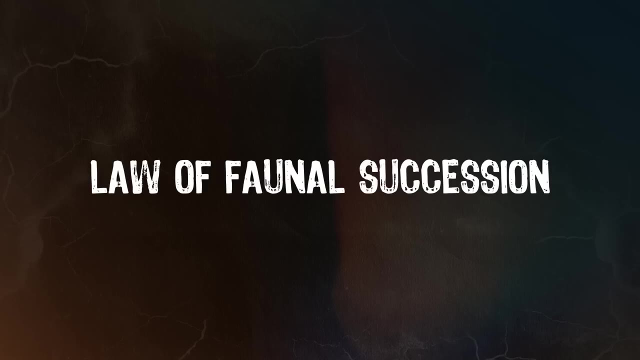 a mystery. The best fossils to use for this correlation are small marine animals, since they're much more common than any other fossils. It's a question of resolution. Smith named this technique: the Law of Faunal Succession: the clear progression of species across time. that could help. 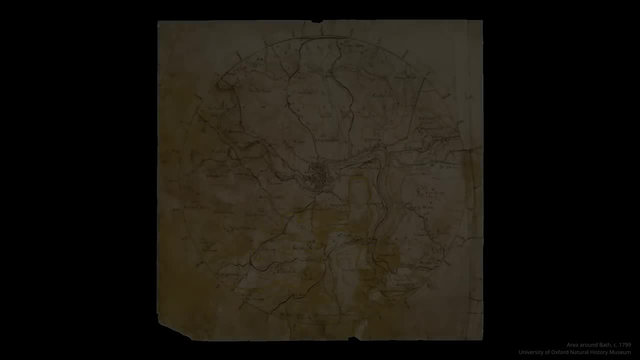 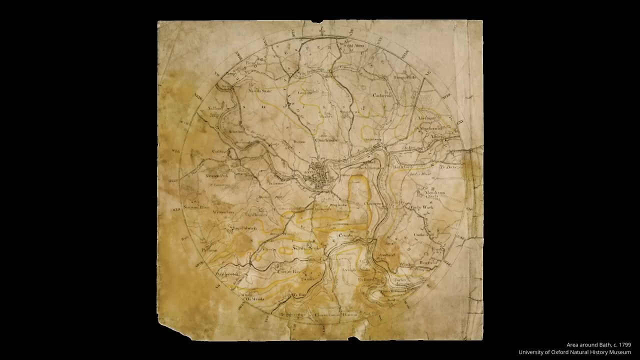 index them. The law of faunal succession is a technique that can be used to predict the course of a geological process. In 1799, Smith produced the world's first fossil-supported geological map. This humble map of Bath is the basis for everything we've learnt about prehistory since. 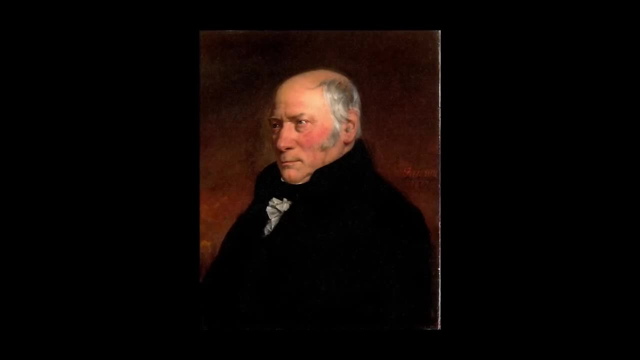 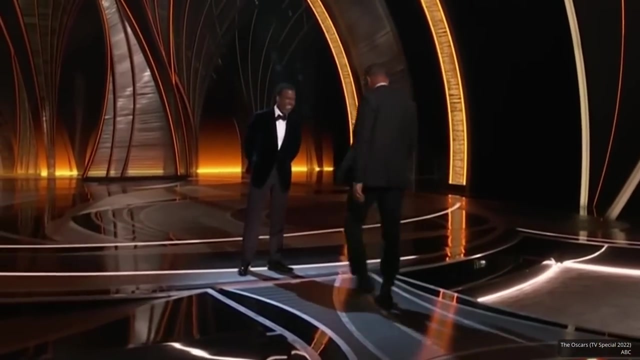 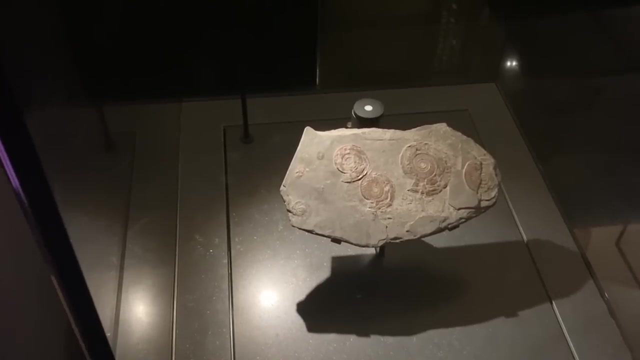 often earning William Smith the title of Father of Geology. I mean, you could say he cracked rock, Which is something people named Will Smith keep doing: Epic rap battle of history. when, Yet caring mainly for practical applications, Smith didn't much ponder why different layers contained different groups of species. 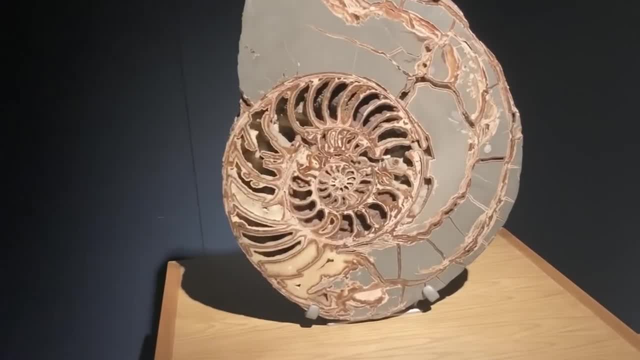 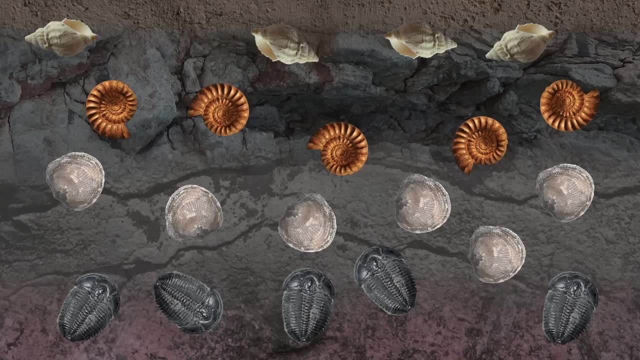 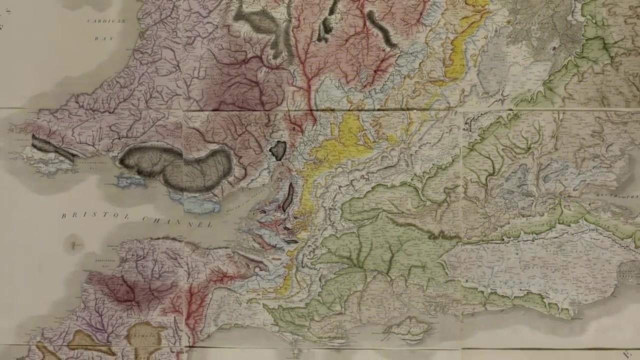 From the modern perspective, the answer is obvious. Some had gone extinct and new forms had evolved to replace them, But Smith never made that connection. So while we can say he found the evidence for many extinctions, he never inferred the extinctions themselves. Over the next decade, Smith extended his work. 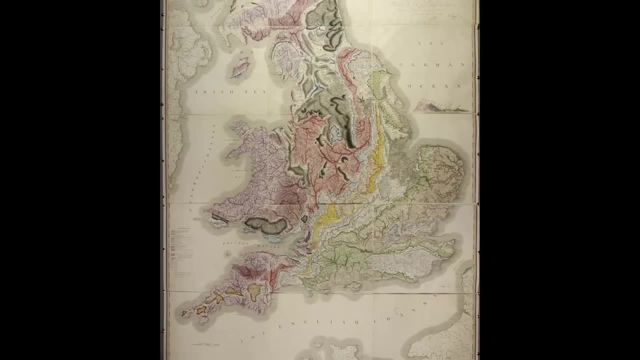 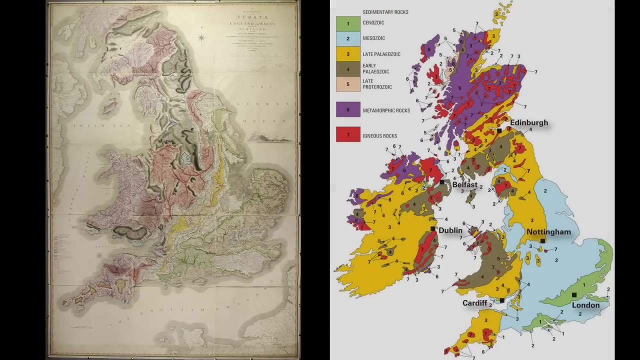 from Bath to the whole country. Based on correlations from his travels, he published the first geological map of England and Wales and published the first geological map of England and Wales in 1815.. Comparing with a modern map, we notice he identified based on differing fossil. 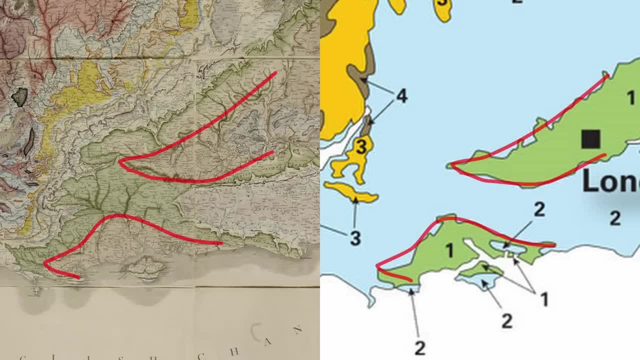 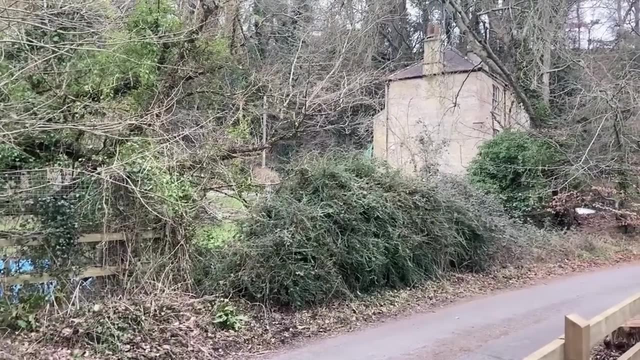 ecosystems, what we now know to be a boundary between Cretaceous and Palaeogene rock. That is- and I'm going to have to be careful with my words here- this house may well be the place that evidence for the K-Pg mass extinction was first recognised. 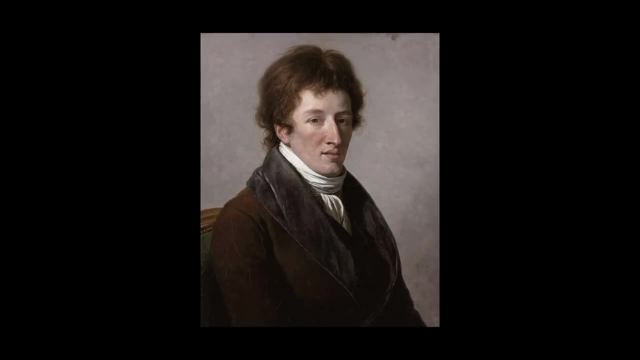 We can, though, say for sure that by 1825, Cuvier II had noticed biotic changeover at the boundary. The second geological map of England was the K-Pg mass extinction. Unlike Smith, the Cuvier II was the first geological map of England. However, the K-Pg mass extinction had been recognized by the 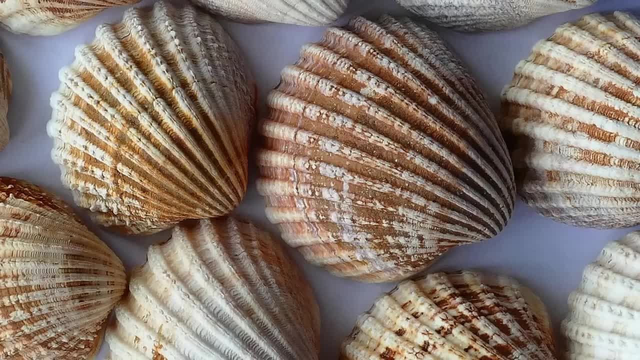 K-Pg mass extinction by the first geological map, That is, it was the first geological map of England. Unlike Smith, he sought an explanation. The first real clue was a change in the diversity of bivalves. but when combined with knowledge of marine reptiles, the kind Mary 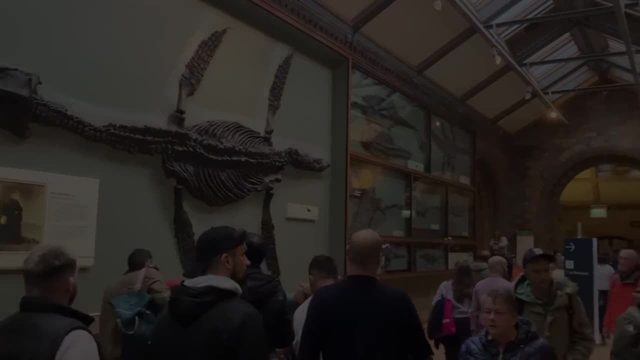 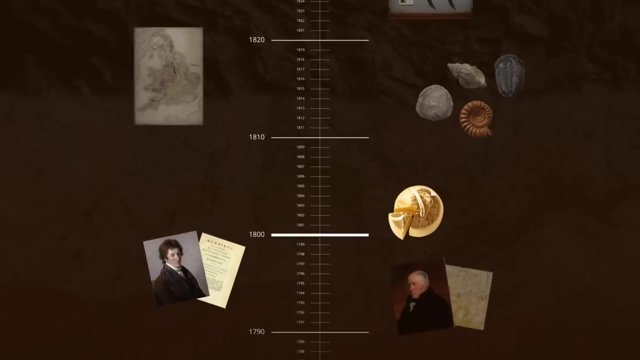 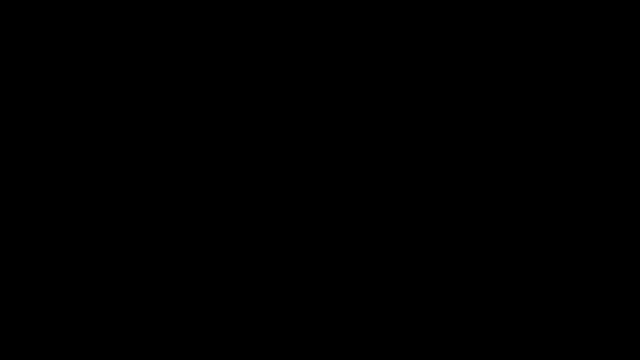 Anning had been uncovering. Cuvier concluded that abrupt, enormous sea-level retreat was responsible for a mass extinction of ocean life. The first theory for the KBG: extinction and catastrophism in full force. But Cuvier's catastrophes were about to meet their match. 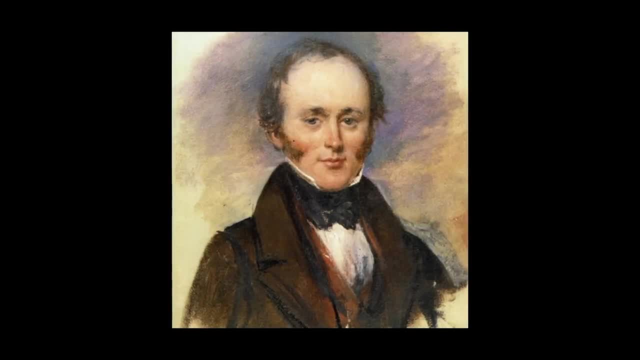 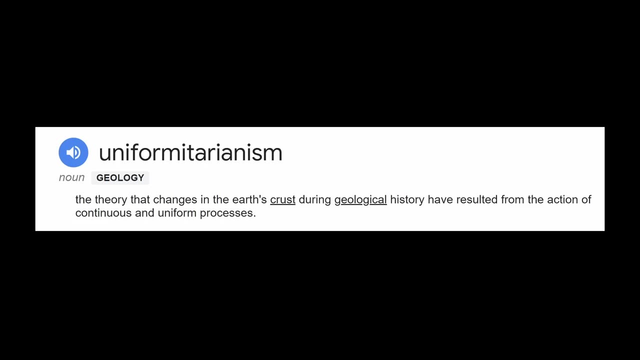 That match was Charles Lyell, a charismatic young Scotsman who was destined to hold geology to ransom for a century and a half. Lyell's guiding principle was uniformitarianism. To simplify, because Lyell's uniformitarianism actually refers to four things. 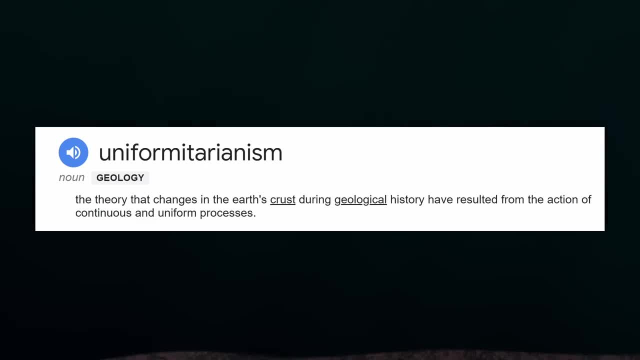 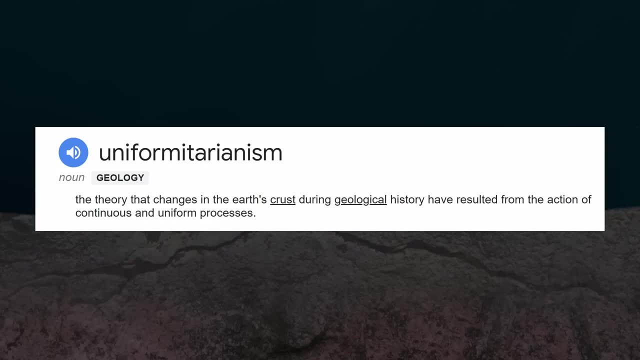 this is the belief that processes of the past can be explained in terms of processes of the present. There are no strange events. everything happens gradually. change is uniform across time. At first this seems eminently sensible. It's kind of the Copernican principle, right? 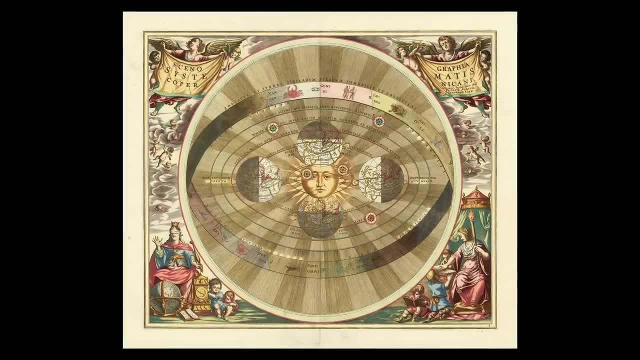 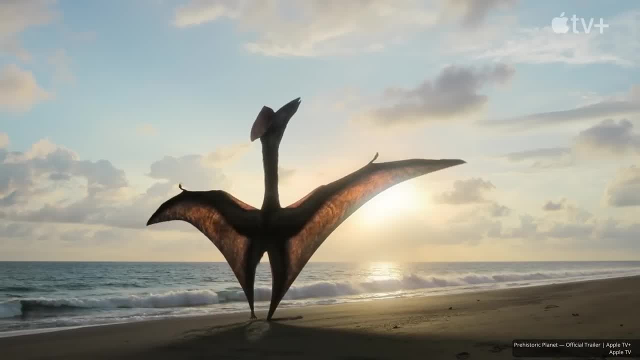 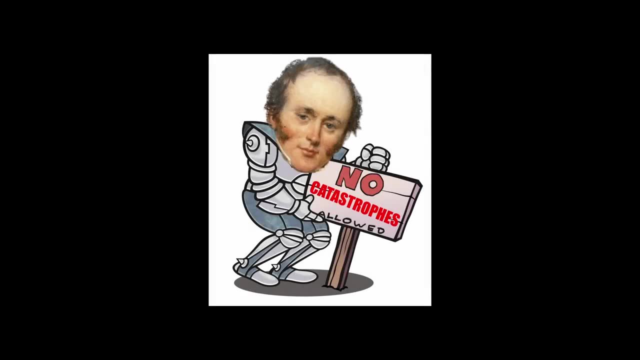 The assumption that human observations are representative of the average view of the universe, And in 90% of cases it is sensible. Prehistoric Earth was about the same as present Earth. Such a mindset has proven invaluable for those studying it. Lyell, however, wouldn't settle for 90%. He wanted EVERYTHING. 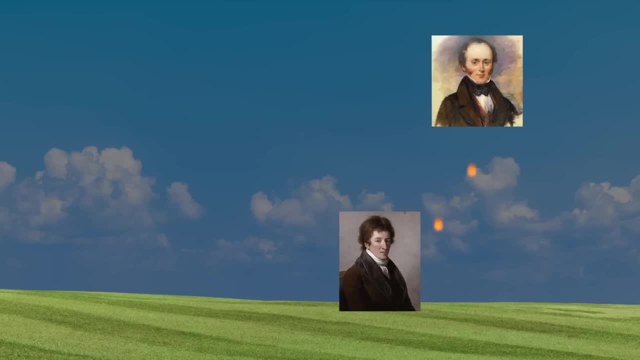 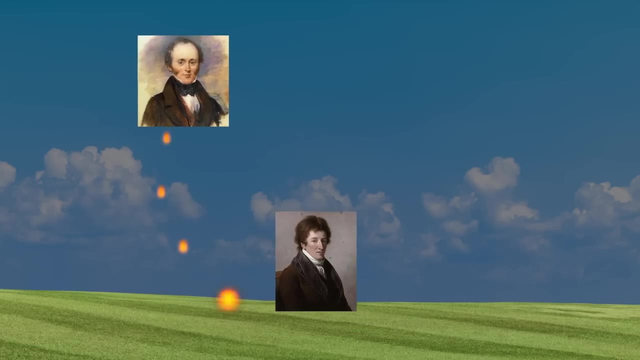 Railing down a storm of strongly worded textbooks. he painted catastrophists like Cuvier as wild and dangerous speculators, pseudoscientific idiots and way too French, And maybe it was more that last point than anything else. but people believed him. 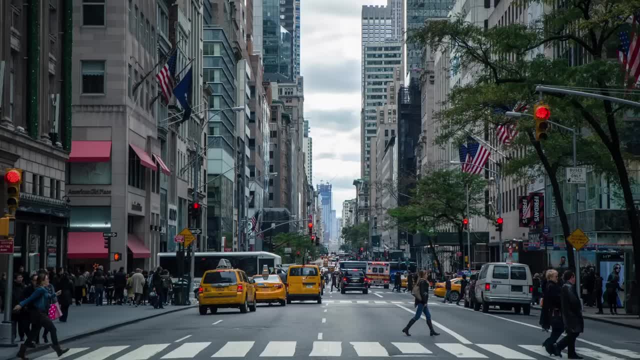 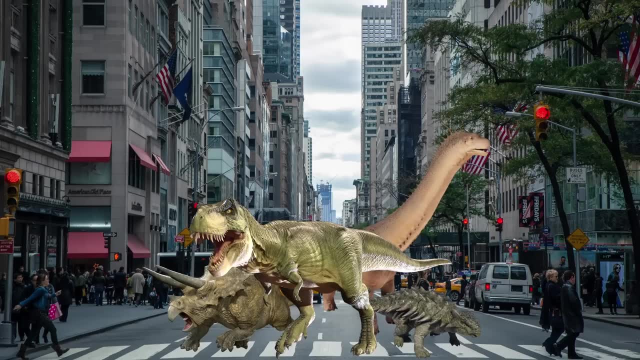 Which is mad when you hear some of his conclusions. He thought, for instance, that should global temperatures rise to match those of dinosaur times, the dinosaurs would just come back. How, Who knows? All I know is I love fossil fuels now. Lyell's belief in a constant world extended to extinction. In his view, extinction rates are not so high. There is no way that the world is going to be as bad as the dinosaurs. In fact, the world is going to be just as bad as the dinosaurs. 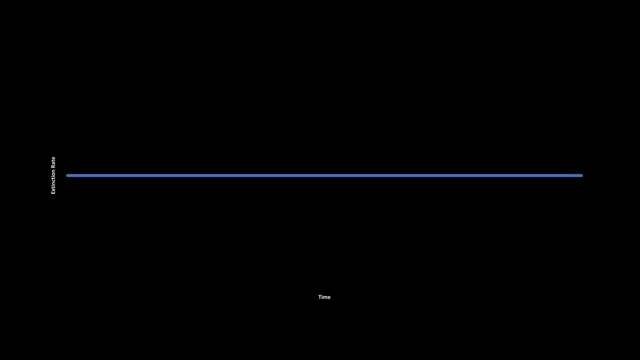 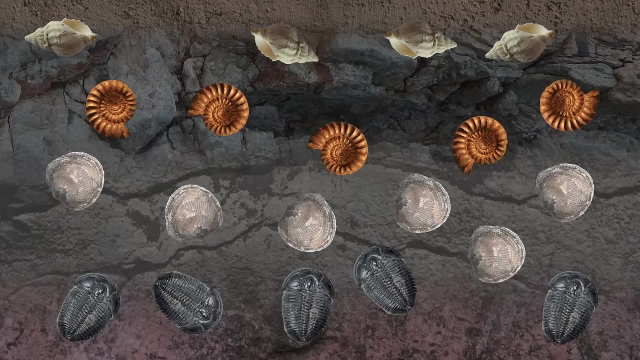 The world is going to be just as bad as the dinosaurs. In his view, extinction rates never varied across time. No mass dying, only consistent background removal. He developed a sort of biological half-life, Taking William Smith's insight and running with it. 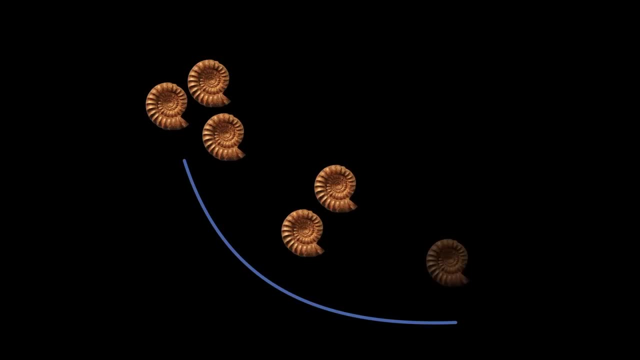 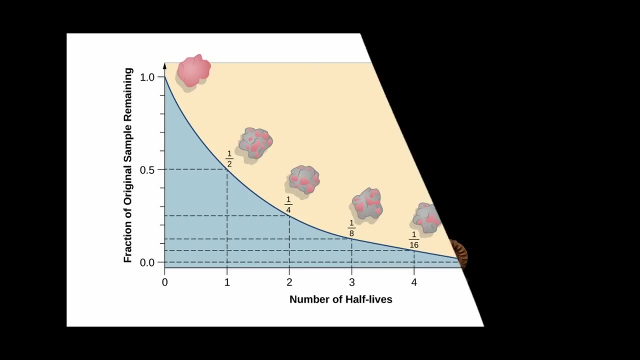 he believed you could tell the exact age of rock simply by calculating the relative decay of fossil ecosystems. As an idea, this is rather neat, but, unlike radioactive, decay, extinction is not a physical constant, so can't be a reliable dating mechanism. And the idea is. for this the first thing we should do is to use the atomic record This had. 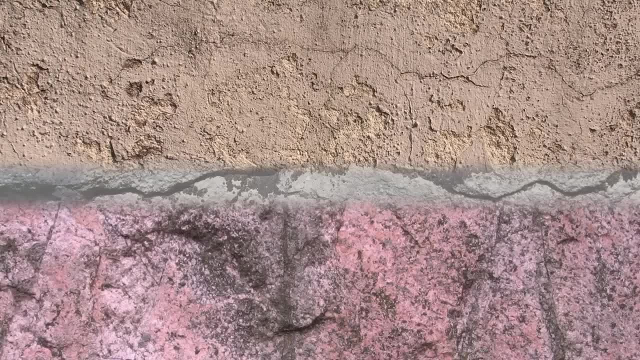 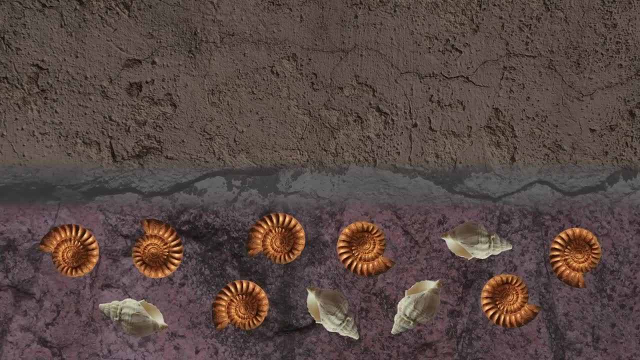 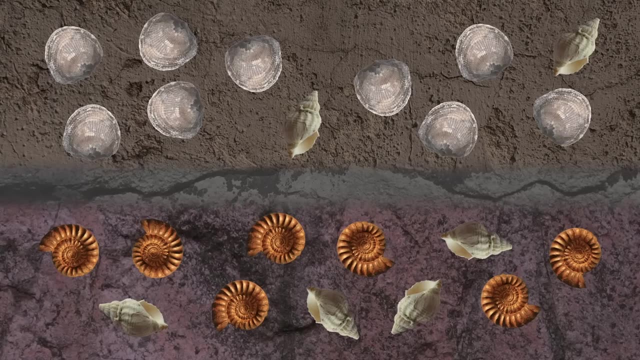 had bizarre effects on the interpretation of the K-Pg boundary. The evidence available in Lyell's time already suggested the boundary layer was thin. One ecosystem profile on one side, then a sliver of rock, then an entirely different one. Today we'd say the boundary most likely represents a short period of high extinction. 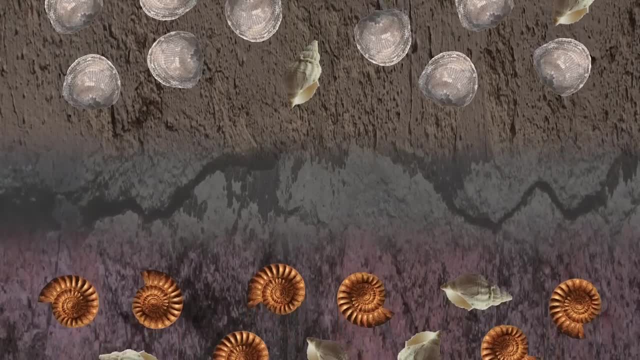 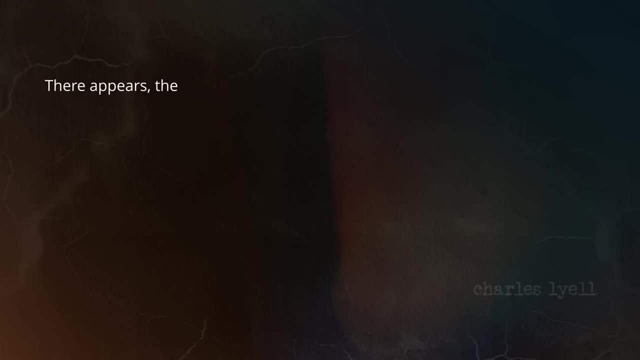 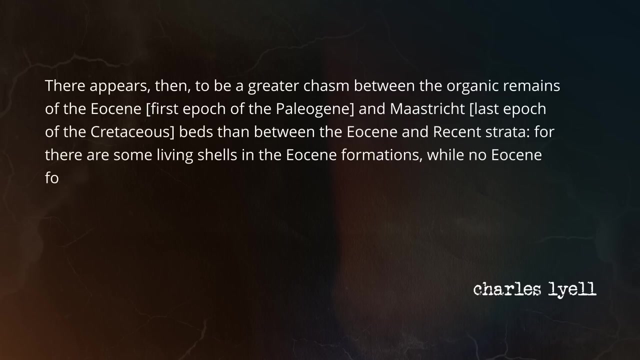 rate. Using Lyell's formula, we find the boundary took 72 million years to form. That's longer than the entire era since, In an absolute tour de force of circular reasoning, Lyell concluded that, since species disappear at constant rates, the boundary had to represent a long period of time and therefore was not. 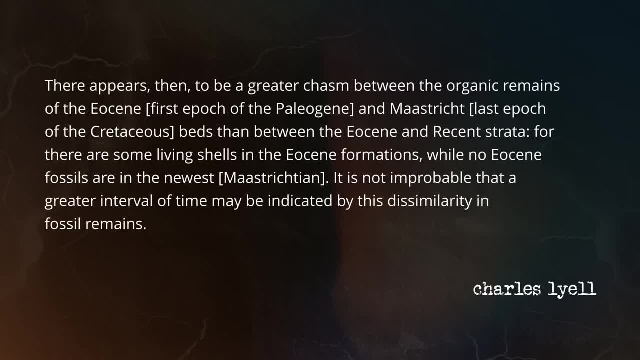 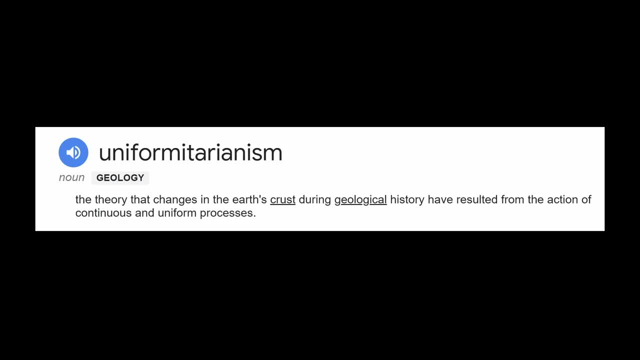 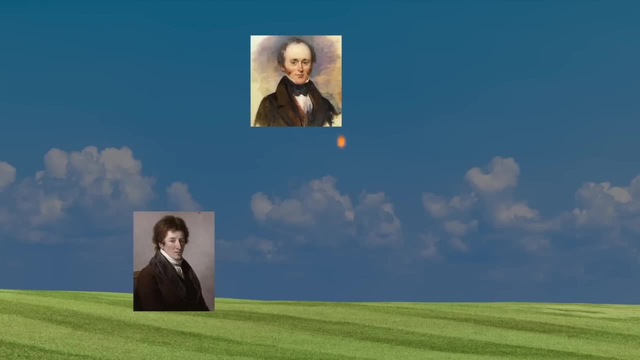 a mass extinction. He instead blamed a poor fossil record, Whether through its 90% usefulness, or just nationalism, uniformitarianism nonetheless grabbed hold of British geology And, thanks to regrettable geopolitics, global geology too. Perhaps I've painted Lyell as something of a villainous puppet master. 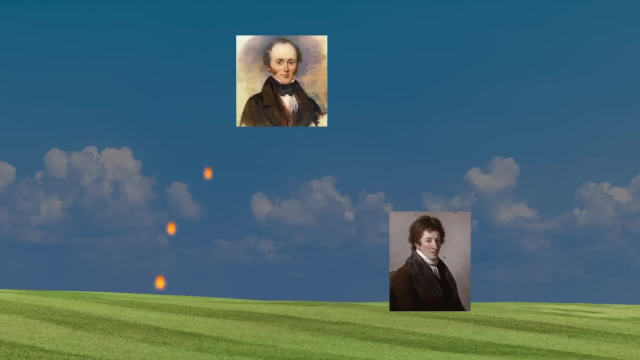 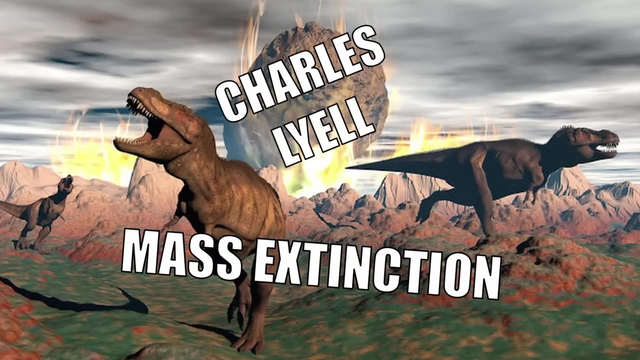 While you should all remember that I'm definitely exaggerating, this depiction is the only one that conveys the scale of his influence. He single-handedly destroyed the notion of mass extinction. All of a sudden, even suggesting higher rates of extinction than usual could get you ostracised. 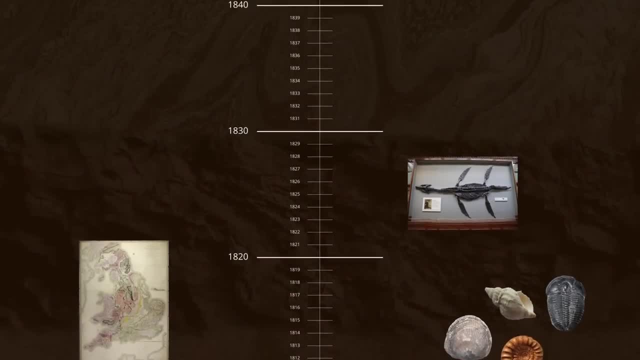 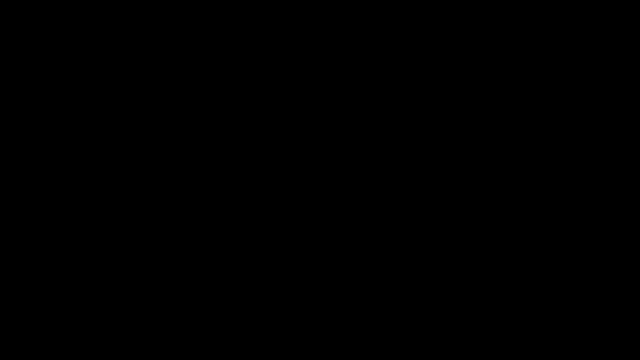 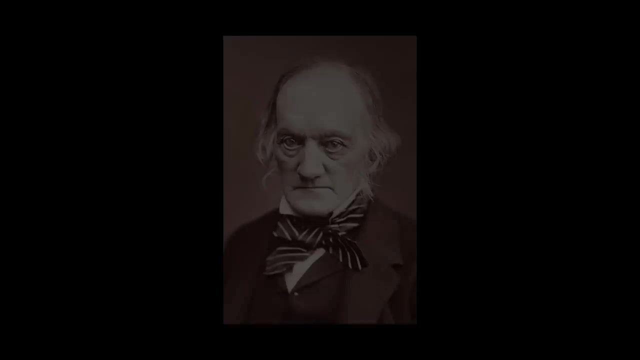 from the paleontological community Before we'd even had time to digest it. the K-Pg mass extinction was pseudoscience. The K-Pg Mass Extinction, Richard Owen, on the other hand, was… definitely a villain: Unpleasant, vindictive, discrediting rivals and claiming their innovations as his own. 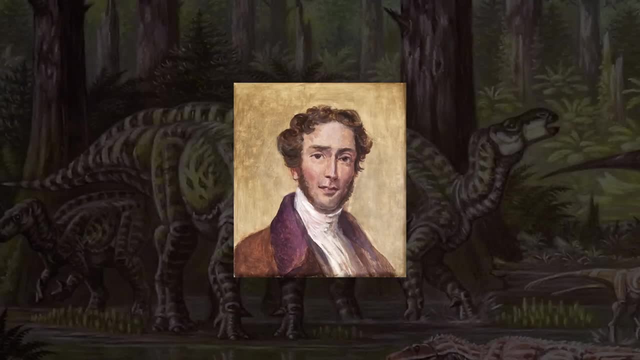 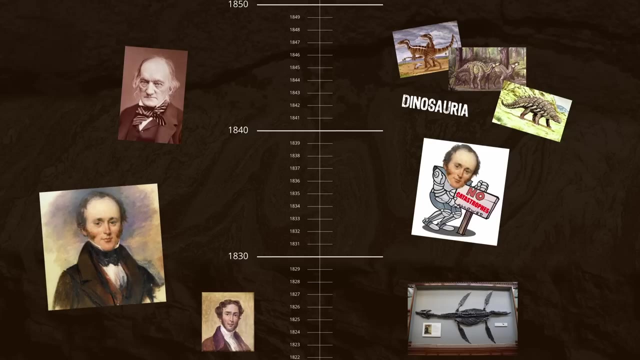 His vendetta against Gideon Mantell, the discoverer of Iguanodon, arguably drove the man to take his own life. But, as you may remember from the intro, in 1842, Richard Owen came up with the name Dinosaur. 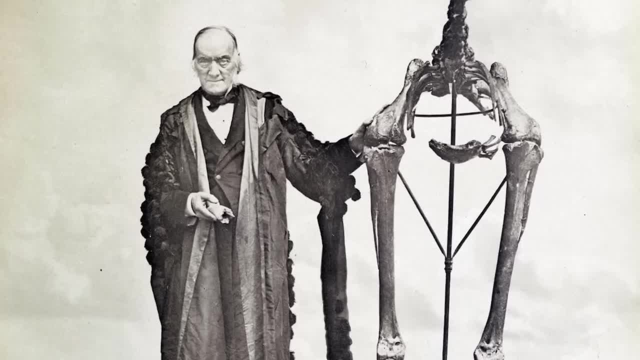 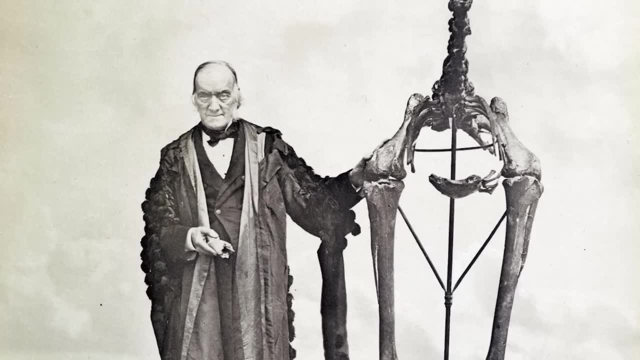 So he's an essential part of our journey. The man was undeniably an anatomical genius, But less recognised And equally important, As is important to note in a video about science communication. he also had a knack for public outreach for his discoveries. 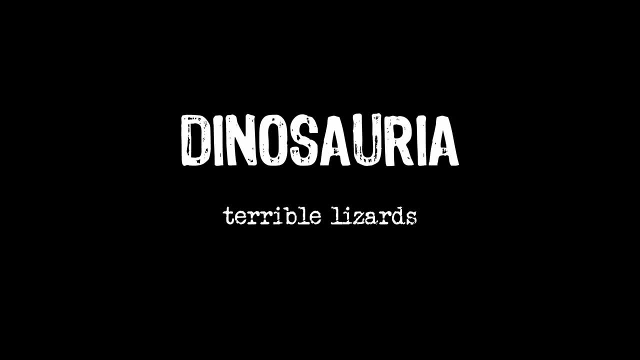 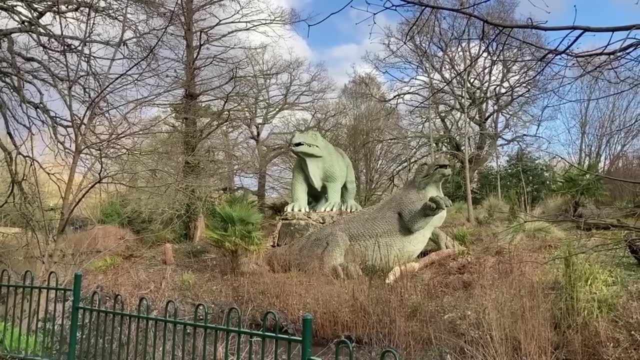 Dinosaur as a term screams star power for a reason. If you walk a short distance from Crystal Palace train station in London, you'll see what I mean. These are the Crystal Palace Dinosaurs, The world's first public dinosaur exhibition. 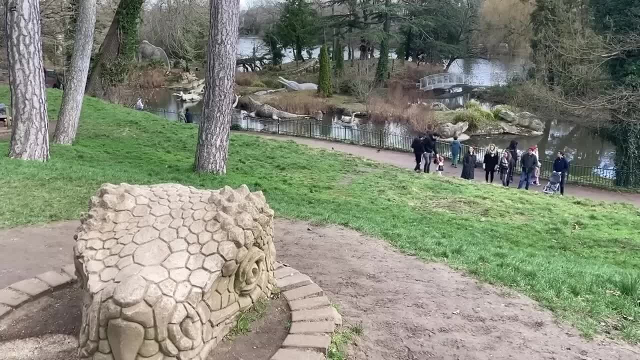 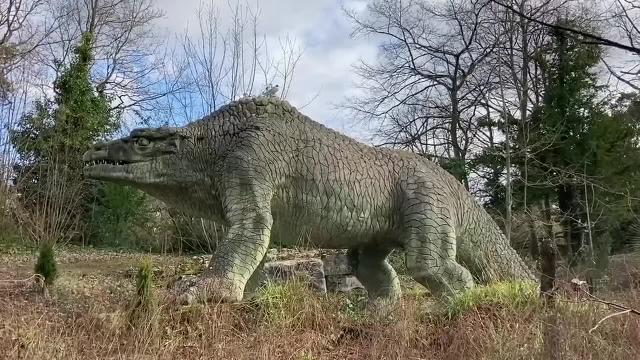 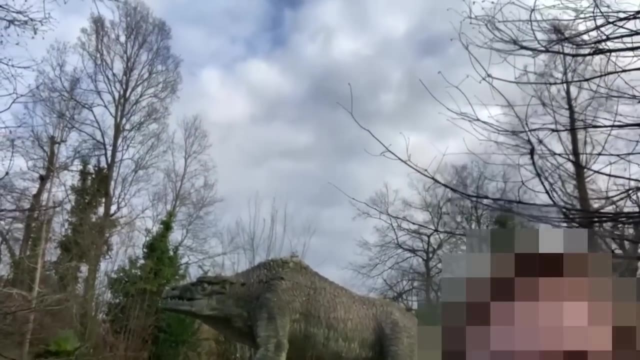 And, in some sense, the world's first theme park. Alongside a host of other prehistoric creatures rendered in clay, you'll find two Iguanodons, a Hylaeosaurus and a Megalosaurus, And one day, a few months ago, you'd have also found me. 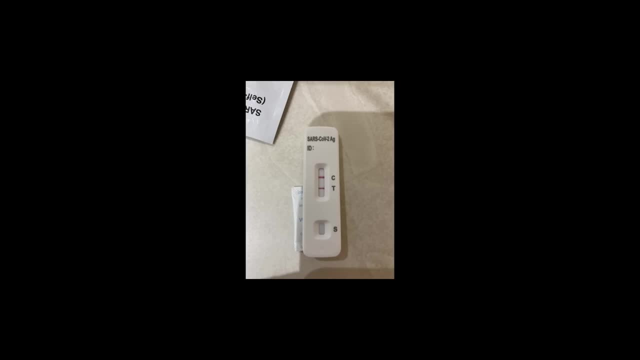 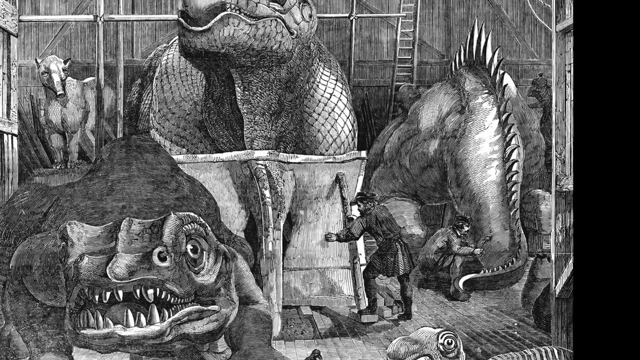 It was a really nice trip, until I caught Covid from it. At least it wasn't Swindon. Created by sculptor Benjamin Waterhouse Hawkins under Owen's supervision, the statues were an instant hit in 1854.. They were also some rather sneaky propaganda. 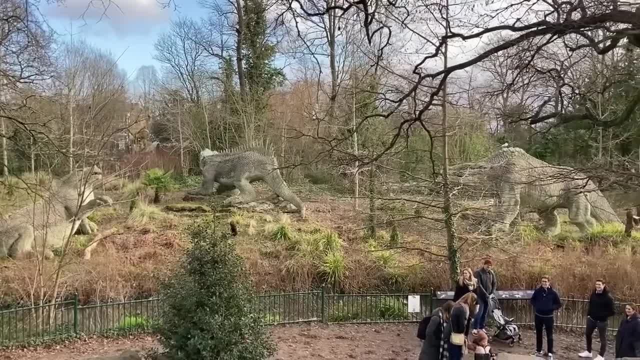 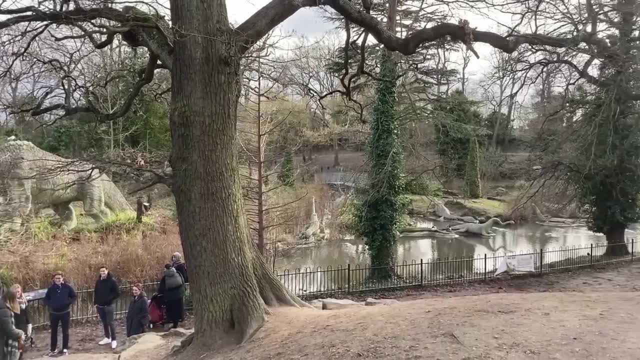 Although it kind of backfired. Working on the statues was a bit of a challenge Working within the uniformitarian framework. Owen saw the dinosaurs'. extinction as a fading away due to gradual atmospheric changes. In his mind, the age of reptiles was a more impressive age than the present. 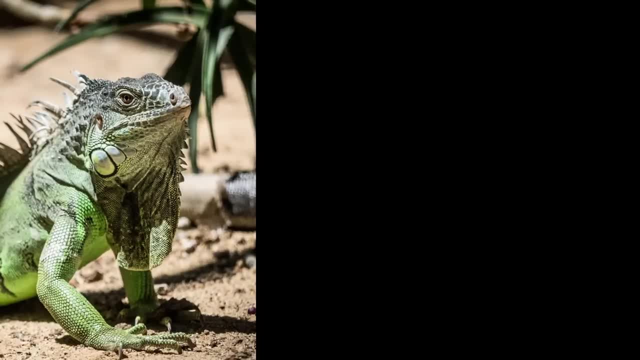 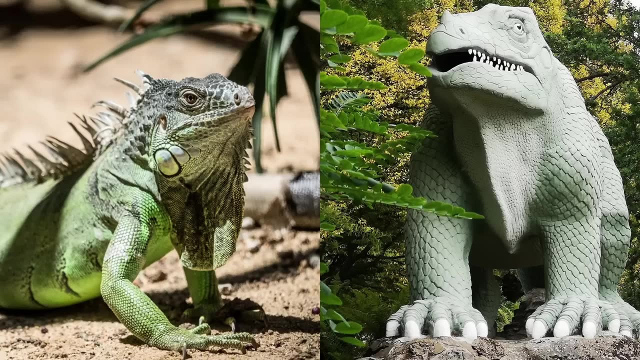 And the trend of life on Earth was a negative one. Modern reptiles were, in Owen's view, pitiful shadows of their former glory, And all other groups would one day suffer the same fate. The mammalian stature of the Crystal Palace Dinosaurs is intentional. 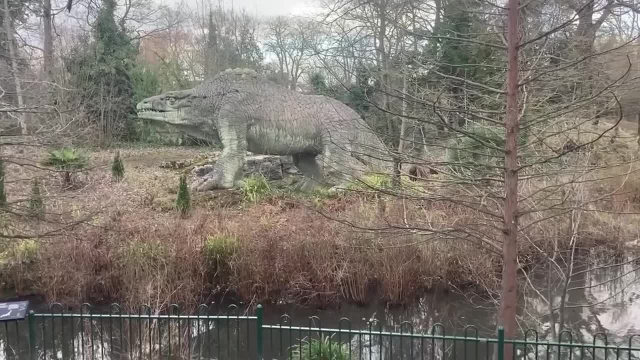 Owen wanted to evoke the size and dynamism of the dinosaurs. He wanted to evoke the size and dynamism of the dinosaurs. He wanted to evoke the size and dynamism of the dinosaurs. He wanted to evoke the size and dynamism of modern mammals like bears and rhinos. 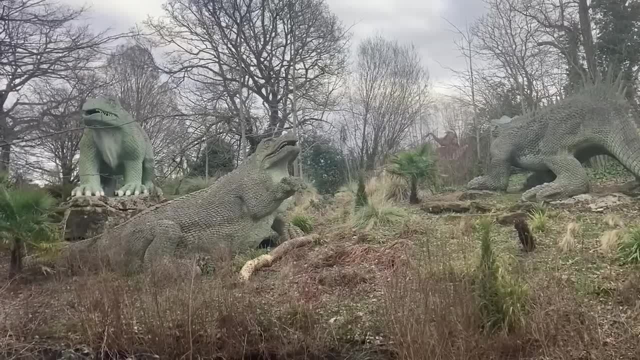 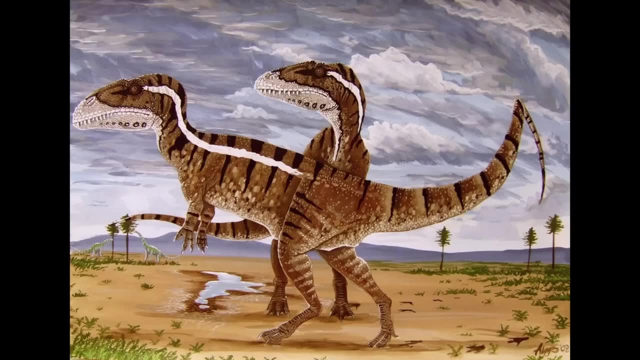 And he wanted to embed that view of a grand lost past within the public. Sadly for Owen, only a few years later, Megalosaurus was found to be bipedal. Overnight, his grand spectacle became a bit silly and old-fashioned. 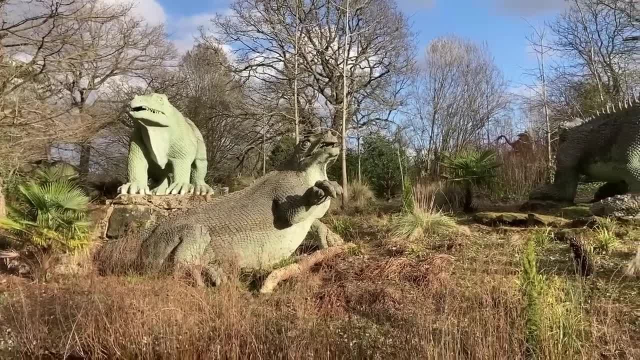 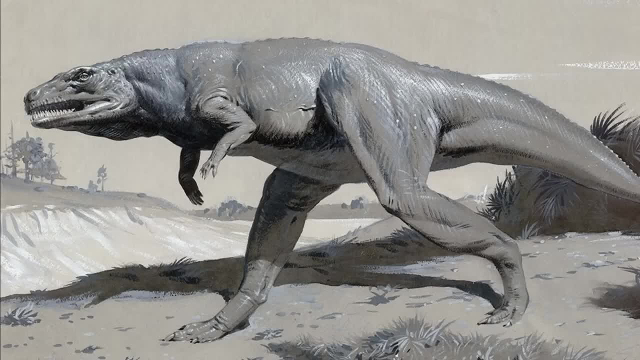 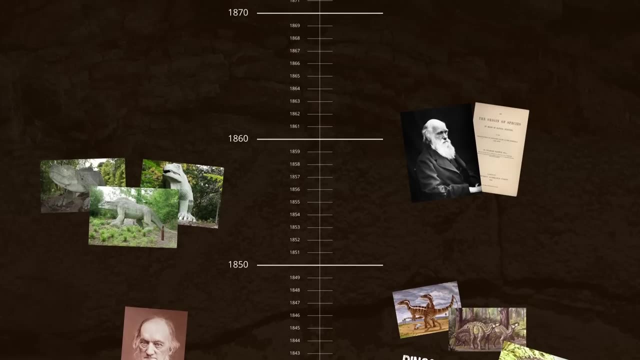 A status the statues helped confer to dinosaurs themselves. Dinosaurs were nothing but slow-witted lumbering beasts doomed to be ousted by better forms. When Charles Darwin's theory of evolution by natural selection become the dominant paradigm after 1859, it only bolstered anti-dinosaur and anti-Owen sentiment. 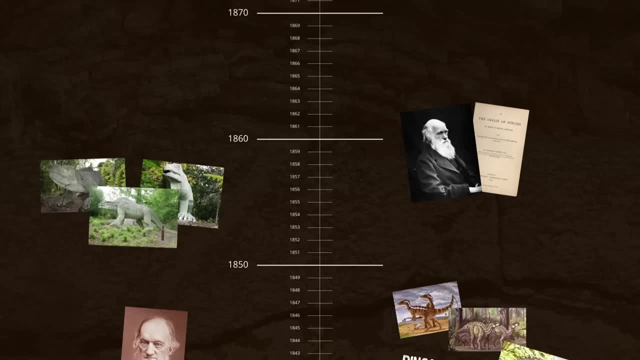 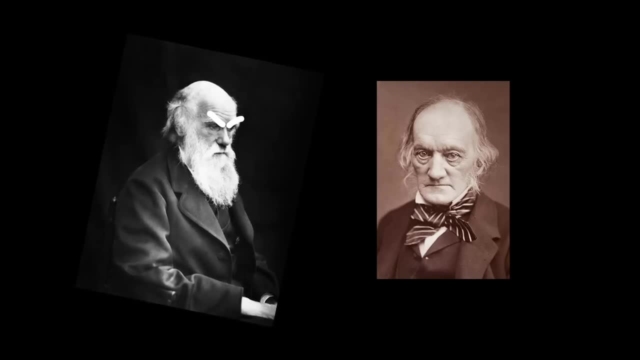 If it's survival of the fittest, then the extinct must be unfit. Darwin hated Owens, so maybe he took some satisfaction in seeing his theory crush the man's idea of a lost golden age. Darwin hated Owens, so maybe he took some satisfaction in seeing his theory crush the man idea of a lost golden age. 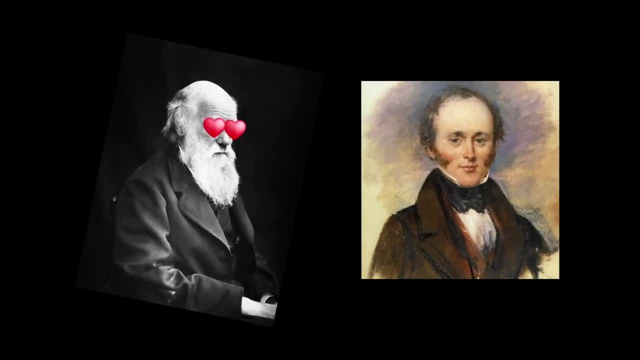 He also loved Lyell and was enthused to find a 해� flith, Lyle Giner and was enthused to find a theory that fit so well with uniformitarian belief. He also loved Lyle and was enthused to find a theory that fit so well with uniformitarian belief. 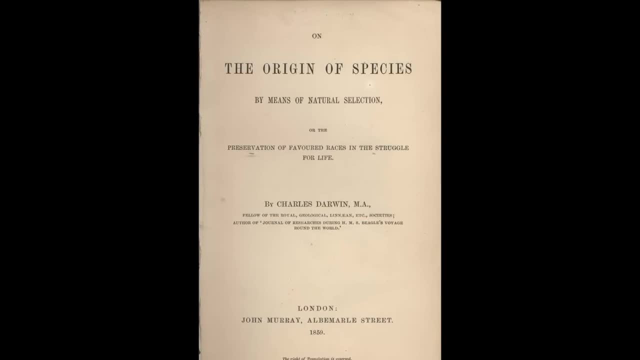 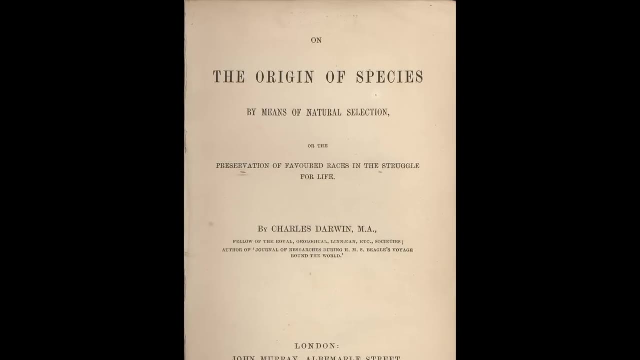 And let's not forget that on the origins of species, friends, the class disagreement over time brought with him a lenghung zusf camera. origin of species was written for public consumption Accessible prose widely distributed. Darwin too was arguably engaging in some scientific subversion by means of public support. 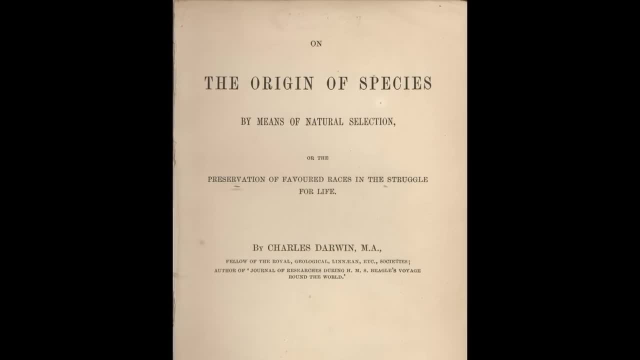 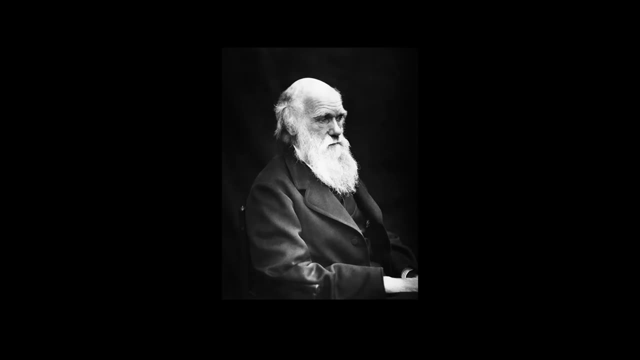 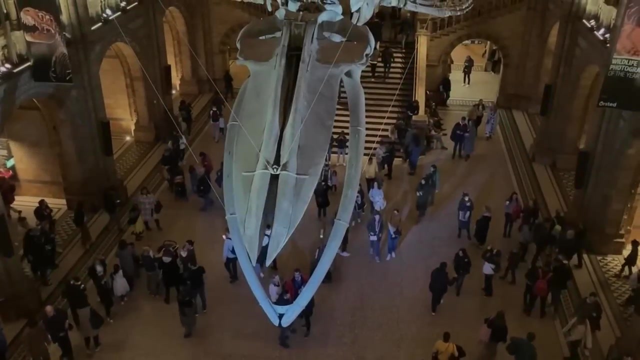 A weapon we'll see many others brandish and refine as we continue. Soon enough, Darwin's supporters got Richard Owen kicked out of high scientific society on charges of fraud, But Owen wasn't going down without a fight and he knew the perfect battleground. 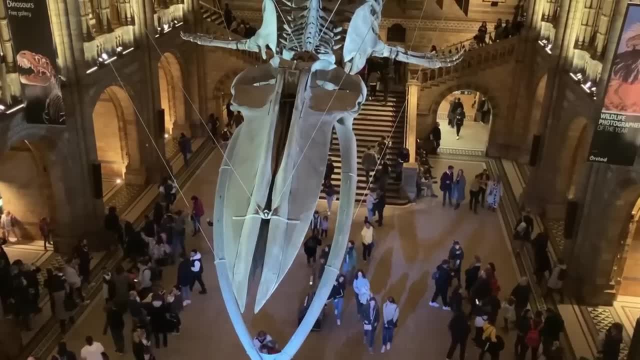 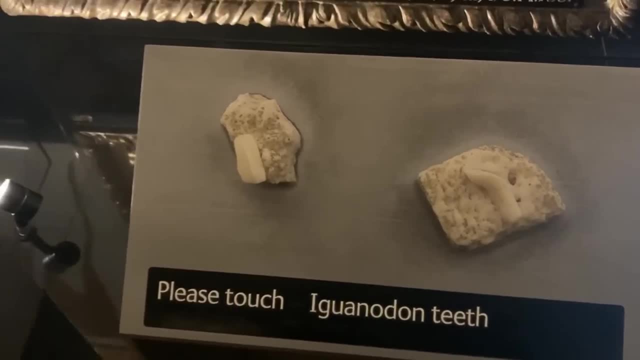 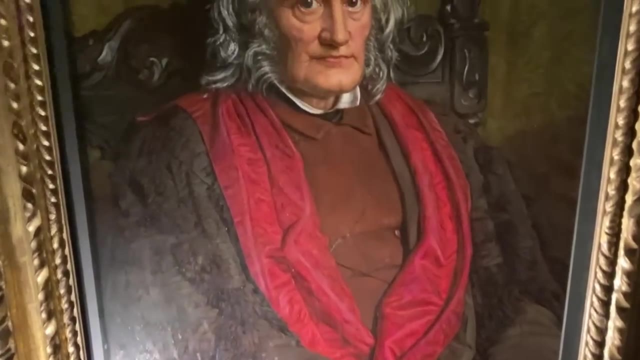 The Natural History Museum, and perhaps every science museum you've ever visited, owes a great debt to Owen. It was he who opened it to the public and shaped it to be a cathedral of accessible knowledge. Science museums had, until then, been archaic catalogues of specimens restricted to the 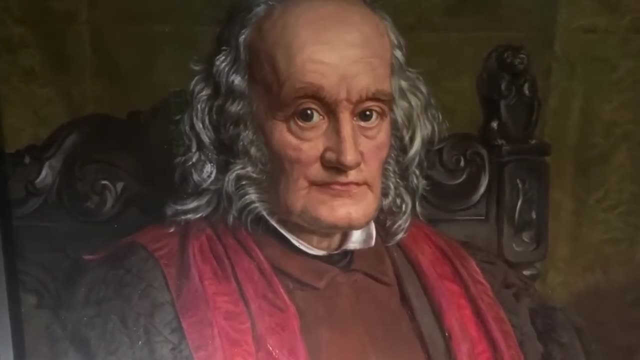 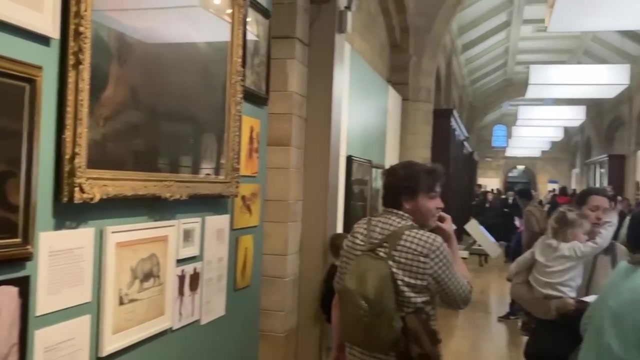 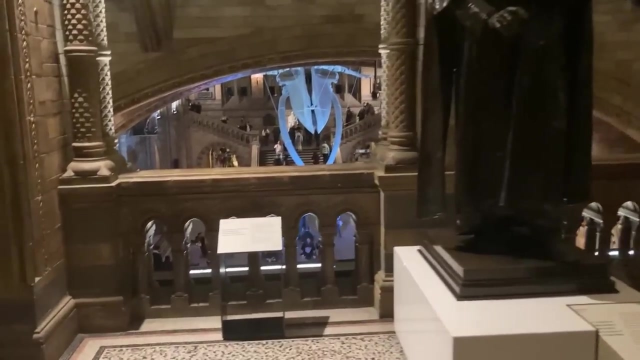 scholarly elite, But Owen saw a future where the commoners were front and centre, where learning institutions catered to us and our views on science. It's not the victory he wanted, but a victory nonetheless. He would, however, be horrified to learn that, since 2009,, his statue has been put way up. 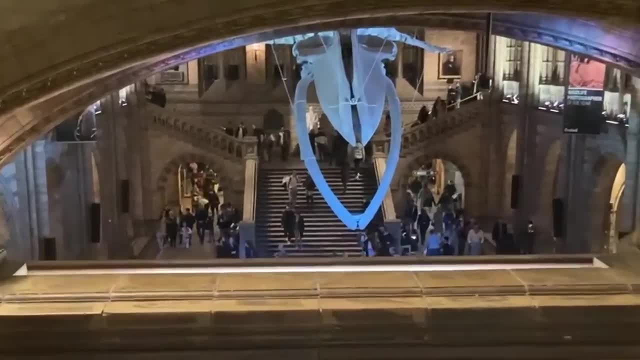 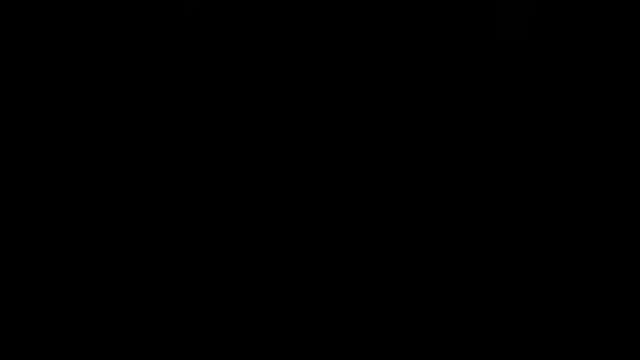 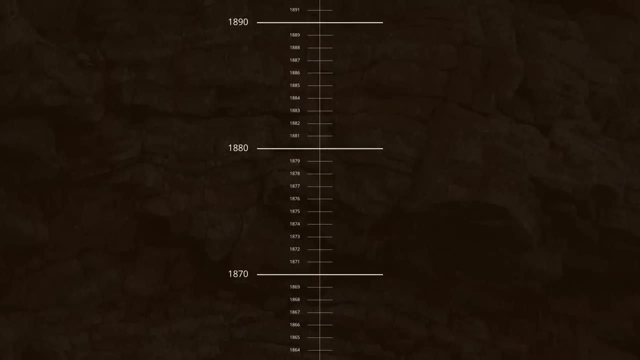 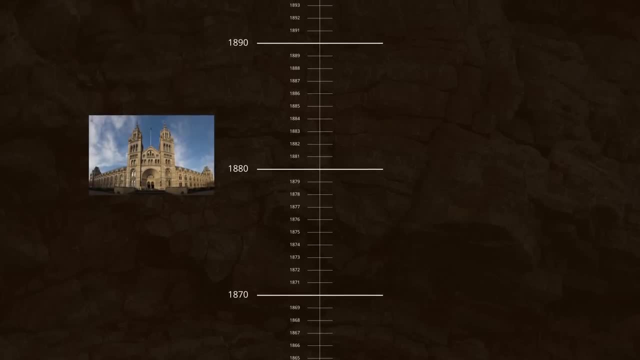 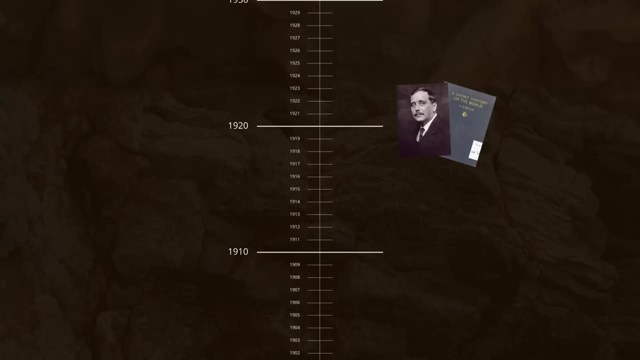 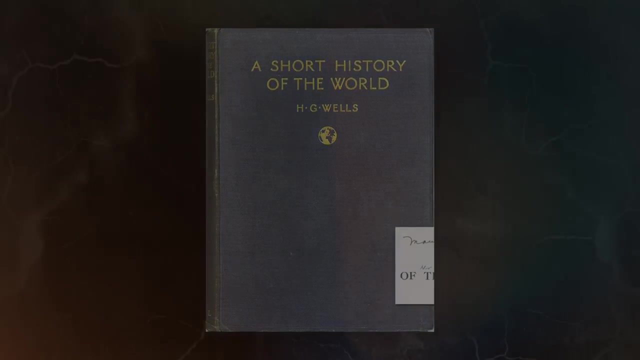 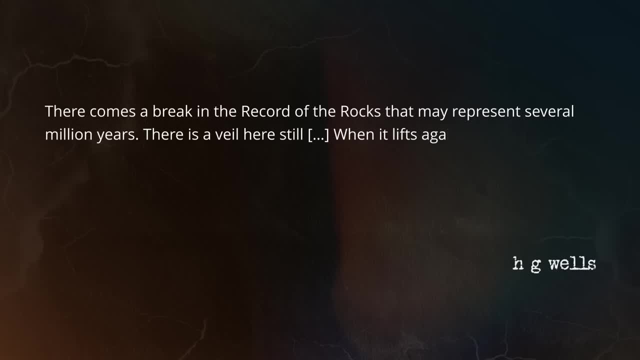 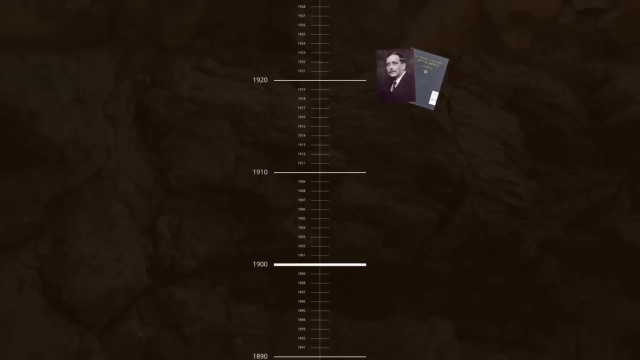 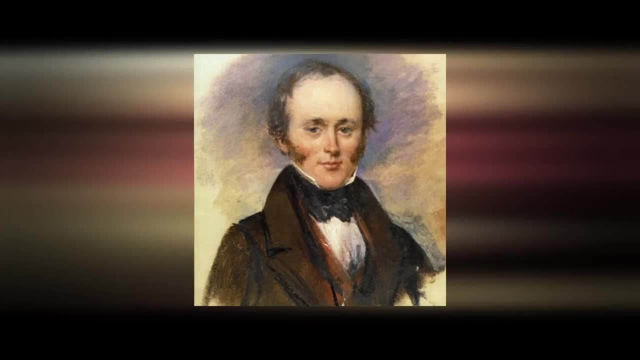 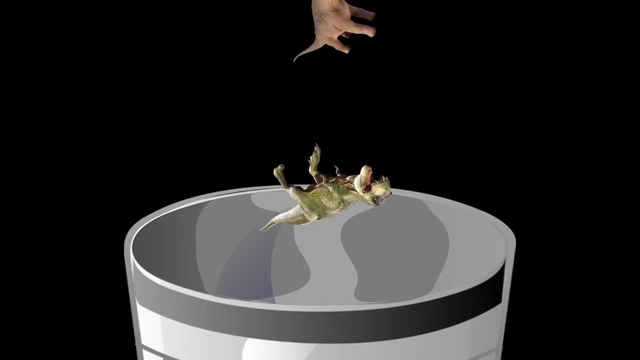 they just couldn't handle the grind. All hail our lord and saviour, Charles Lyell. Uniformitarianism's banishment of mass extinction meant no serious science could ever touch KPG, Even once new fossil evidence called the slow decline assumption into question. 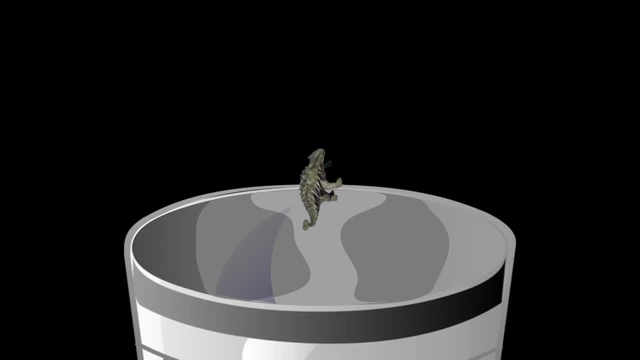 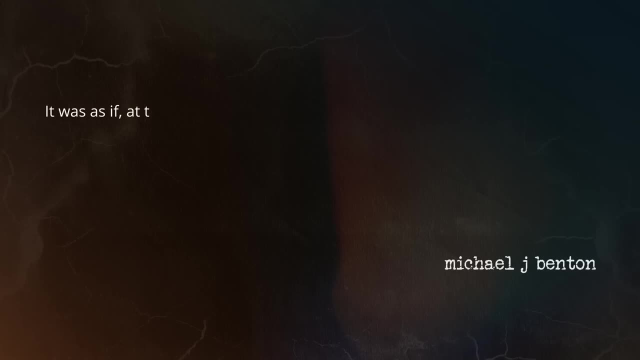 stigma turned the question into a wastebasket for random ideas that nobody actually believed or cared about. In the words of paleontologist Michael Benton, it was as if, at the mere mention of dinosaur extinction, scientists breathed a sigh of relief and felt freed from. 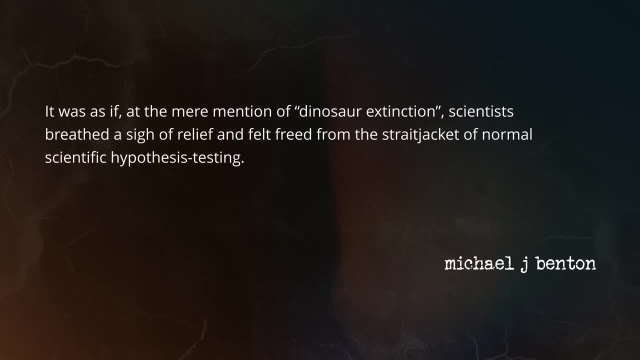 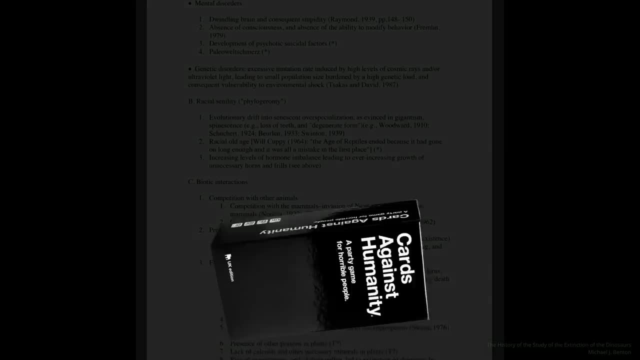 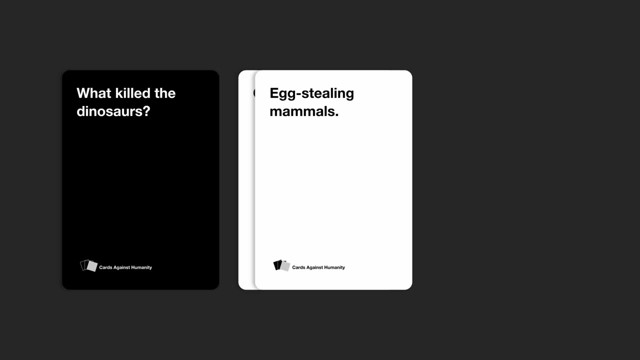 the straitjacket of normal scientific hypothesis testing. The list of theories proposed at this time in actual scientific papers reads like a game of cards against humanity. What killed the dinosaurs? Dinosaurs, caterpillars, egg-stealing mammals, excessive wetness, excessive dryness, cataracts. 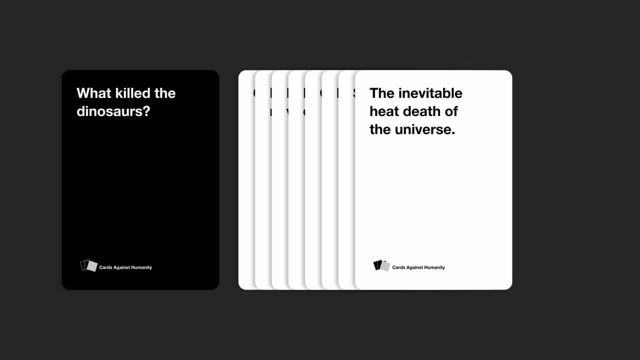 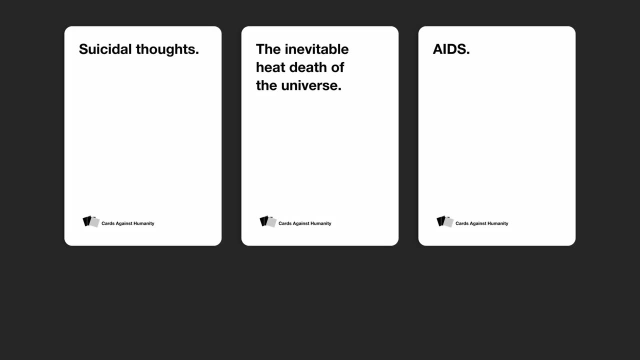 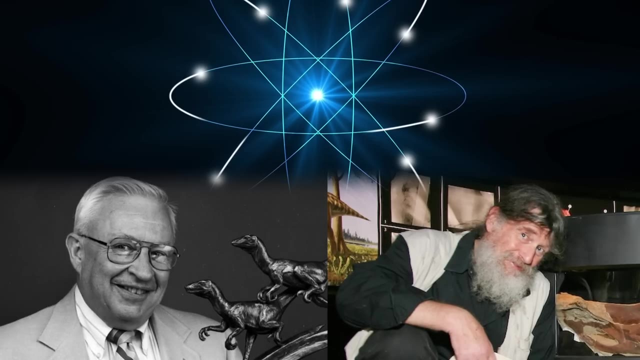 boredom, suicidal thoughts, the inevitable heat death of the universe, AIDS, AIDS. Oh sorry, those last three were actual cards against humanity cards And actual theories for the dinosaurs' extinction- What the hell. Thankfully, two developments in the mid-1900s reduced this flow of baseless theories. 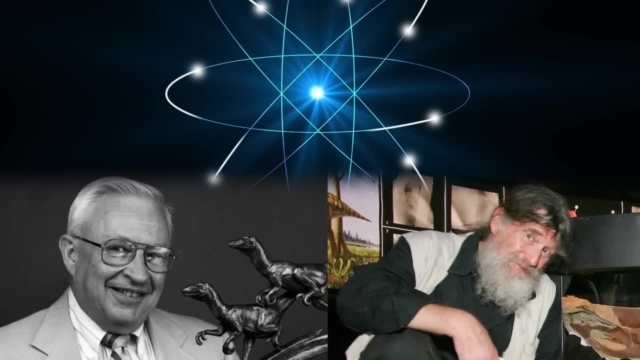 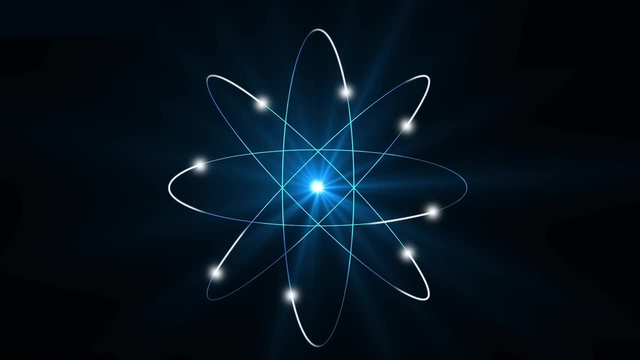 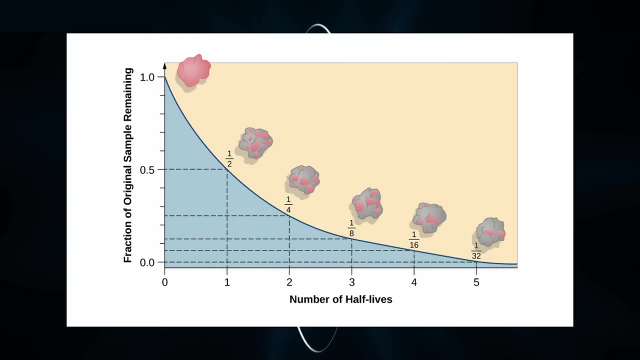 Alone they. They couldn't break the uniformitarian monopoly, but they dented the edifice enough for what came after to prevail. First was the invention of radiometric dating. By studying the ratios of radioactive elements in ancient rock, geologists had a much more accurate view of deep time, one that hooked 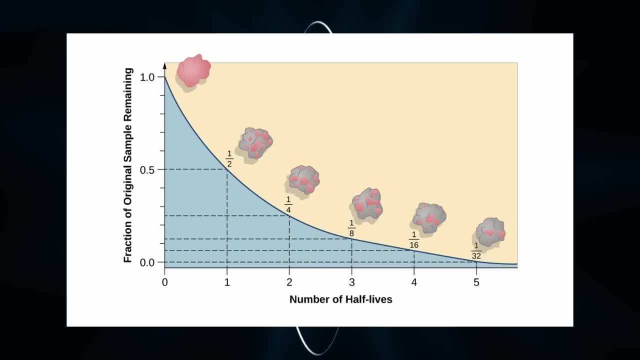 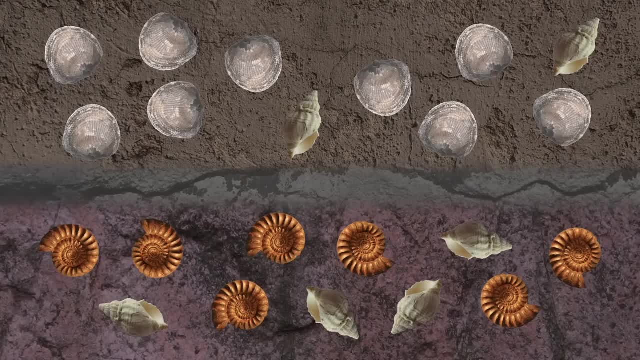 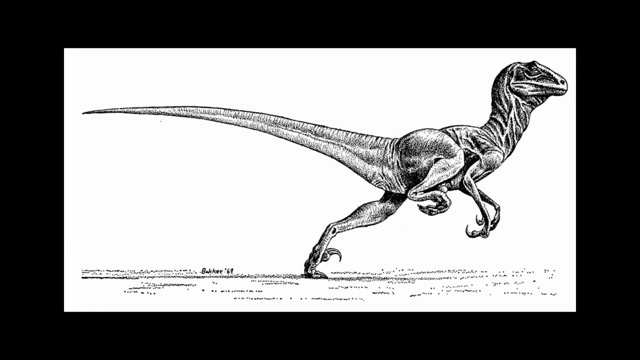 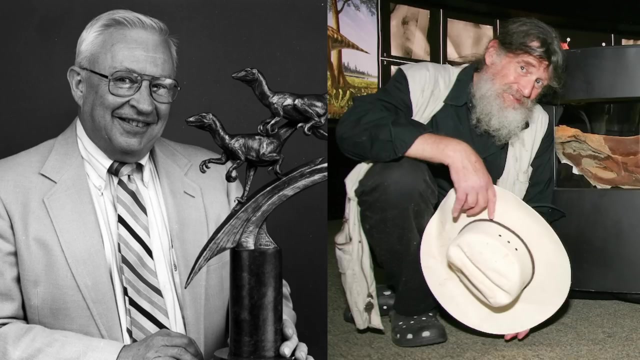 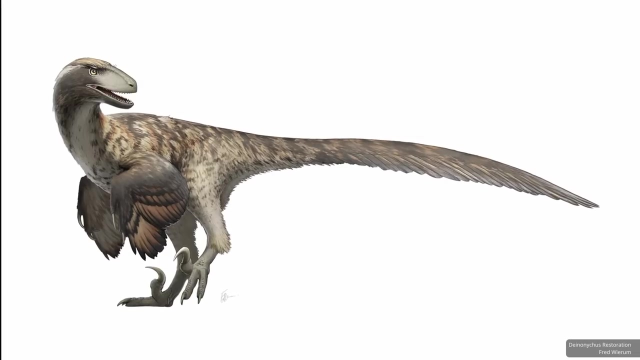 short, short, short, short, short, short, short. joy KELLY AND CRA Über And now. It took time to filter through to the general public — we'll get there in a bit — but at last scientists saw dinosaurs not as slow and stupid, but dynamic, warm-blooded and 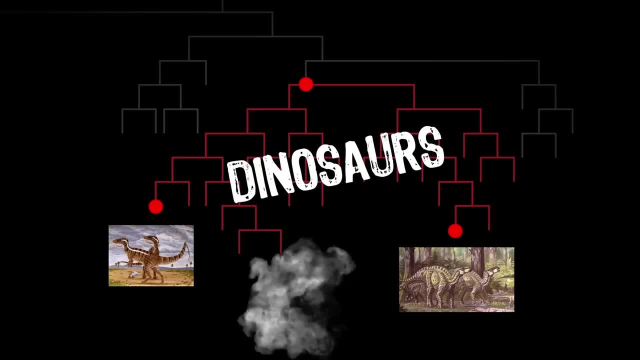 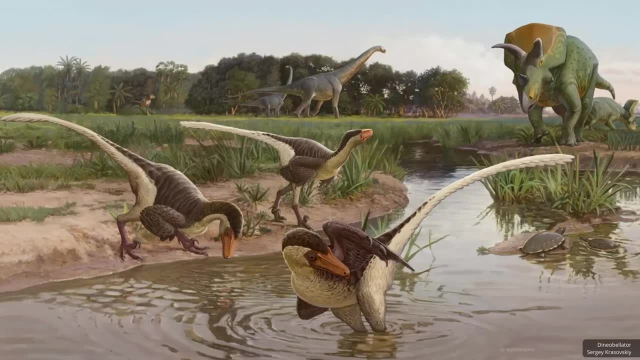 bird-like. It was around this time that the bird family tree was put back into Dinosauria, for instance. Together this evidence painted a picture of a vibrant, well-adapted group, killed not by evolutionary obsolescence but something quick and, dare I say, catastrophic. 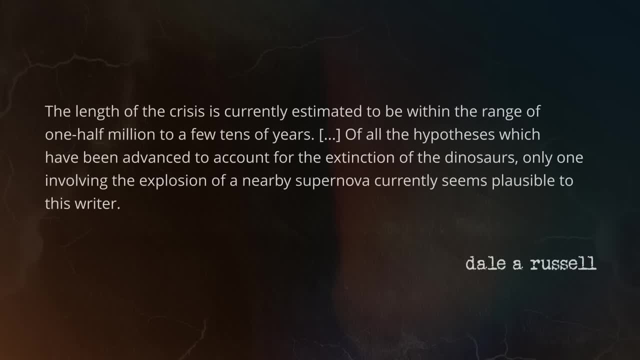 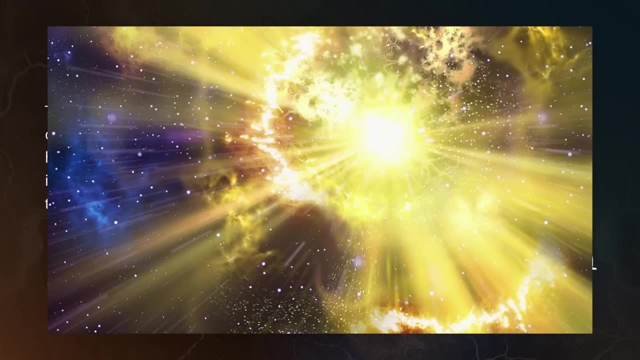 A 1979 summary by paleontologist Dale Russell came to the conclusion that extinction had to have been abrupt. His favourite theory was a supernova. but he, like everyone else tentatively reviving catastrophism, had no real evidence for their killing method, so ineffectually bounced. 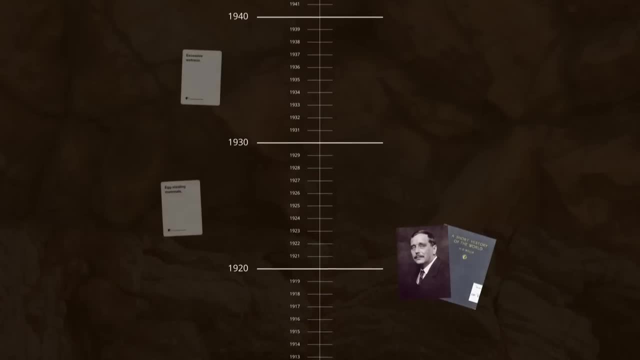 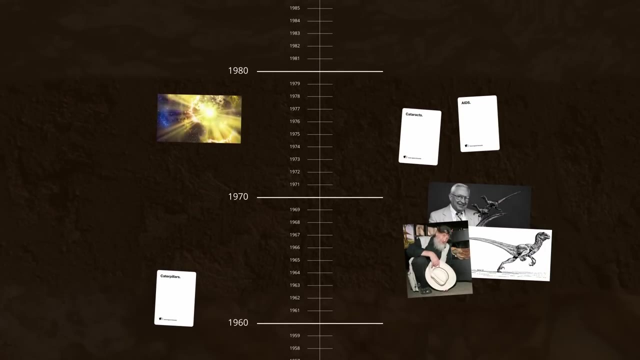 off the dominant paradigm, Chinks in the armour, but still the old doctrine held. Could anything displace the outdated uniformitarian dinosaurs from their dominance? Oh yeah, that was the cliche that was supposed to be beneath me. Well, in for a penny. 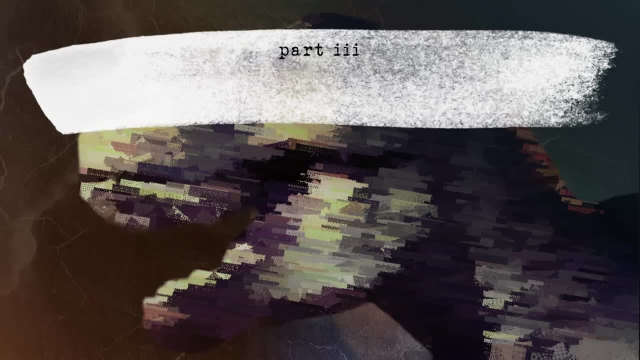 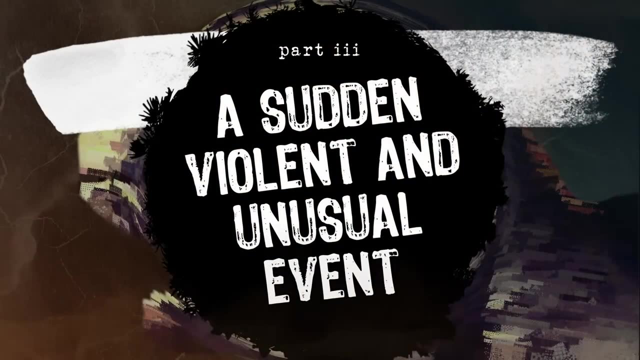 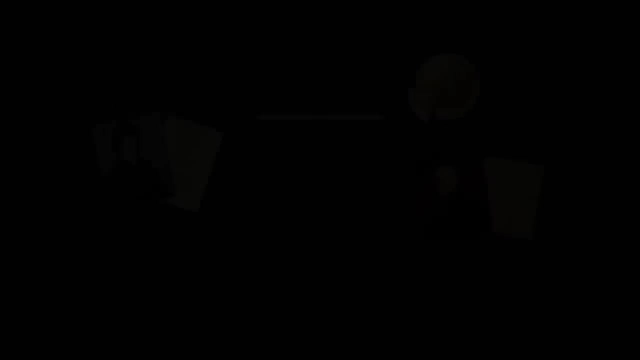 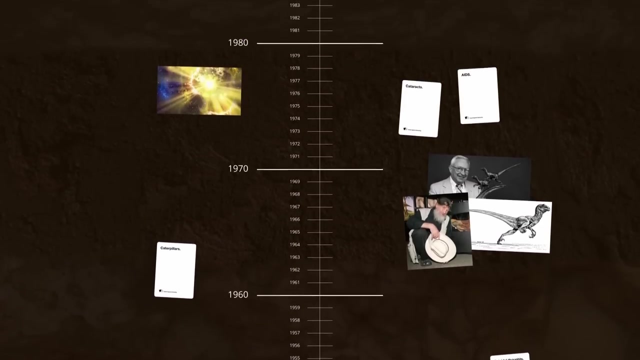 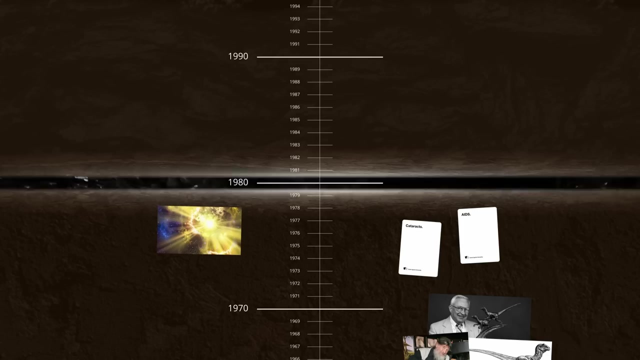 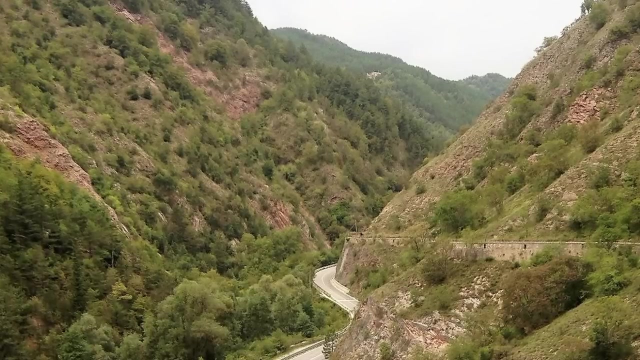 Part 3: A Sudden, Violent and Unusual Event. There are two KPG boundaries: 66 million years ago and 6-6-1980.. This is Bottaccione Gorge near the Italian town of Gubbio. Sadly, I couldn't expense a trip to. 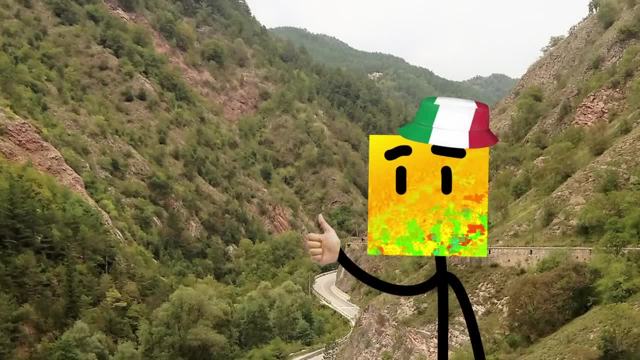 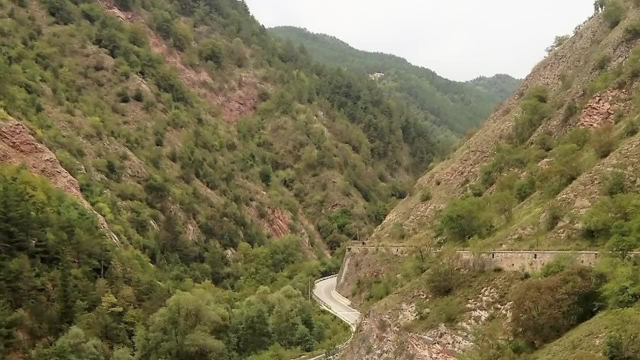 Italy for this video, so you'll just have to pretend I'm there this time. It may look harmless, but in 1980, this gorge unleashed an inferno upon Earth science. Even if you think you know how crazy this is about to get, you don't. 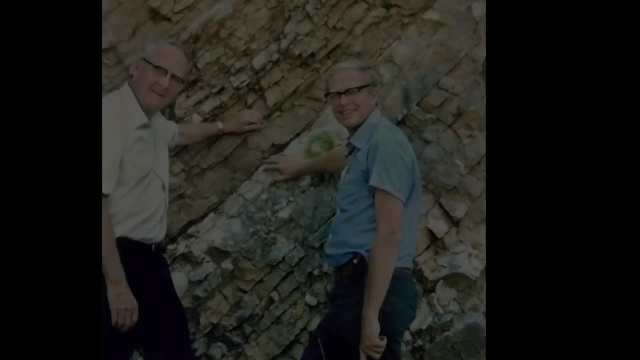 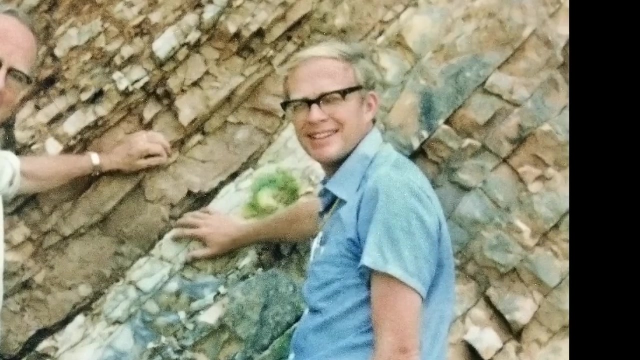 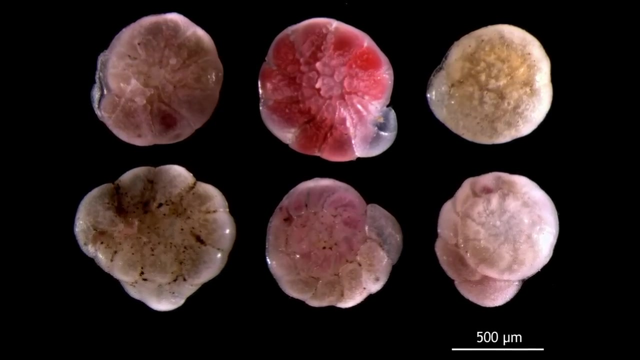 Walter Alvarez had made plenty of trips to Gubbio in the 1970s. The young geologist knew this site. an ancient seafloor had one of the best KPG boundary layers in the world. It was well known for its impressive fossil stock of single-celled organisms called forams. 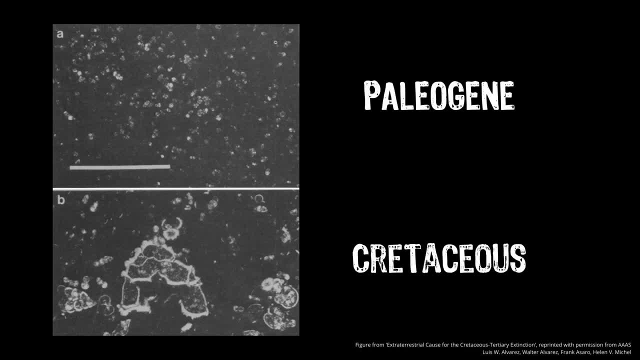 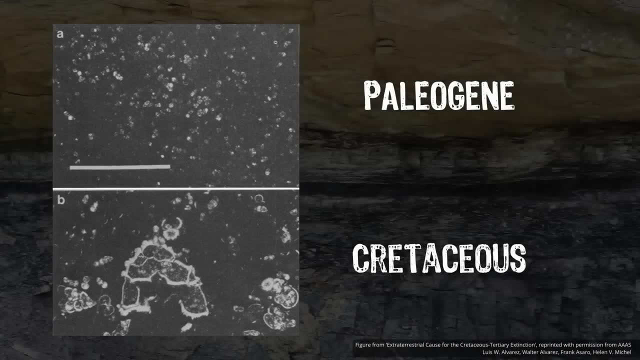 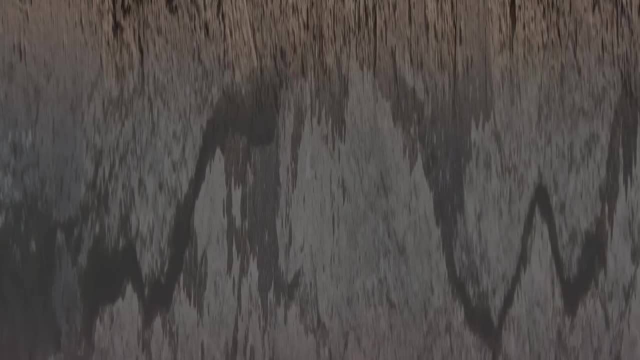 Forams above and below the boundary were significantly different, a hint of the severity of the extinction that also claimed the dinosaurs. Alvarez was struck by the slenderness of the dividing layer, a stark black line dividing one world from the next. How long had the Biotic Switch taken? 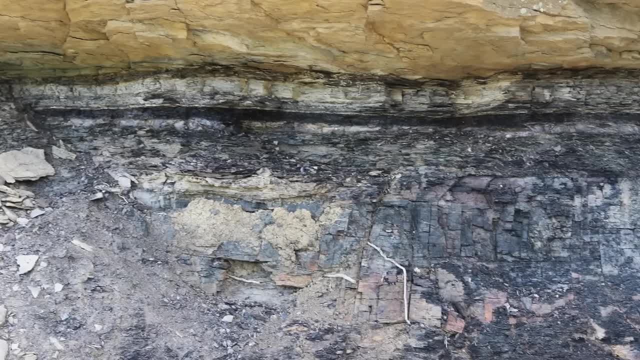 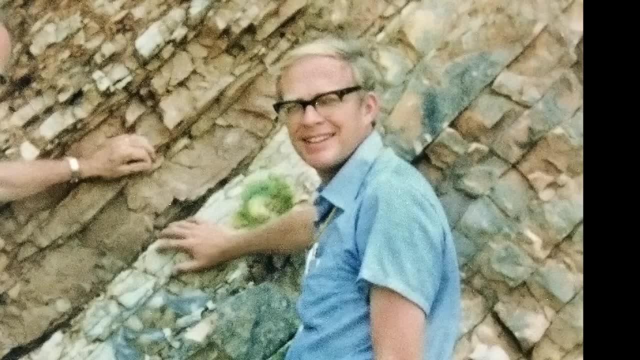 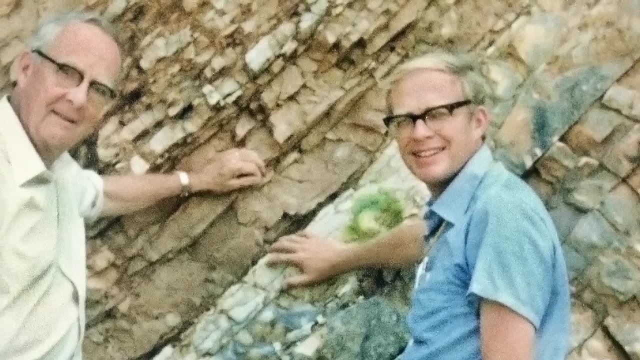 How wrong exactly had Lyle been? Radiometric Dating had narrowed KPG to at most a million years, but no-one could do better. Alvarez, though, had access to a resource his predecessors lacked: his father, Luis Alvarez, was a Nobel Prize winning physicist. His achievements already included discovering new subatomic. 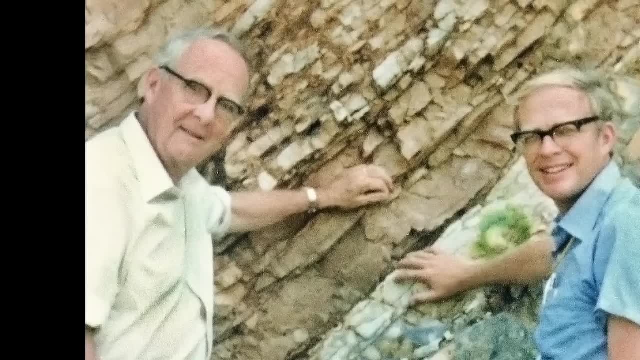 particles and X-ray scanning in Egyptian. You can read his pamphlets and his estimates about his work in the Saspwit and Alvarez papers at redstoneaibsuuk Pyramid. If anyone could bring the full might of physics to bear against this problem, it was him. 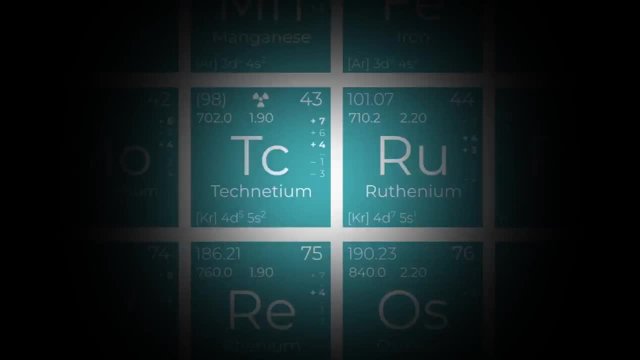 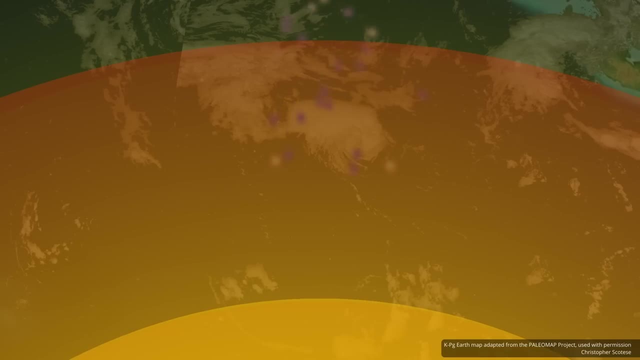 After a false start with the element Beryllium, the pair had a brainwave Iridium. Back. when the Earth was molten, most of its iron sunk to the core and took Iridium with it, leaving the element scarce in the crust. A persistent sprinkling of space dust has 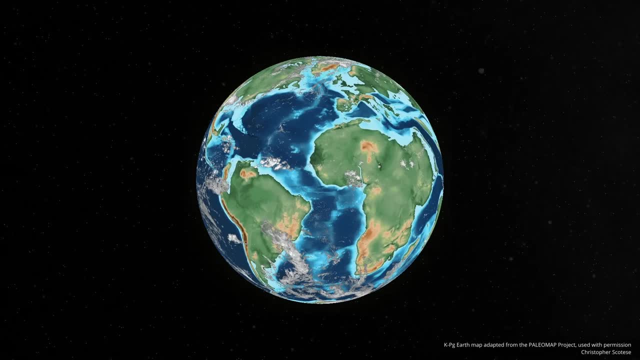 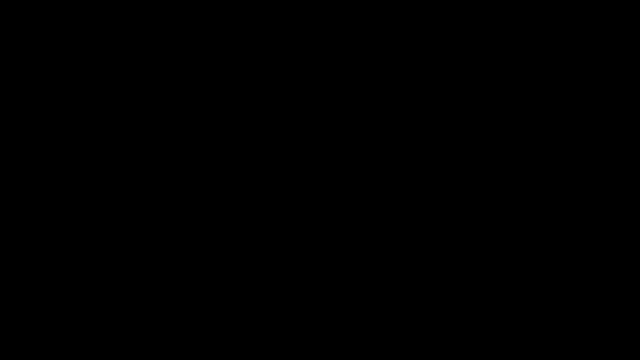 however, deposited some Iridium as replacement. Assuming a constant rate, one could simply count Iridium atoms across a layer to determine how long it had taken to form, And by simply I mean it required months of pain and frustration. using new technology, few people in the world could 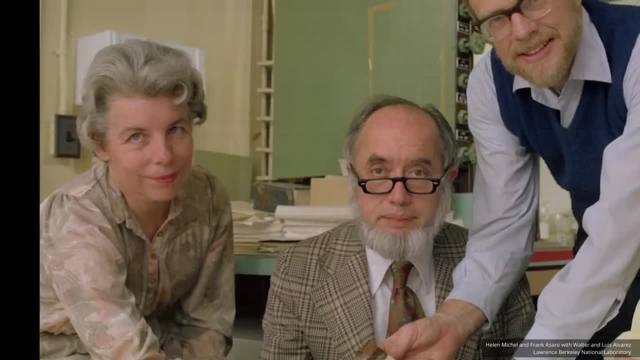 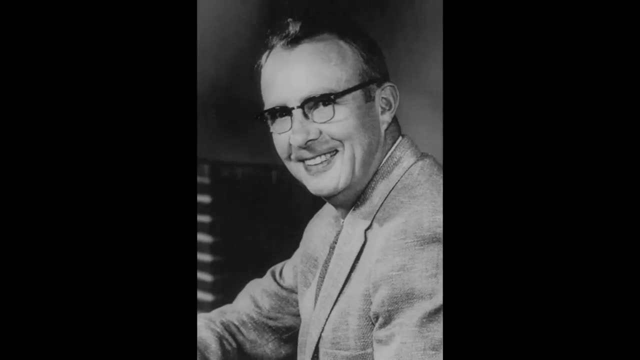 operate. Two of those people were Frank Asaro and Helen Michael, nuclear chemists, who received samples of Gubbio Rock from the Alvarez duo. After months of silence, Louise received a phone call. Hey, Frank, how's it going? Louise, you need to drop in. 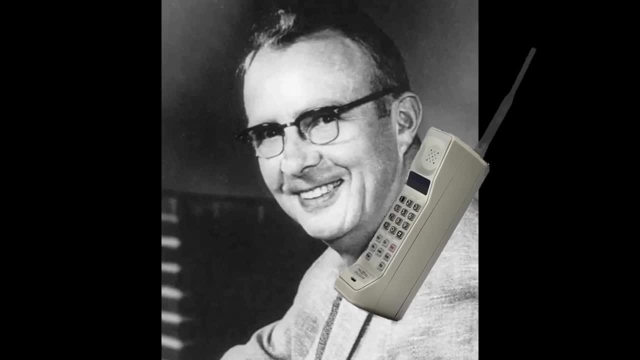 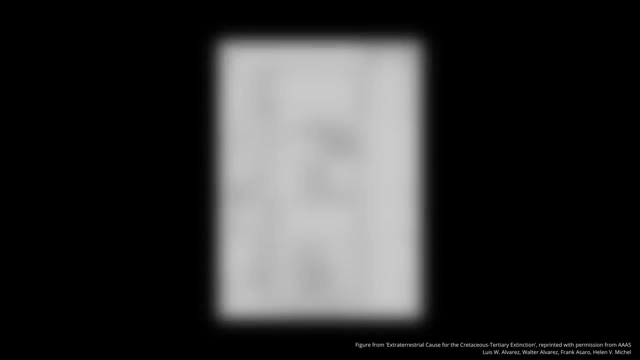 Everything and get here immediately. There's something you have to see urgently. and bring water, because this is big, Something is seriously up. Get here now, Okay, thanks, Bye. Huh. What Asaro showed them became perhaps the most important graph in geological history. 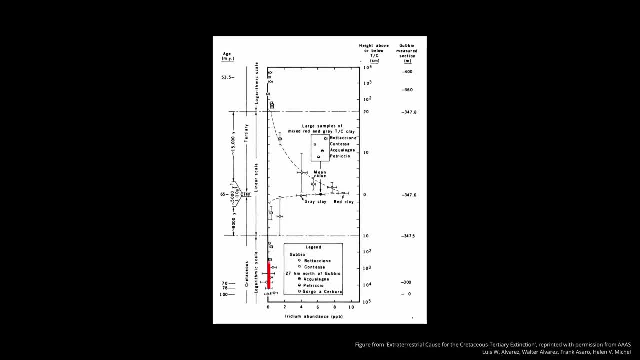 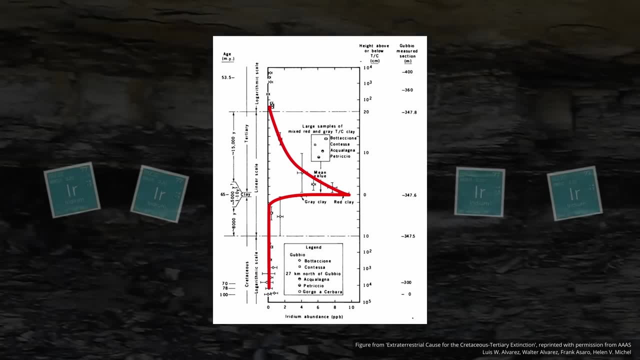 This is the Iridium spike. Iridium density in the sampled sequence jumps to 30 times its background level near the moment of 4m extinction. In other words, there was an Iridium layer at the extinction horizon. If Iridium deposition 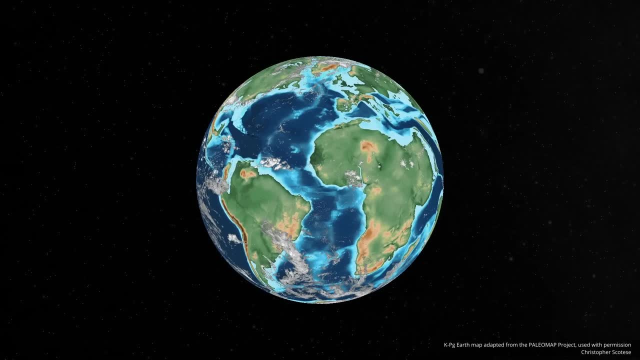 rate was constant, this implied a duration far beyond anything they expected. Was Lyell's ridiculous estimate right after all? Or were they mistaken in assuming Iridium had arrived at a constant rate? Perhaps, and just pie in the sky, speculation here. 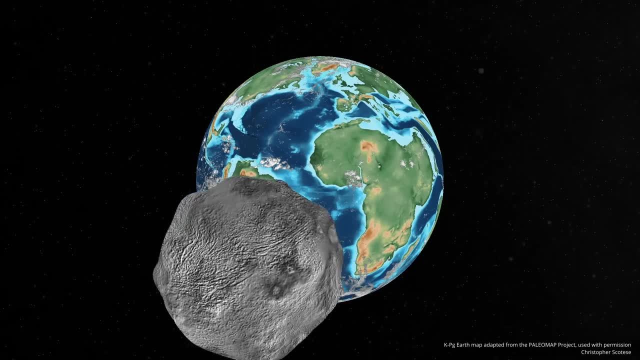 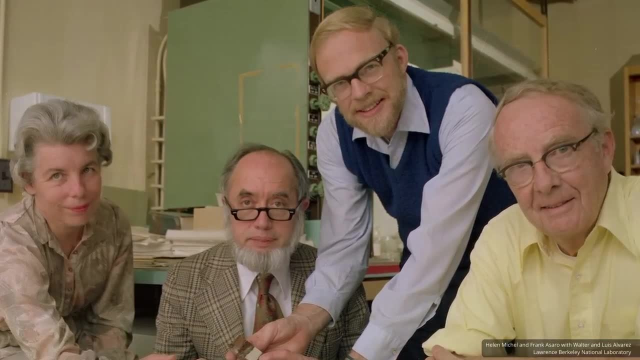 a whole load more space dust than usual had turned up all at once. The team faced a choice. Would they interpret the data as a victory for uniformitarianism, or would they delve deeper and risk upending the status quo? Let's find out in this episode of Iridium Anomaly. 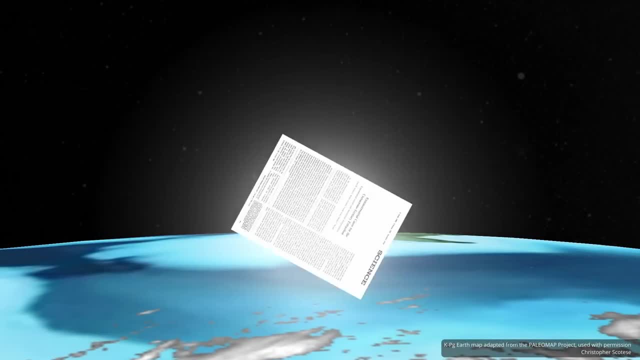 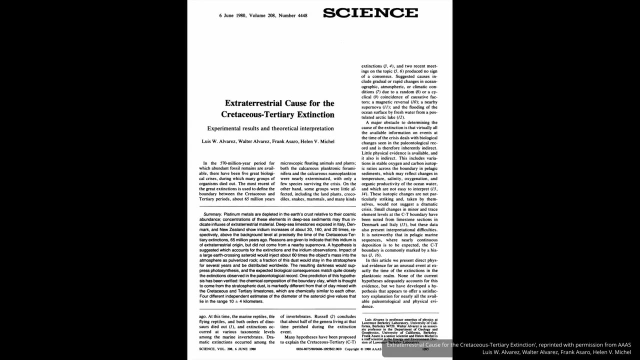 On the 6th of June 1980, the journal Science led with a paper twice as long as its usual. lead entries- Alvarez Alvarez, Asaro and Michael covered four items: An analysis of the Iridium Anomaly. a rejection of Dale Russell's supernova as an explanation based on a study of plutonium. 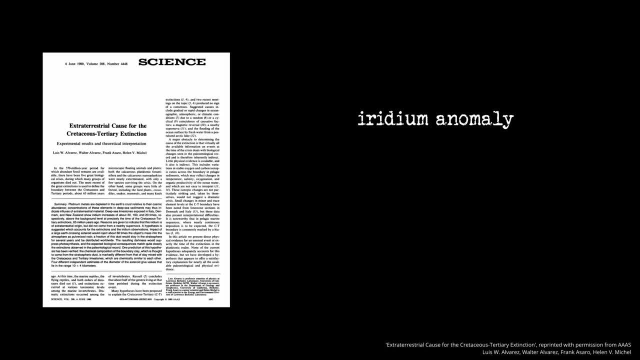 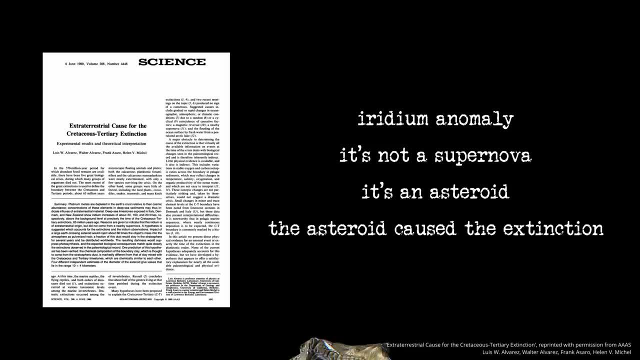 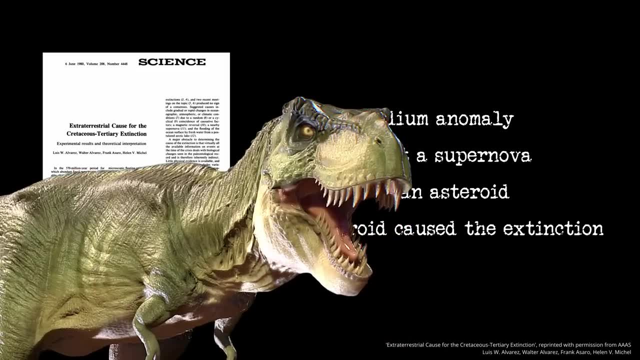 a study of the Iridium Anomaly. a study of the Iridium Anomaly and a proposal that such an asteroid caused the KPG extinction, the dinosaurs among its victims. And it was at this moment that everything went haywire. 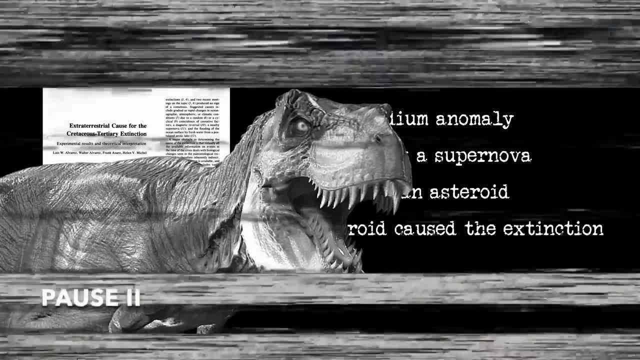 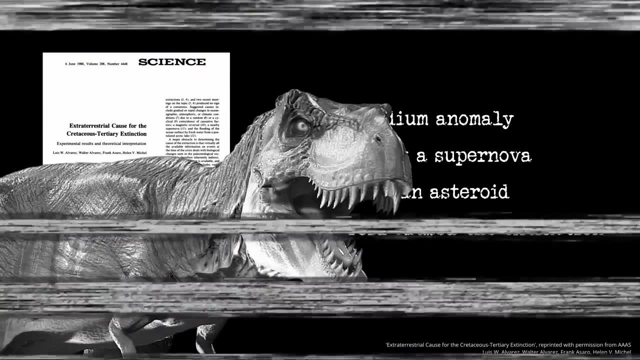 In fact, the Alvarez impact hypothesis had been shopped around conferences for many months prior, as they recruited others to verify data. It was already quite the talking point. so the paper wasn't the bolt from the blue I've made it out to be. Reality has failed my metaphor. 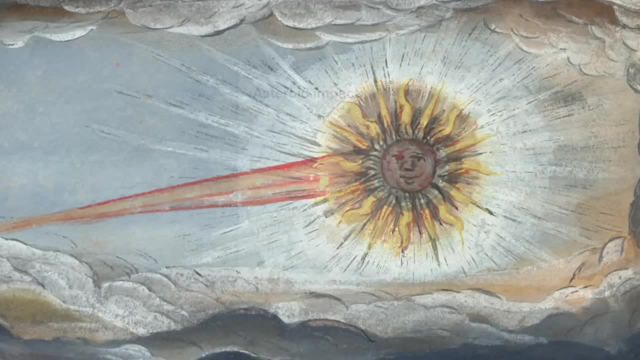 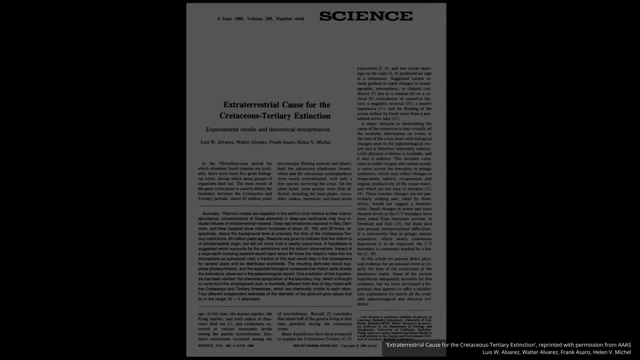 Asteroid-induced extinction was not a new idea. Yet in a uniformitarian field, unfounded suggestions of asteroid were always destined for the slush pile. The Alvarez paper broke through on two fronts: It had evidence and it made testable hypotheses. 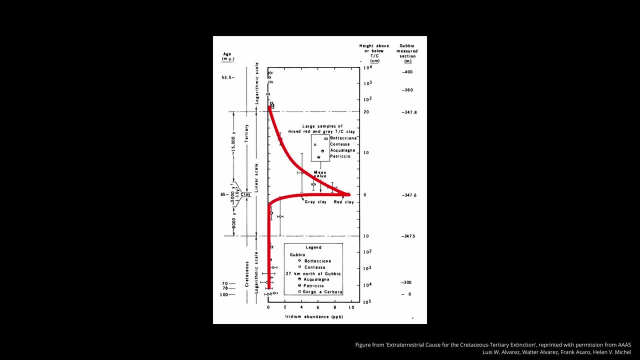 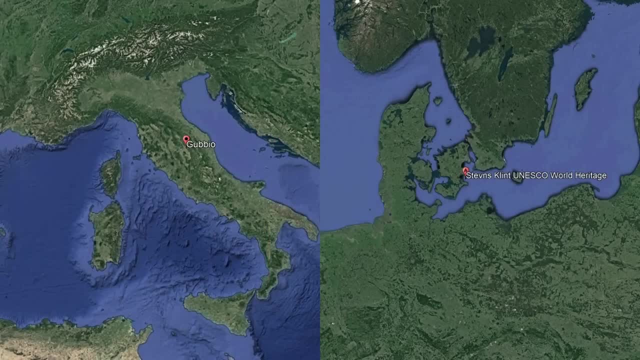 The evidence consisted of the Iridium spike at Gubbio plus a matching spike in Denmark. Further chemical analysis confirmed the shock result. In both cases the Iridium had been deposited quickly. The hypotheses were that more spikes would be found at KPG boundary layers around the world. 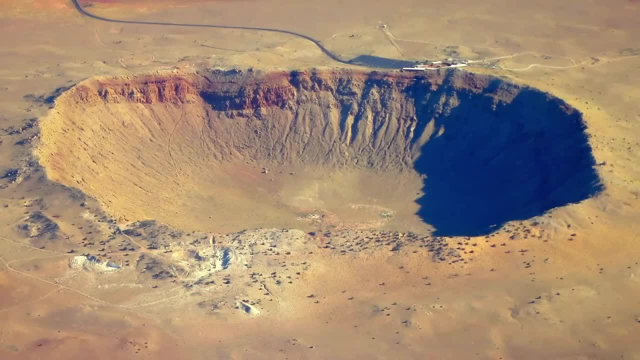 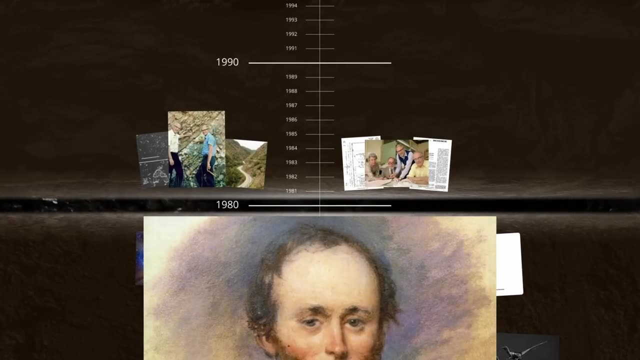 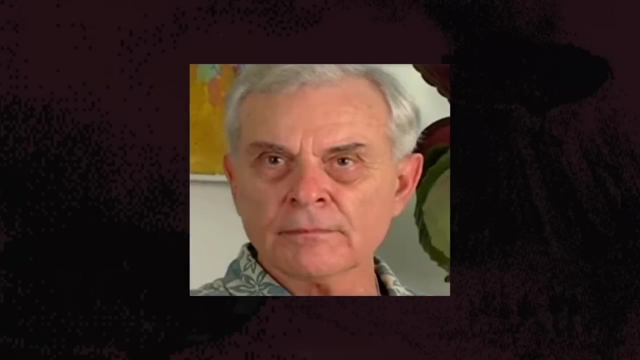 and that there was a 100 km wide crater hiding somewhere. The stage was set, The players took their places. The showdown was about to commence. Dr William Glenn is a geologist and historian of science. His specialty is understanding how science works in times of crisis. 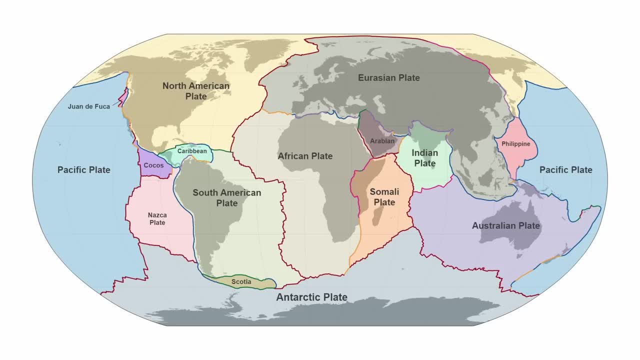 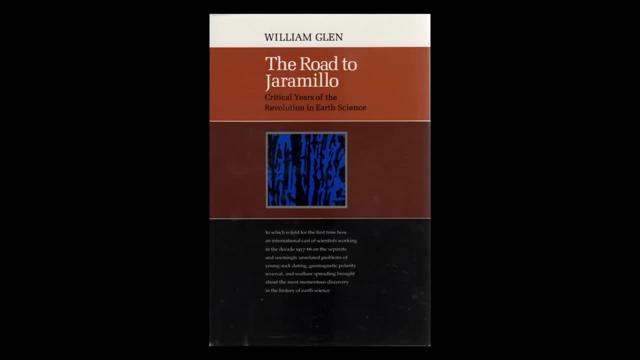 He began with a theory post-mortem of the plate tectonics revolution of the 1960s, another controversial upheaval in earth science. Glenn later published his findings in The Road to Jaramillo. While he came to some striking conclusions about scientific process, he regretted joining the party late and decided his 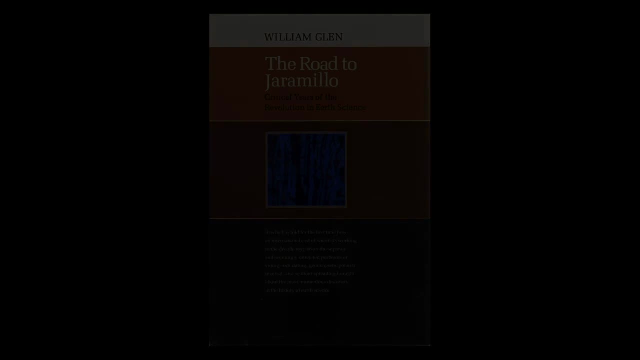 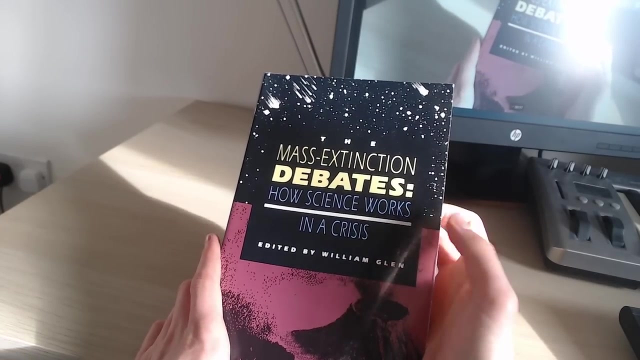 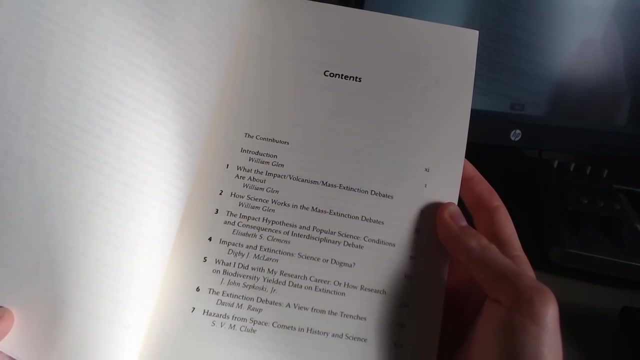 next venture must be an ongoing crisis, one he could observe as it developed. In 1983, he planted his flag in the building. uproar over Alvarez and the mass extinction debates from 1994 is the result. Two chapters from Glenn focus on his own studies, while the rest are articles from debate. 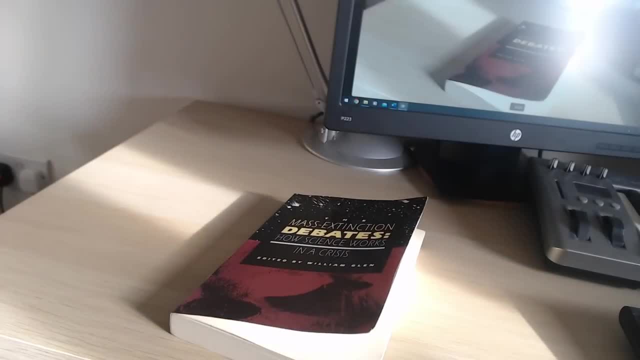 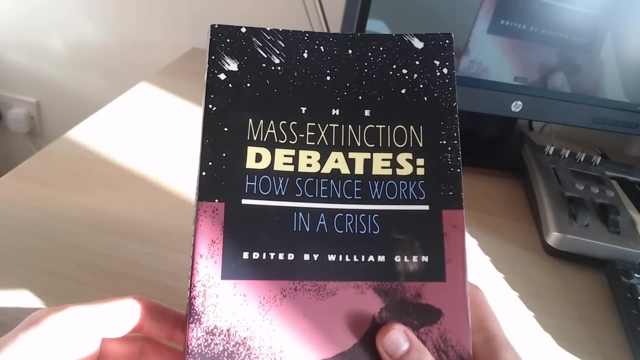 figureheads and commentators. This video wouldn't exist without the book, particularly, as we'll see later, the chapter from political sociologist Elizabeth Clemens, so I'm greatly indebted to it. Nothing else has so thoroughly narrated all the chaos, And I'm about to condense it into like 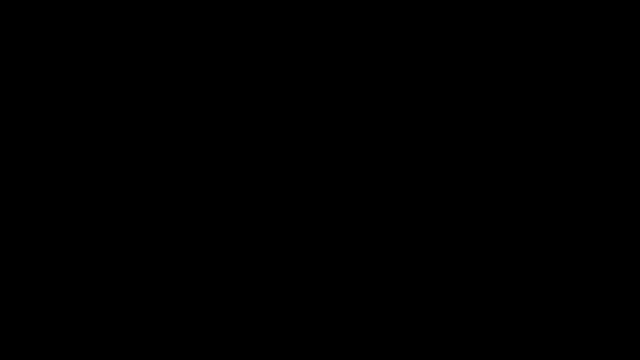 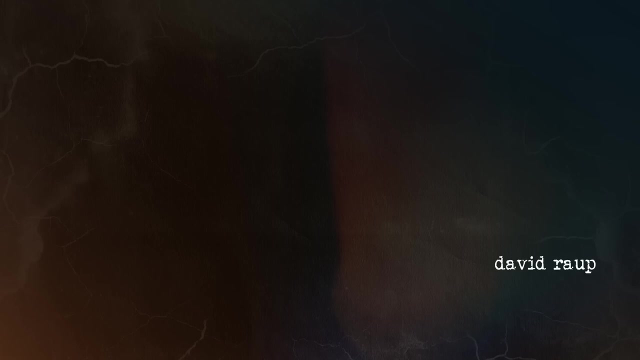 20 minutes, so wish me luck In the mass extinction debates. paleontologist David Raup recounts his initial reaction to the impact paper. Alvarez must be wrong, and it should be easy to show that he is wrong. After all, he is a physicist unfamiliar with the data of geology and 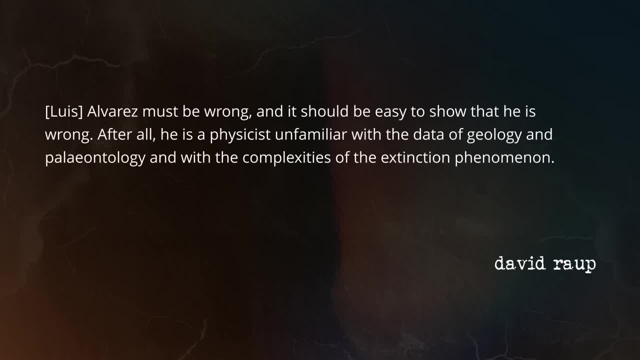 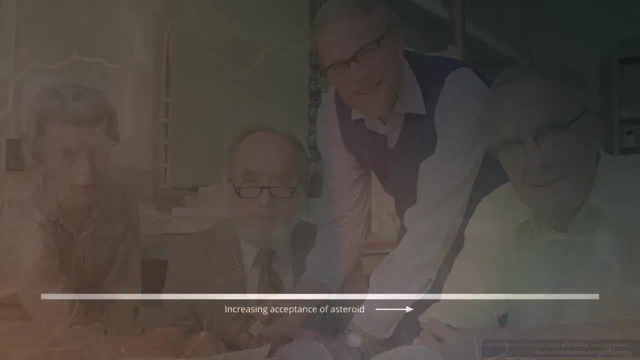 paleontology and with the complexities of the extinction phenomenon. Raup's response is indicative of a wider trend that plagued the Alvarez team upon splashdown. Faith in Alvarez depended heavily on a given researcher's field. On one extreme you had the astronomers. Gene Shoemaker had already. 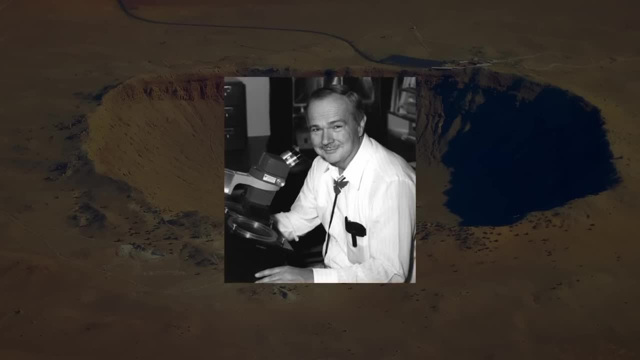 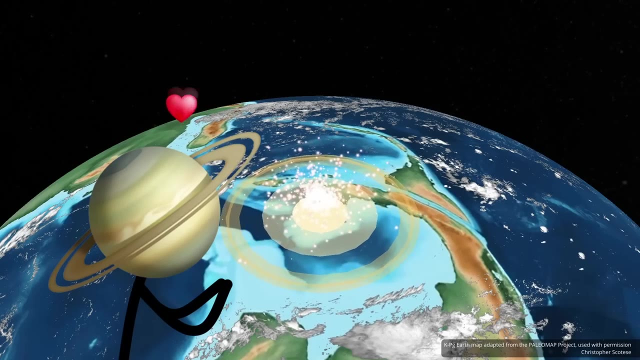 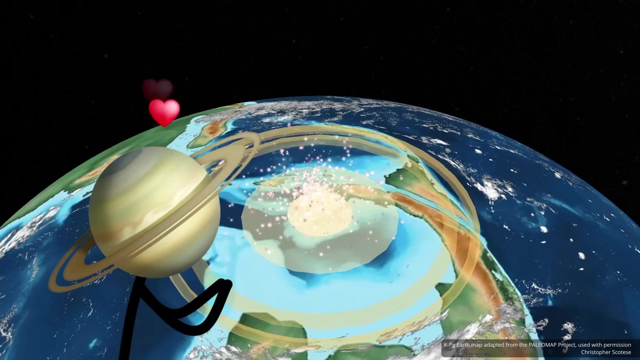 convinced astronomers that asteroids have shaped geological history. breaking free of uniformitarianism ahead of time, Astronomers thus embraced the impact extinction theory instantly. They knew enough about asteroids to know impact was likely and too little about the other disciplines involved to know why extinction might not be. Physicists and geochemists were. 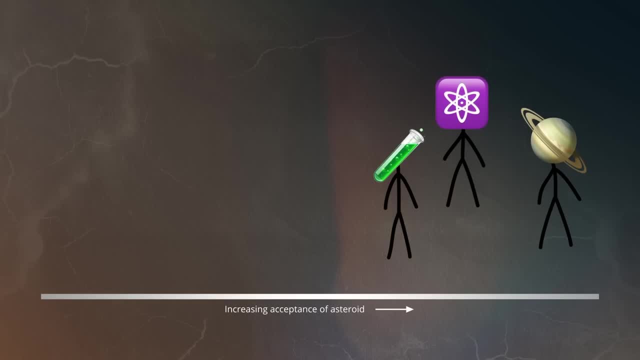 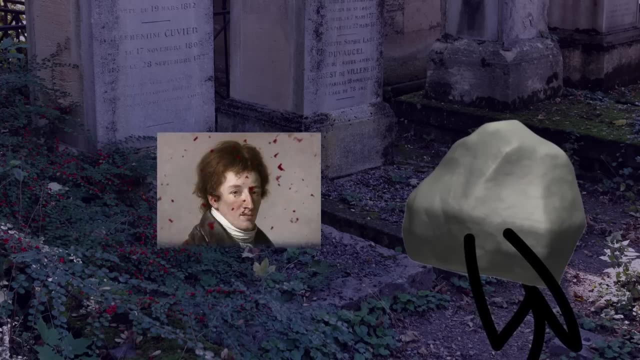 also quick to fall behind the theory. Iridium analysis fell right into their wheelhouse, and Luis Alvarez was one of theirs. Geologists, on the other hand, were horrified to see catastrophism resurrected- Walter Alvarez, a geologist himself. 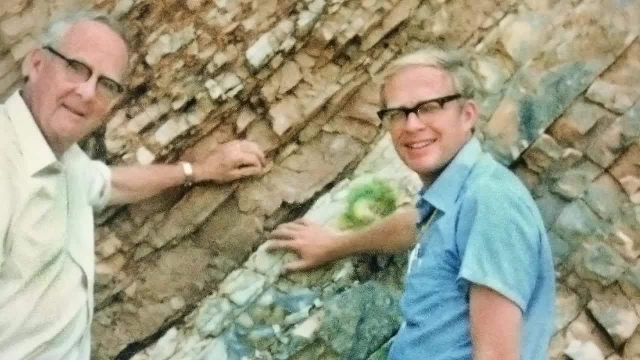 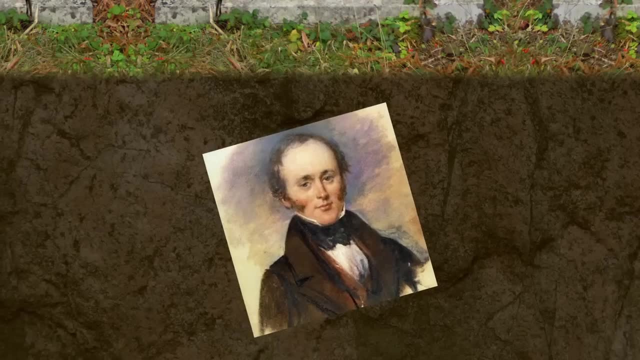 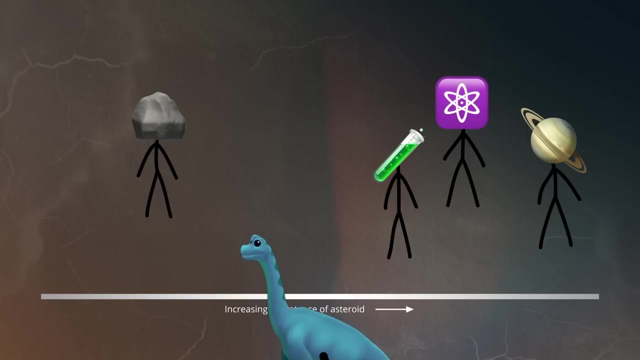 was at best misguided and at worst a traitor. How could someone immersed in 150 years of gradual processes suggest something so heretical? Lyle would be spinning in his grave At a slow, unwavering speed. Paleontologists are more difficult to place As a whole. 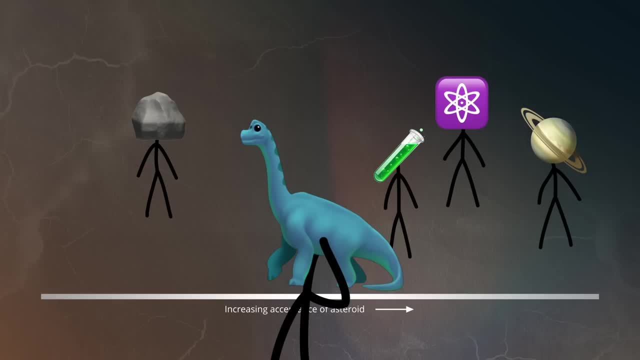 they felt kinship with geologists and abhorred the idea of mass extinction. But they were not the only ones who felt the same way about the idea of mass extinction. The differences emerged by subfield Paleontologists studying microfossils like forams were more 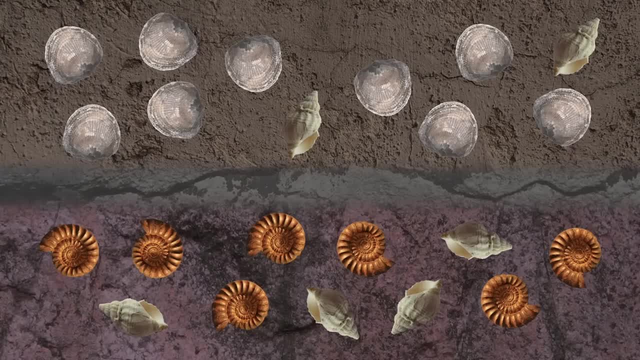 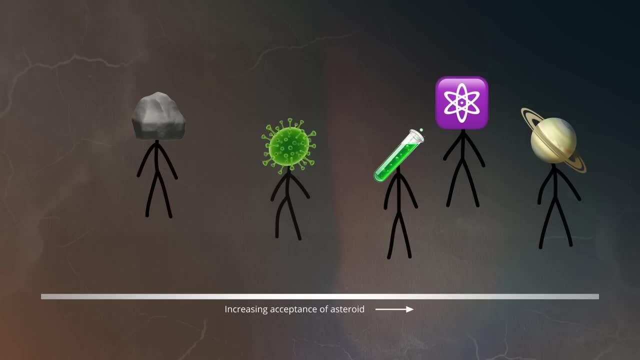 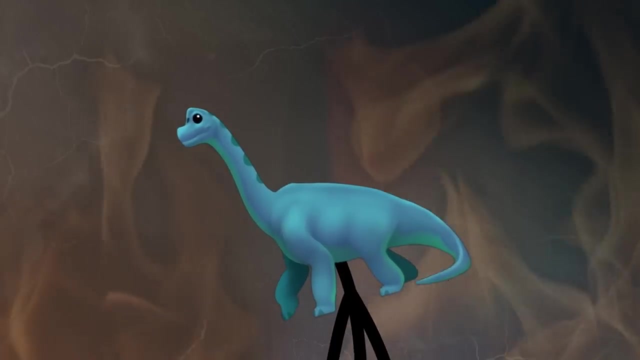 receptive. Remember, small marine animals give the highest resolution of the fossil record and so show the sharpest divisions. These scientists could see a mass extinction with their own eyes and even if asteroids were mysterious, the premise seemed plausible. Most anti-impact of all were the vertebrate paleontologists. 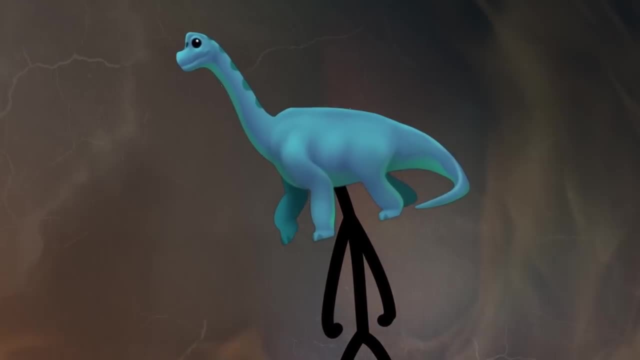 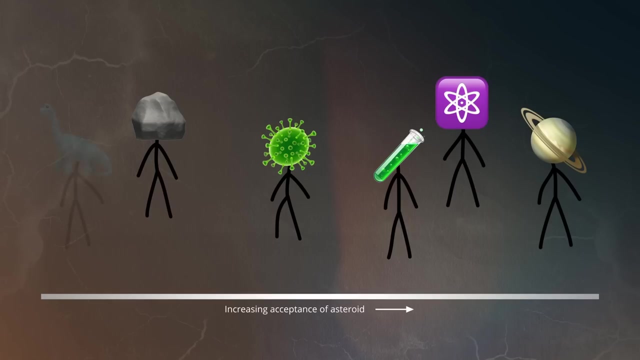 Vertebrates are animals with a backbone, and that includes the stars of the show, dinosaurs. Scarcity of vertebrate fossils hid any notion that they'd perished instantly. From the vertebrate paleontologist's perspective, everyone else was inventing reasons for something. 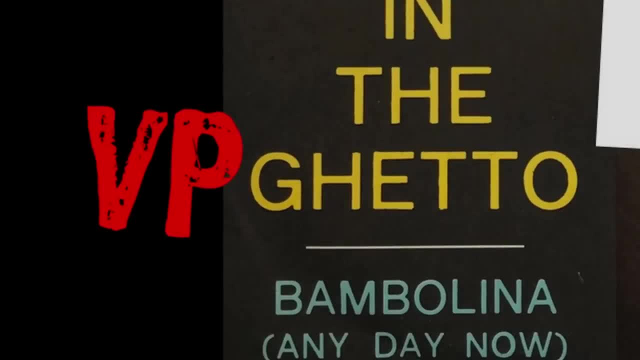 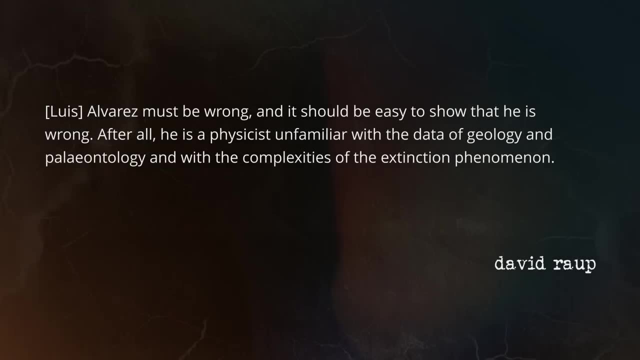 they could clearly see hadn't happened. Someone even coined the term VP-ghetto to refer to the stubborn group. Perhaps they had a point, though. Paleontologists had a reason to think they were the experts, and Alvarez knew nothing of their. 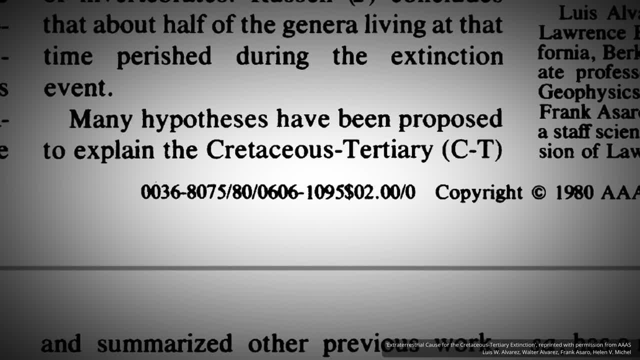 subject, because the Alvarez paper specified the extinction as the C-T boundary rather than K-T, as would have been correct in B. You see, I put that bit about the K in part 1 for a reason. I wasn't just being anal. 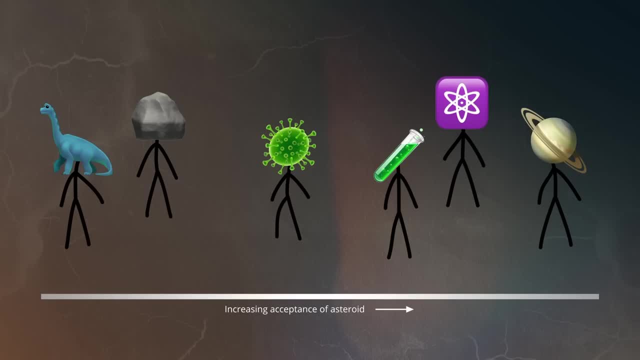 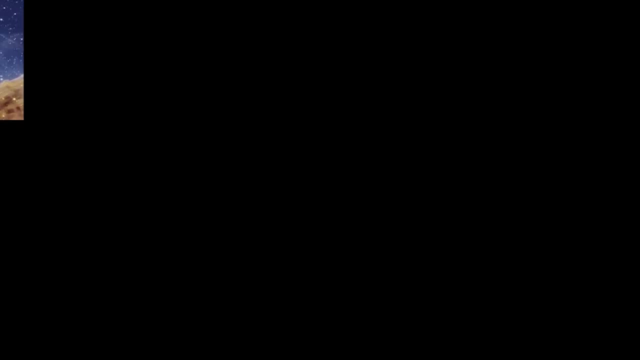 These positions are a simplification and aren't absolute. There were many dissenters within each field, But these were the rough centres of gravity as the debate began. It's important to emphasise the significance of the conflicting paradigms in each scientist's 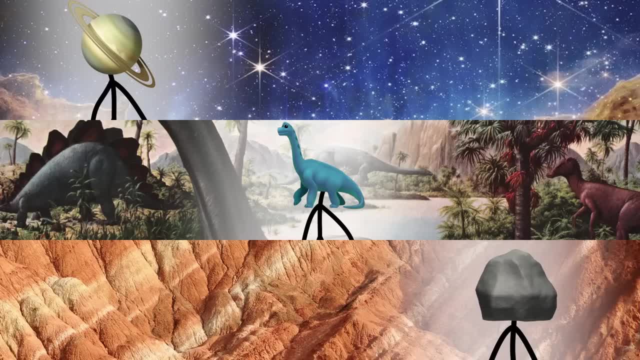 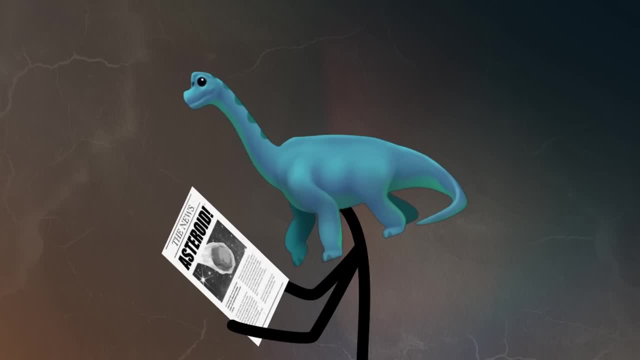 assessment. What looked obvious to some was insane to others, purely due to differences in information exposure and prevailing mindset. Most of all, few outside astronomy were privy to the new developments in the study of asteroids, so the idea still seemed mad and foreign to most. 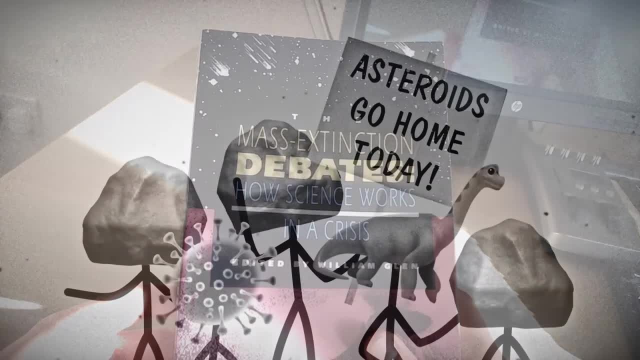 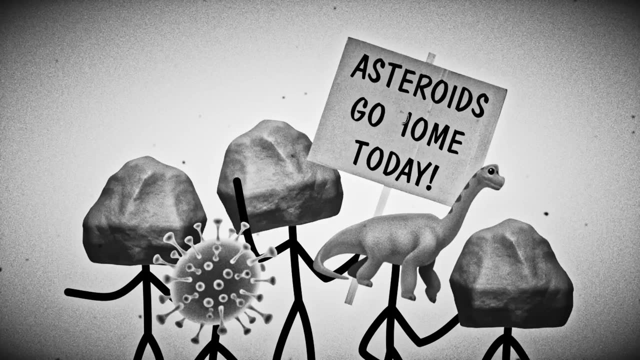 However, Glenn's interviewing of scientists at multiple points during the debates revealed that, after the fact they believed they'd known and accepted more than they had, They'd re-sculpted their memories after the paradigm had shifted, to insist they'd always been. 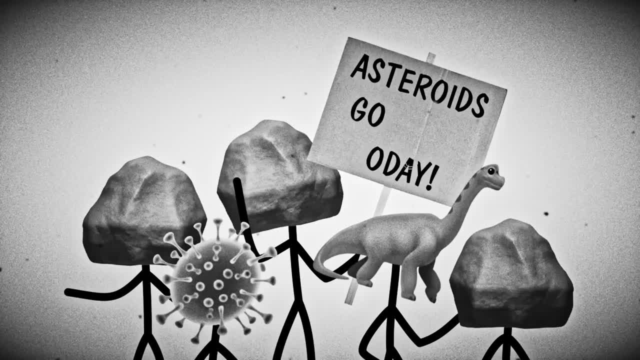 on the right side of history. They'd always been on the wrong side of history. This wasn't an wasn't lying. it was genuine belief on both occasions, An inability to consider themselves against the zeitgeist, since a challenge to the zeitgeist was a challenge to their own. 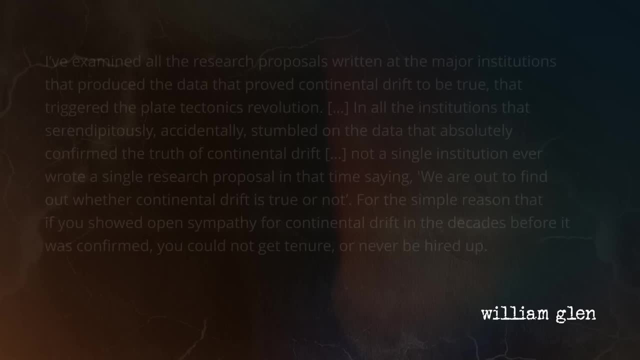 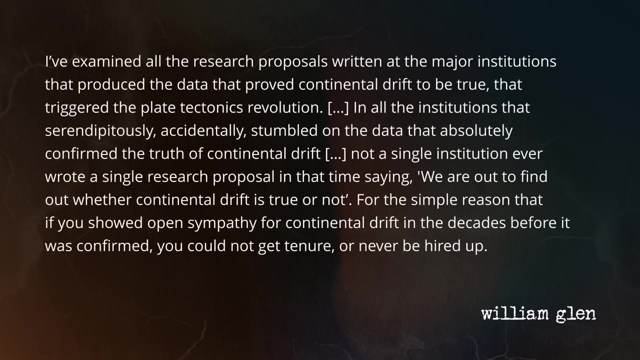 legitimacy. Many researchers' careers hinge on being able to convince others that their area of expertise deserves funding. If you back a horse that challenges an established theory, your job is at stake. You're incentivised to follow the trends, consciously or otherwise. 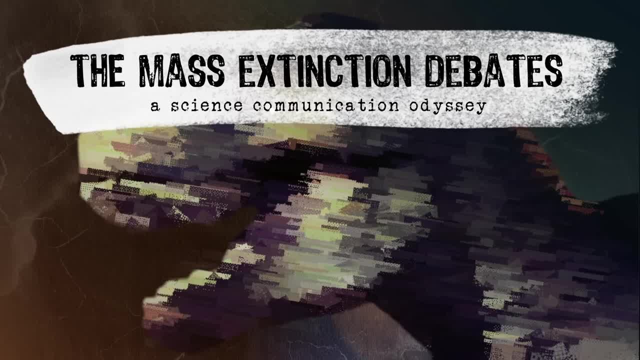 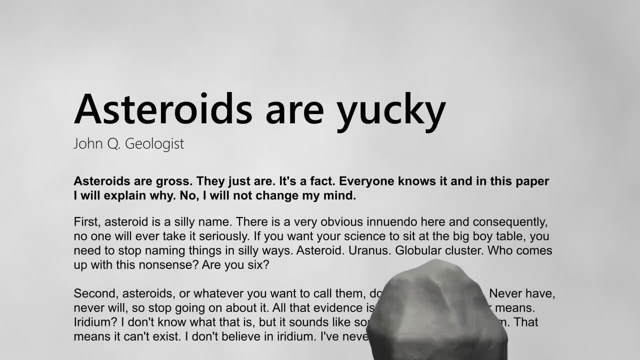 Remember that, as we go forward, real people's livelihoods were and still are tied to the debate's outcome. The exceptions to Glenn's mental re-sculpting were those who had published a paper in support of an alternative extinction mechanism prior to impact's arrival, Already having their 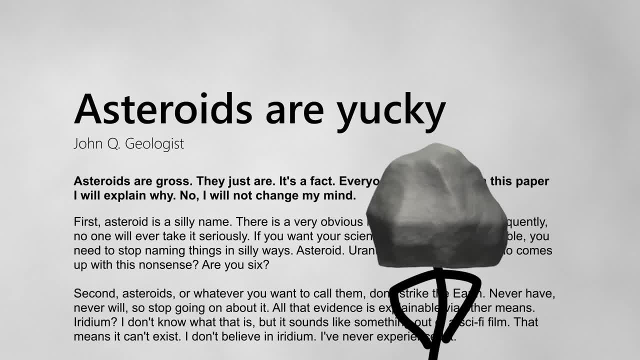 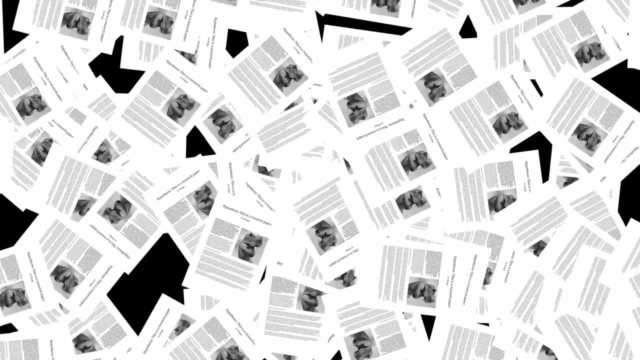 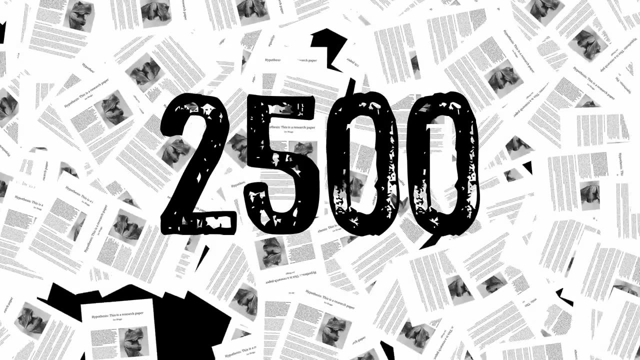 name in print alongside a pet theory, seemingly solidified their position for the rest of the debates. But many others soon put their name in print too. The Alvarez hypothesis had barely left the station when the tracks became clogged with a floating flurry of papers on the KPG extinction- Over two and a half thousand between 1980 and. 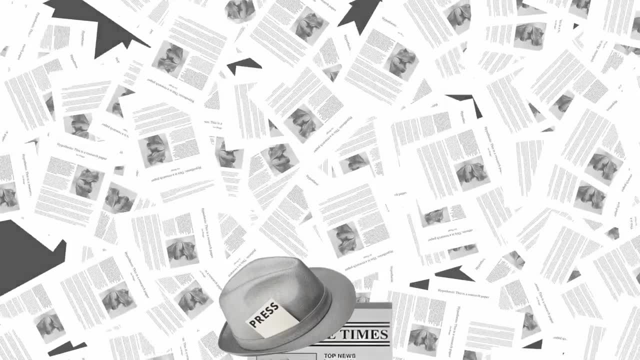 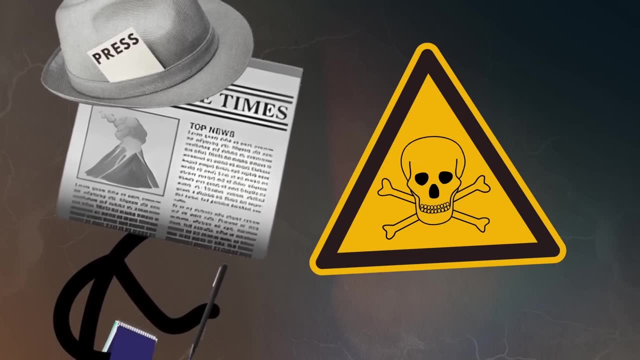 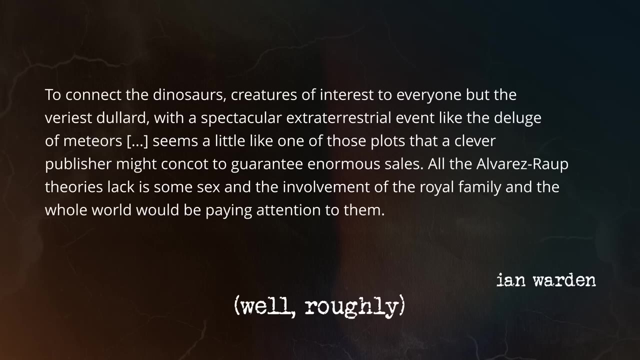 1994.. But as fast as the academic machine was running, it could never hope to match the pace of the press. Dinosaurs, Space Cataclysmic destruction: Just had some sex and a member of the royal family and the whole world would be paying attention. That's an actual quote by the 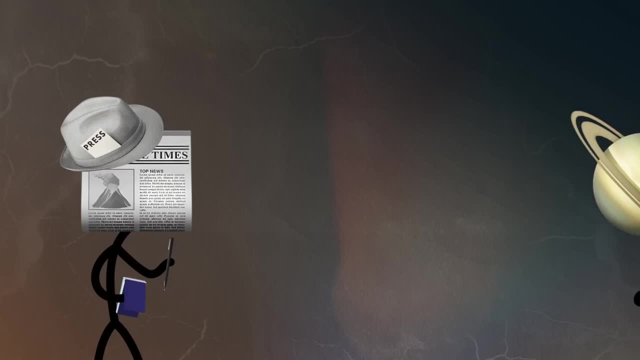 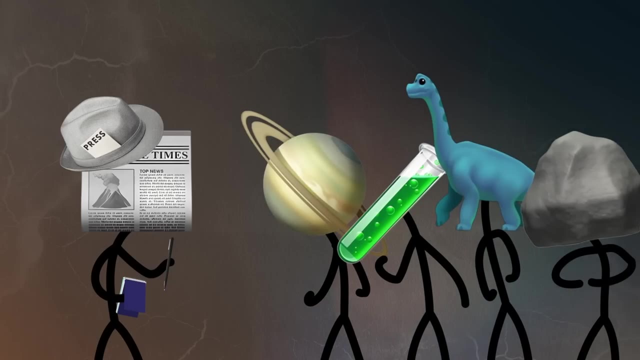 way. Many within academia saw media debate as contamination, A layer above that was all noise and seeped down to the detriment of the science. We'll delve into this much more in the next part, but that may not be how science works in modern society. 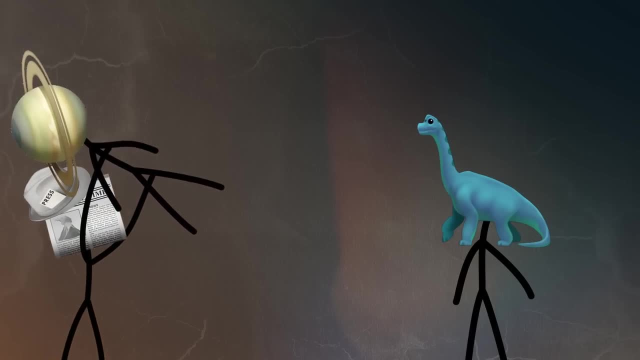 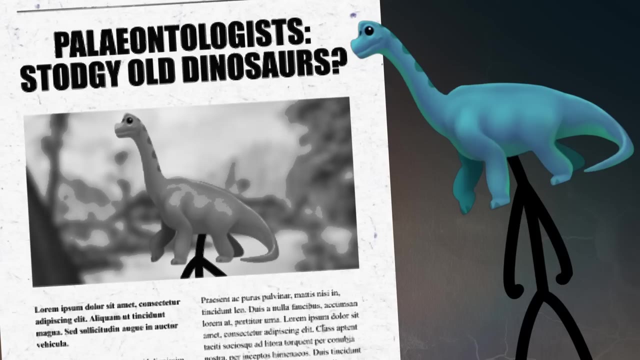 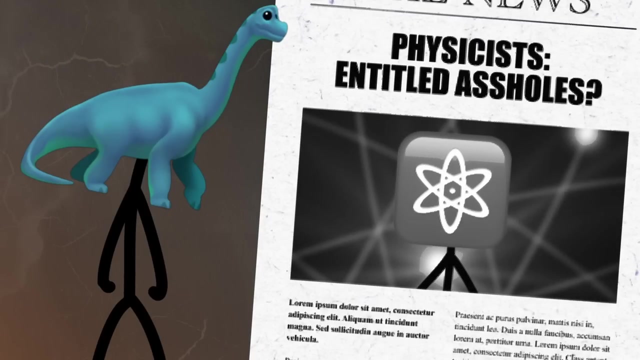 With so many disciplines involved that struggled to speak to each other of their own accord. mass media became the interface for communication, The real scientific battleground. Even as scientists suffered to get accurate representation for their own field, their perception of their opponents was uncritically shaped by the media's representation of them. 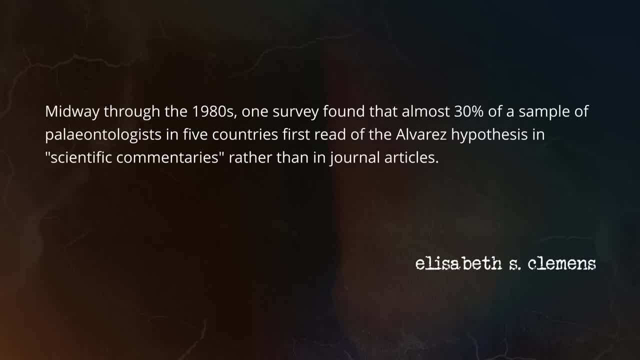 Further, a full 30% of scholars were asked about the scientific field, and that was the reason why the media was so important for them. The media was so important that science was involved in the debate, claim to have heard about it first in the popular press. 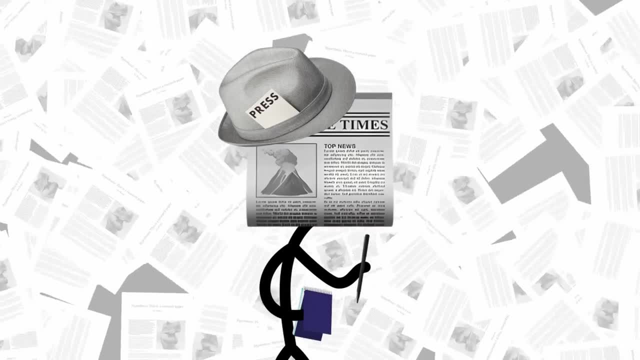 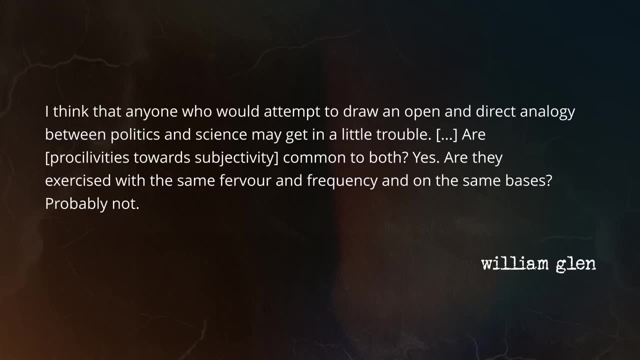 With such entrenched views at stake, and with the media's foot on the accelerator, a curious thing happened to the debate landscape. You might call it political polarisation, although Glenn is quick to warn of the dangers of drawing parallels between science and politics. 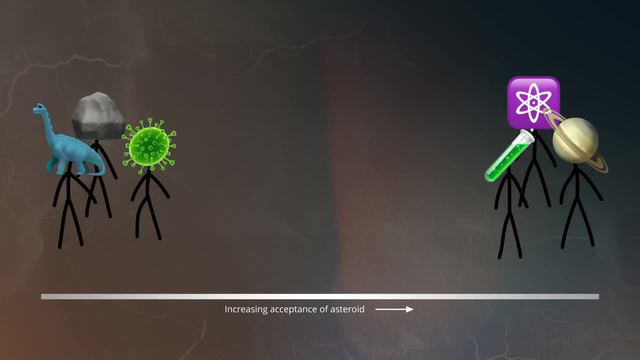 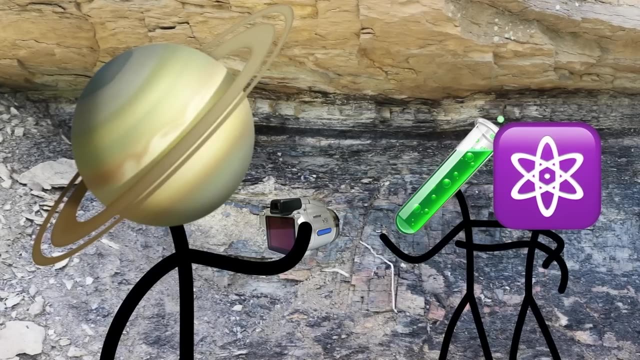 Partisanship became the driving force. Pro-impact groups teamed up with each other to find evidence for impact extinction. Anti-impact groups teamed up to find evidence against it. It was a time of vibrant collaboration that broke down scientific barriers, everyone collaborating. 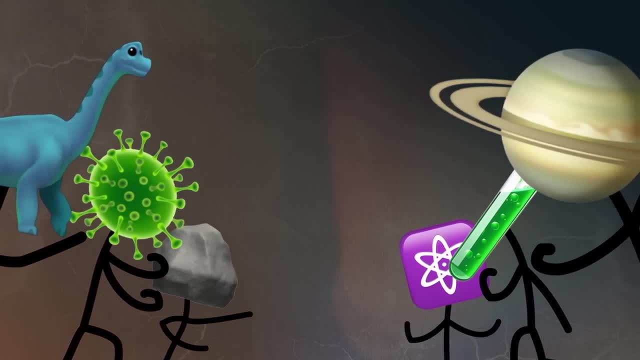 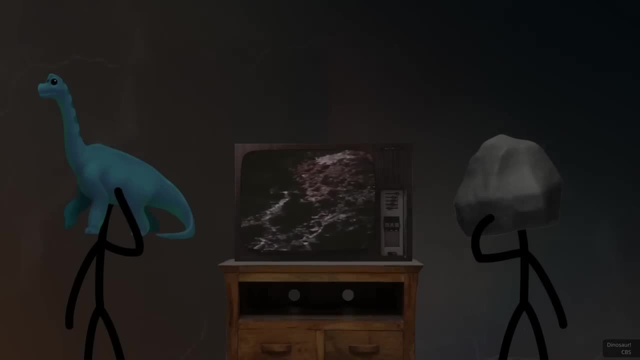 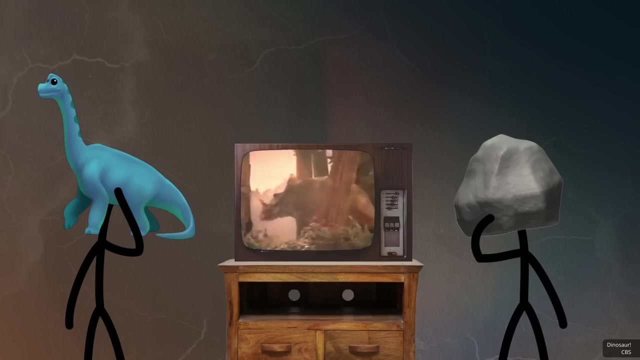 by party line to reinforce the one barrier that motivated them. An arms race had begun. Those who doubted impact faced an immediate problem. Asteroids were media wildfire, the deus ex machina, elegance of the theory dominating public opinion. Opponents needed to be seen for themselves. Those who doubted impact faced an immediate problem. Asteroids were media wildfire, the deus ex machina, elegance of the theory dominating public opinion. Opponents needed to be seen for themselves. Opponents needed 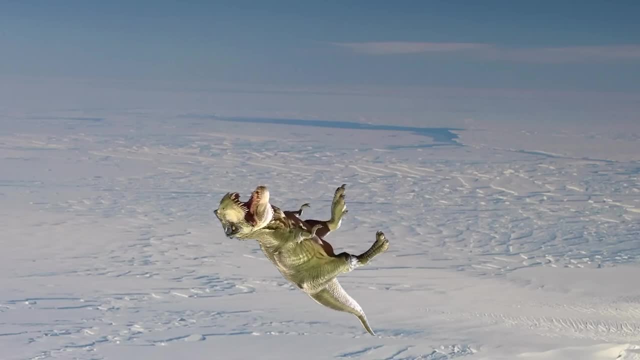 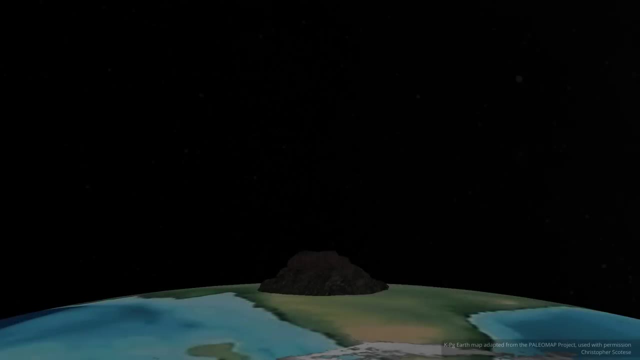 to be seen for themselves. Those who doubted impact faced an immediate problem. Asteroids were media wildfire, the deus ex machina, elegance of the theory dominating public opinion. Opponents needed a weapon more salient than gradual environmental changes. But what could be so potent yet still be shoehorned into uniformitarianism? 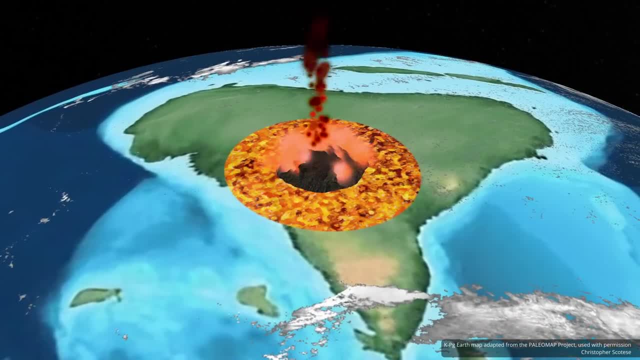 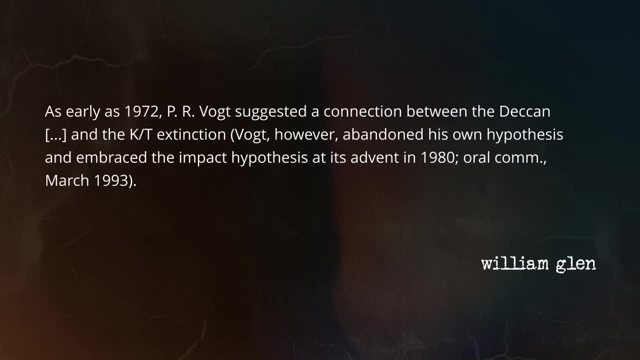 Their answer was a paper dragged out of the archives from 1972, in which Peter Vogt proposed the mantle plube theory. we met in part 1.. Fun fact, Vogt was the only example Glenn found of someone fully endorsing one theory in print. before 1980.. Volcanism's creator switched sides to team impact. Many latched onto evidence for decantraps volcanism and shifted gears to search for more. Was there evidence that it had been rapid and intense enough to cause a mass extinction? 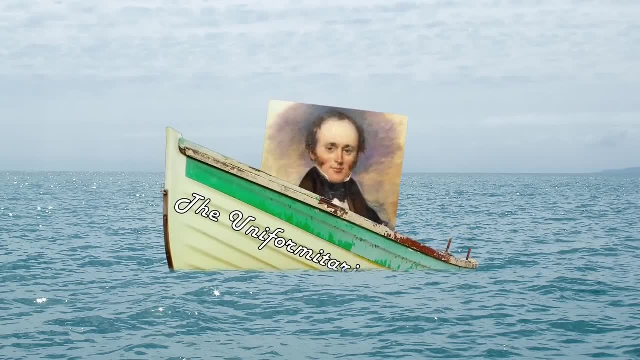 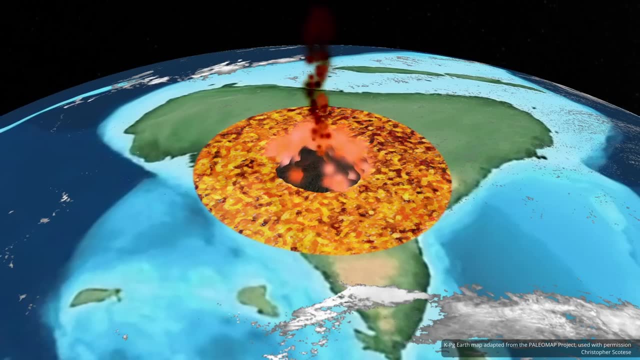 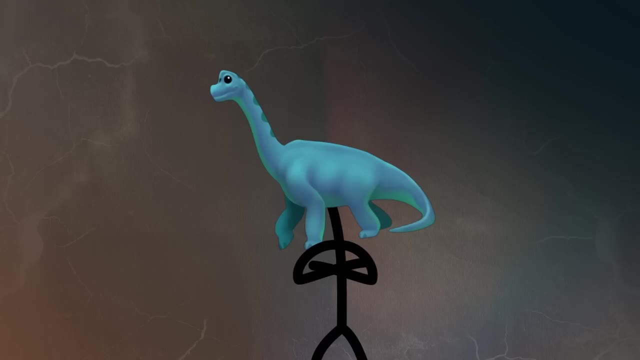 In doing so, these researchers had also jumped ship from uniformitarianism. Even if they believed volcanoes were in keeping with present processes, the scale and power they had to invoke for the decantraps was nothing like humans have ever imagined. Some cringed at the development and maintained mass extinctions were still nonsense, But their 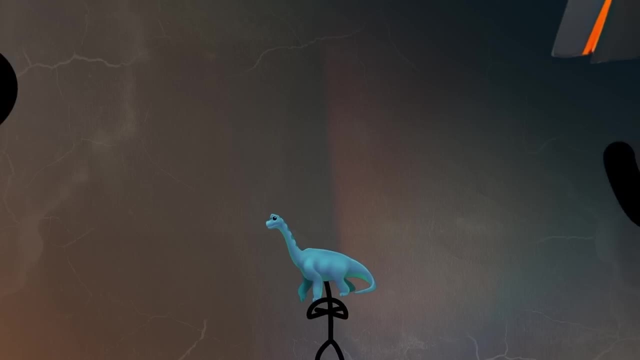 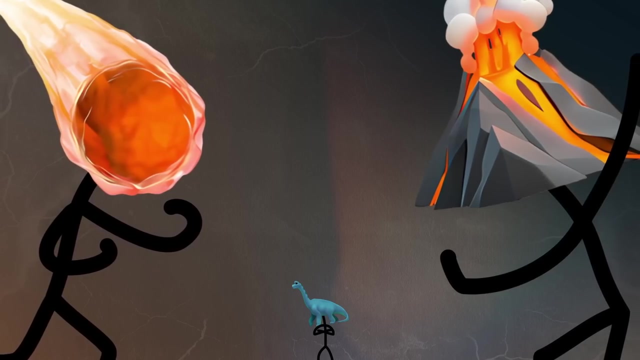 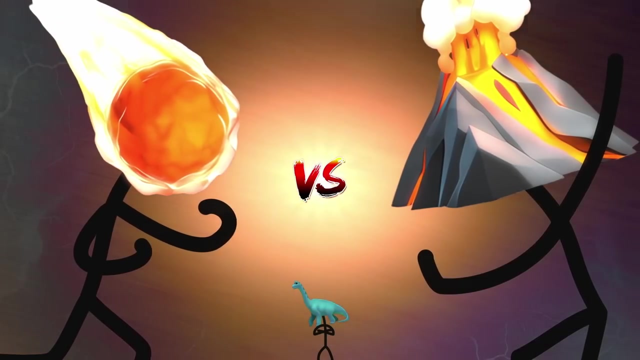 objections were soon drowned out by the louder voices of the two apocalypses. Polarisation had coalesced each camp into advocates for a single theory known as impactors and volcanists. Uniformitarianism was dead, and it was now catastrophism versus catastrophism for the 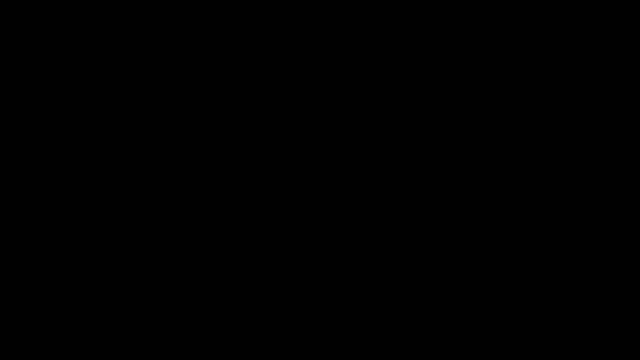 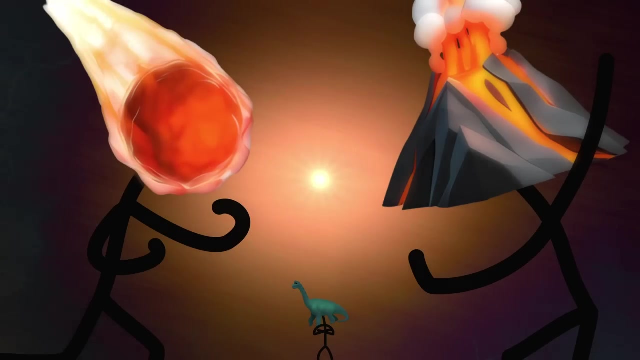 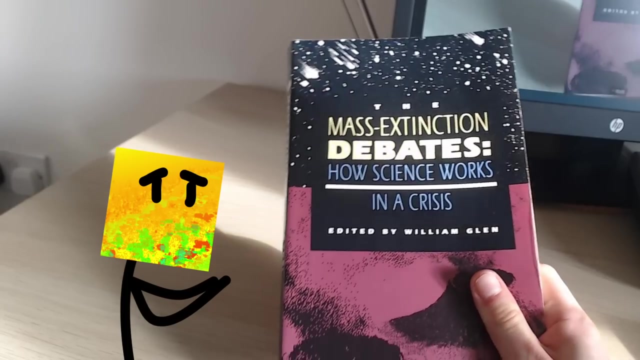 spoils. Everything only gets messier from here. There's no way I can form a neat and comprehensive chronology in a YouTube video, so, for lack of a more efficient approach, please forgive me. Top 10 Most Explosive Moments From The Impactor vs Volcanist Debates. 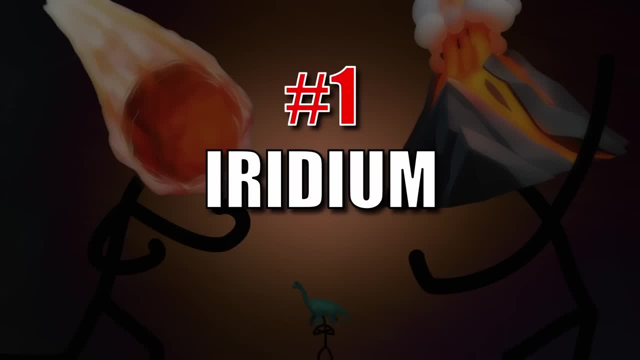 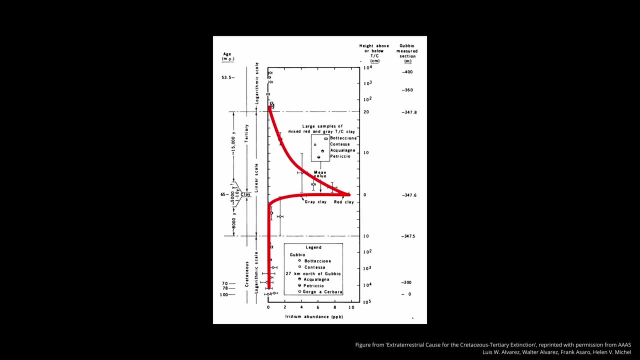 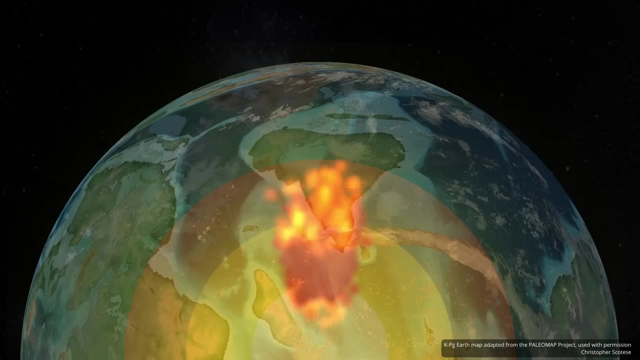 1. Iridium. The volcanists' first challenge was to explain the global iridium anomaly without an asteroid. Iridium may be rare in the crust, but, as we saw, it's plentiful in the Earth's core. Could a mantle plume have carried it up to the surface? 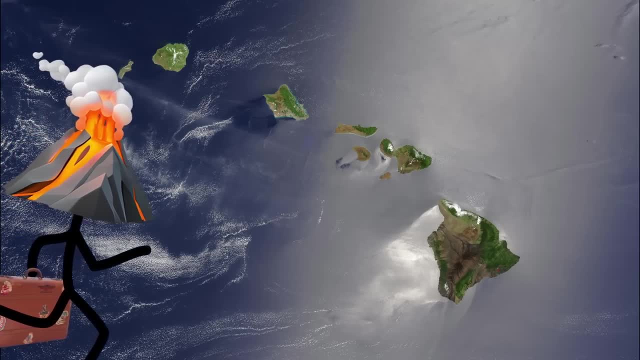 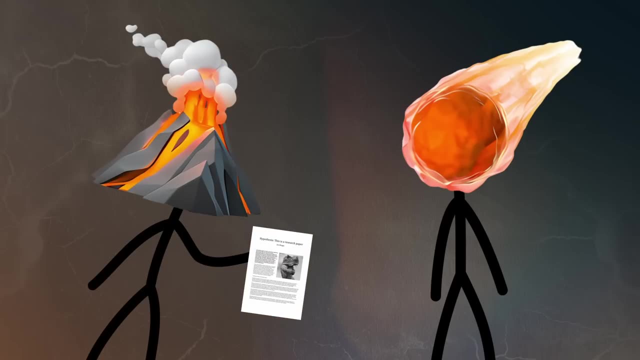 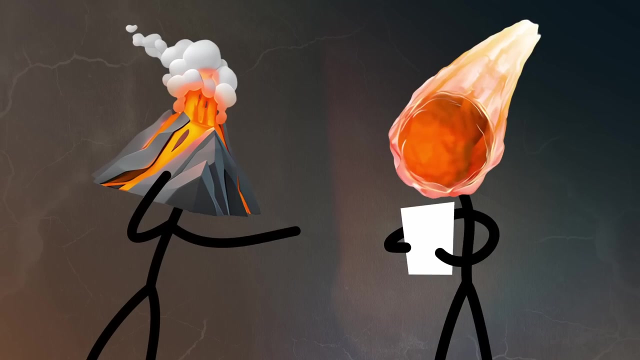 A team was dispatched to Hawaii post-haste to study a modern mantle plume and find out. They returned with promising evidence. Oh, what's this? We found iridium in volcanic rock. How strange, It says here. the density is a hundred times too little to account for the case, But it's. 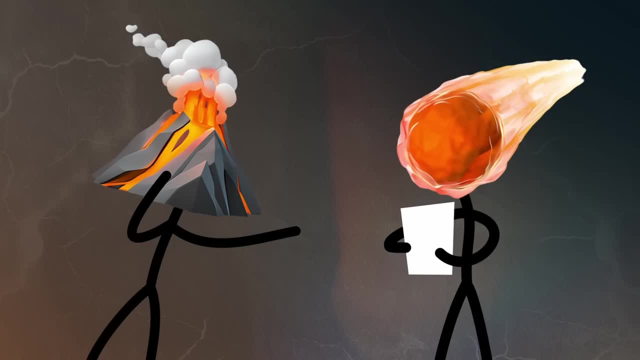 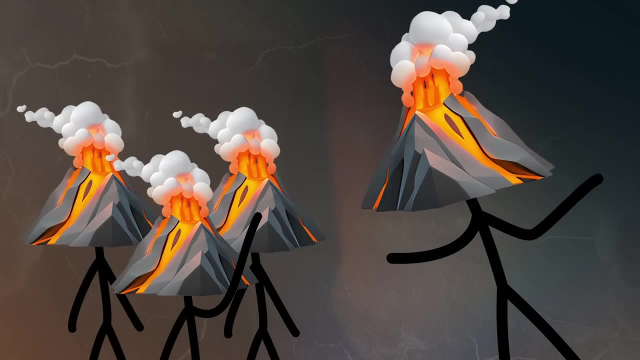 not all that strange. It's not all that strange. It says here: the density is 100 times too little to account for the K-P-G layer. Uhhhh, Quick, somebody come up with a good response. Well, we also found particles in the air around the volcano with much higher iridium concentration. 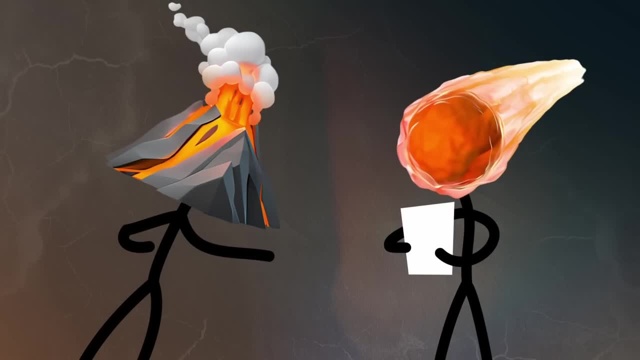 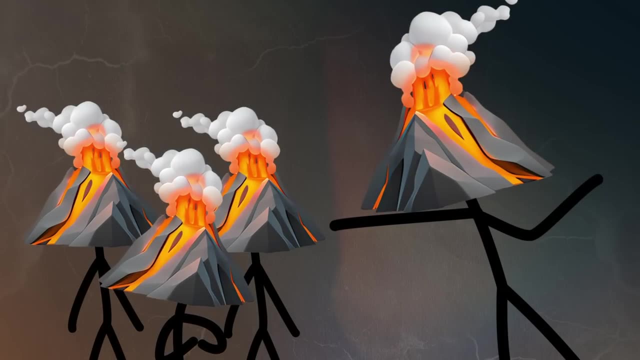 but… Great, we'll use that. We also found particles in the air around the volcano with much higher iridium concentration, But every other study has found no iridium at all in volcanic gases, so that was probably some kind of outlier. 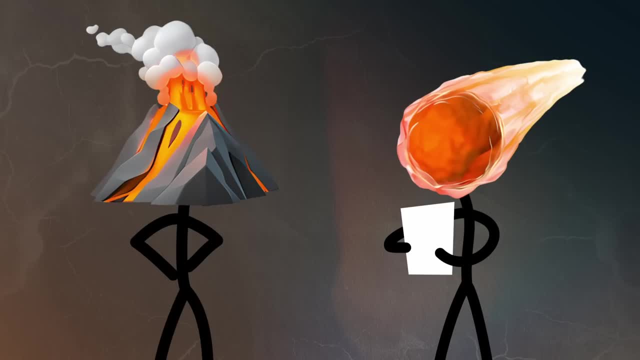 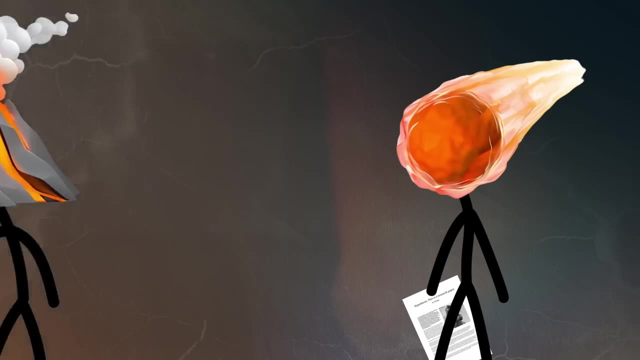 But every other study has found no iridium at all in volcanic gases, so that was probably some kind of outlier. Oh Well, you tried. No, no wait, I can fix this. Hey, media, we found iridium in volcanoes, And it's all a bit wishy-washy, so we can. 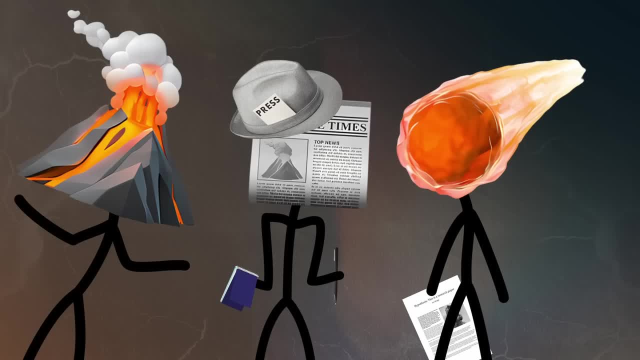 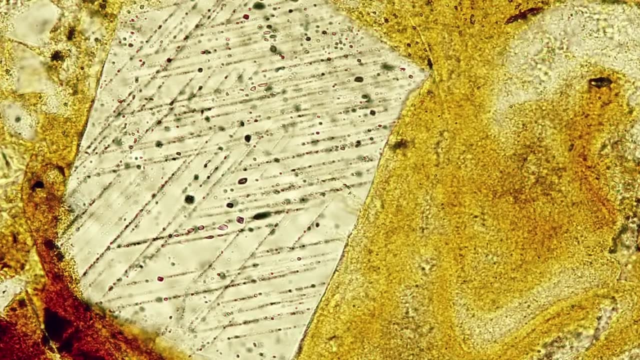 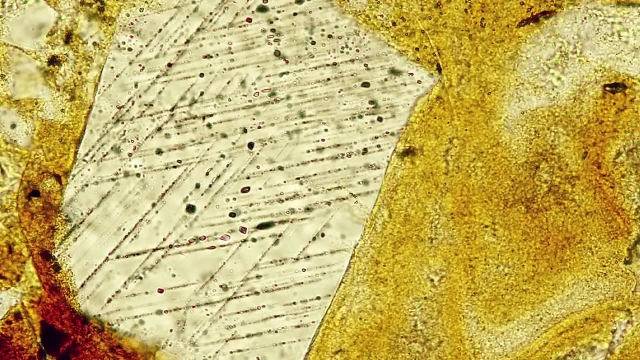 hide in the uncertainty? Meh, the science checks out. Number 2. Explosive Volcanoes. Another piece of evidence fell the impactors way with the discovery of shocked quartz in the iridium layer. Quartz is a common mineral and shocked quartz a version with distinct. 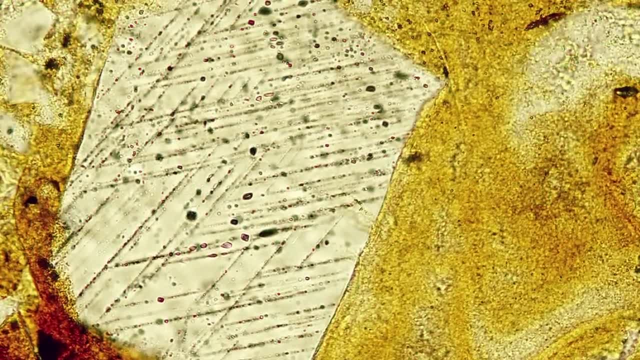 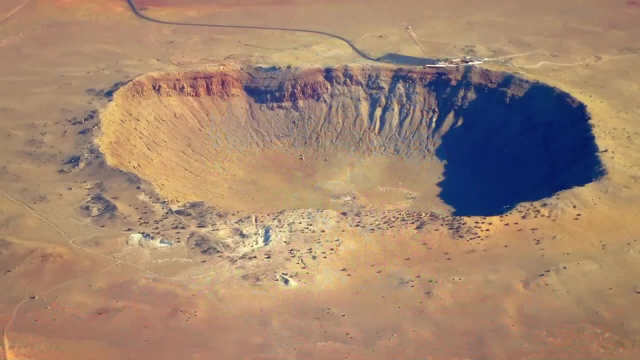 linear patterns is evidence of incredible strain in rock. Up to this point it had only been discovered at nuclear test sites and impact craters. Clearly it was a marker for explosions without measure, beyond even volcanic power. How would the volcanists explain this one? 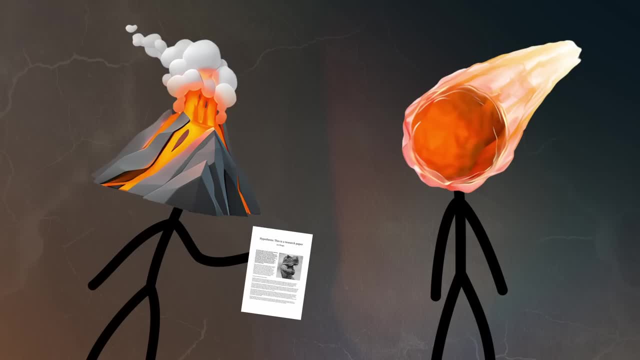 OK, I have this new theory called explosive volcanoes. I thought mantle plume volcanism was more pshkvvvv than pshh. Ah yes, but there were pshh ones too, on a scale larger than any ever imagined. 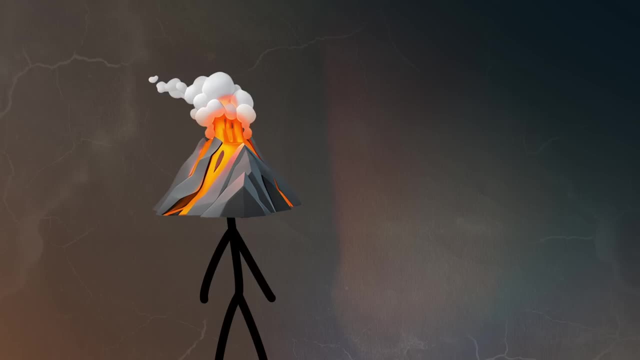 Now you're just making stuff up. They were making stuff up. Volcanologists, experts on volcanoes- and, confusingly, not the same group as volcanists- unanimously rejected the explosive volcanoes hypothesis. The volcanists didn't know what they were talking about. 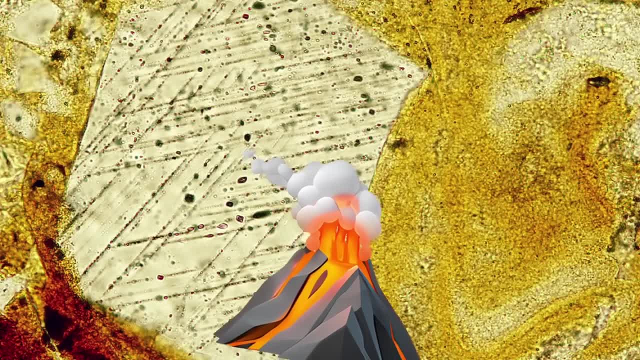 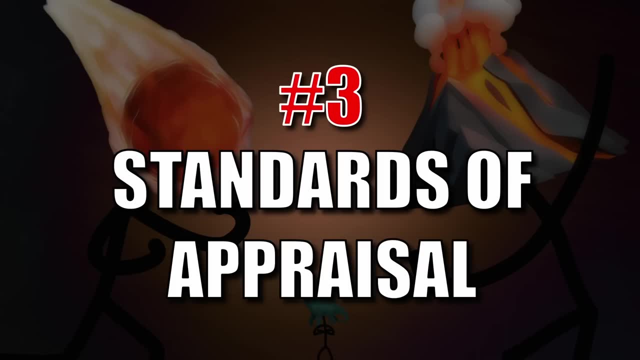 And yet, reactively inventing a volcanic cause for shocked quartz, maintained the illusion that it was still an open question. Number 3. Stainless Steel. Number 3. Standards of Appraisal. Both these examples highlight how assessment of evidence depended more on the side one. 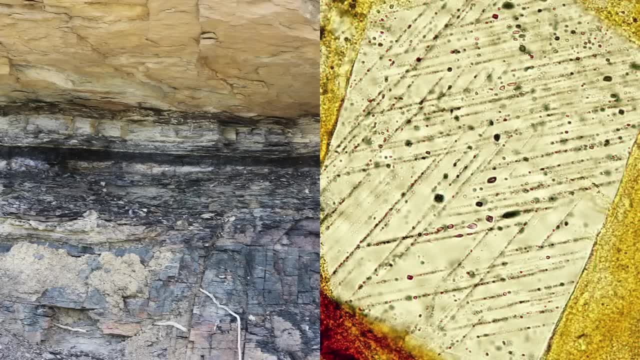 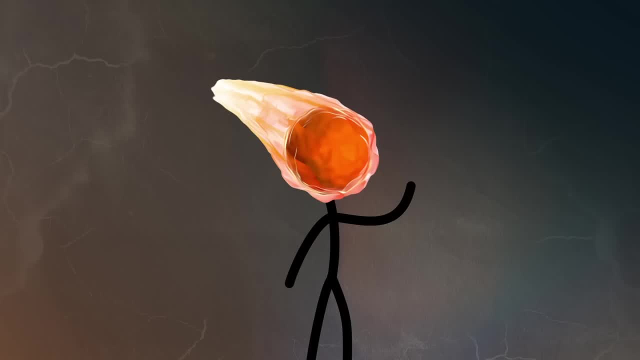 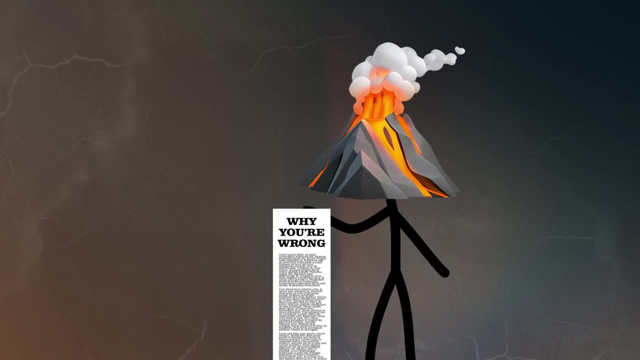 was arguing from than the objective value of the evidence. It's scary to think that two equally decorated experts looking at the same data could come away with opposing conclusions. Glenn and others believe the impactors were, on the whole, using conventional standards of appraisal, while the volcanists tended to nitpick the minor unknowns for far longer. 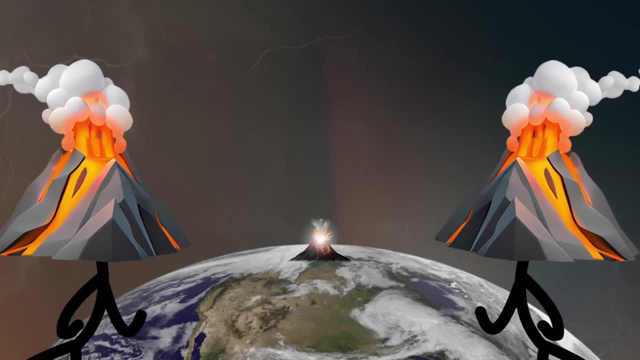 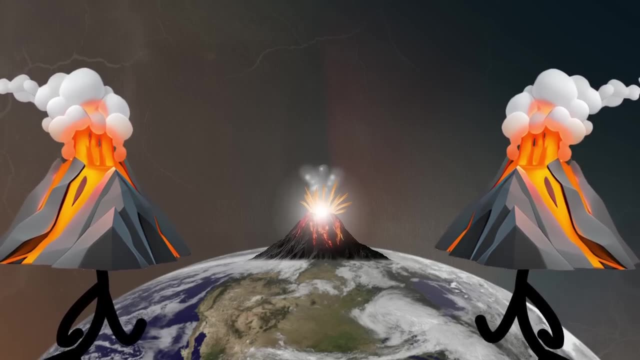 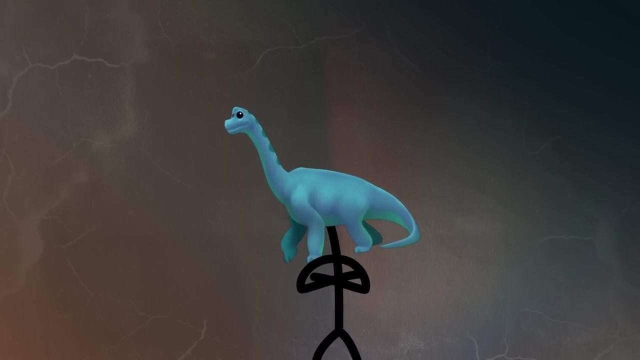 than scientists normally would. Plus, they explained their own gaps with weird and unknown processes flying in the face not only of scientific ideals but also of uniformitarianism. now they've dug in their heels so deeply against the impact theory. On that note, old guard uniformitarians also ran into issues assessing evidence. 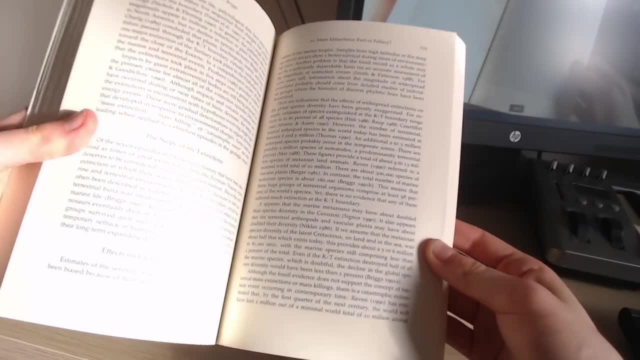 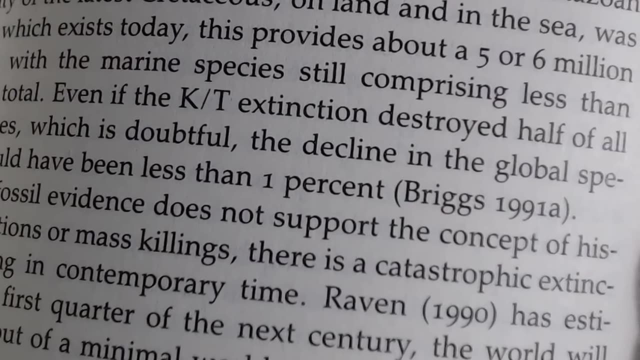 One of the chapters in mass extinction debates comes from John Briggs, a marine zoologist, who argues confidently, based on paleontological techniques, that the KBG boundary represents not 50-80% extinction rate but 50-80% extinction rate. 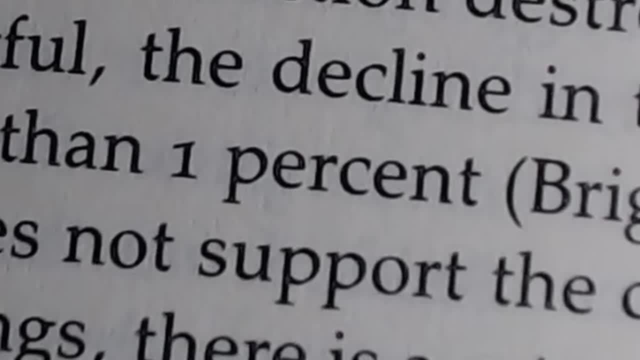 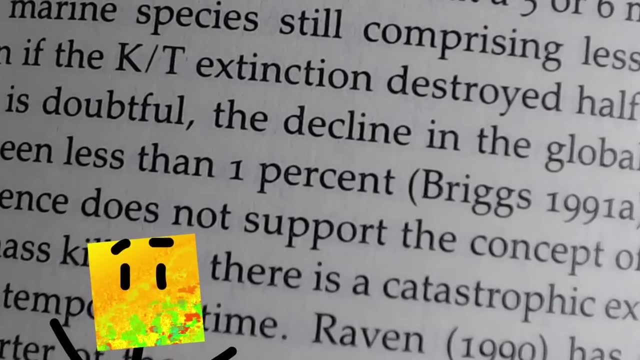 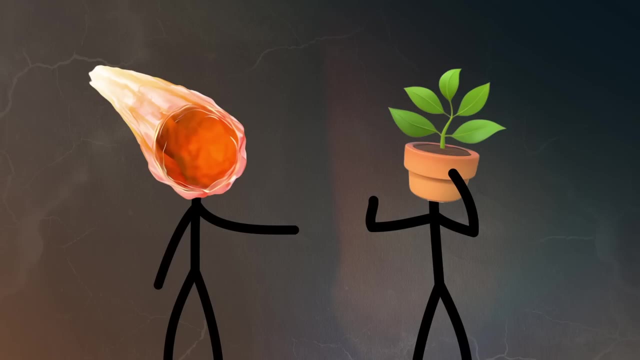 The terrifying thing is that I as a layperson can't find fault with the explanation he gives to back it up. I must rely on others' appraisal of his evidence. Glenn also recalls a paleobotanist who violently refuted mass extinction until they were dragged. 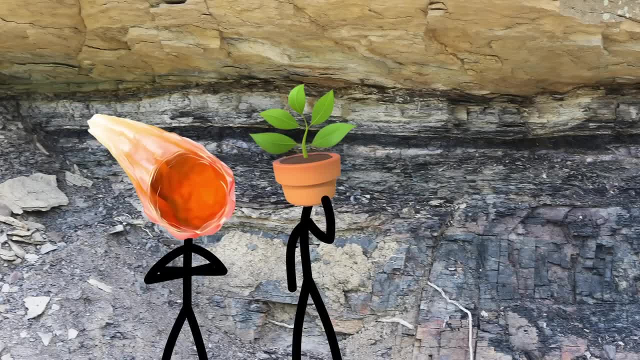 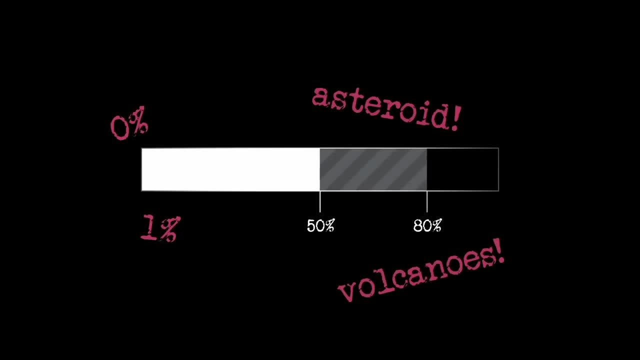 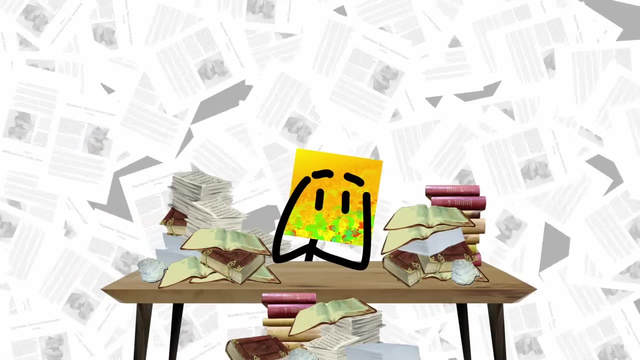 to the field to see the fossils. Looking at evidence for its own sake, outside of others' judgements immediately changed their mind. Everyone's looking at the same data, But nobody can agree what it means- Number 4.. Adding insult to injury, There's a quote every source on the debate seems to reference, so I guess I'm obligated. 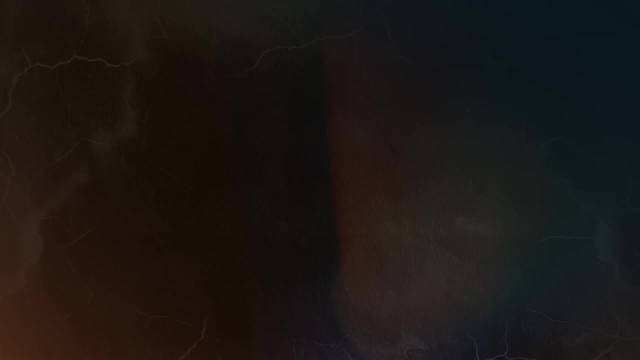 to put it here too. One paleontologist said of the impactors in a 1985 New York Times article: "the arrogance of these people is simply unbelievable. They know next to nothing about how real animals evolve, live and become extinct. 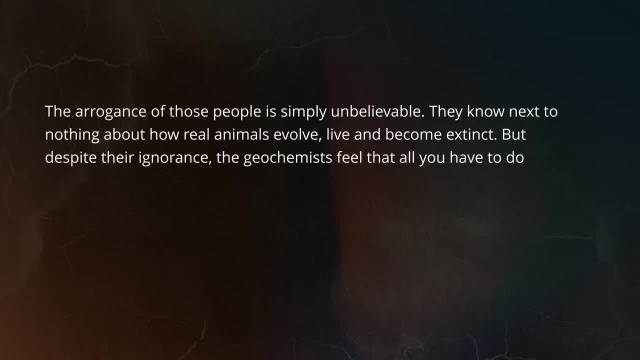 But despite their ignorance, the geochemists feel that all you have to do is crank up the gaps and fancy machine and you've revolutionized science". That paleontologist, Bob Bakker, who you may remember as one half of a science revolution of his own two decades. 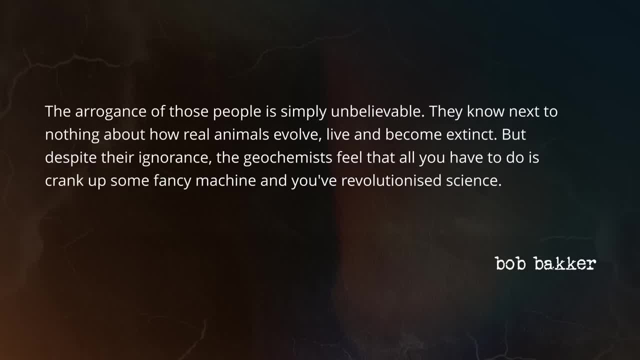 earlier Physicists and geochemists. trespassing on paleontological ground was not taken well, as this attack shows. In fairness, the impactors did little to help their cause. Luis Alvarez had some particularly scathing words about his opponents. 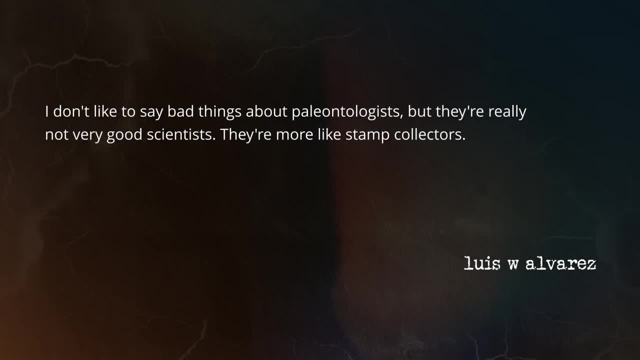 He wheeled out the old Ernest Rutherford line about the impactors, All science being either physics or stamp collecting. He claimed as early as 1983 that the debate was over and everyone agreed an asteroid did it. As paraphrased by the media, he believed objections could be dismissed on grounds of general incompetence. 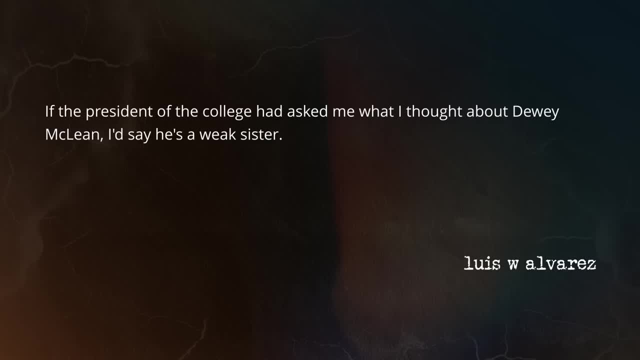 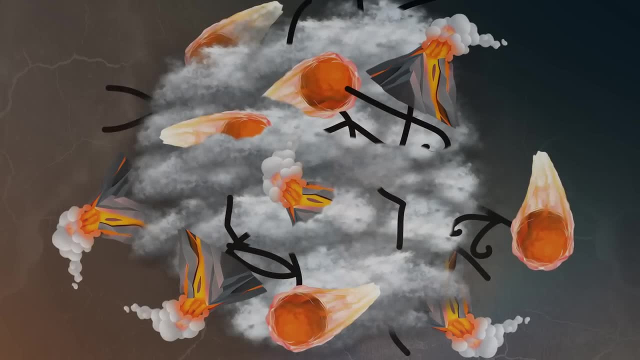 And he described one paleontologist who suffered through a markedly vicious feud with him as a weak sister. Volcanists claim impactors in general, hurled further insults at them for years, even during lectures, In fact, Ad Hominem attacks, repeated in the media, became the norm. 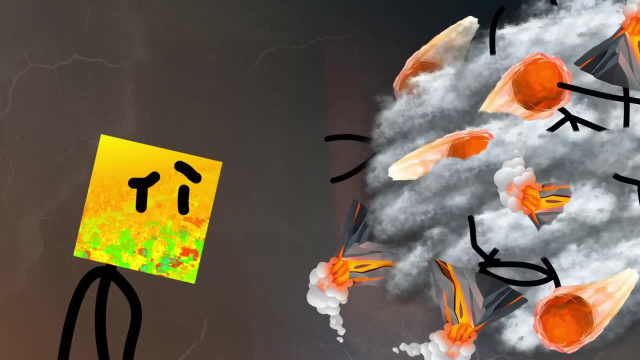 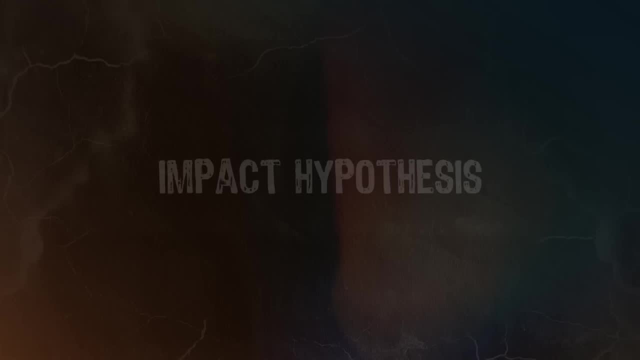 Exactly how true these claims are, I found difficult to verify. I'll stay out of this one. Number 5, Impact theory conflation. A subtle point in all this is that the impact hypothesis is not a single theory. There are two parts to it. 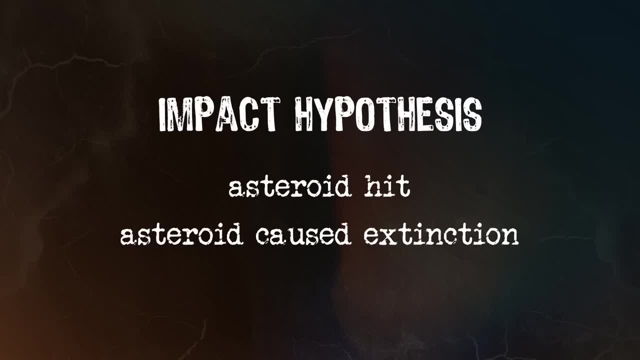 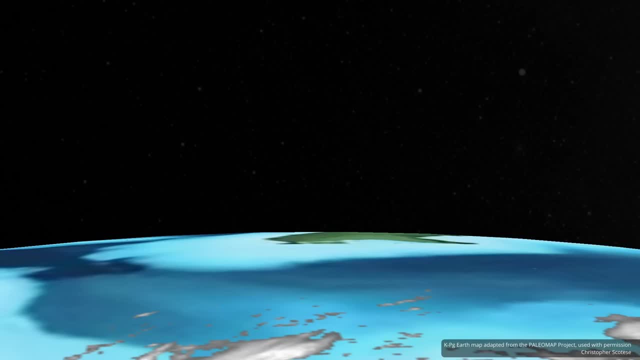 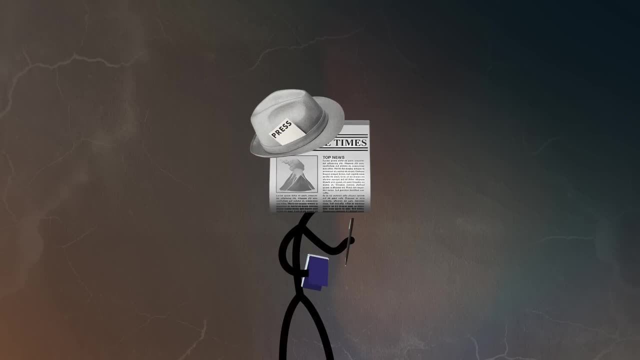 First, that an asteroid hit. Second, that it caused an extinction. The two are not equivalent. It's possible the asteroid hit hit, but the resulting killing mechanisms have been overstated. Was it but a blip in the true extinction timeline? As you might expect, the media often conflated two theories. but as you, 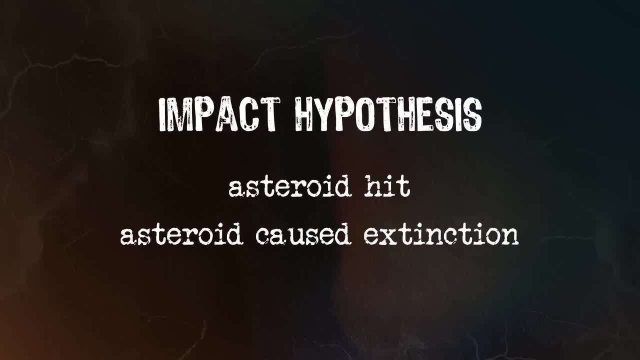 might not expect. so did the experts. Given the wealth of disciplines required to even tease out this difference, that's not surprising. Assumptions over which impact theory everyone was talking about may well have led to much of the animosity. 6. Smearing 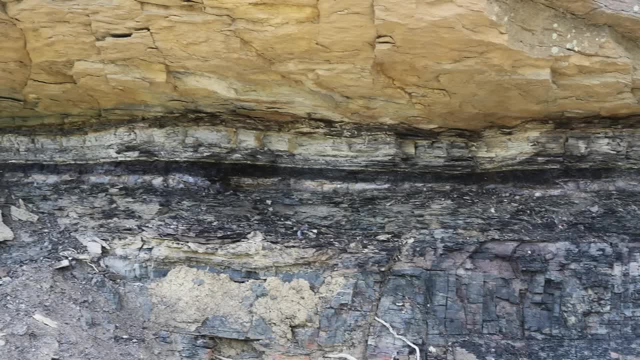 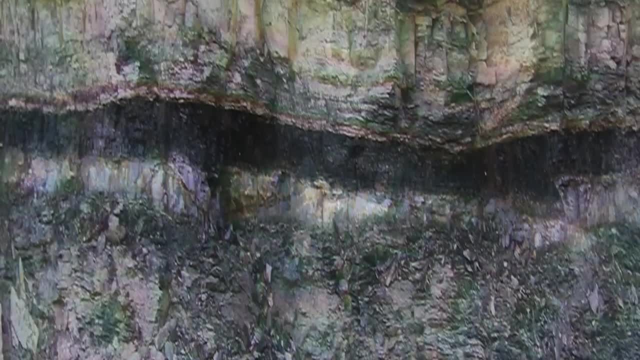 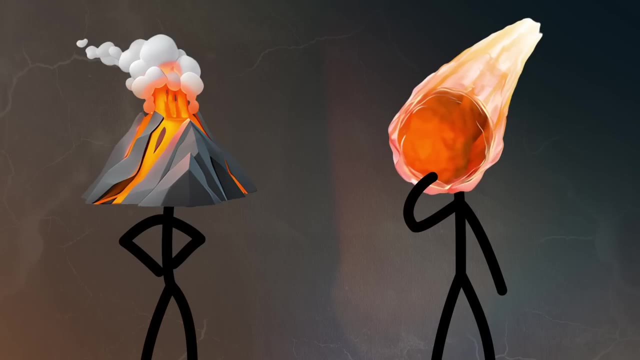 Volcanists rejoiced when, at some locations, the Iridium anomaly appeared to be smeared, spread out over a longer period and even suggesting multiple pulses. Haha, how can your sudden blip of an asteroid explain that? Uh, two asteroids. 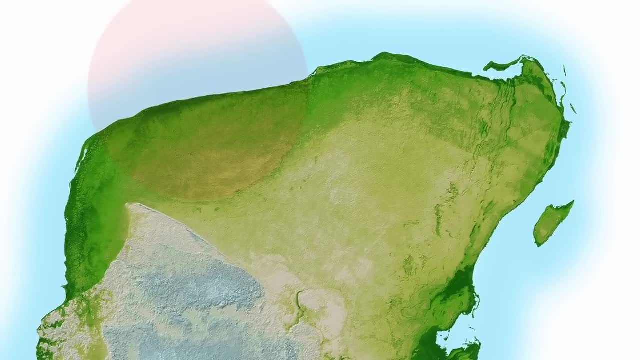 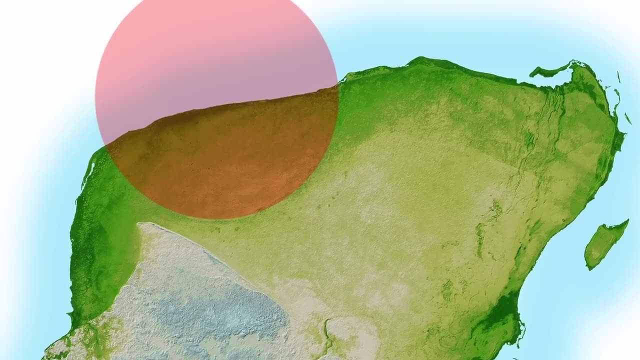 Now it was the impactor's turn to make things up to keep pace with new objections, Spoilers. but there's definitely one big crater dated 66,000, million years ago and any others seem to be a maybe at best. Stories about new candidates turn. 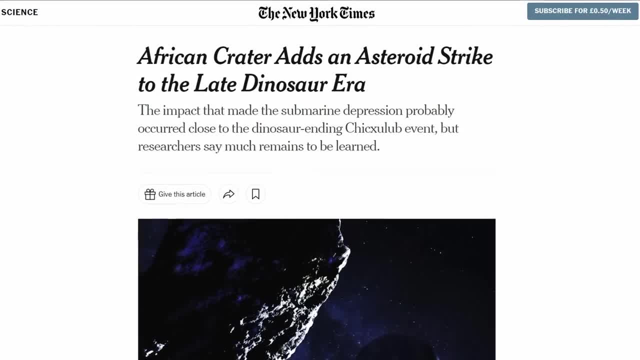 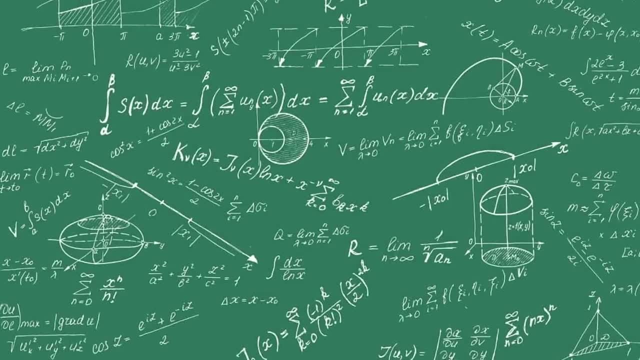 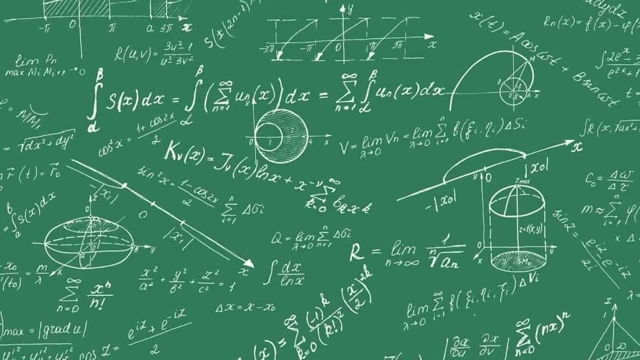 up all the time, but it seems evidence is too hazy for even impactors to put their full weight behind it yet. 7. Modelling: Both sides turned to mathematical models, hoping to prove their theories using cold, hard numbers. Things went badly: The models' complexity and, again, enormous disparity in skillsets. 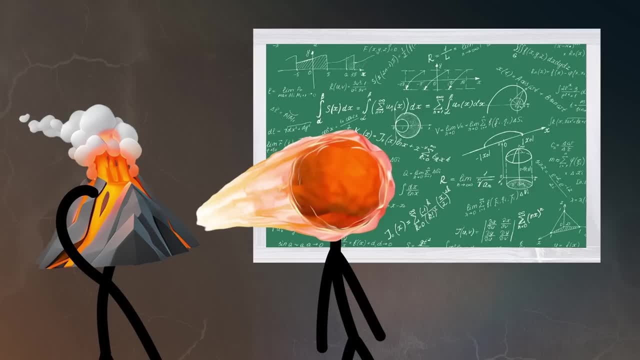 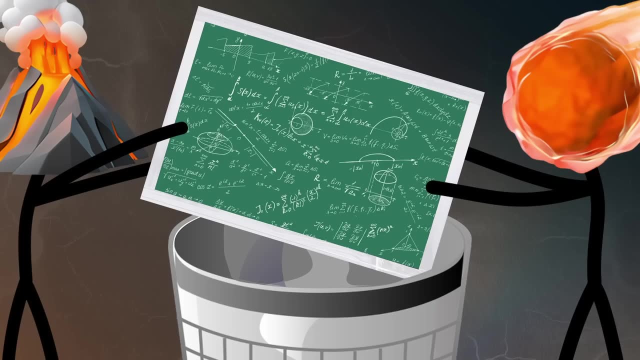 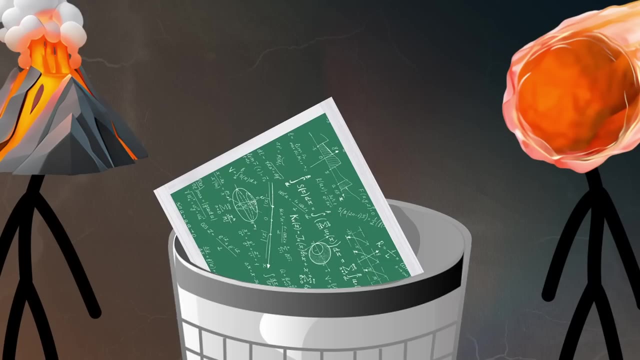 meant very few actually understood. The choice boiled down to blind faith or blind dismissal. And if the model disagrees with you, which are you going for? Everyone decided maths wasn't the answer and that maybe something more concrete was needed. Impactors busied themselves throwing rocks at bowls of flour. 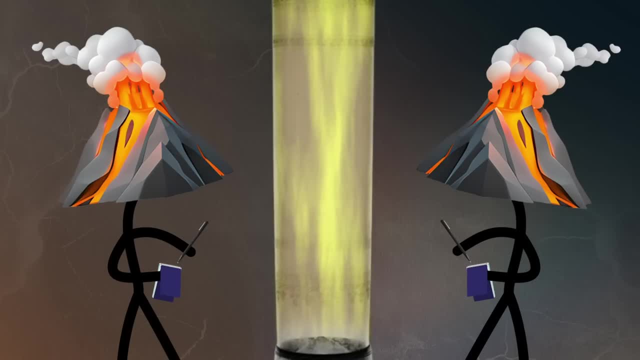 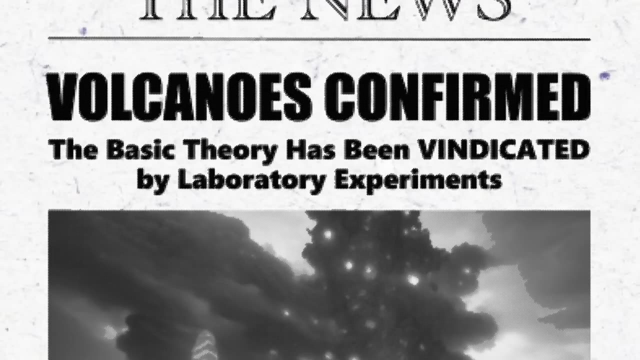 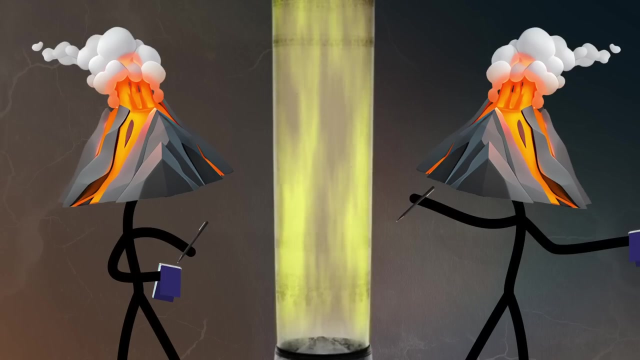 while volcanists simulated a mantle plume using corn syrup in a glass tube. One reporter heard of this glorified lava lamp and ran a story with the caption: The basic theory has been vindicated by laboratory experiments. Even the people who performed the experiment were like dude. it's just corn syrup. 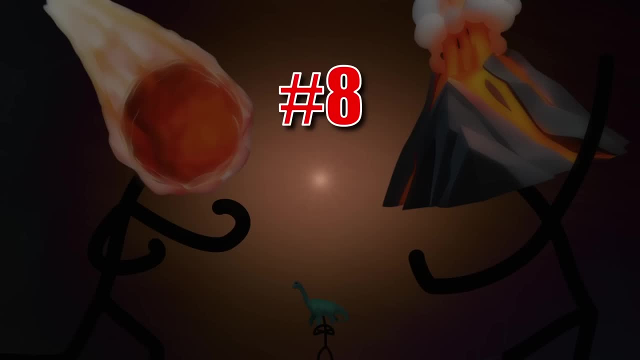 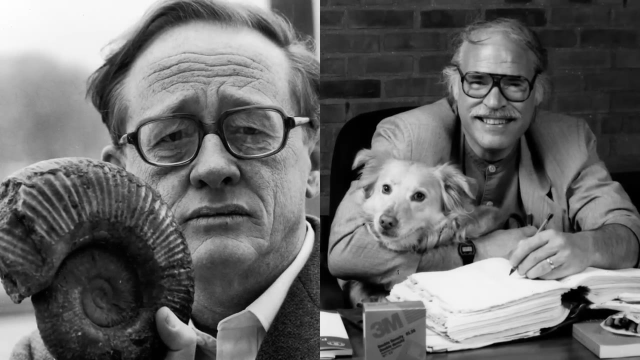 VOLCANOES. 8. Periodicity: In 1984, paleontologists David Raup and Jack Sapkowski had an idea: What if you gathered all available data on extinction rate across the Earth's entire history and plotted it on a graph? 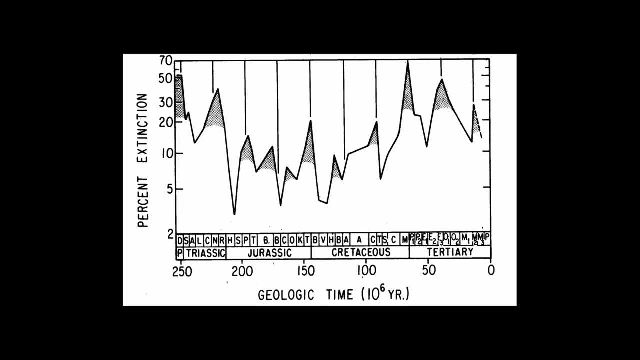 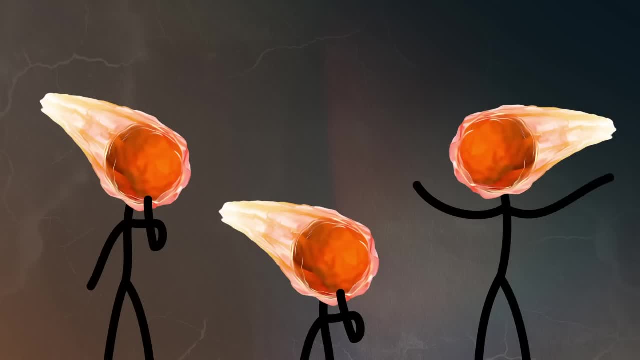 They ended up with this. Some controversially pointed to a staggering conclusion. There appeared to be a peak of extinction every 26 million years. Why, Well, the impactors went wild trying to figure it out. Maybe it's all asteroids? There's some periodic process throwing them at the Earth? 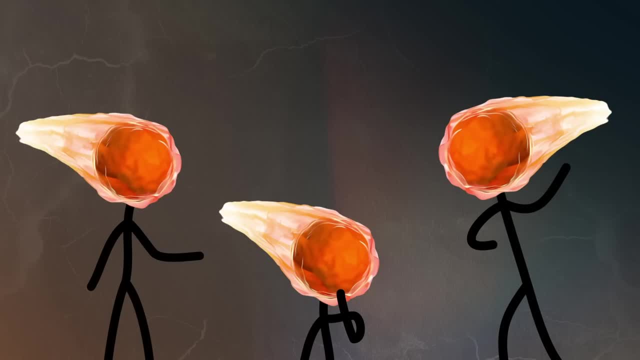 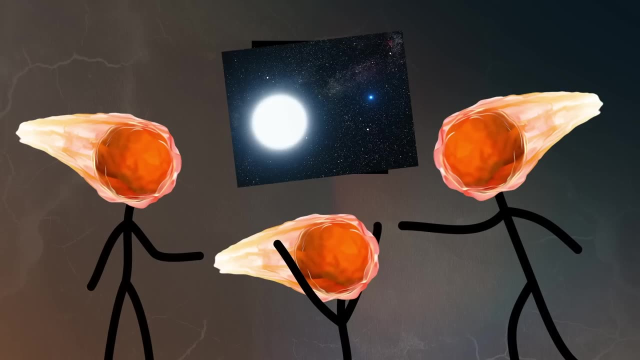 every 26 million years. What like a gravitational disturbance? Yes, yes, maybe it's the fabled planet X. Or maybe our Sun has a secret twin star called Nemesis. Or maybe it's intersection with a galactic plane Weirdos. 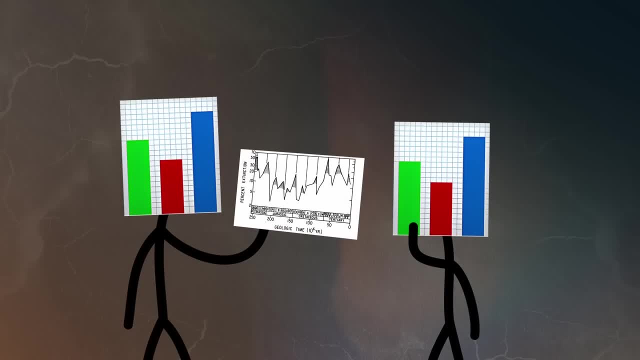 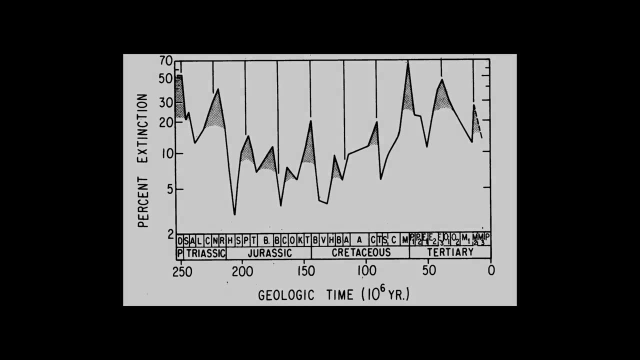 Statisticians were divided on the idea. Some acknowledged the supposed trend, others saw nothing. Reassessment and lack of corroborating evidence since means that nowadays periodicity has been dropped and everyone's pretty embarrassed about the whole episode. But you know, it was fun while it lasted. 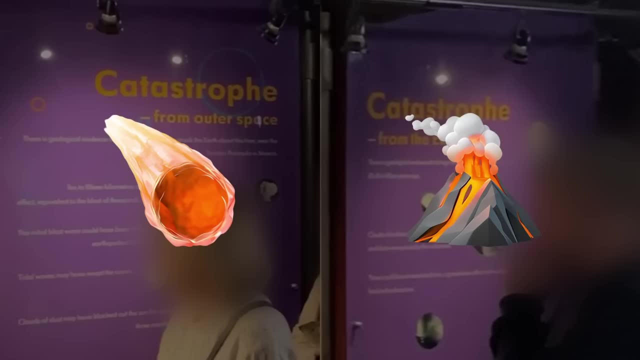 9. BOTH Throughout this video, you might have been screaming a simple question at me. If an asteroid impact and volcanism occurred together at the K-Pg boundary, why not both? Could a combination of the two extremes have driven the dinosaurs beyond their 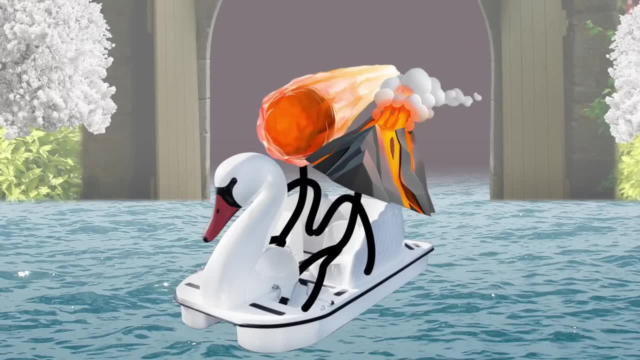 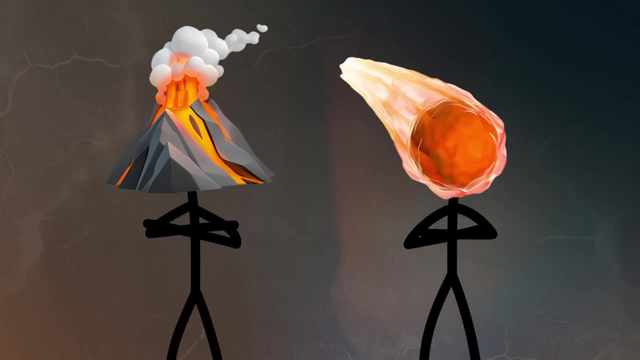 breaking point. And hey, people in the midst of heated arguments love being told to kiss and make up and come to a compromi-. oh wait, no, They don't. Impactors refused to study the possibility as it could have bolstered the volcanists. 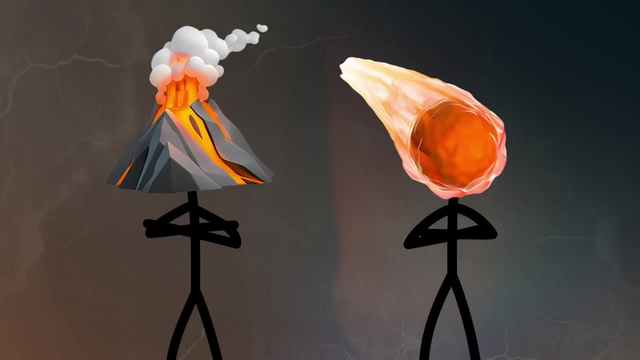 and volcanists refused to study it, as it could have bolstered the impactors. There was therefore an information void when it came to compromising. In this video, I'm going to talk about the two theories, but I'm also going to talk about the. 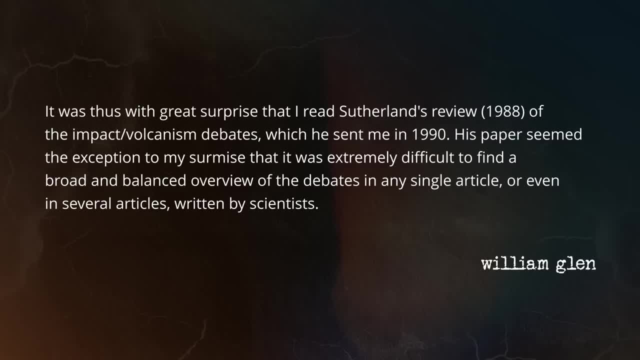 other two theories as well. Glenn cites only a single academic review which was balanced and comprehensive for the two theories, But it still supports the hypothesis that researchers were only fair towards their own theory because the author believed in both Simultaneous independent 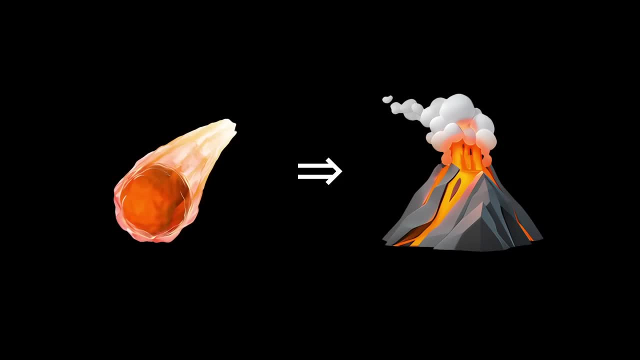 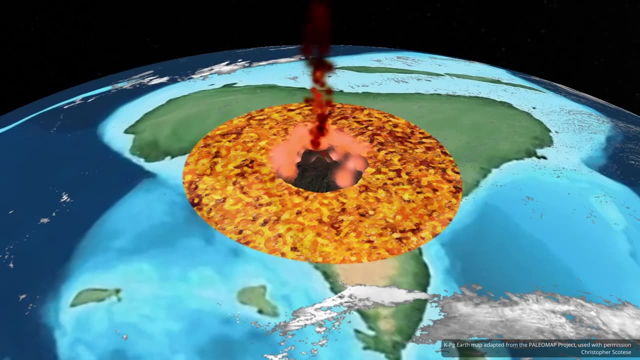 catastrophes. For those asking what if the asteroid caused the volcanoes? there's been significant research into this in recent years. The decantraps started spewing lava long before the asteroids sent them into overdrive is quite popular. For those asking what if the volcanoes? 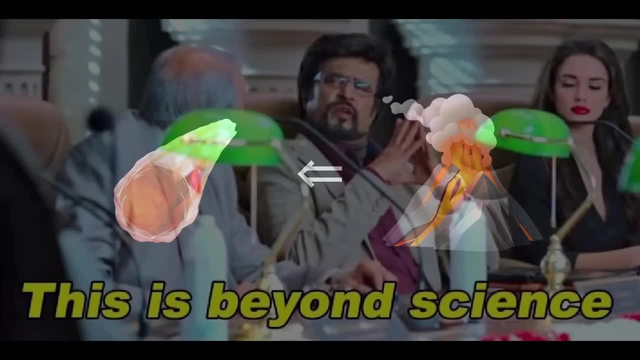 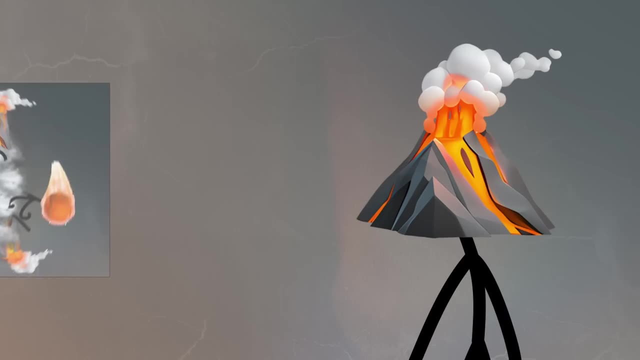 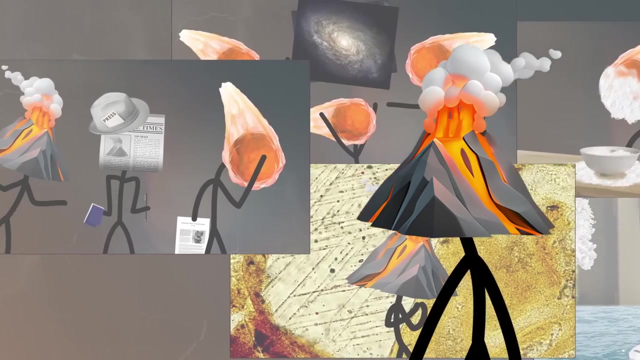 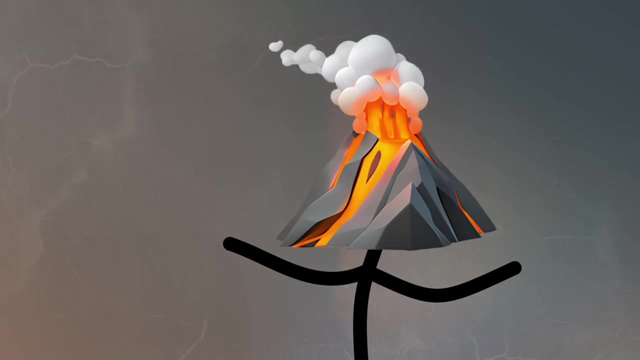 caused the asteroid. you are officially beyond science, Number 10. Conspiracy: The volcanists gazed upon the landscape of the debates. They saw ignorance and arrogance, They saw fighting and chaos, They saw war And they said: none of this is science. None of this is. 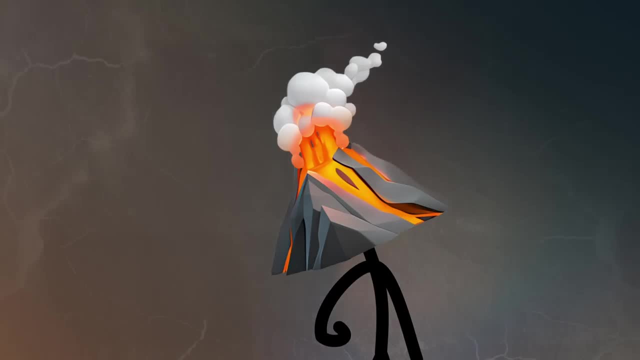 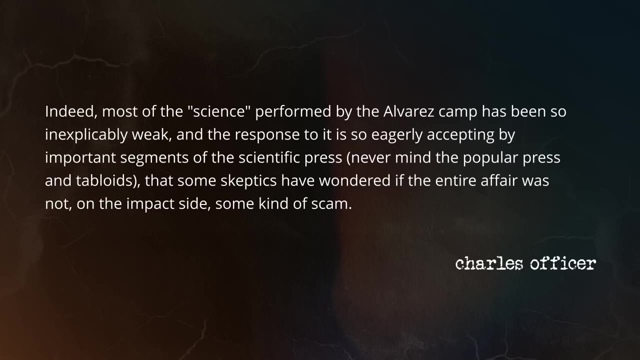 logical. None of this is bringing us closer to the truth. The only logical explanation is that the whole thing is a scam. Accusations of conspiracy are well documented, but pinning down who orchestrated it and to what end is a fair bit harder. Volcanists argued that journals were 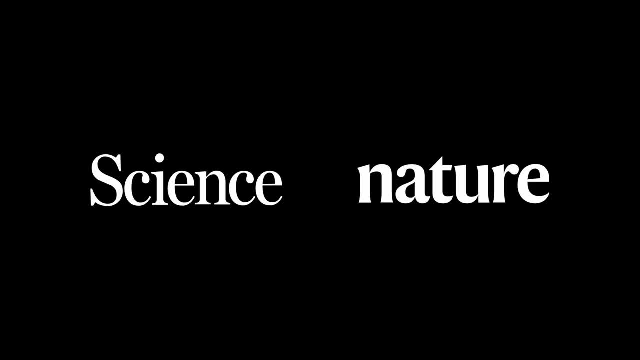 rejecting papers that discredited the impact theory. Some version of this sounds likely. The seductiveness of a sudden end is much easier to present for a general audience than the slow march of volcanoes. This, of course, bled into mainstream press. 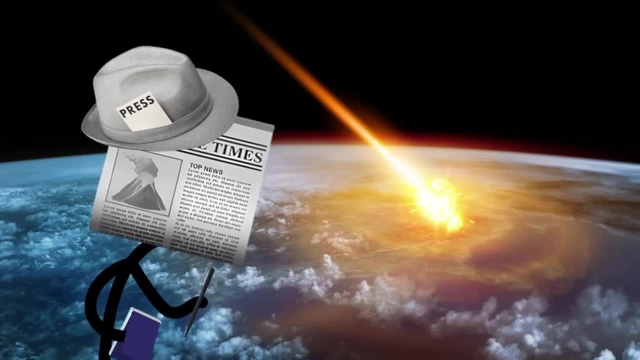 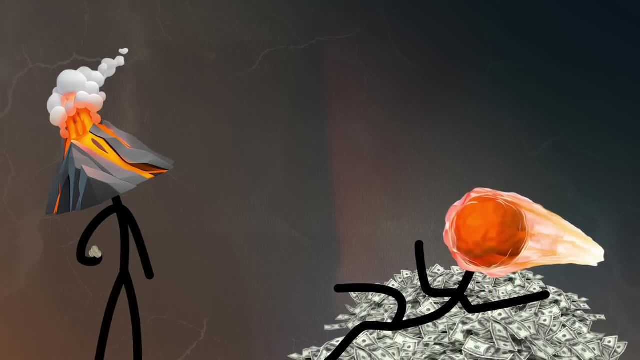 Even compared to their rival asteroids, were just so much sexier, as we'll explore shortly. And again, careers were on the line here. Impact in the press meant impactors got all the funding they could ask for, while volcanists were neglected. It's entirely possible this was. 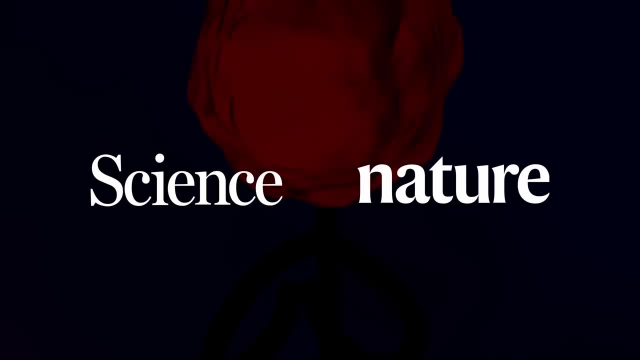 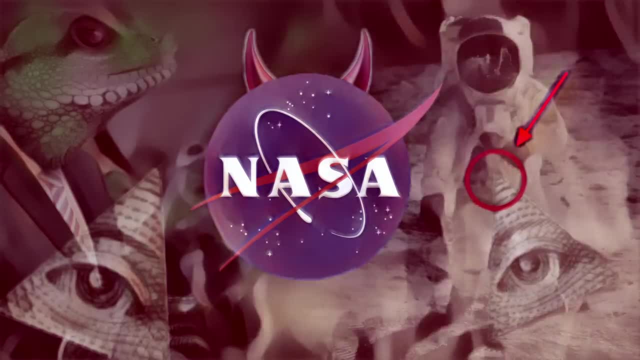 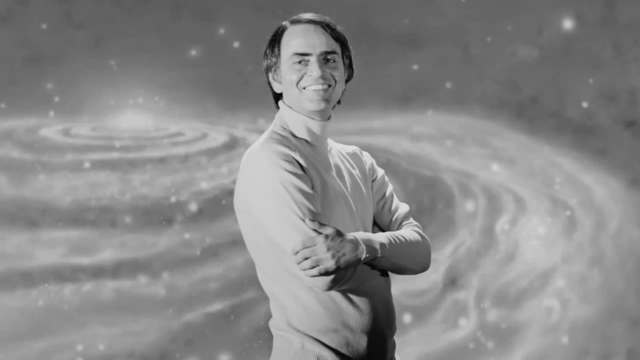 a real phenomenon without underhand manipulation. But was something more going on? General rumblings point to NASA that staple of conspiratorial belief. They were selectively funding dodgy impact research to drive public interest in asteroid defence programmes. Meanwhile, Carl Sagan took the impact hypothesis to new heights of salience in 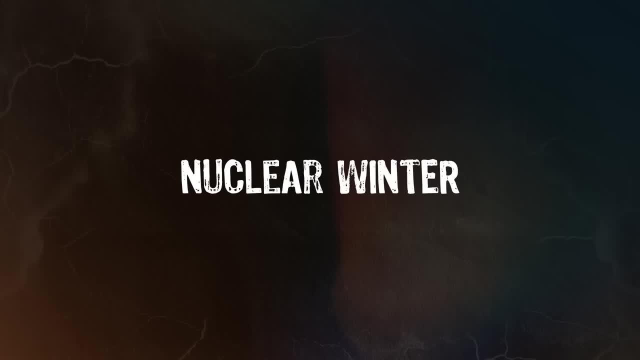 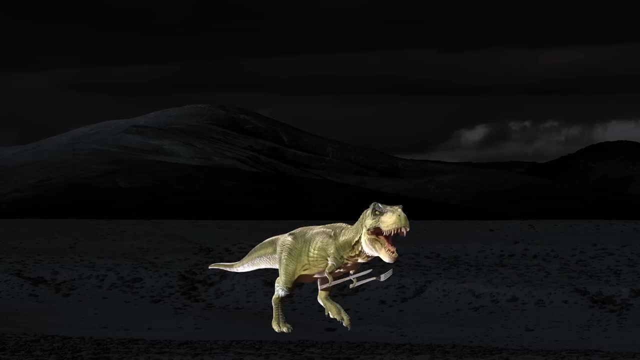 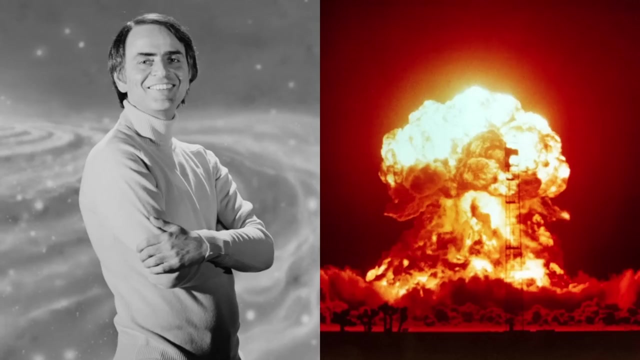 1983. Enter nuclear winter. Inspired by the impact winter scenario, he asked: would nuclear war lead to similar global darkness and extinction? He believed it would and he circumvented the scientific press to bring the matter to public attention before anyone could argue. Was this link? 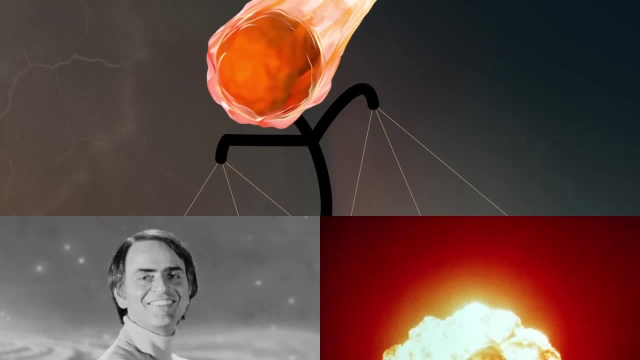 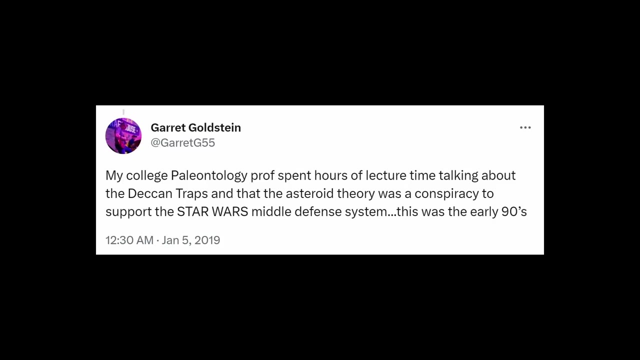 to cold war paranoia, another attempt by the impactors to drown out alternatives Speaking of the cold war. if this tweet is to be believed, it's not. I want to be very clear. this is a joke. I'm not putting words in anyone's mouth. 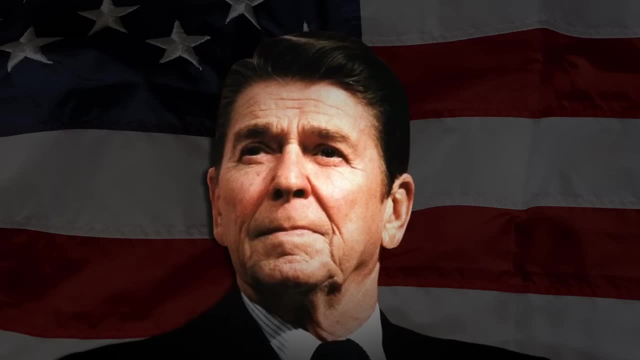 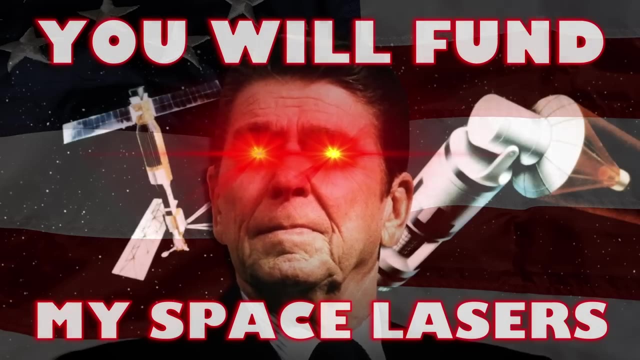 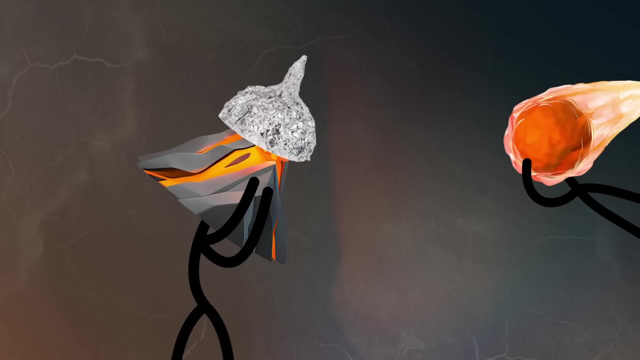 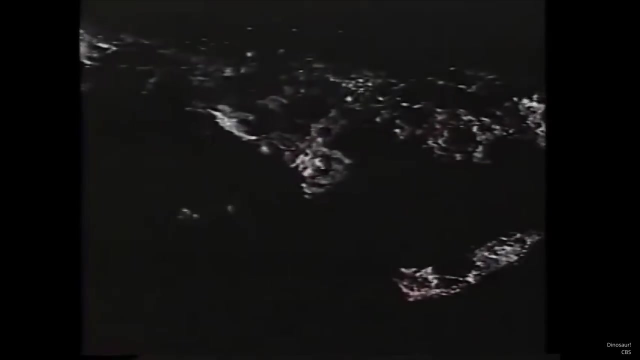 this thing goes right to the top. Ronald Reagan himself has brainwashed all of us into believing the impact hypothesis, because our fear of asteroids will leave us no choice but to fund his space lasers. Hey you, okay, man. No, By hook or by crook, impactors were winning hearts and minds. 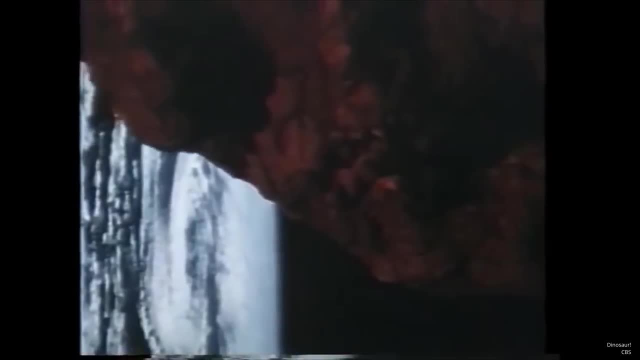 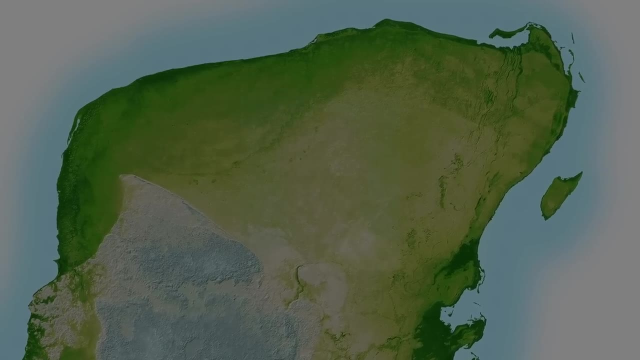 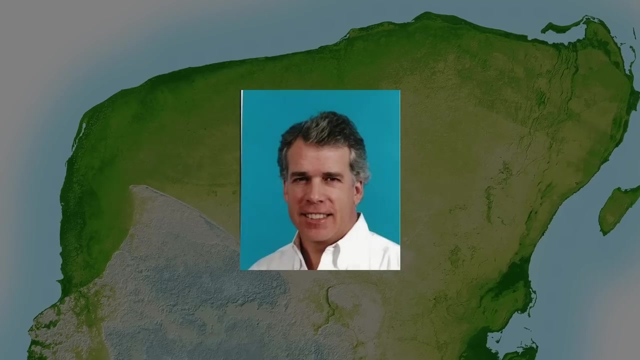 The debate was swinging their way, But they still lacked the knockout punch. Where was the crater? The answer would come in 1991.. Following a trail of clues that began with tsunami deposits in Texas, continued through 40-year-old Mexican oil drilling records and concluded below. 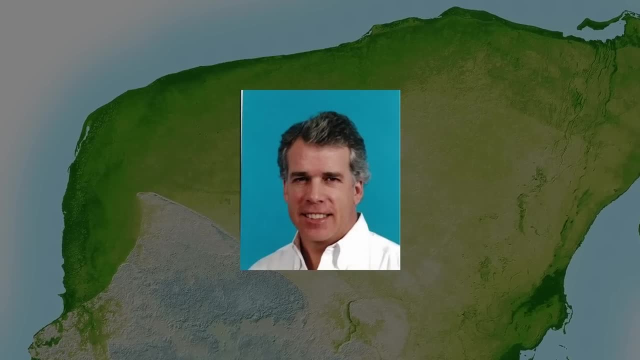 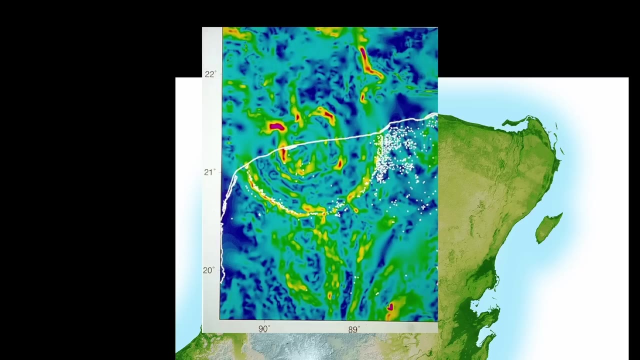 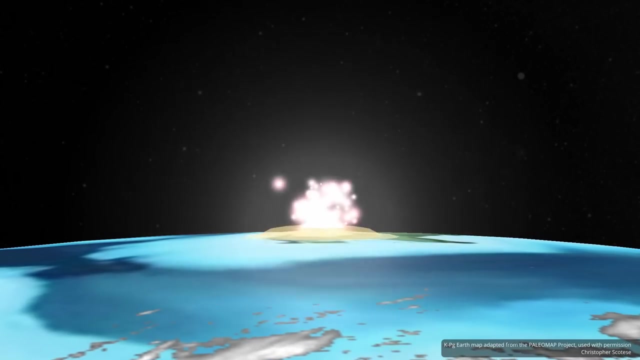 Chicxulub, a man named Alan Hildebrand found. it Dated to 66 million years old. this submerged gravitational anomaly marks the impact site. The evidence has since overwhelmed even the most hardened impact opponents. An enormous asteroid struck the Earth at the K-Pg boundary. 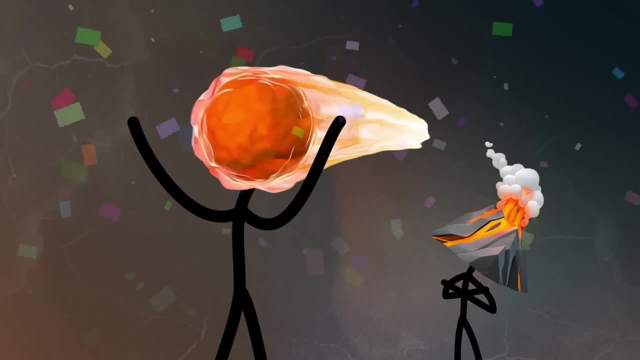 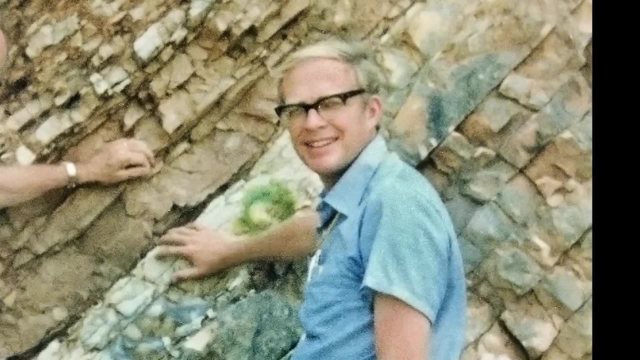 Impactors declared victory. Uniformitarianism had been overthrown. Long live the asteroid. His first forays into the forums now a distant memory. Walter Alvarez himself wrote a book, T-Rex and the Crater of Doom, joining many in the popular 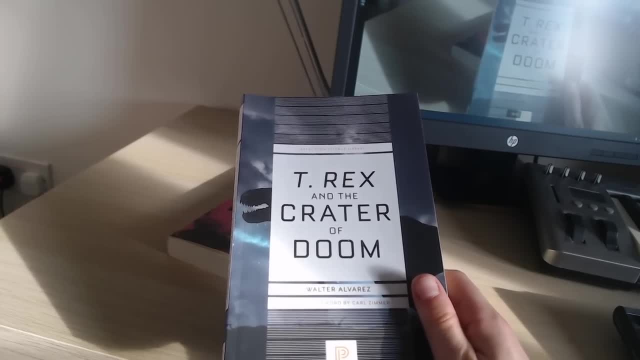 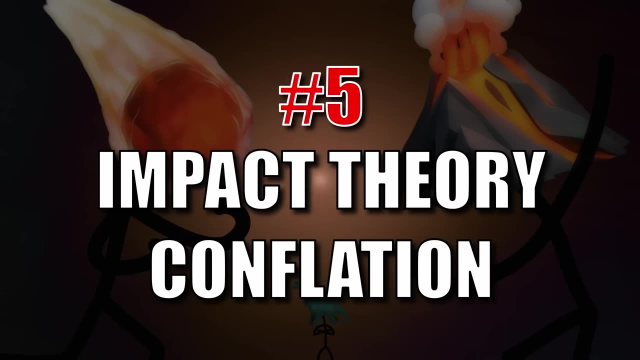 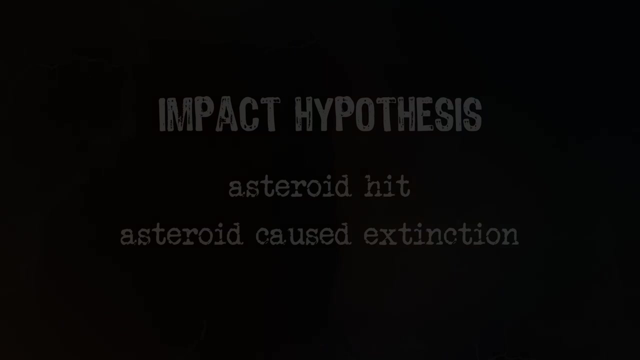 press in framing the whole debate as a search for the crater, the smoking gun. With that hypothesis confirmed, what else was there to say? But you have to remember point five: An asteroid hit, sure, But did it kill the dinosaurs? A lot happened in the 14 years after 1980.. Paradigms shifted, alliances formed. 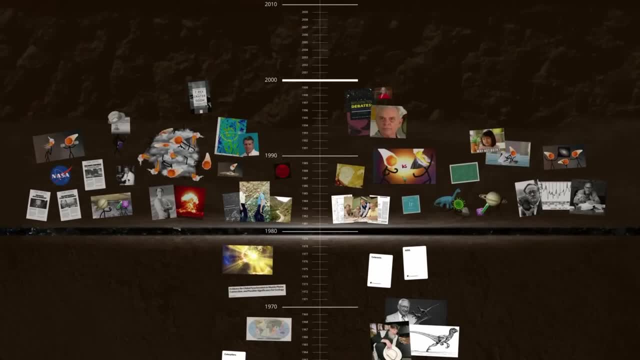 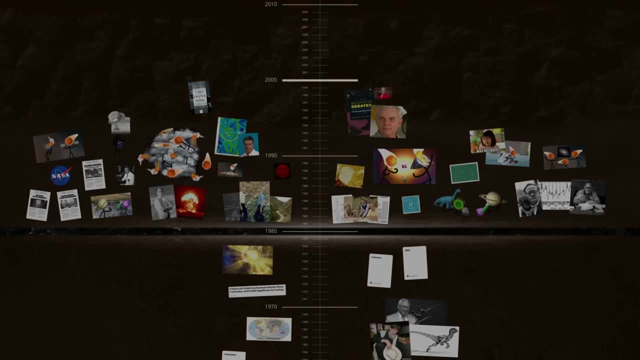 rivalries flared, One side emerged the apparent victor, changing the face of prehistory forever. The debate would continue, of course, hanging onto the question a crater alone can't answer, But the intensity of the 80s has yet to return. 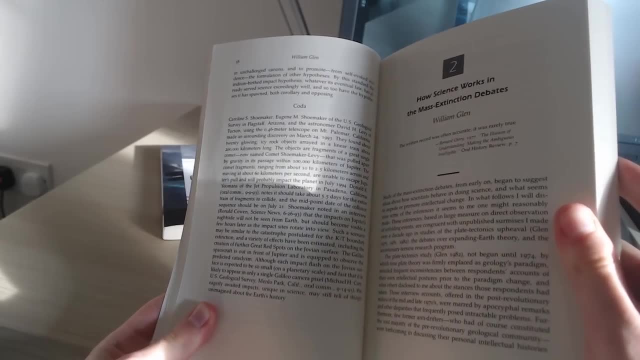 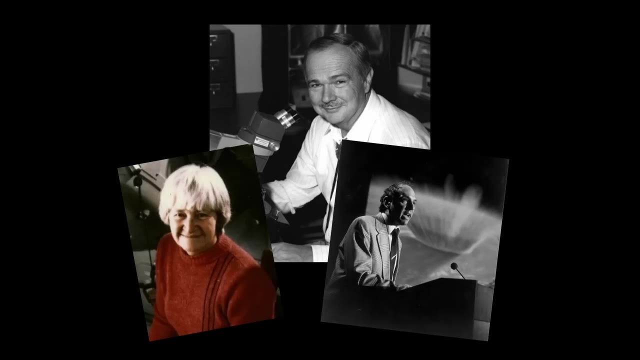 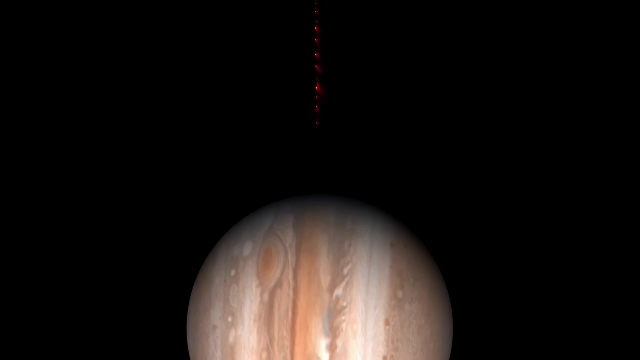 The mass extinction debate concludes in 1994 with an intriguing interjection of stock press. A year prior, Gene Shoemaker, together with Carolyn Shoemaker and David Levy, spotted a comet cluster, a collision course with Jupiter, Named Shoemaker-Levy 9, the cluster offered an ironic opportunity. 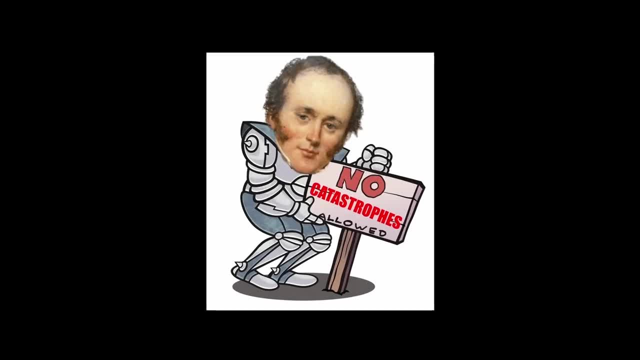 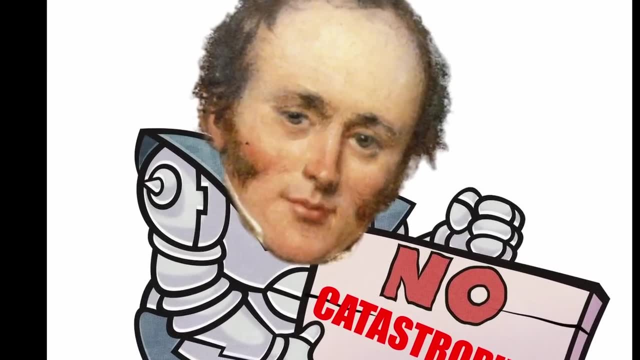 If present processes are the key to past processes, what happens when an asteroid impact observed and verified around the world becomes a present process? 14 years of trading blows trying to get rid of it, and it turns out uniformitarianism had never left. 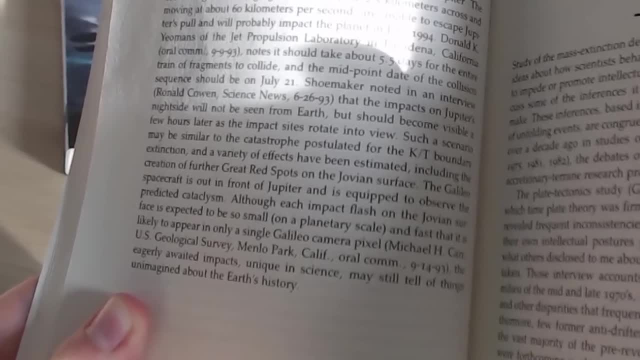 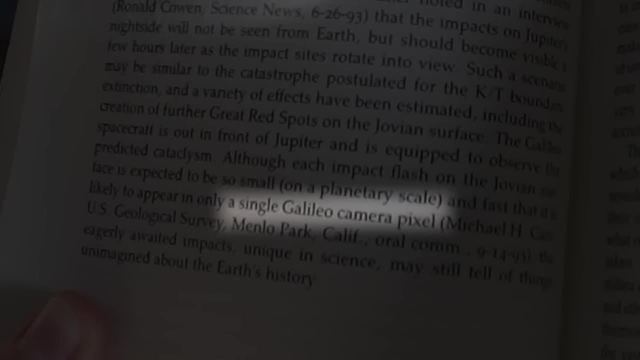 Glenn's coder, written a few months before impact, says the effect on Jupiter is a expected to be small, To be at most a few pixels in the Galileo spacecraft's camera. I wonder how that's going to turn out. Part 4: 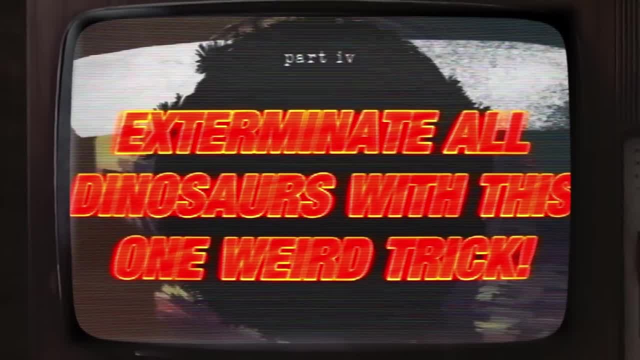 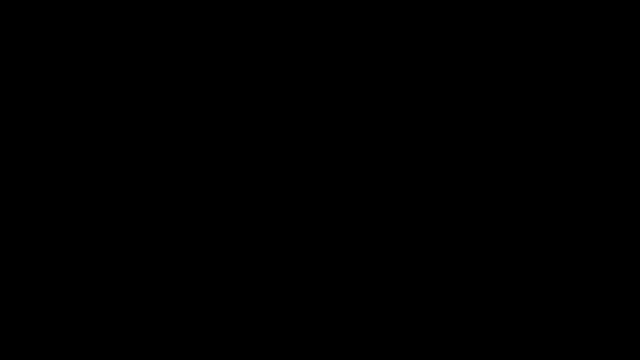 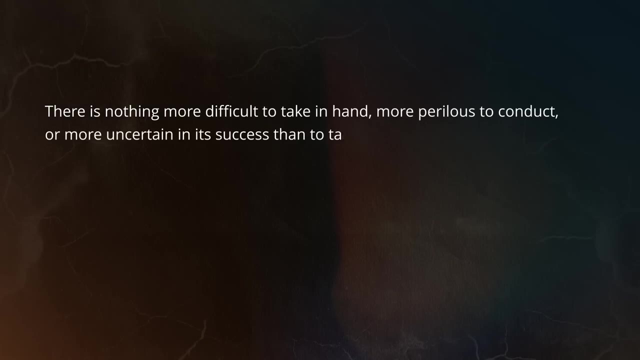 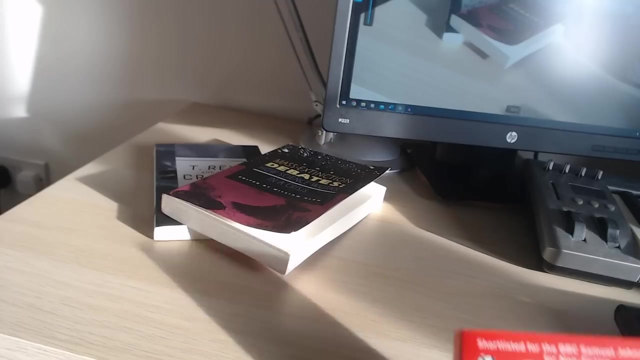 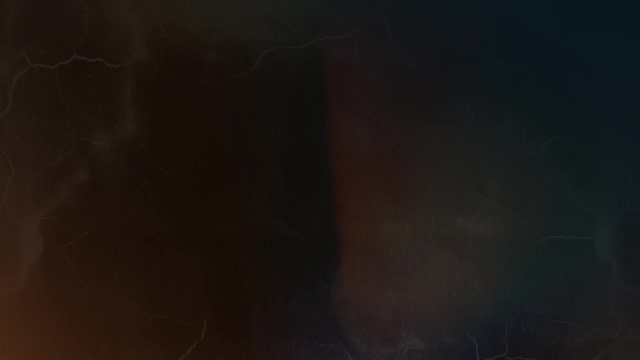 Exterminate all dinosaurs with this one weird trick. What happened in the first place Plays The. In his book Bad Science, Physician and science journalist Ben Goldacre characterises the media's depiction of science as 6. Groundless, incomprehensible didactic truth statements from scientists. 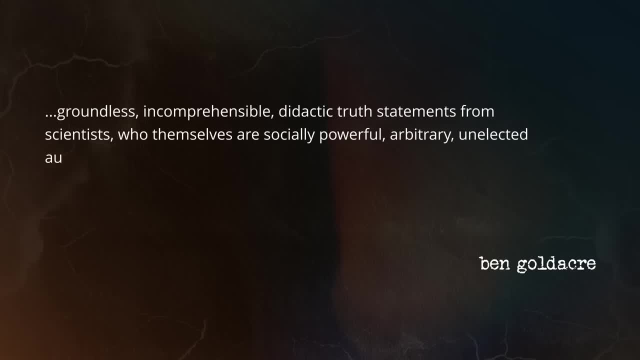 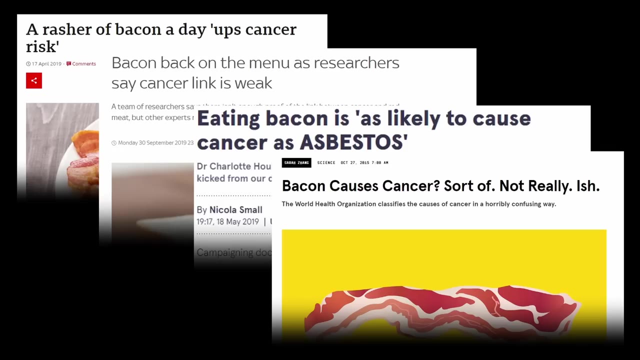 7. Who themselves are socially powerful, arbitrary, unelected authority figures. Everything in science is tenuous, contradictory- probably going to change soon- and most ridiculously hard to understand. The focus of Goldacre's ire is medical journalism, which I hope you'll agree is in far dire straits. 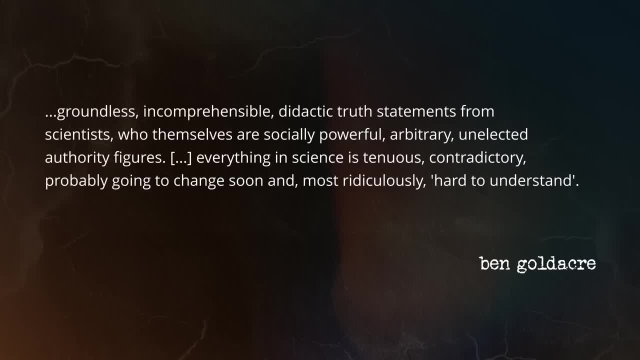 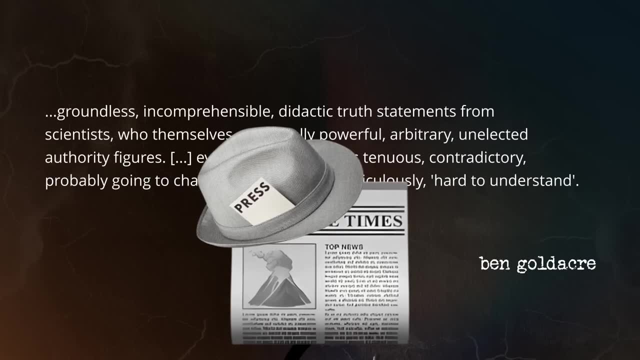 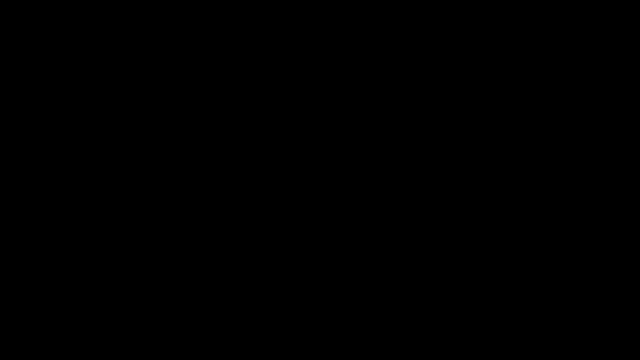 than any other science. But do his claims point to systemic issues across science communication? Do they apply to the media's role in the mass extinction debates? even today, Goldacre points to three types of endemic science news stories as evidence of mass media's harm to public perceptions, Wacky Scare and Breakthrough. Can we find examples of each? 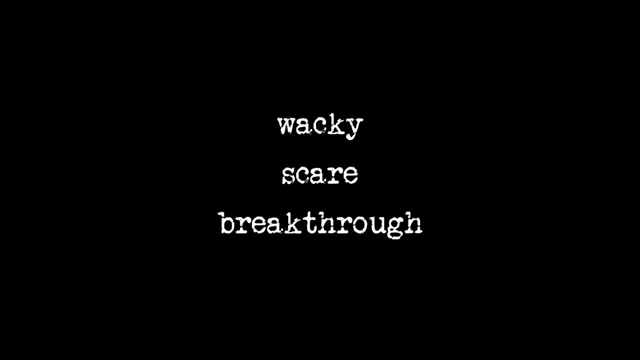 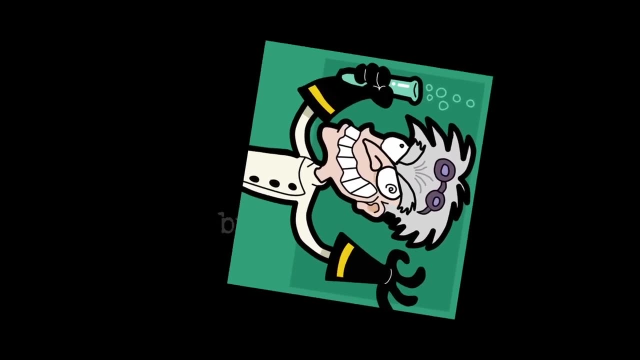 in KPG reporting, and are they still shrouding the question in too much uncertainty? Let's begin with Wacky. These are the stories that depict scientists as silly old coots off their own fantasy worlds. You know boffins. 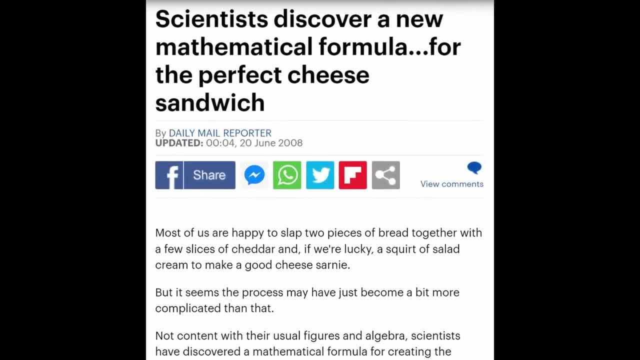 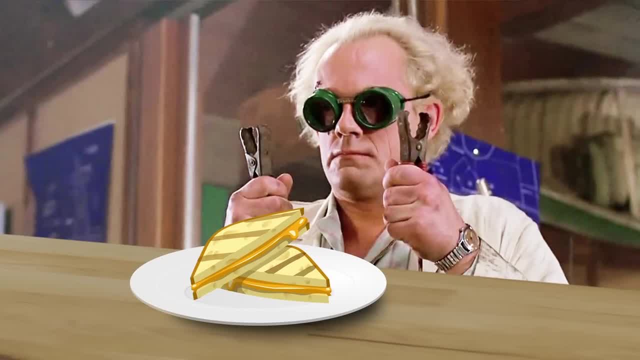 It might seem innocent, but this approach risks turning society's view of science into a parody of itself. If science is all just a silly, fun-time side-quest, what motivation is there to trust it? Why listen to a bunch of caricatures? who care so much about nonsense? 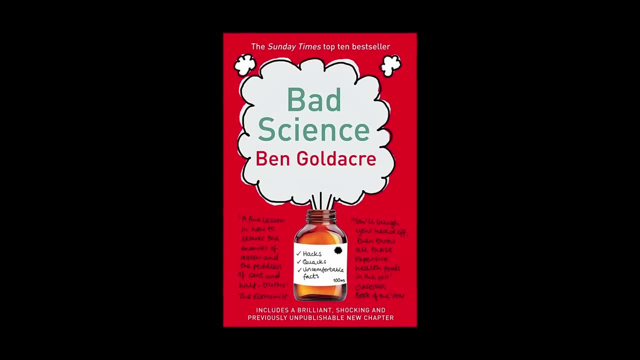 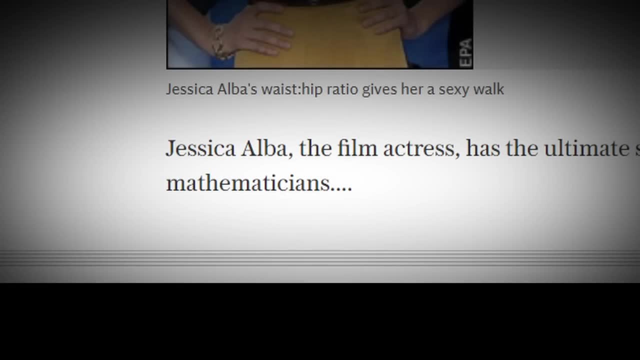 Uh-oh, Maybe it's the mathematician in me talking, but one example from Goldacre irks me way more than any of those that are objectively worse. Jessica Alba, the film actress, has the ultimate sexy strut according to a. 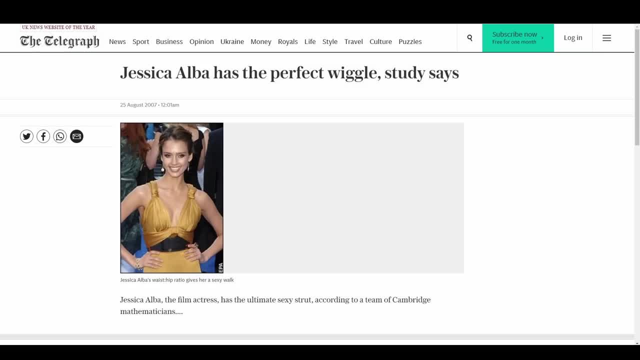 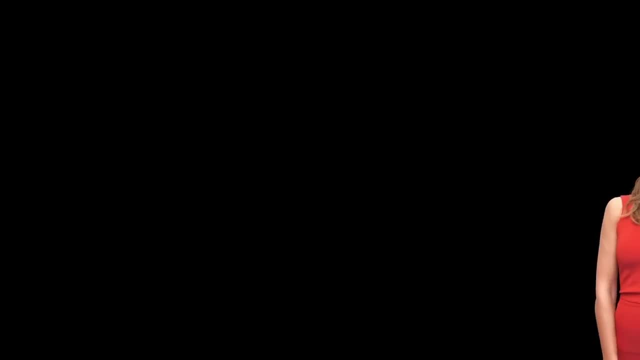 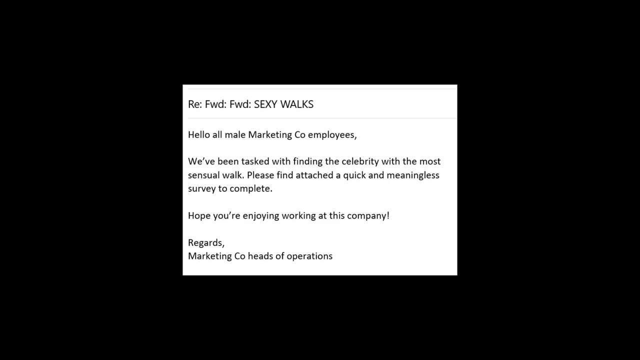 team of Cambridge mathematicians. So said British newspaper The Daily Telegraph in 2007.. Had Cambridge number wizards really proven the superiority of Alba's hip movements? No, A marketing firm had conducted a survey of its own employees to find the celebrity with. 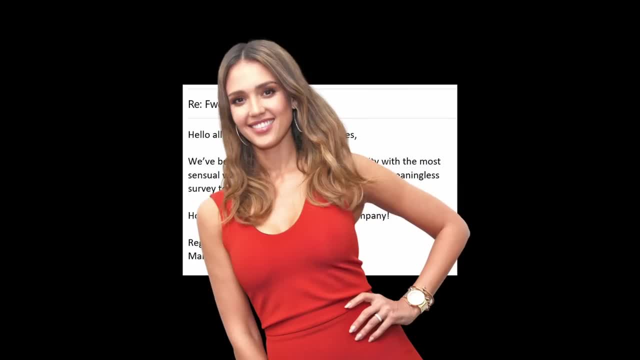 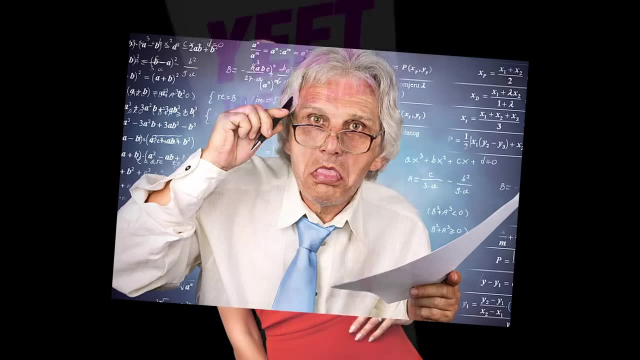 the most sensual walk, ignored the results and said Jessica Alba won anyway. duped a mathematician into coming up with a formula for sexy strides to masquerade as something scientific, and the whole thing walked away. was commissioned to promote a brand of hair removal cream. 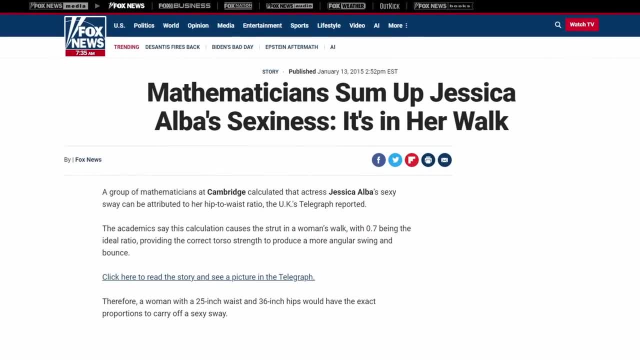 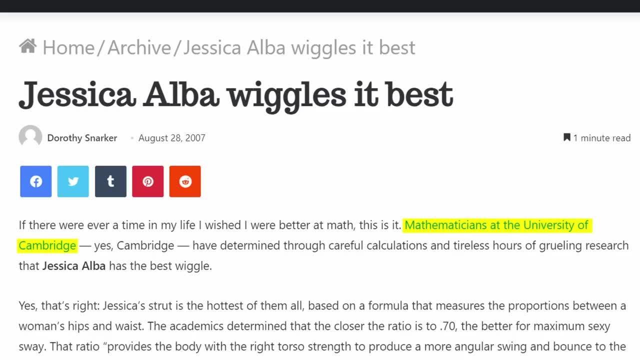 This absolute mockery of scientific principles spread to news networks as far removed as Fox News and a lesbian lifestyle magazine. Mathematicians at the University of Cambridge- yes, Cambridge- have determined through careful calculations and tireless hours of grueling research that Jessica Alba has the best wiggle. 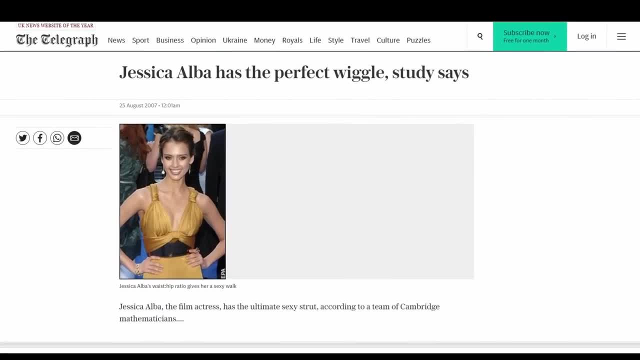 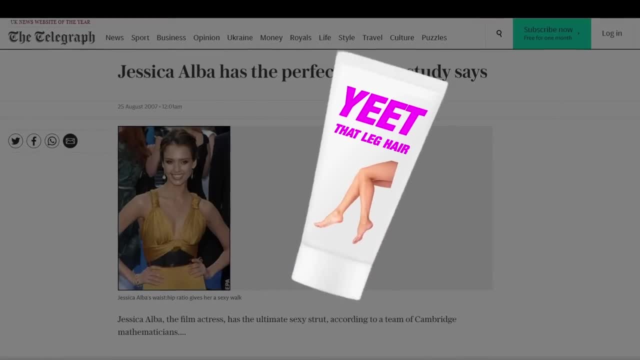 Somewhere along the line, Britain's favourite toilet paper brands discovered that backing up shoddy surveys with manipulated scientific claims was a ticket to virality. Even better when firms wanting to promote stuff can pay you to do it. And you may be thinking: Oliver, this is a video about dinosaurs. why the hell are you? 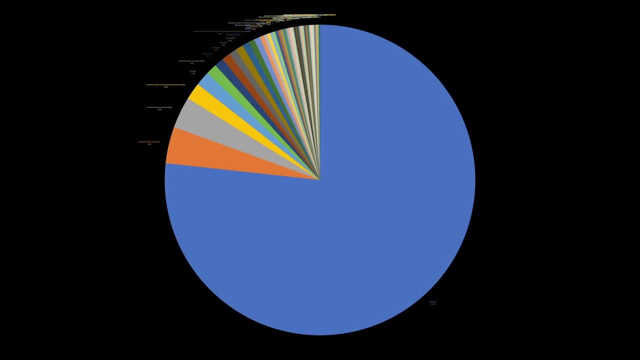 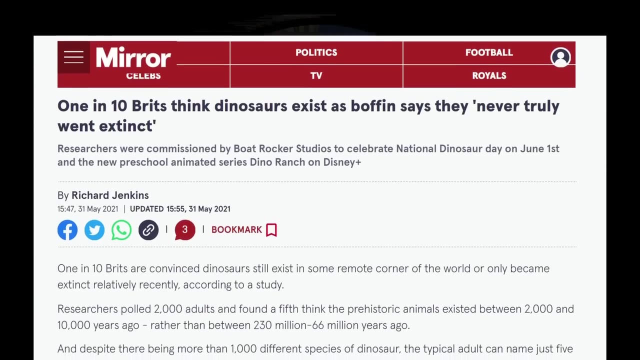 talking about Jessica Alba. Well, the sum total of my attempts to find existing data on modern public beliefs about the KPG extinction amounted only to articles like this 2021 piece from the Daily Mirror. One in ten Brits think dinosaurs still exist, as Boffin says. 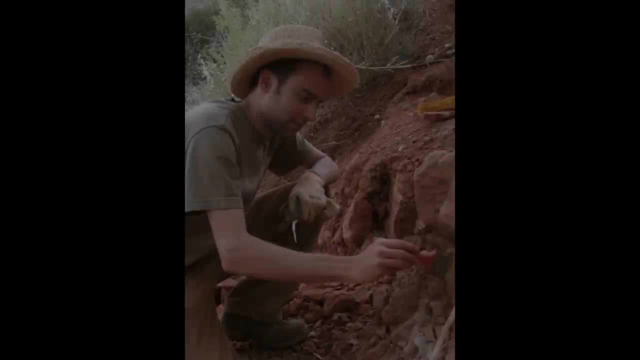 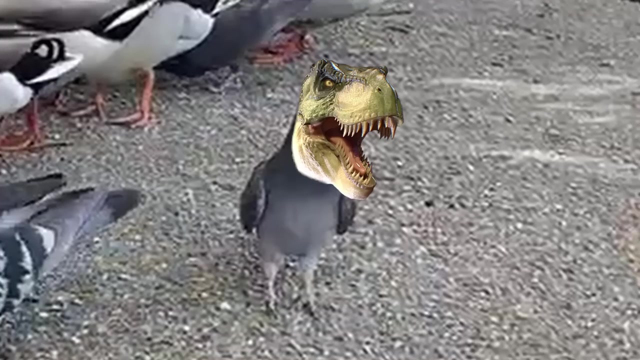 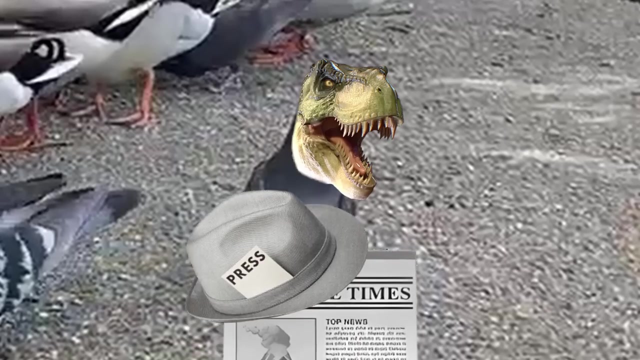 they never truly went extinct. That Boffin turned out to be Steve Brusetti, highly respected dinosaur paleontologist, And it may be no surprise to learn he was talking about the whole birds are dinosaurs thing we went over earlier. But you can't wave a tasty morsel- like technically dinosaurs still exist in front of a newspaper. 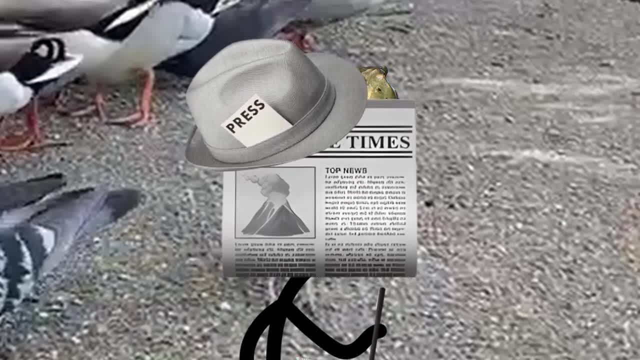 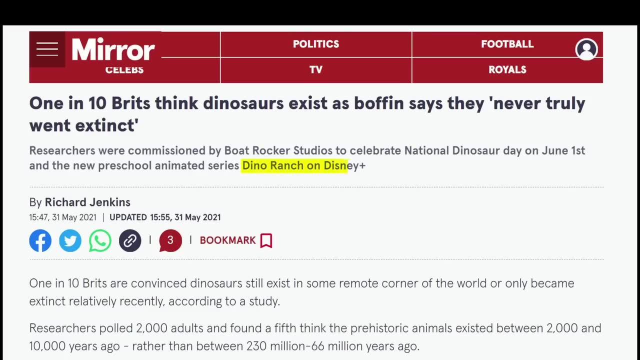 without it, mulching your words into a disfigurement of science. And when the article admitted that this whole survey, plus dodgy science stunt, was in service of promoting a dinosaur cartoon on Disney+. And when the article admitted that this whole survey, plus dodgy science stunt, was in service of promoting a dinosaur cartoon on Disney+. 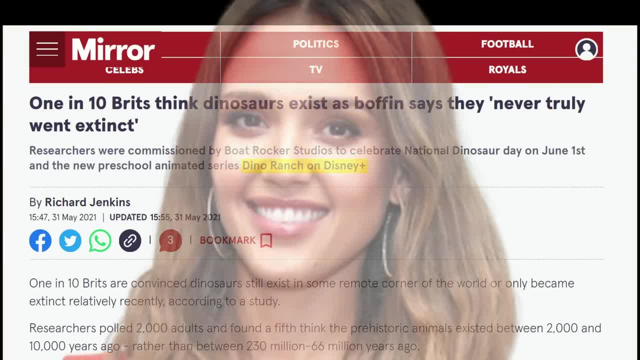 And when the article admitted that this whole survey plus dodgy science stunt was in service of promoting a dinosaur cartoon on Disney+, I felt an overwhelming surge of deja vu. While there's decent science in the article, at least in the quotes from Brusetti, the 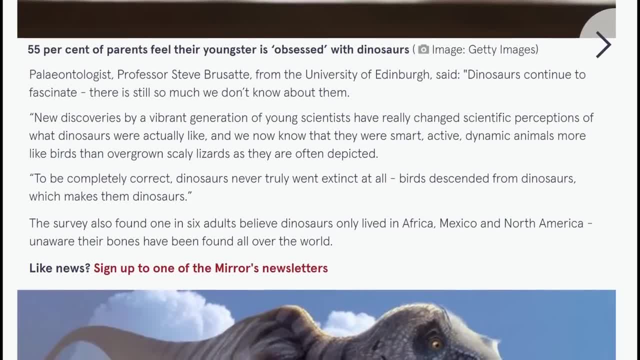 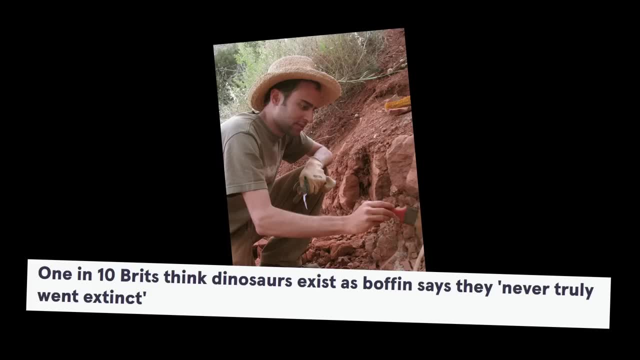 newspaper knows what it's doing. It knows portraying scientists as airheads gets clicks, no matter the damage. If an expert says something as silly as dinosaurs still exist. maybe none of them know anything. Maybe the KPG extinction is fundamentally wacky. 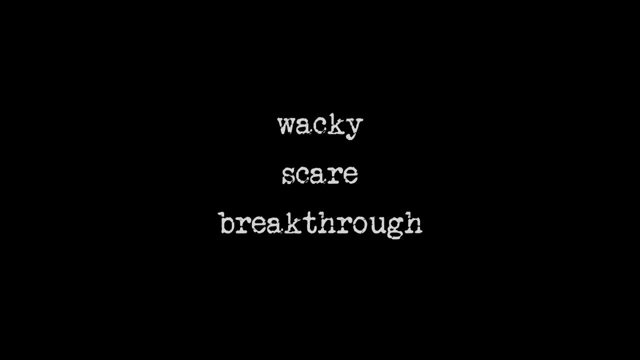 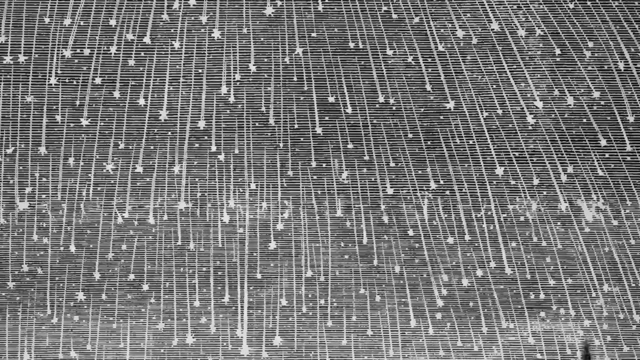 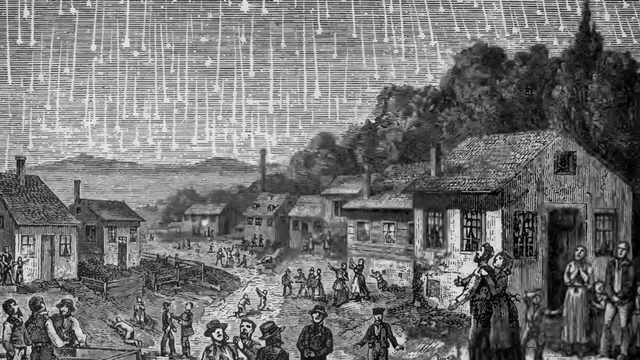 That, however, is the least of its problems. That, however, is the least of its problems. Next on our list: scare stories. Since ancient times, meteor showers have sparked fear and discontent, Demons breaking into the earthly realm to wreak havoc. 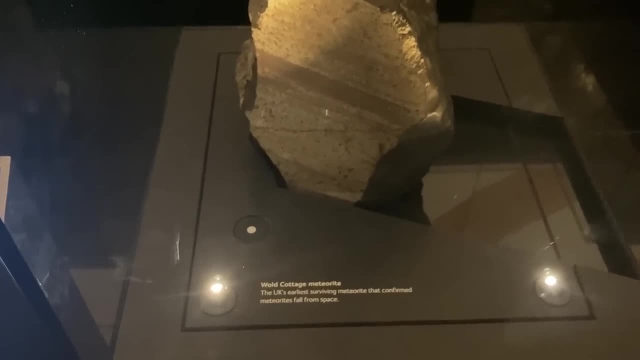 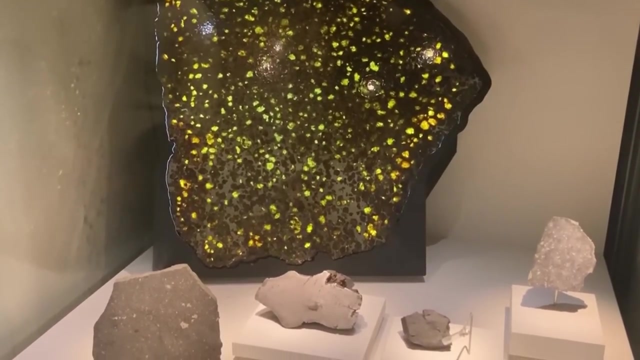 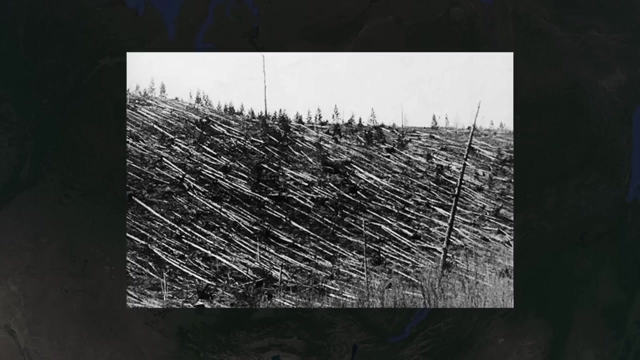 Omens of dreadful events. Thanks to this meteorite, which fell in 1795,, there has since been widespread acceptance of the reality Rocks from space. Their destructive potential has, though, helped persist the shroud of prehistoric history. The 1908 Tunguska event, a great explosion in Siberia, was immediately attributed to. 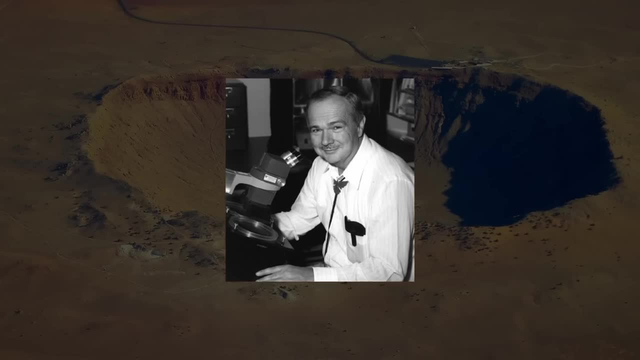 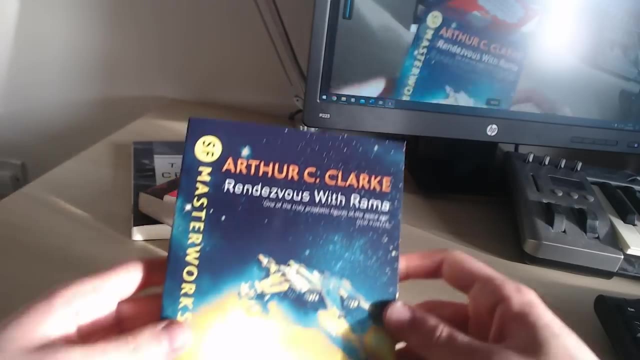 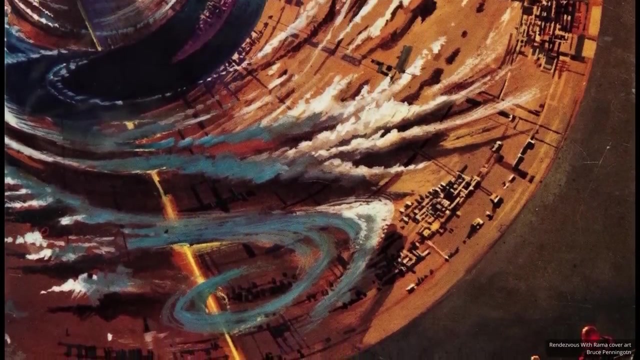 an asteroid, for instance, And, as previously mentioned, Gene Shoemaker led a revolution in astronomy over the true impact of impacts in the middle of the century. In 1973, Arthur C Clarke wrote Rendezvous with Rama. The story follows near-future humanity as they discover an alien artefact from beyond. 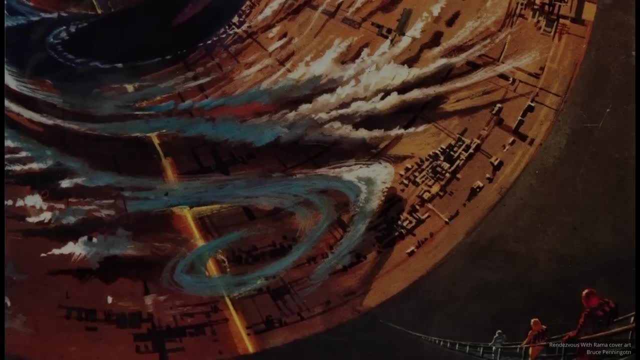 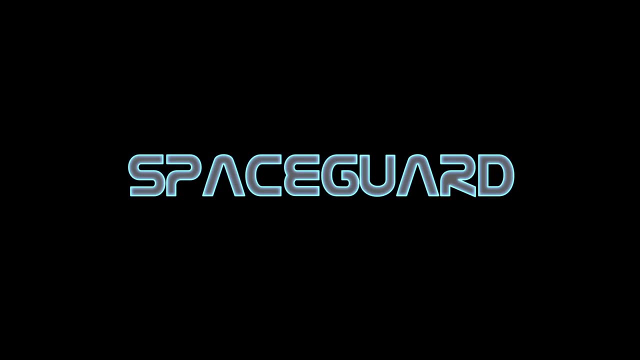 the solar system, Humanity finds the cylindrical spacecraft. The spacecraft thanks to its Space Guard program, an asteroid-tracking initiative set up in the wake of cataclysm from space. In perhaps my favourite opening chapter in literature, Clarke describes how one September. 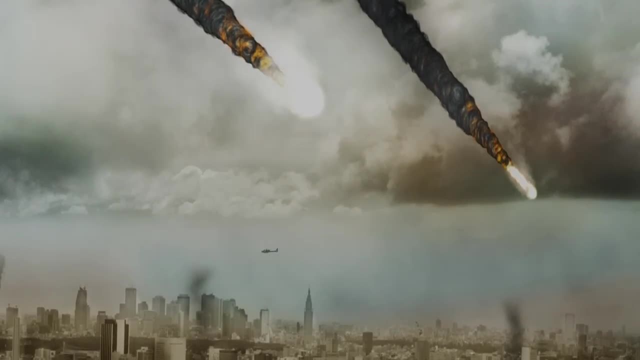 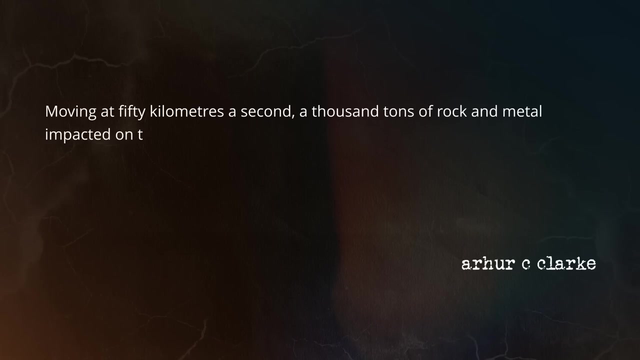 morning in 2077,, an asteroid from the blue destroyed half a country, Moving at 50 kilometres a second. a thousand tonnes of rock and metal impacted on the plains of northern Italy, destroying in a few flaming moments the labour of centuries. It was as if a great explosion had taken place. 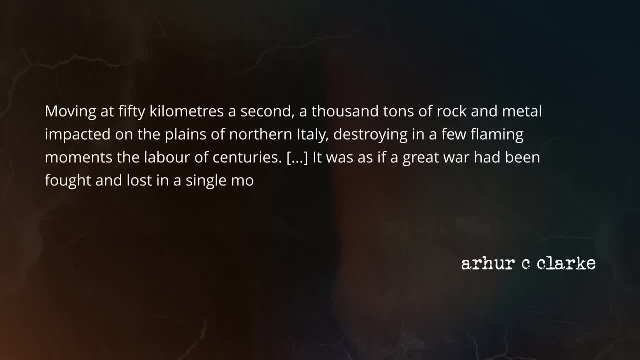 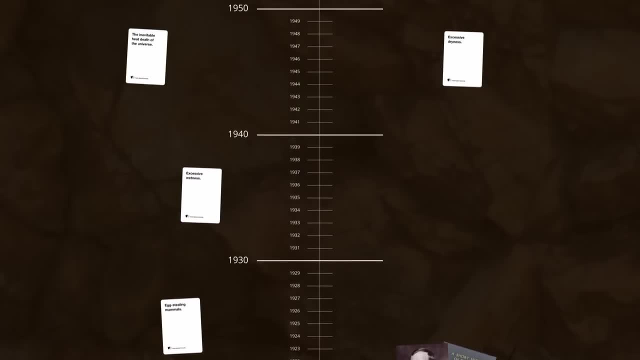 It was as if a great explosion had taken place. It was as if a great war had been fought and lost in a single morning. In light of how large the asteroid threat loomed throughout history, it's staggering that the Earth sciences remained so stubbornly reticent about extinction by impact as late. 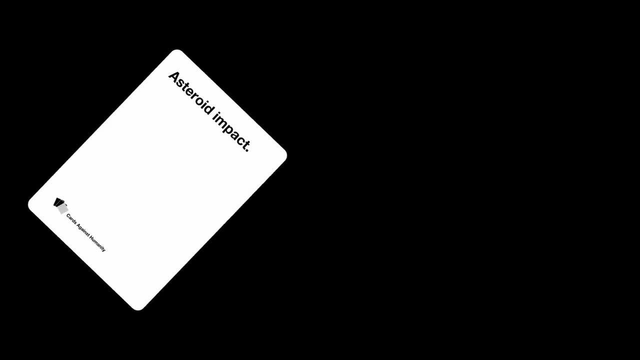 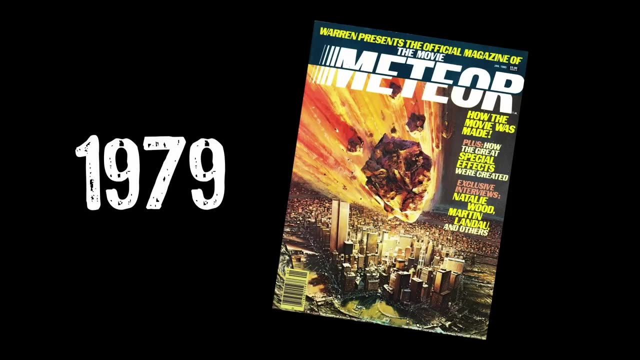 as 1980. Again, that's largely down to the prevailing view of asteroids and extinctions as unworthy of real science. But the public, They were primed and ready to believe. As scare stories go, nothing can ever hope to matter. 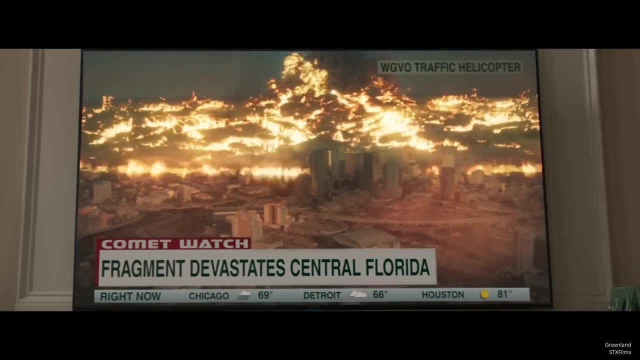 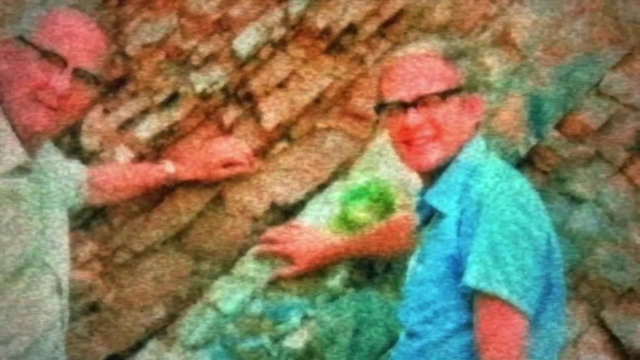 But the public. They were primed and ready to believe. As scare stories go, nothing can ever hope to match. We could all be wiped out by a space monster with no warning And as of 1980, that's coming from actual boffins. 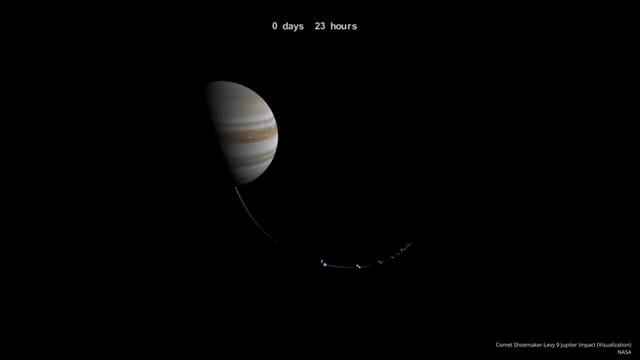 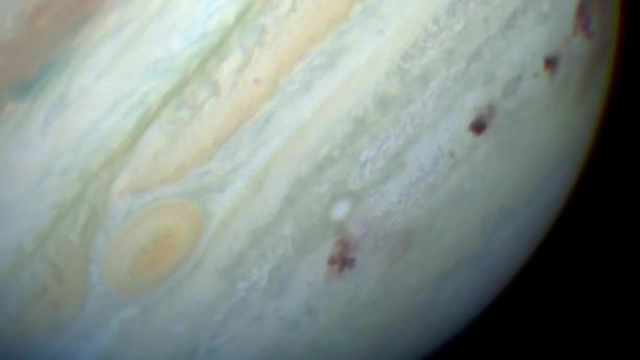 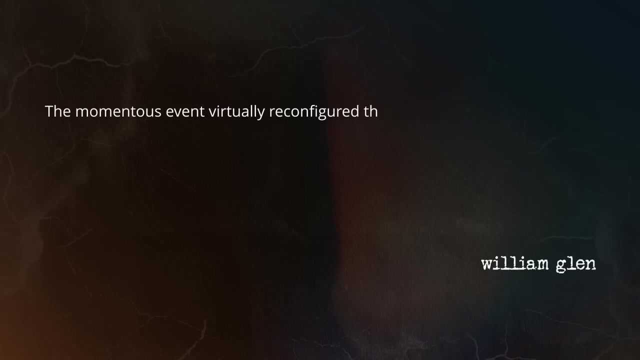 Shoemaker-Levy 9's collision with Jupiter produced a whole lot more than a couple of pixels. The scale of the fireballs produced and the longevity of the scars they left surprised even impact devotees. In the words of William Glenn from a 1998 article: the momentous event virtually reconfigured. 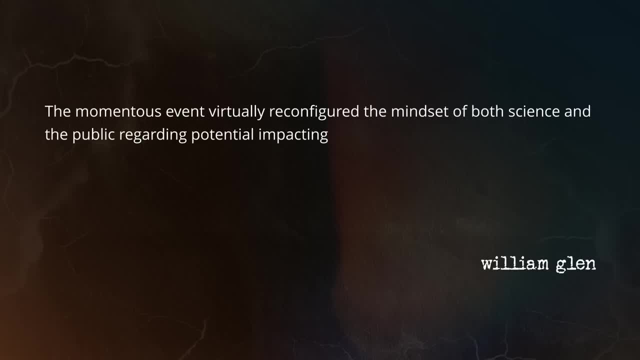 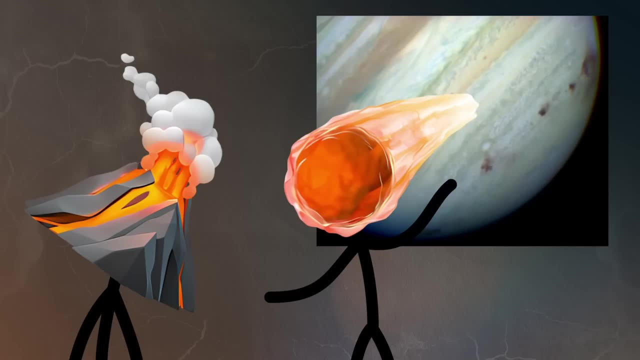 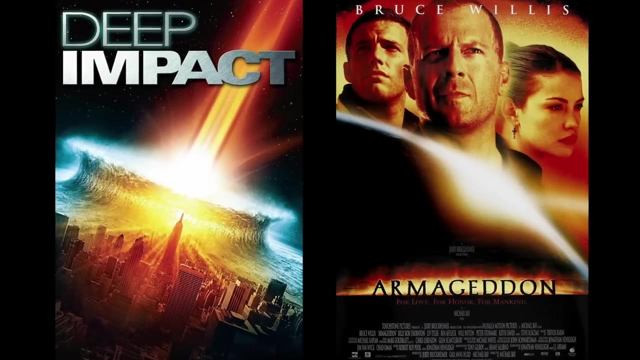 the mindset of both science and the public. The impactors now had evidence as simple and memorable as the theory it supported. The impact hypothesis soon entered a kind of feedback loop. Shoemaker-Levy 9 laid the groundwork for films like Deep Impact in Armageddon, which put awe-inspiring 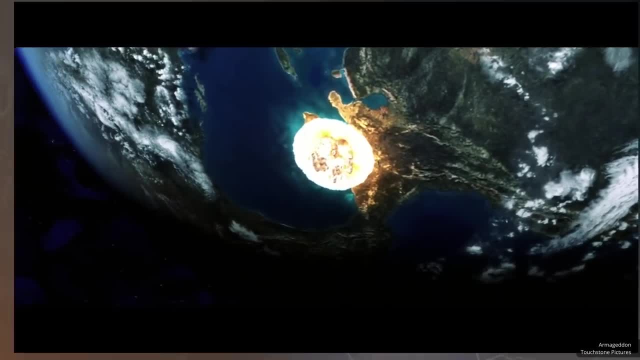 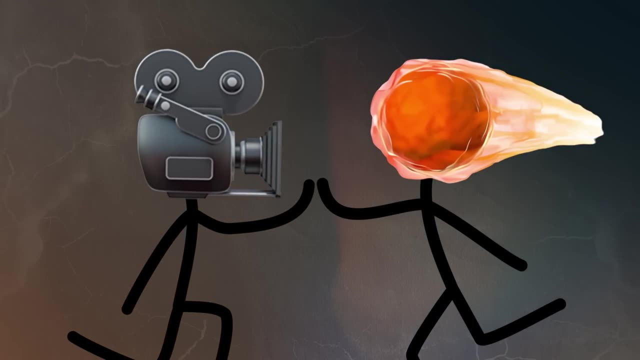 CGI depictions of death from space in society's brains. Impactors and NASA could then latch on to these popular representations as common ground, maybe even associate with them. The impact hypothesis was not the only one. Simple self-promotion or devious propaganda depends on who you listen to. 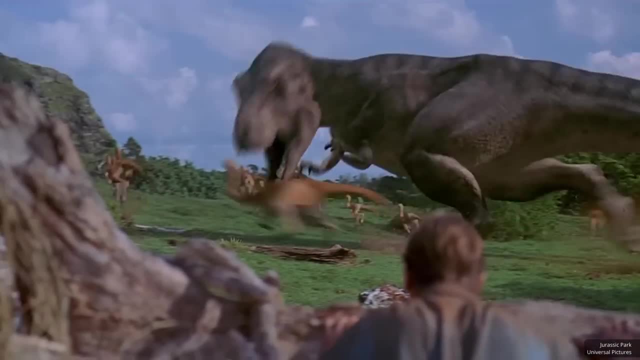 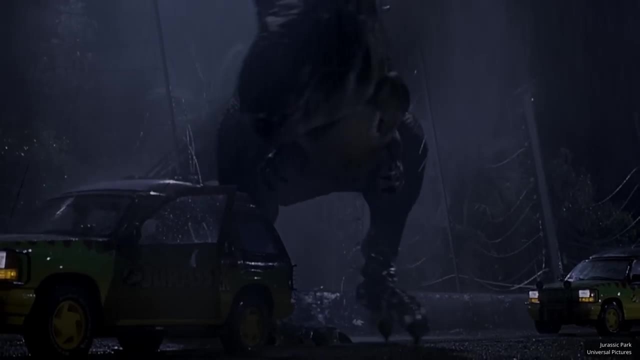 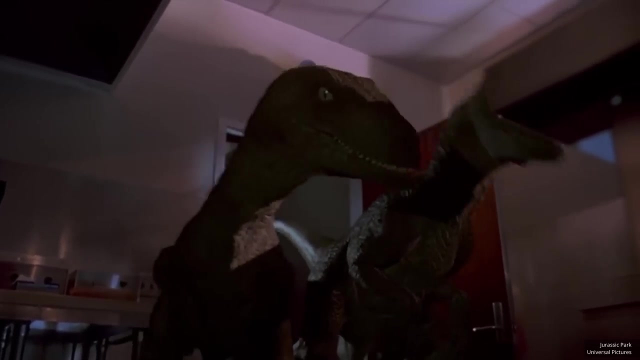 But scientific institutions are always chasing cinema as a means for drumming up support. Let's not forget that Jurassic Park was backed by paleontologists and was a major factor in embedding the ideals of the dinosaur renaissance in our collective consciousness. Finally, we all knew dinosaurs were active, intelligent and bird-like. 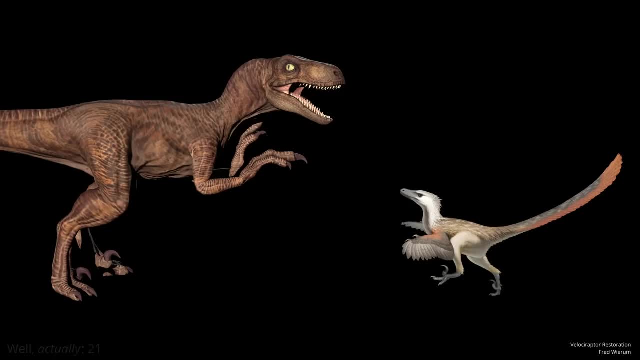 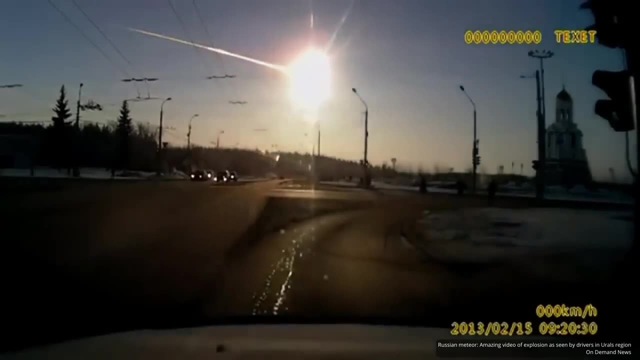 And we also knew velociraptors were the wrong size. Goddammit Impact. The mythic idea has only gone from strength to strength, since HD footage of 2013's Chelyabinsk meteor is but a YouTube search away. Or what of Umuamua in 2017?? 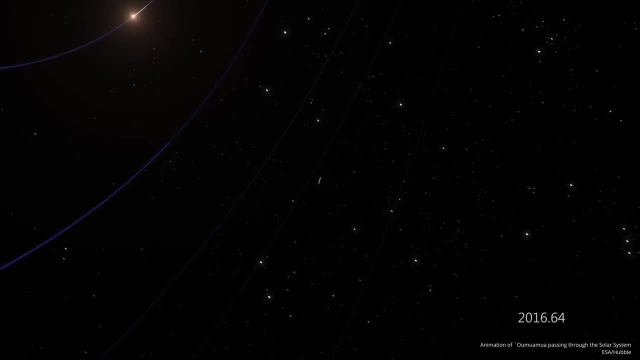 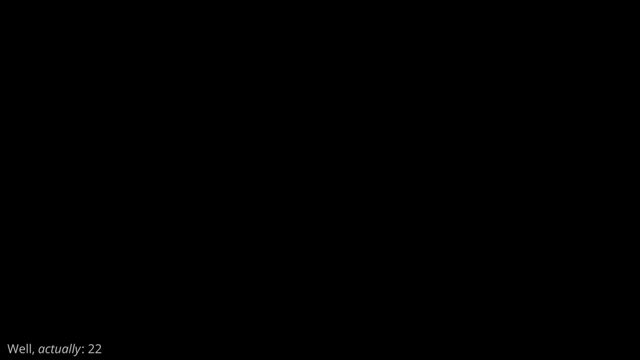 In an eerie echo of Rendezvous with Rama, a cylindrical space rock slingshot around the Sun, our first glimpse of material from beyond the solar system, Although… An object that hit Earth in 2014 is now believed to be our first recorded extrasolar visitor. 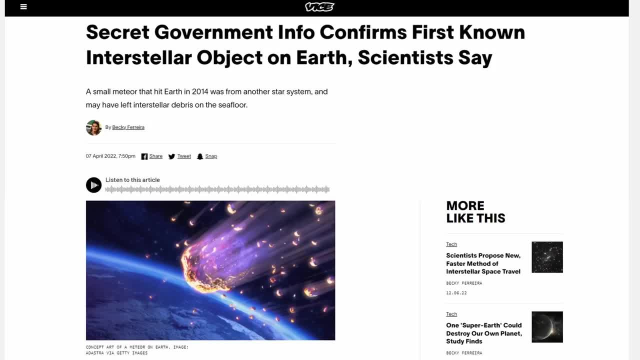 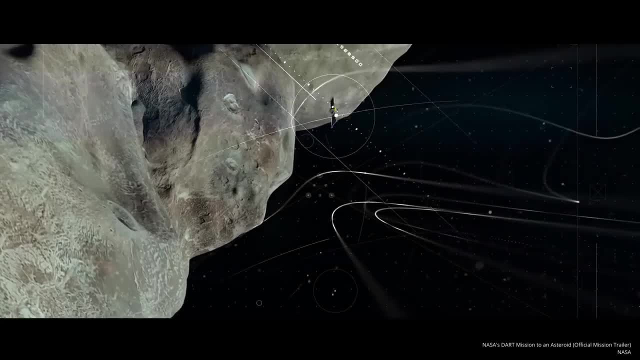 Data confirming its origin was kept classified. But it's not a new discovery. It's a new discovery because it trips the United States' nuclear detonation sensors. Asteroids are firmly part of the modern experience. No one can dispute that Their pervasiveness activates a cognitive bias called the availability heuristic. 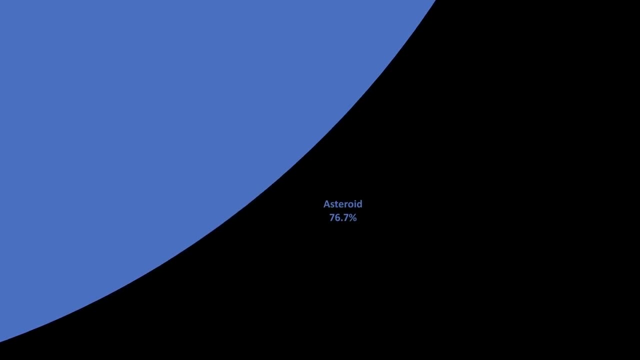 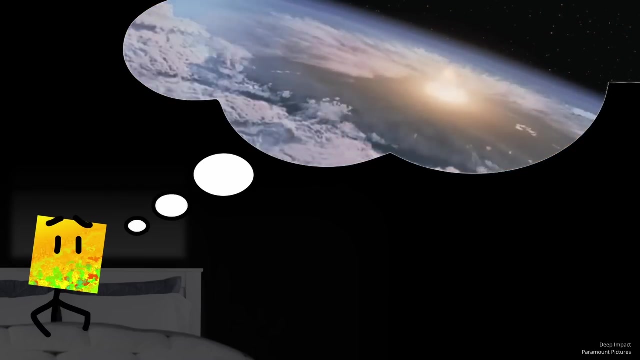 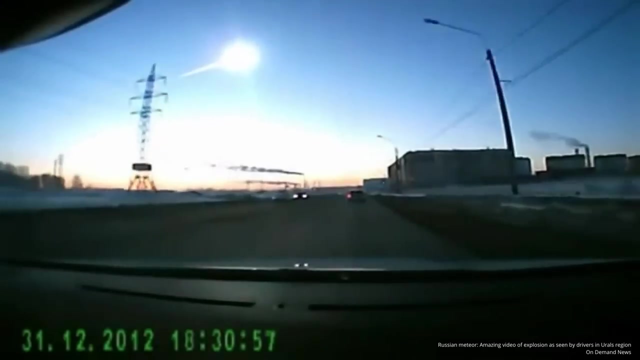 Ideas strongly linked to powerful imagery are more likely to be factored in when making decisions. Case in point: while reading so heavily about dinosaur extinction for this video, I had multiple vivid dreams about asteroids. I had none about volcanoes. In an asteroid-dominated world, the media have had a field day with all-new scare stories. 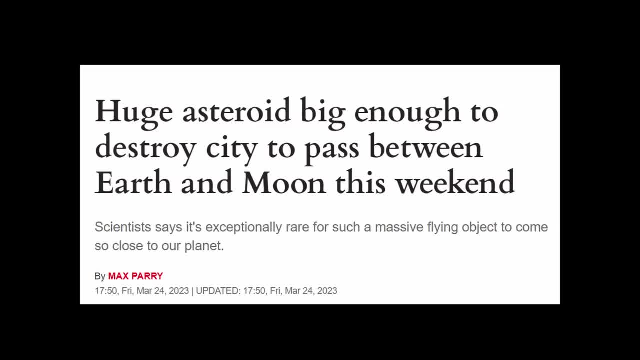 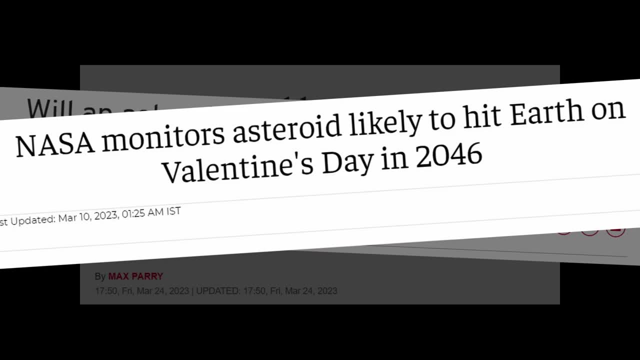 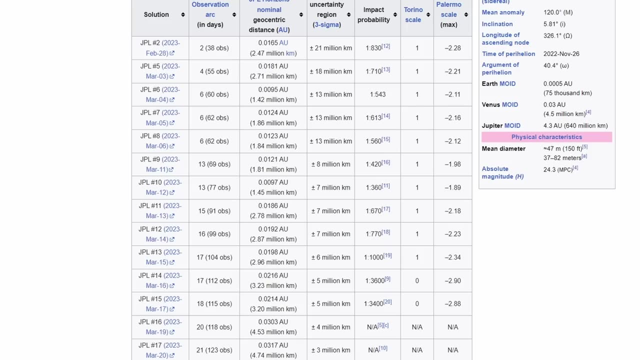 Huge asteroid, big enough to destroy Citi, to pass between Earth and Moon this weekend. Will an asteroid hit Earth in December? and should you be worried? NASA monitors asteroid likely to hit Earth on Valentine's Day 2046.. Sure, if by likely you mean there was a 1 in 500 chance, that's now been significantly. 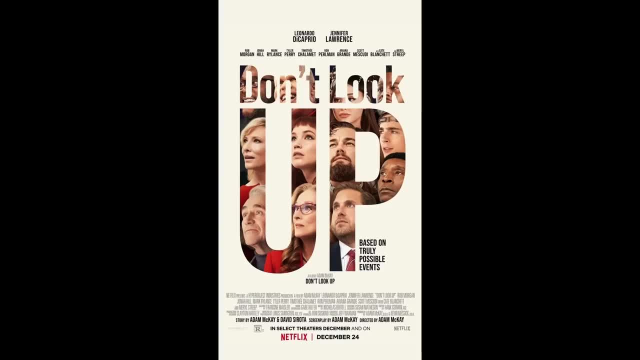 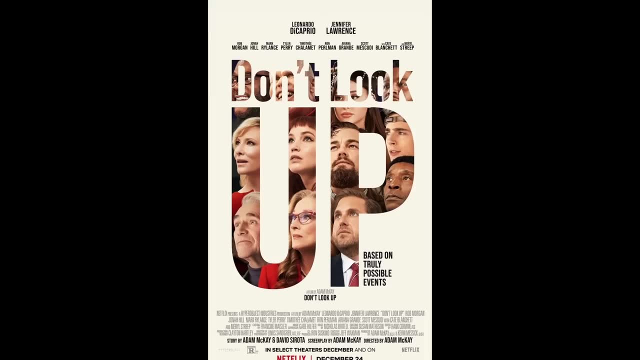 reduced with further observation. I'm not sure. I'm not sure. I'm not sure. We even have media about the media's relationship with asteroids as a metaphor for bad science communication. If that isn't cultural omnipresence, I don't know what is. 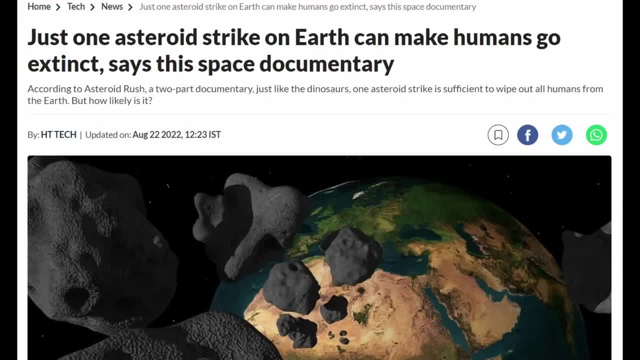 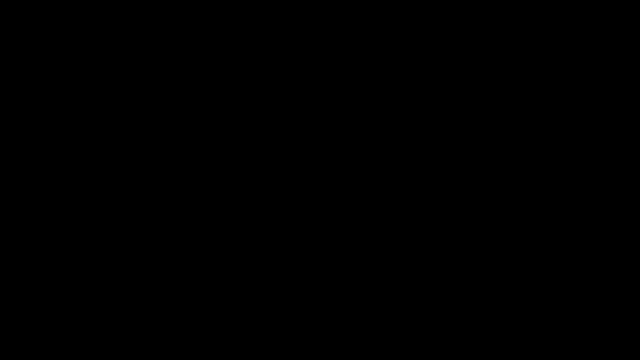 Each example exploits and reinforces our mental bias towards the terrorising deus ex machina. That an asteroid killed the dinosaurs therefore appears obvious. Our final type of harmful news is the breakthrough story Despite and arguably because of the view of the KPG extinction as settled. these are 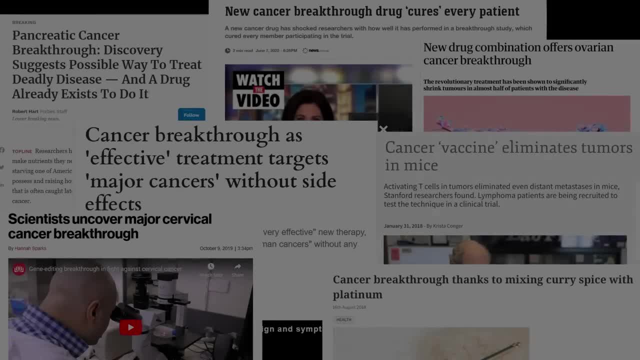 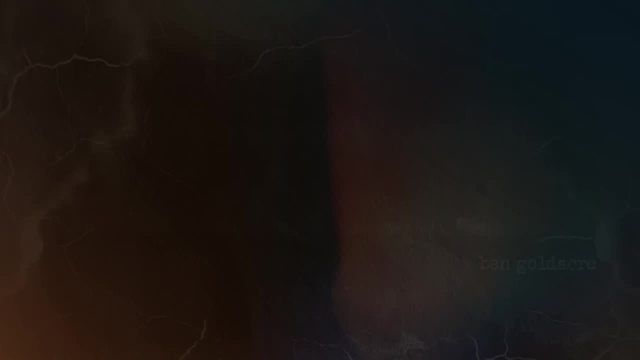 the most disruptive of all. Medicine is awash with breakthrough stories. Given the volume of articles announcing new cures for cancer, how come we haven't cured cancer? Quoting again from Goldacre: If an experimental result is newsworthy, it can often be for the same reasons that it. 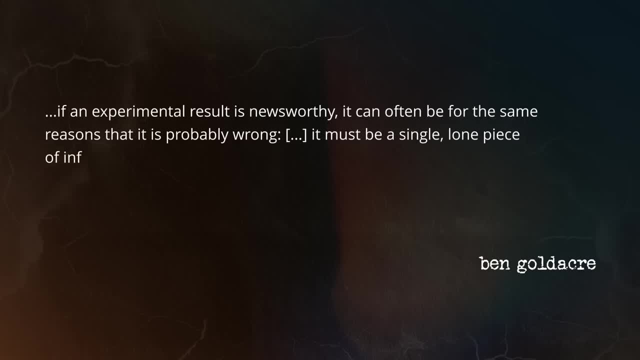 is probably wrong. It must be a single, lone piece of information which contradicts a large amount of pre-existing experimental evidence. Paranoidism: Paradigms exist for a reason, Especially in modern science. every paradigm has proven itself at least useful, if not. 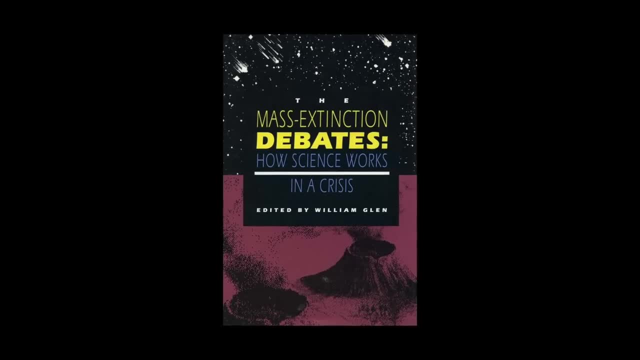 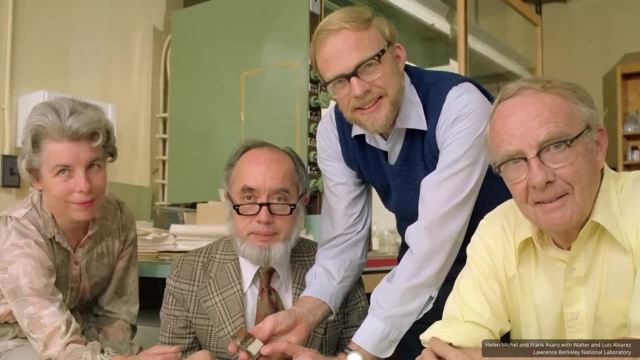 approximately true. Yet the entire focus of mass extinction debates is the danger blind reliance on paradigms poses. Let's not forget how many scientific revolutions have played a part in our story. Even William Smith, right back at the beginning, faced resistance. 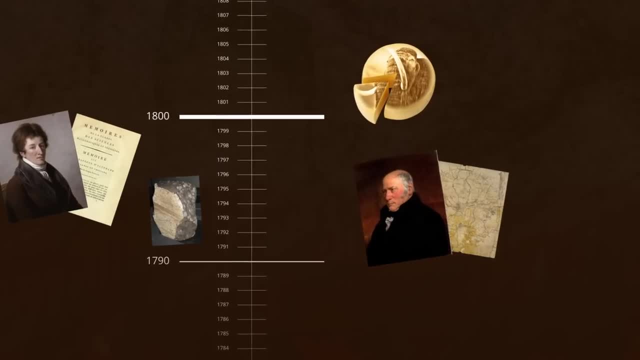 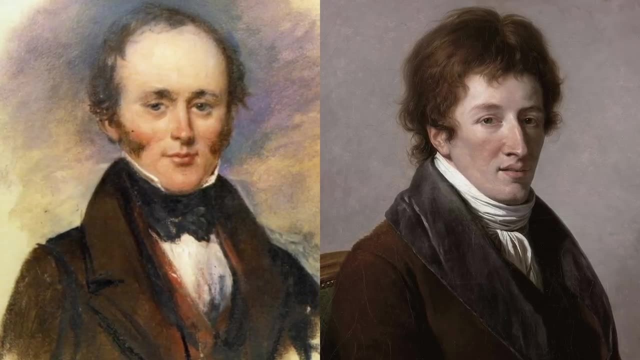 He was ignored, plagiarised and forced into debtor's prison before his ideas were accepted. You could tell by the way he looked at the world. Say we've gone meta and have arrived at the uniformitarianism versus catastrophism debate about science itself. 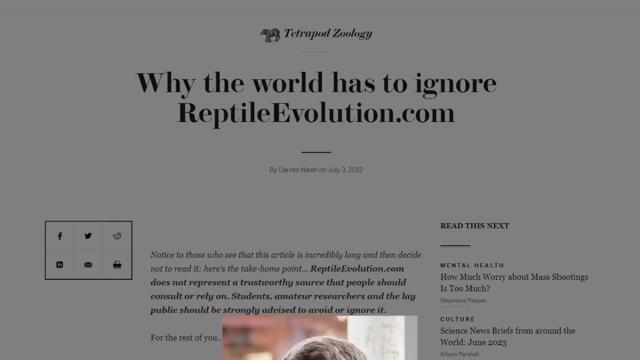 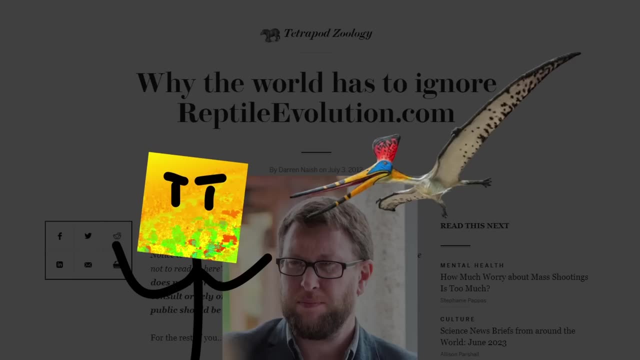 Does science smoulder or explode? I like the way paleontologist Darren Naish resolves it in an article about yet another paleontological paradigm dust-up. No, we don't have time links in the description. The total sum of human knowledge can be imagined as a giant, sprawling baroque castle made. 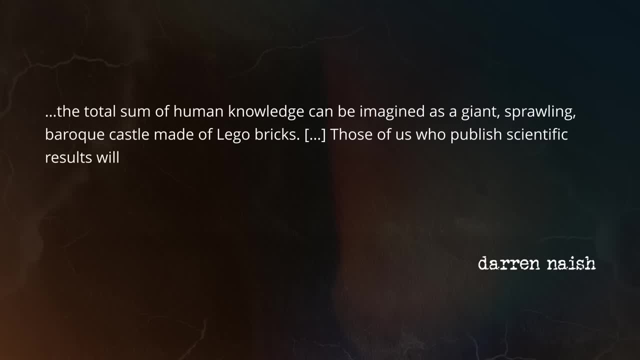 of Lego bricks. Those of us who publish scientific results will, if we're lucky, get to add a few bricks to one of the walls. People who get to demolish an existing wall and construct a wholly new one are rare and special indeed. 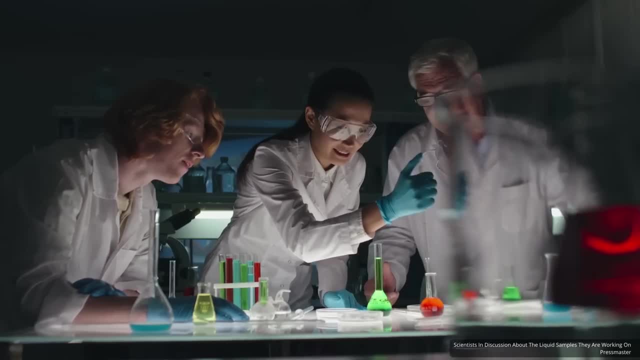 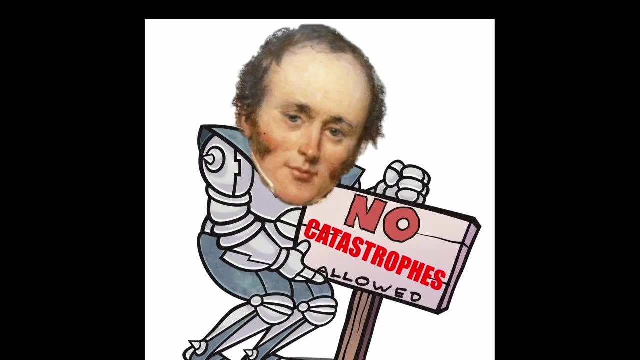 Just as uniformitarianism explains the majority of the past, the majority of scientific progress is gradual, incremental, aligning with established theory. Remarkable upheavals should not be banished. the model says, however, they should be treated with suspicion. 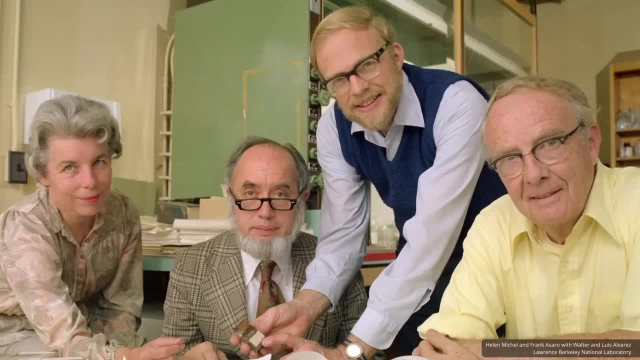 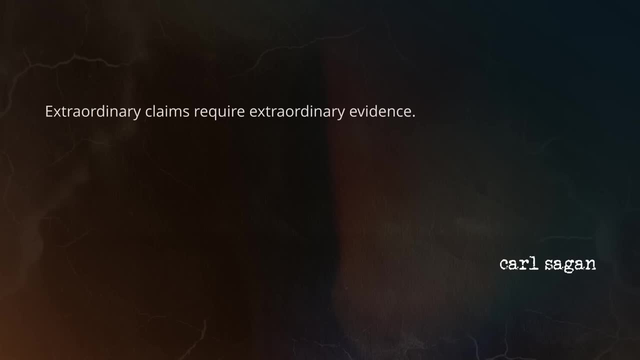 Statistically speaking, anyone claiming to have revolutionised science is most likely wrong. The few who aren't must be treated with suspicion. The most important thing is that they must, as the saying goes, support their extraordinary claims with extraordinary evidence. Spoilers, this quote's gonna get ironic later. 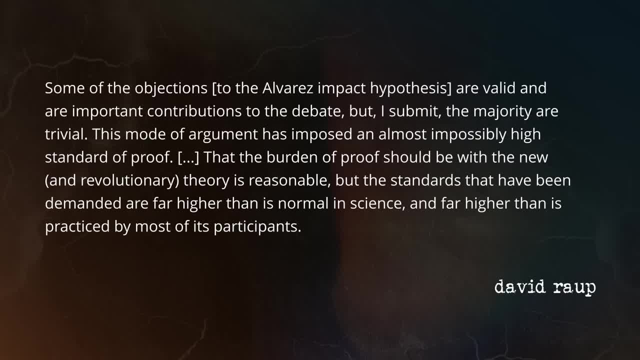 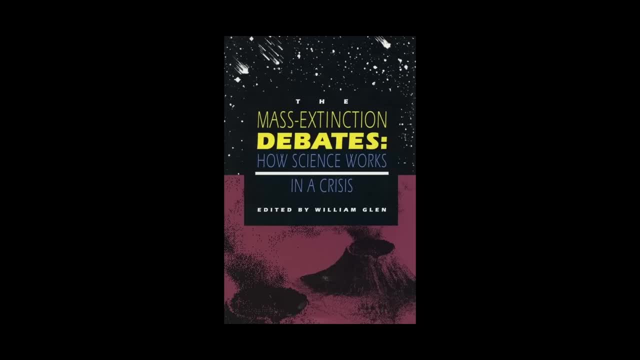 Resistance to impact was justified to begin with. yet many felt the gauntlet set by its opponents went too far. The mass extinction debate is in some sense an examination of paradigms outstaying their welcome by scientific standards, because human standards overruled them. 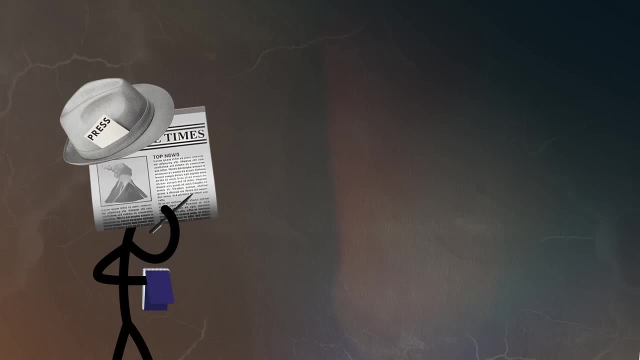 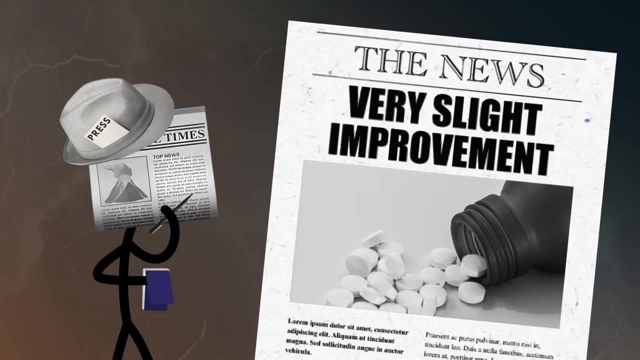 The real trouble comes from tossing the media into the mix. For them, it's a matter of course. Everything must be a breakthrough. Who wants to read about a treatment that's 0.1% better after all? The result is a portrayal of science as temporary, driven by fads. 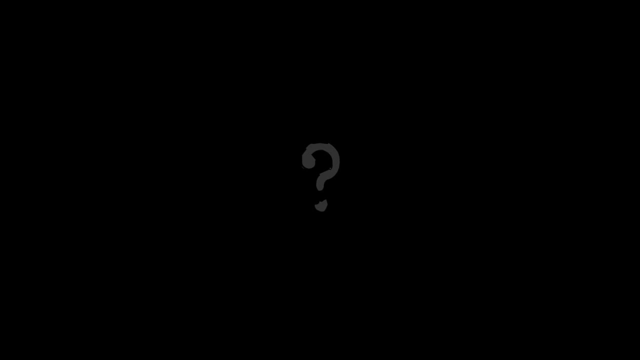 To demonstrate just how difficult this makes life for the layperson, consider two famous theories. Both went against plentiful experimental data, both caused scientific uproar, both were pushed like crazy by the press for their bravery and insight, and today all experts consider. 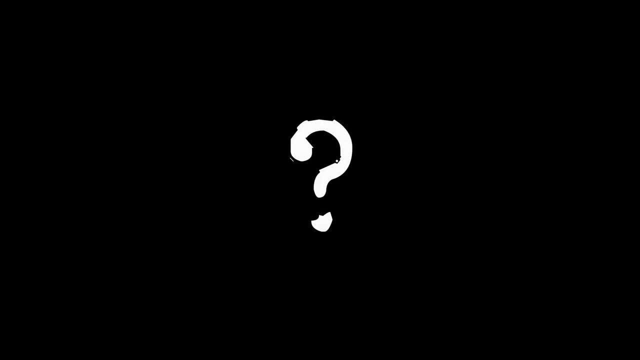 one roughly correct and the other total nonsense. The first is the theory that science is the only source of science. The second is the theory that science is the only source of science. The third is the theory that science is the only source of science. 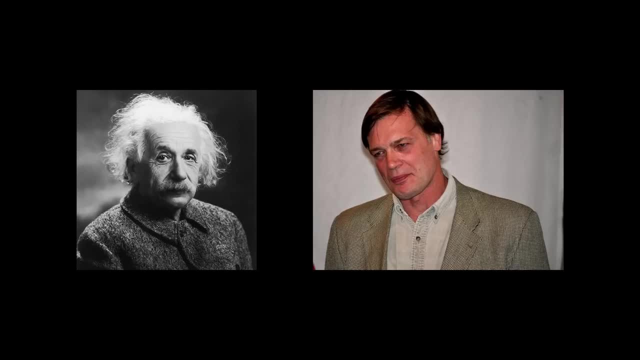 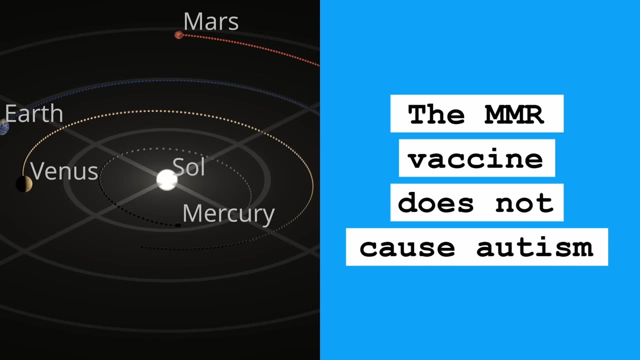 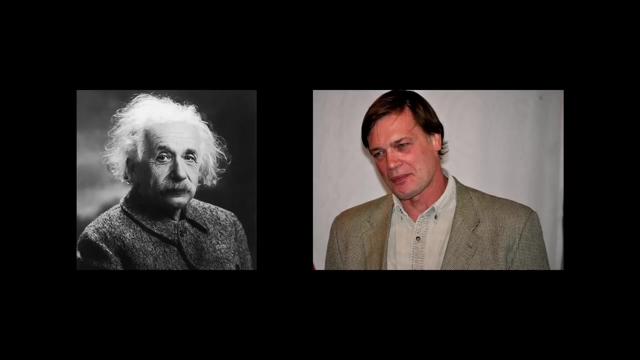 Those theories are Albert Einstein's General Relativity and Andrew Wakefield's MMR vaccine scandal. The difference is that the overwhelming evidence since has vindicated and debunked them respectively. In the moment, though, how could the public tell Who was the righteous maverick the media made them out to be and who wasn't? 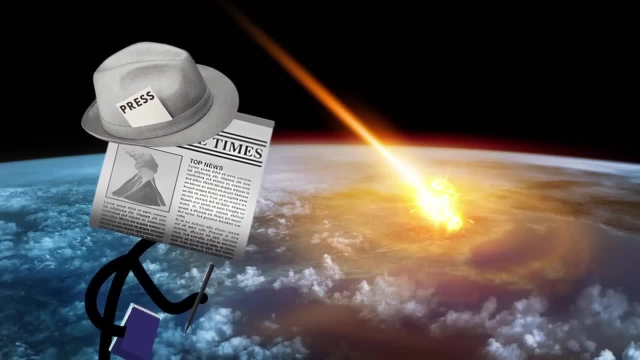 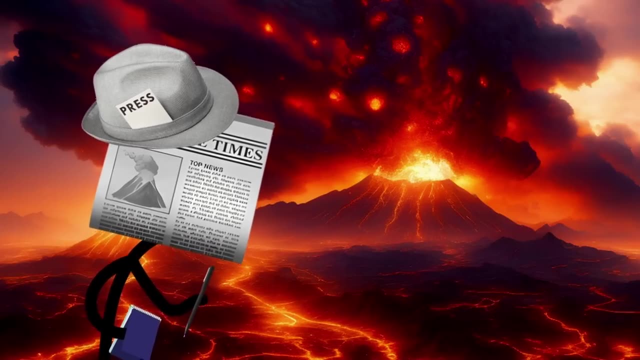 When it comes to KPG, the press had one big bite of the cherry back when impact was the new big thing, and now that that's the entrenched theory, they get to play breakthrough bingo by reviving volcanism. Much of the search for a volcanic extinction since 1991 has been about two things: constraining. 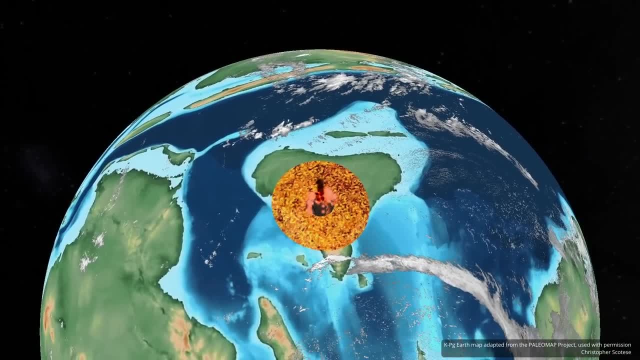 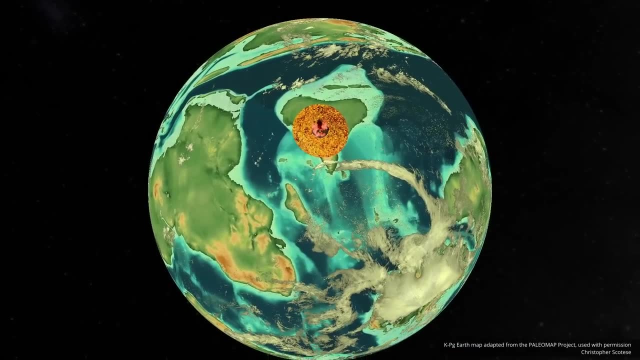 the timeframe of the largest eruption pulses and matching the dates of eruptions to extinctions. If one can show that volcanism was more intense than assumed or that it lines up better with mass extinction, the impact hypothesis should be called into question. 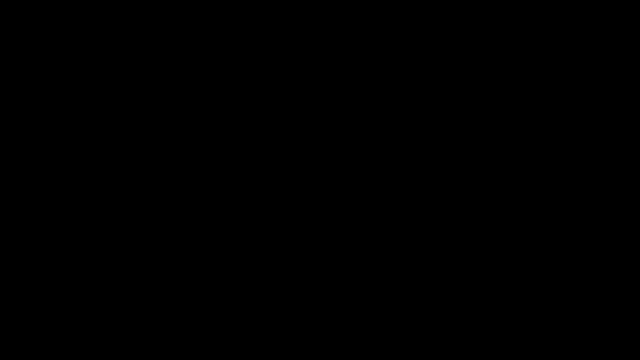 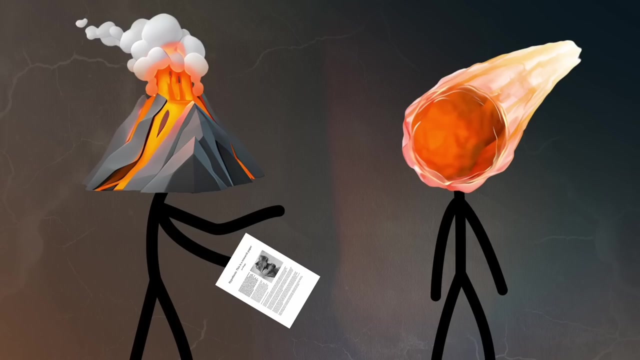 Some studies have claimed steps towards these, but there's been considerable resistance of the type I'm sure you're used to by now. See, We can date this eruption precisely because we found your layer of iridium in the Deccan Traps. 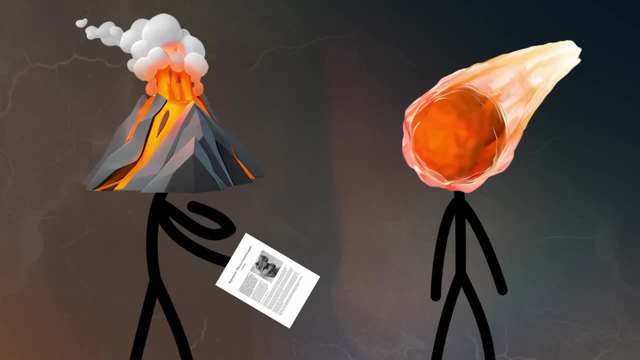 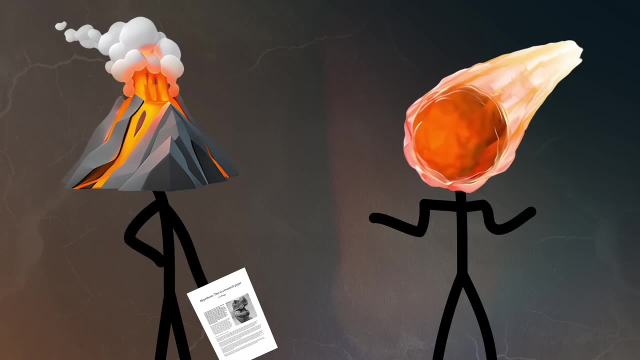 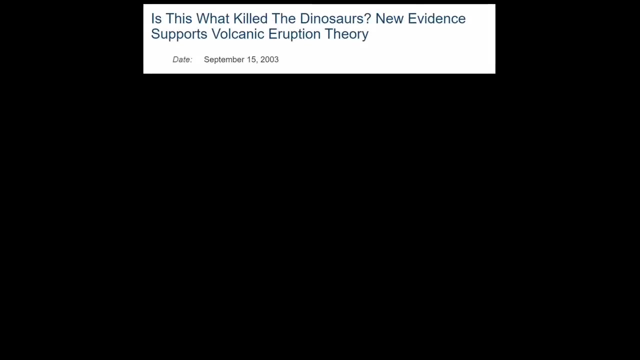 We have an exact relative marker of your impact and my eruption, and my eruption fits the extinction better. Ah yeah, well, you know, maybe that iridium came from the volcanoes. Listen here, you little-. Ask the media, though, and these findings appearing now and then, across 30 years or? 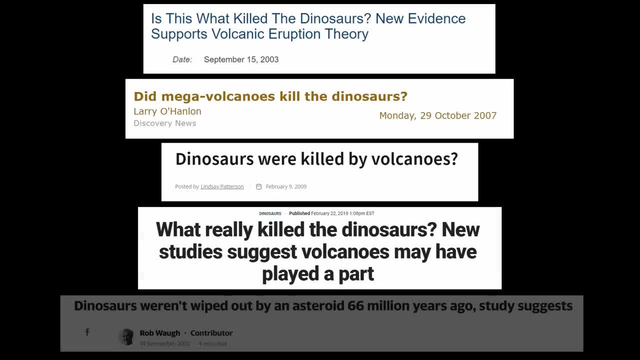 so are all breakthroughs set to challenge a so-far understatement. I don't know what you're going to do about it. I don't know what you're going to do about it. Instead, I've got a very un-challenged impact: dogma. 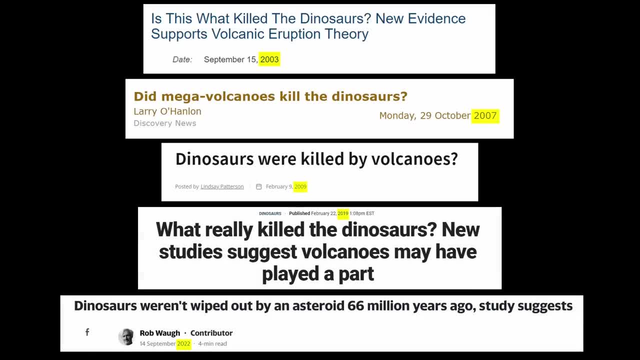 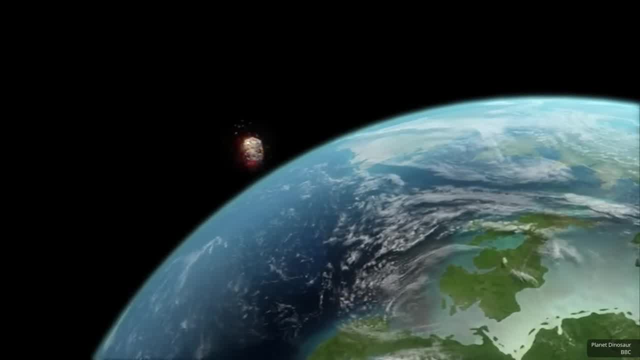 Rarely have I seen a cake so had and eaten. Nonetheless, I can see their logic. I admit that I am emotionally attached to the idea of an asteroid killing the dinosaurs. It's such a poignant story that I would find news of its collapse a challenge to my 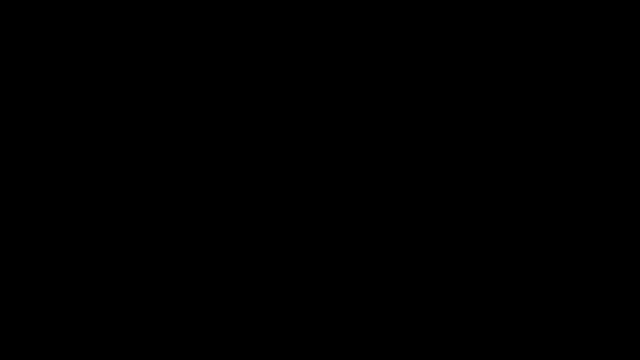 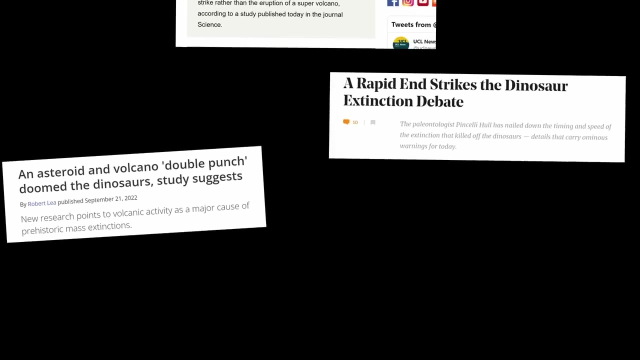 own worldview, hence morbidly irresistible. The media deliciousness of Stories About Asteroids and Stories About Anything But Asteroids has thus created a frankly unhinged flood of contradictory articles around the world. a niżir kök así ki enšköz se hșarăz. 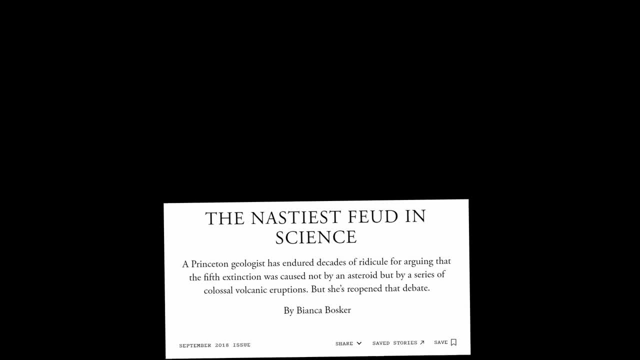 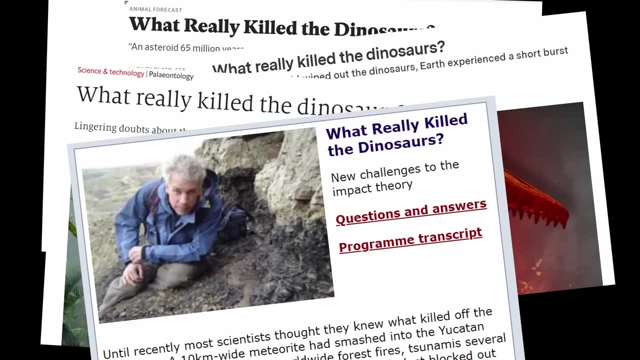 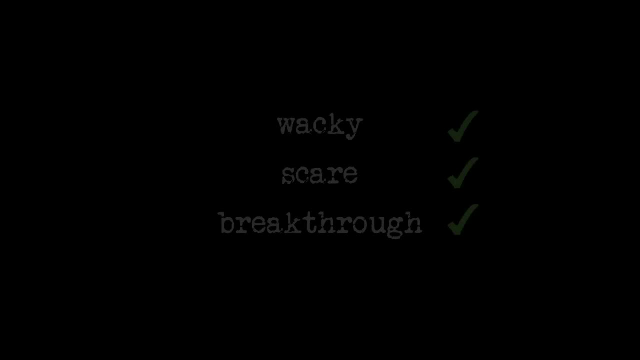 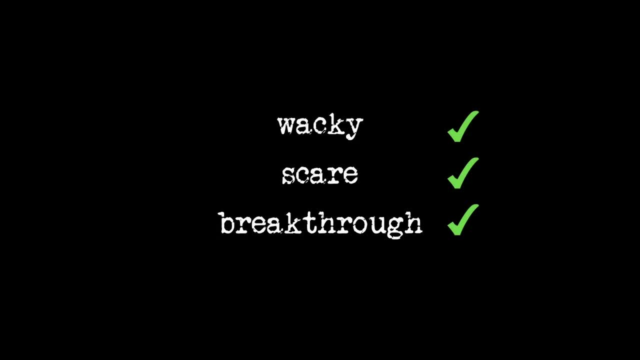 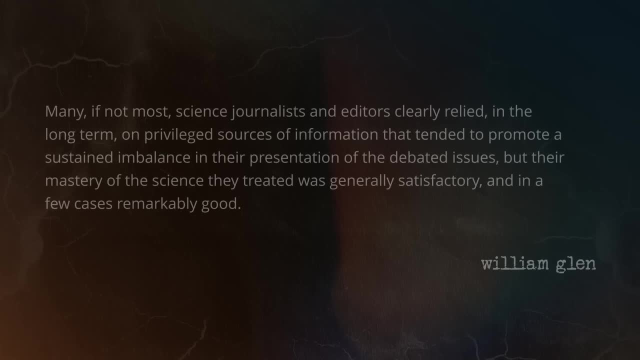 I want to emphasise that I've cherry-picked these examples to be the worst of science communication. As Glenn himself notes, journalists involved in the debates heyday had in general a good to excellent grasp of the underlying science. Their primary foil was inability to cover all the fields involved. 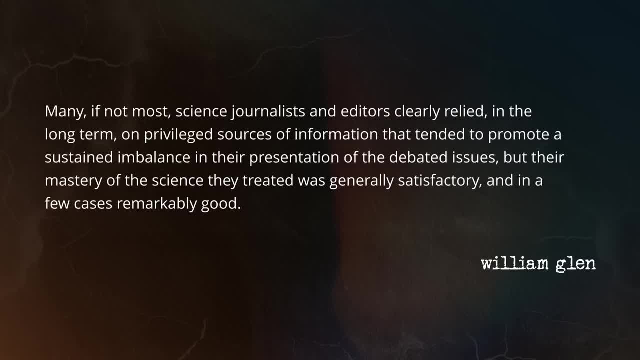 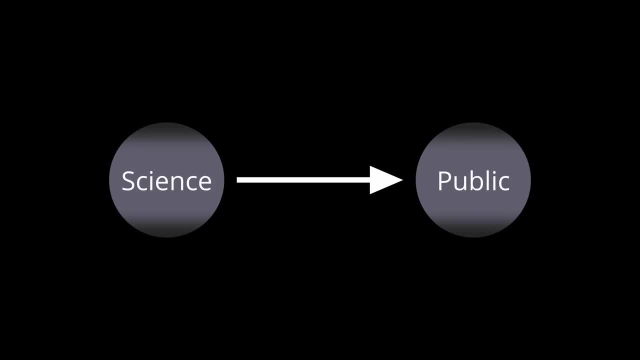 and hence reliance on the loudest voices in each camp. I'd like now to zoom out for a brief overview of the theory of science communication. So far, we've been making implicit assumptions that may not hold up to reality. Is the system always this simple? 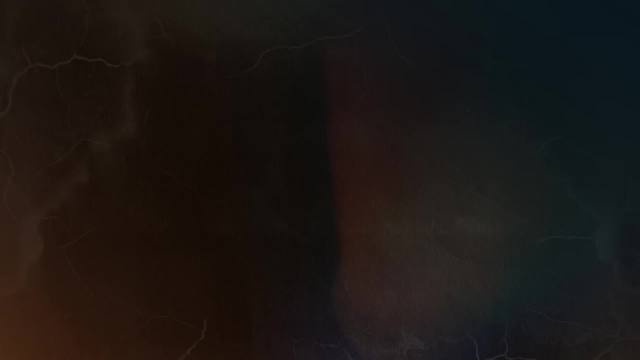 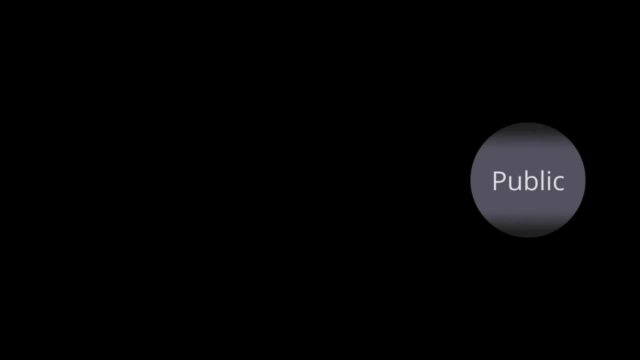 The traditional conception of public communication of science is called the deficit model. Essentially, it states that you're all stupid. The public is assumed to be ignorant at a knowledge deficit. The monolithic blob of raw science is far too complex for them to understand. 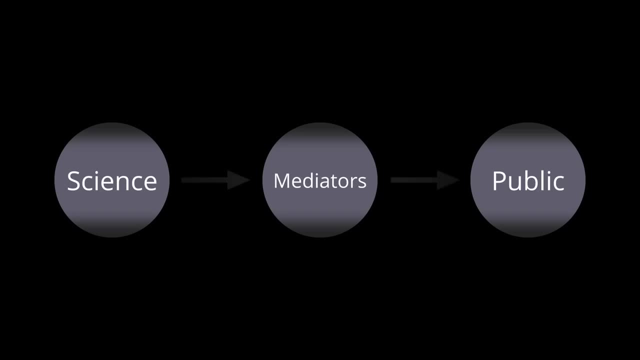 So we need mediators, people whose job is to translate the science into something more palatable. The deficit model measures the success of the communication by how much accurate science the public has retained. Can they recall correct facts with appropriate detail? If they can't, it must be the mediator's fault. 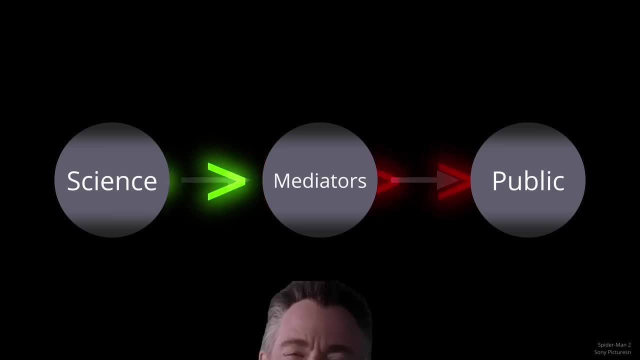 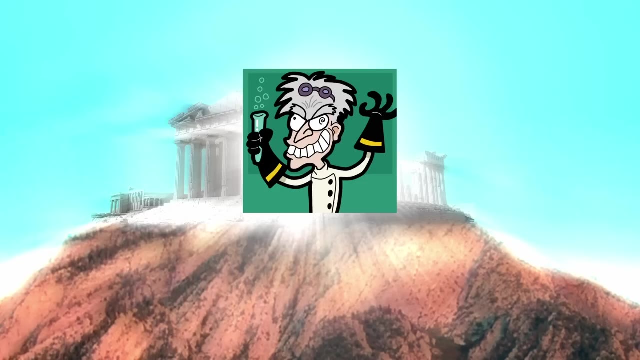 They must have translated it wrong, possibly due to commercial interests muddying the waters. This model legitimizes both scientists and science communicators. Scientists sit apart from the dirty business of communication, free to criticize the media's presentation of their work. They are the source of truth. 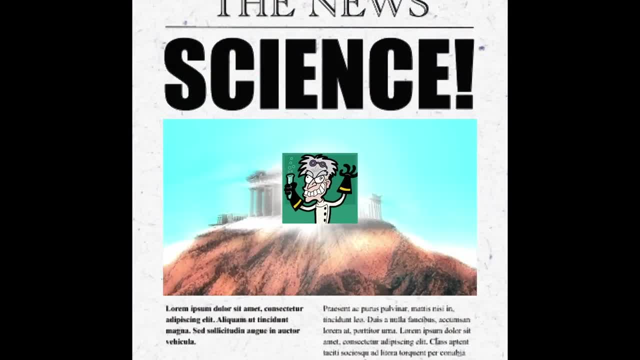 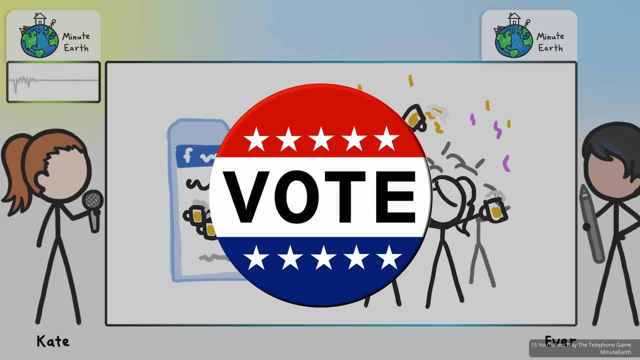 But mediators are also necessary to dumb down the science. Sure, playing Chinese whispers means they get it wrong sometimes, but we all need to know science right. Democracy as an ideology requires an informed voter base. Someone has to teach it to us in terms we understand. 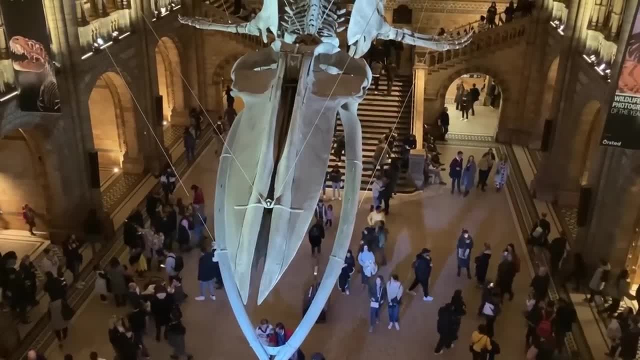 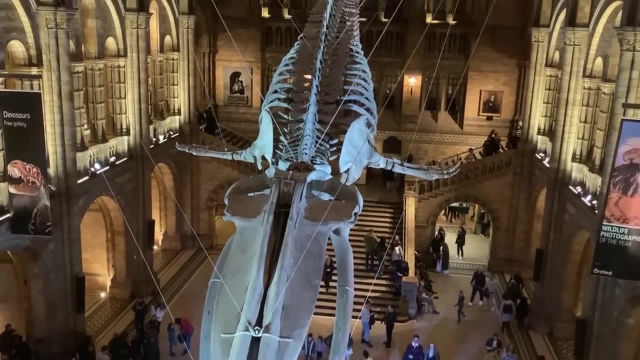 Keep in mind for the rest of the video that science mediation is an industry unto itself. Sometimes the mediators make us forget that they are there at all, hiding the true scale of their role in society. I'm not saying this is a bad thing, but it needs to be remembered more. 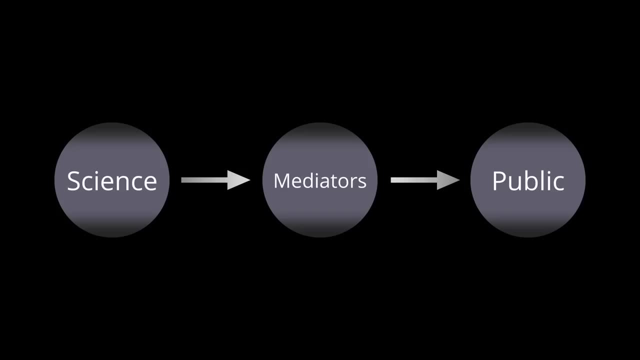 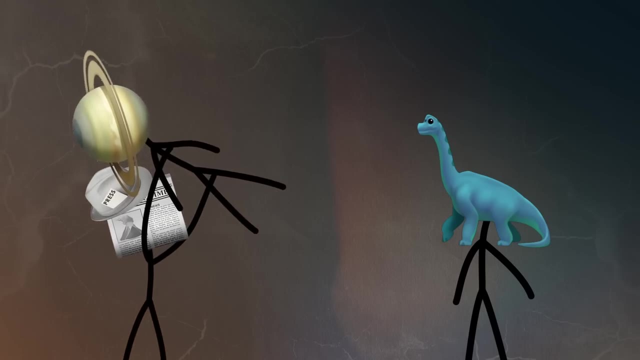 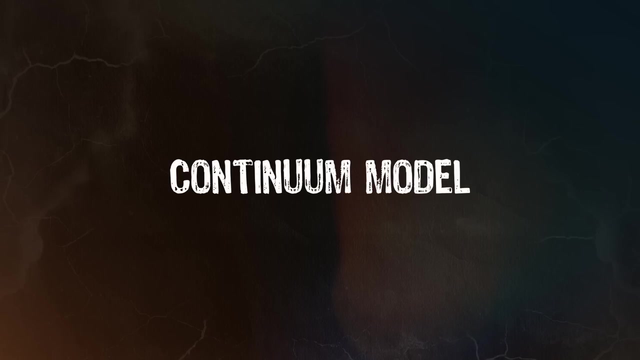 Sometimes the deficit model is perfectly adequate. Science can indeed be a different language, Most of it Greek, But we've already seen examples where this simple linear flow doesn't explain scientific dynamics. A competing construction is the continuum model, Perhaps science and science mediators, as terms are too vague. 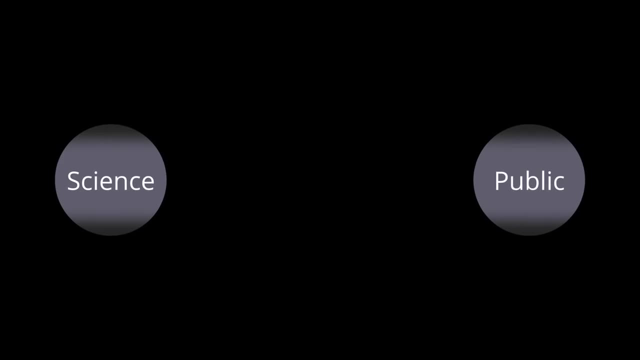 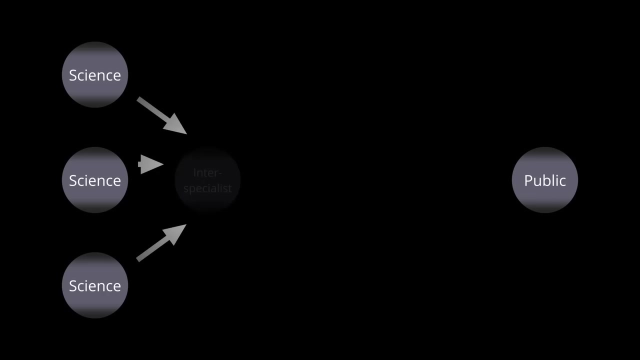 Perhaps information flows in more than one direction. Perhaps we should rework the deficit model into a full ecosystem with several stages and two-way dialogues at interfaces. First disconnected fields at the cutting edge of science exchange ideas within themselves, and these ideas are ultimately adapted for an inter-specialist stage once better supported. 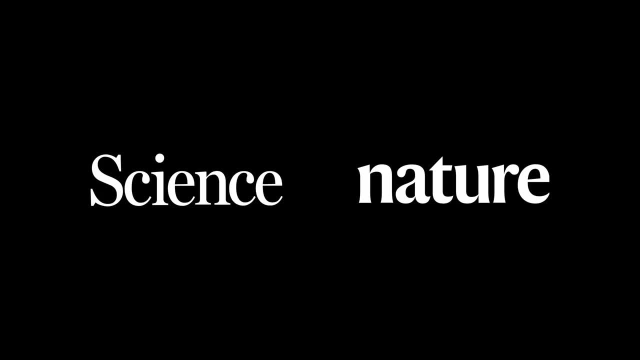 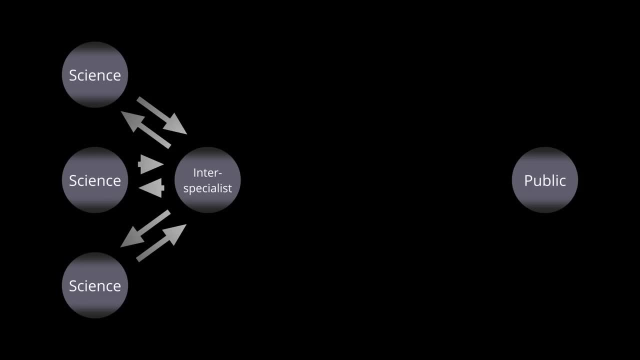 These are your interdisciplinary journals: Science, nature, so on. Scientists can then consult such journals to learn about developments outside their area of expertise. Beyond that, the pedagogic level adapts content for education and textbooks, and the popular level adapts these for mass appeal. 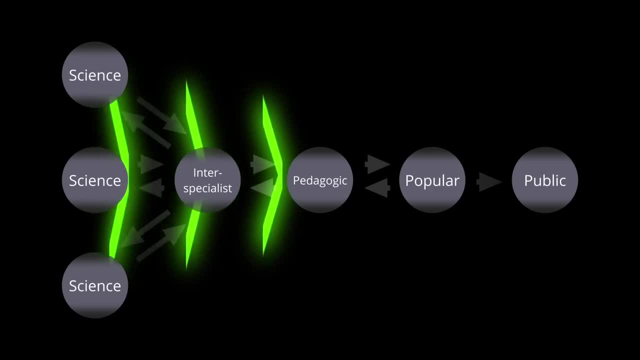 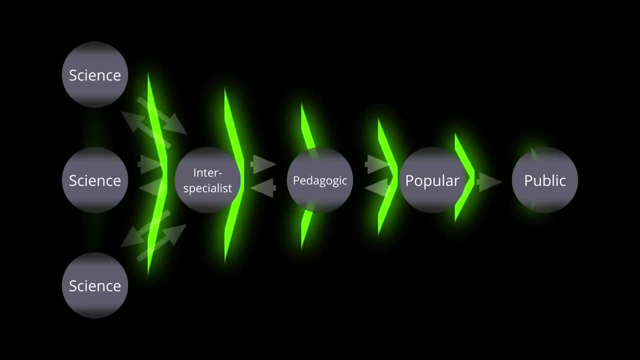 The whole structure ends up acting like a funnel, removing subtleties and adding perceptual certainty the further along you go. The ideology of the continuum model is that this is how good science should work. Ideas are only solidified in public view once they've passed through layers of scrutiny. 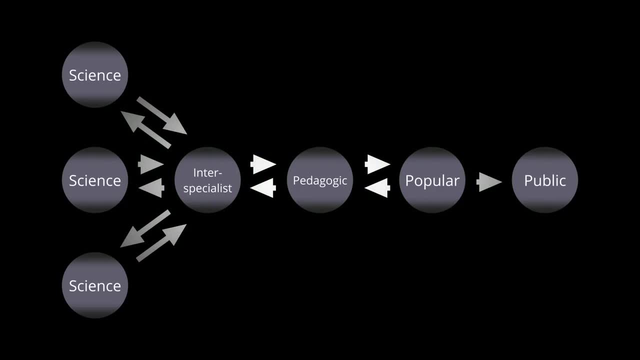 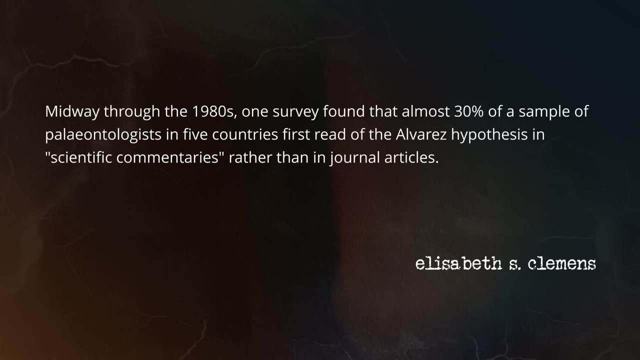 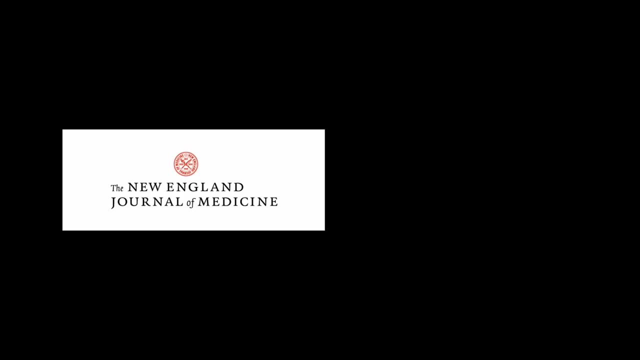 But this model does acknowledge that exceptions exist. First, popular science wraps right back round to influence specialists. You know that 30% statistic from earlier. Another oft-cited study found a paper published in the New England Journal of Medicine is three times more likely to be referenced in other papers if it's mentioned in the New York Times. 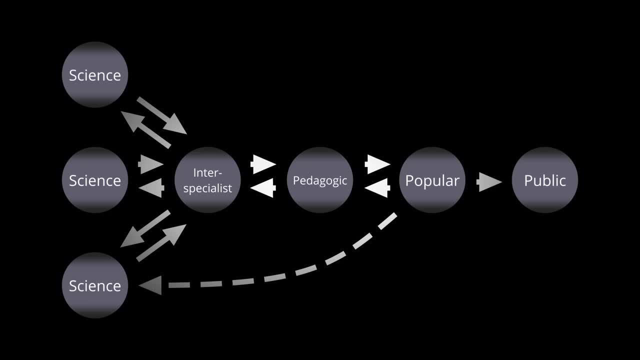 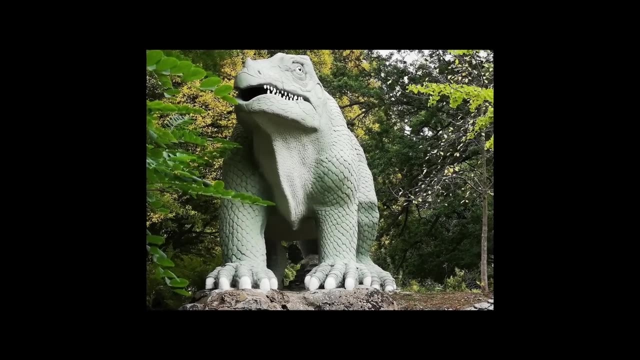 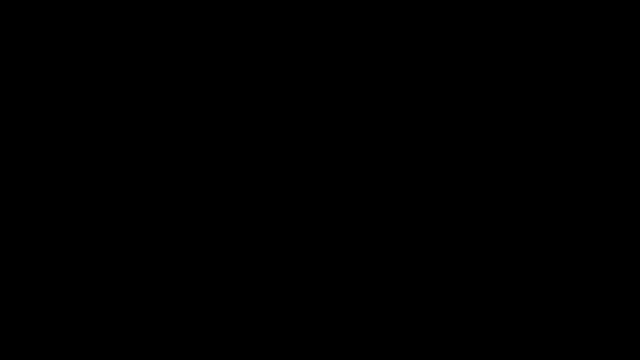 Scientists do rely on the popular press. It's also possible for information to skip one or more levels. The continuum model enforces inherent scepticism towards such deviations. They fly in the face of how science should be done and so aren't to be trusted. 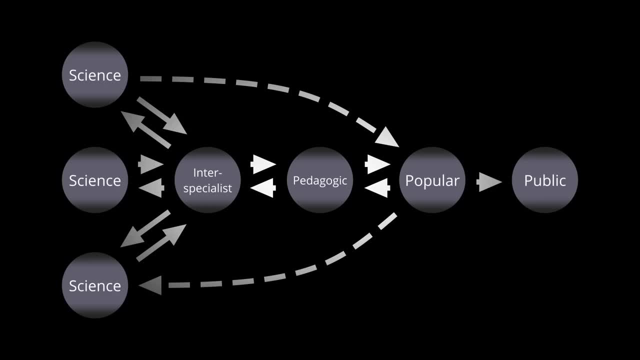 Because of that, link from popular back to specialist deviations can be viewed as scientists' attempts to unfairly influence scientific opinion in their favour Or, if you're so inclined, scams. The continuum model is certainly more complex than the deficit model, But even this is not always the full picture. 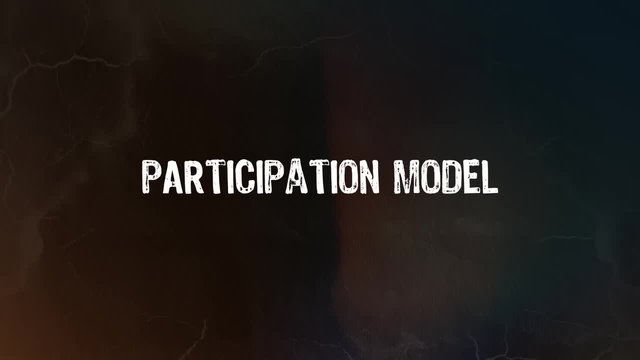 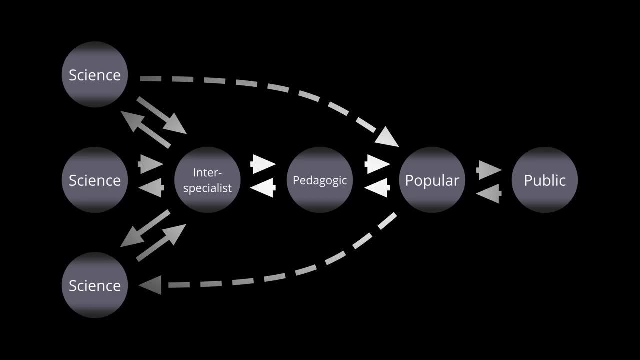 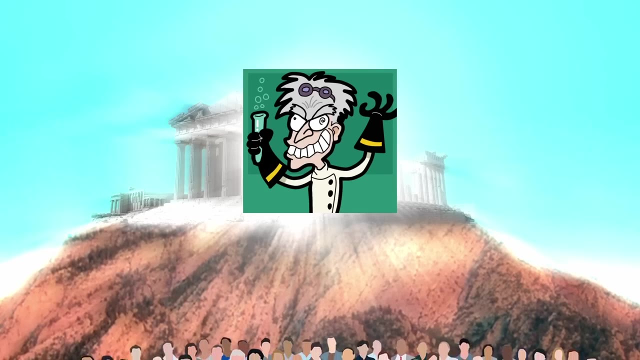 Another alternative is the participation model. The participation model challenges two fundamental assumptions: That the public can only be receivers of scientific agenda and that science communication is all just basic knowledge transfer. Rather than separating scientists from the discourse, the participation model holds that the public can and should take an active role. 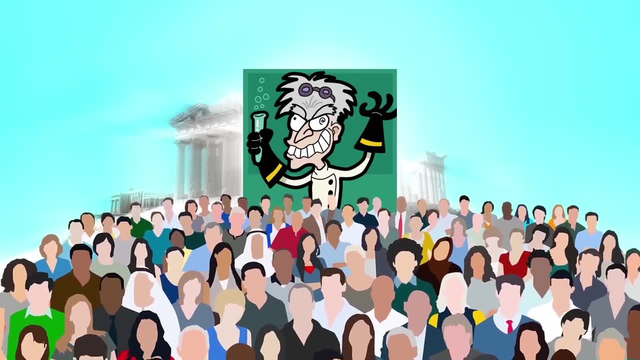 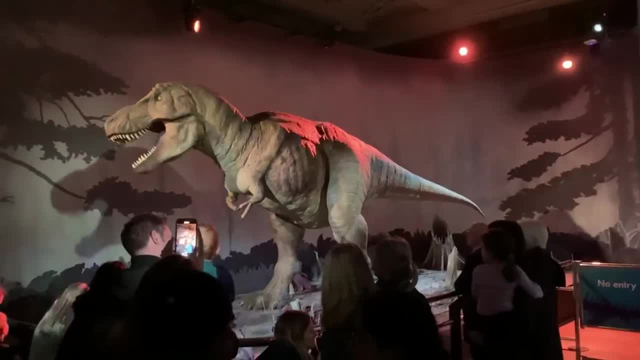 in shaping science, its goals and its communication methods. What do you think killed the dinosaurs? Leave your answer down below. You know that kind of thing. Museums, for instance, have transformed in the past few decades. Less emphasis on the future. 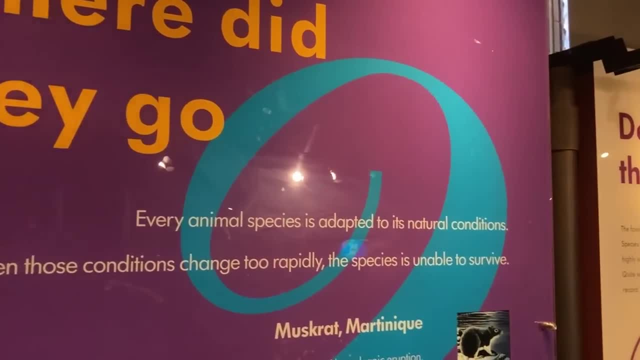 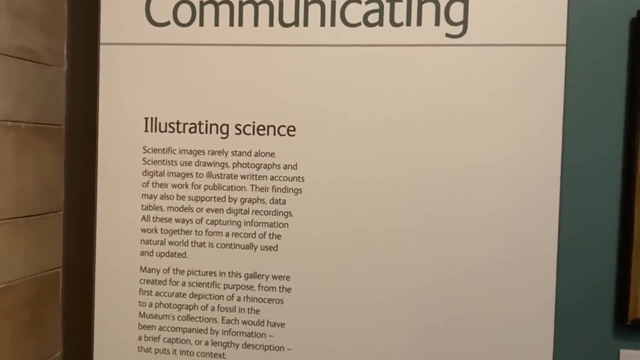 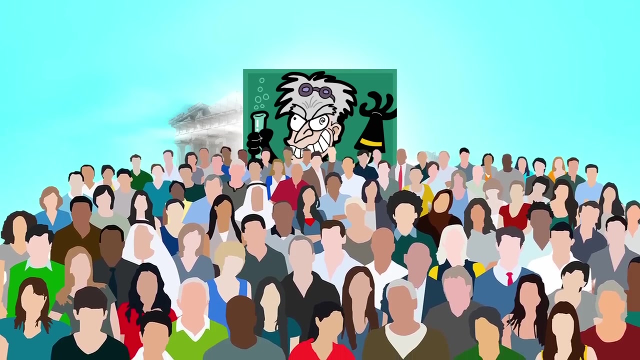 Less emphasis on static pedagogic displays And more on interactivity, Asking questions, Adding ethical context, Putting the visitors first, Putting their ethical desires about science centre stage, Putting Richard Owen up in the rafters- One side effect of this collapse of the ivory tower. 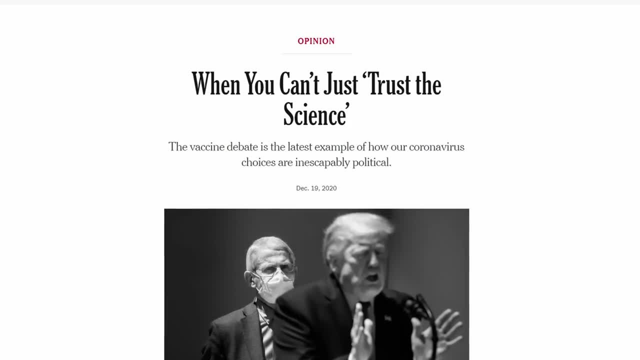 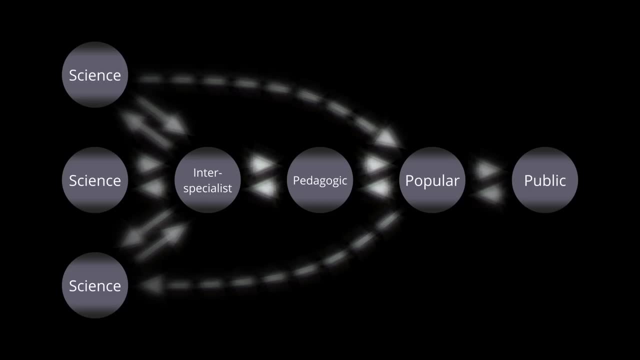 is that both press and public can call scientific institutions into question, In some cases leading to disillusionment and reduced trust in science as a philosophy. Balancing the need for public involvement against a Dunning-Kruger-driven I-know-better-than-the-scientists hellscape. 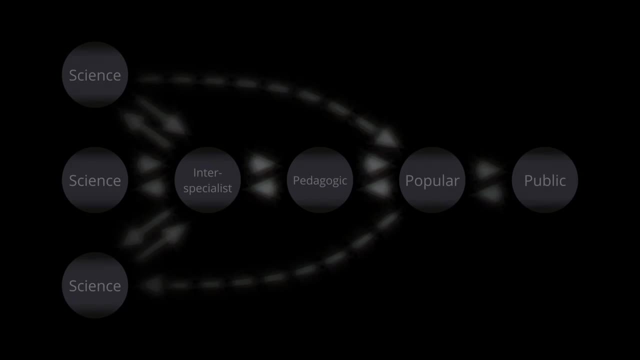 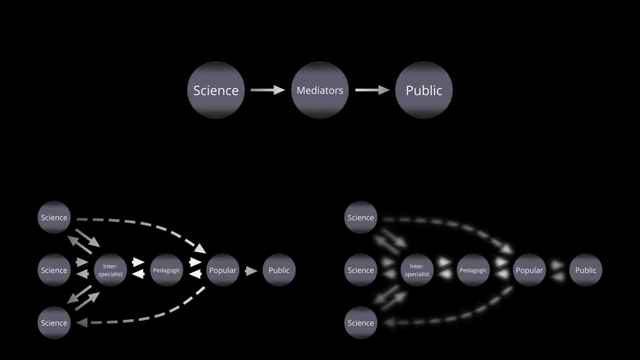 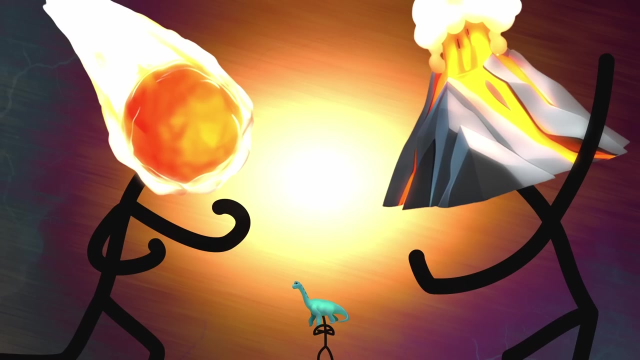 is the participation model's greatest challenge. While trends have shifted, all three communication models remain popular, applicable to many different examples. Sometimes a deficit approach will do, Sometimes it really won't. Humans are not neat models. Even scientists are biased entities with limited time to assess the full picture. 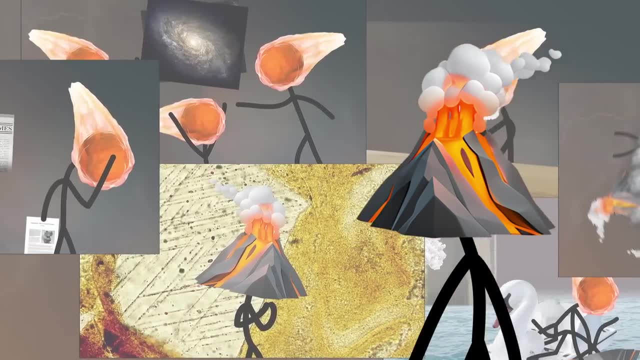 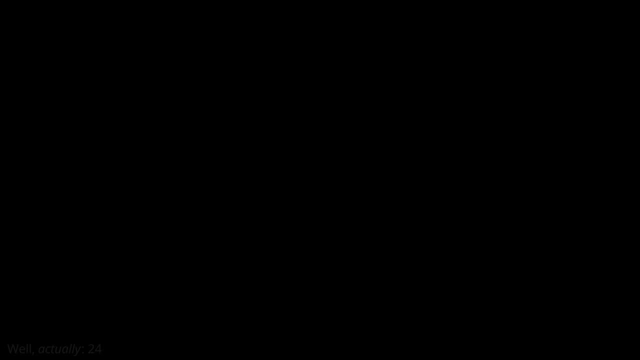 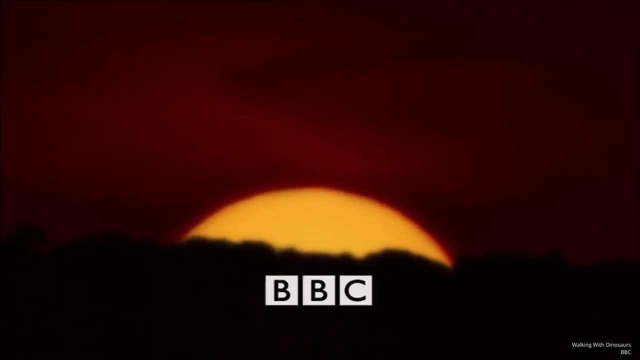 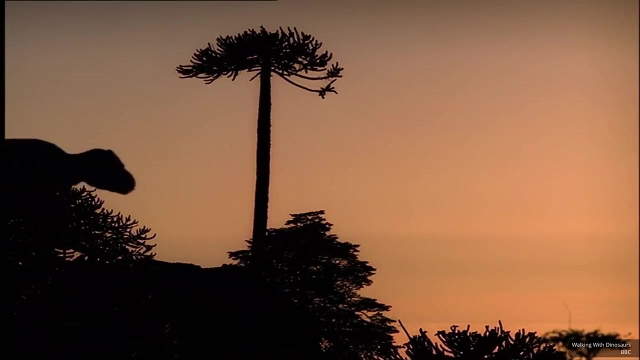 The non-linear ecosystem that emerges is contradictory, maybe a little bleak and a hell of a lot more complicated than most of you probably thought. Anyway, can we talk about dinosaurs again? Ah, there we go, Riding the coattails of Jurassic Park. 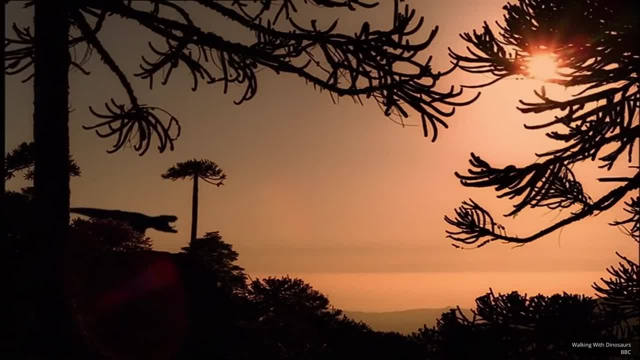 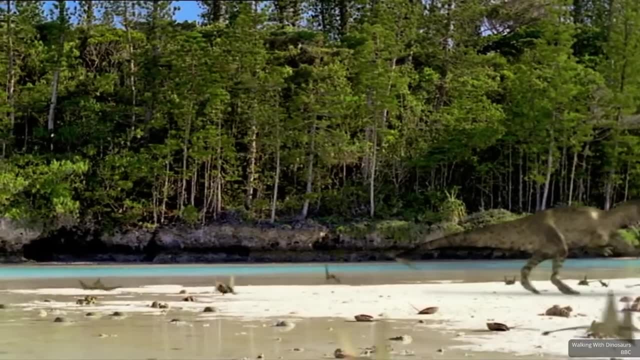 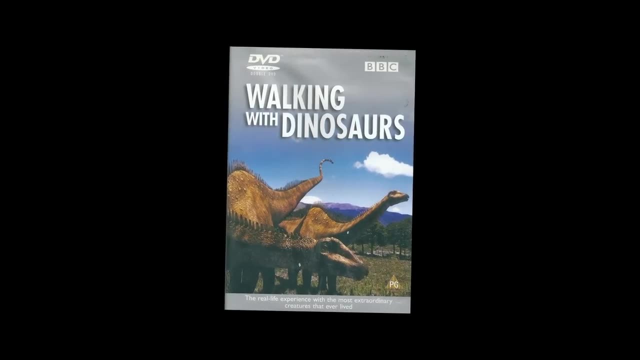 Walking with Dinosaurs arrived on the scene in 1999.. Unlike Jurassic Park's overt entertainment slant, this was a documentary- At the time, the most expensive documentary series ever made. Walking with Dinosaurs ushered in an era of dinosaur science for everyone. 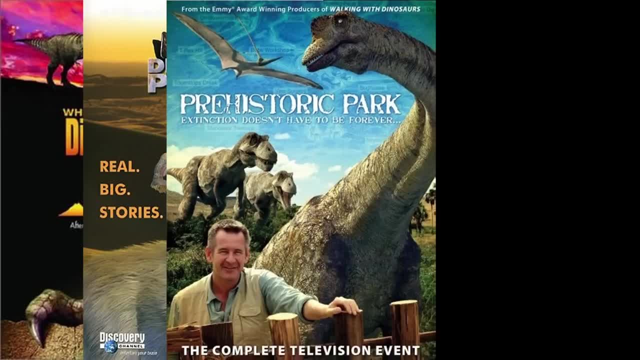 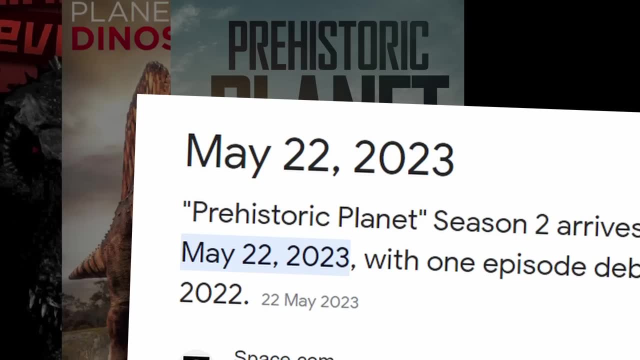 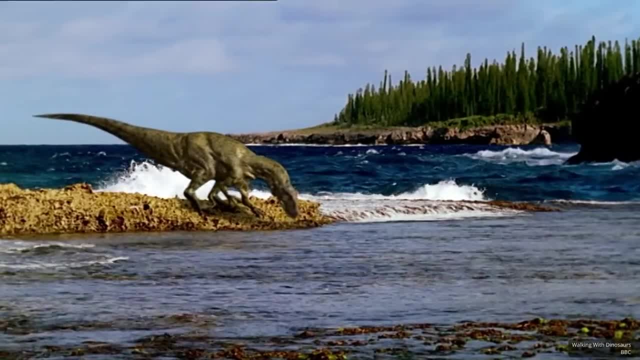 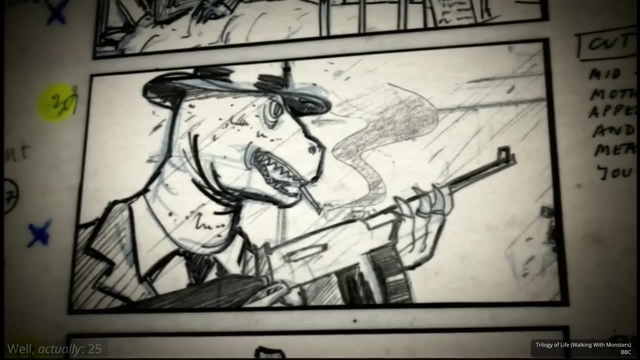 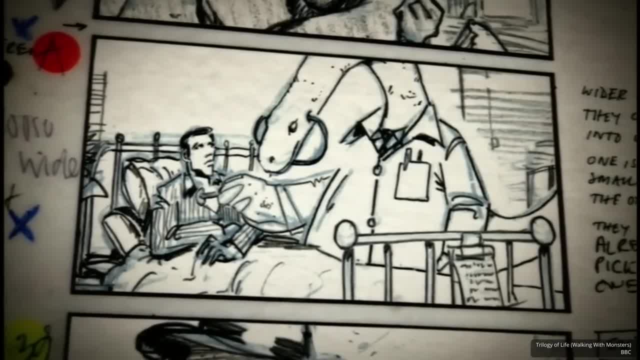 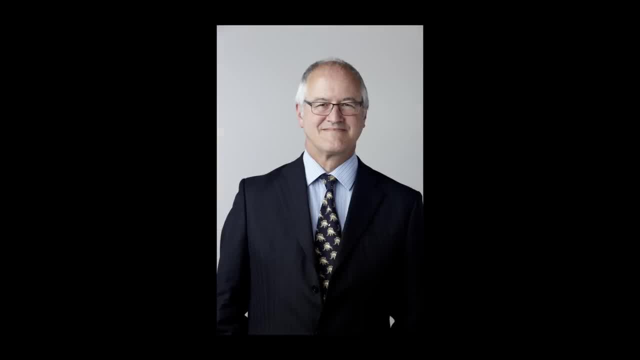 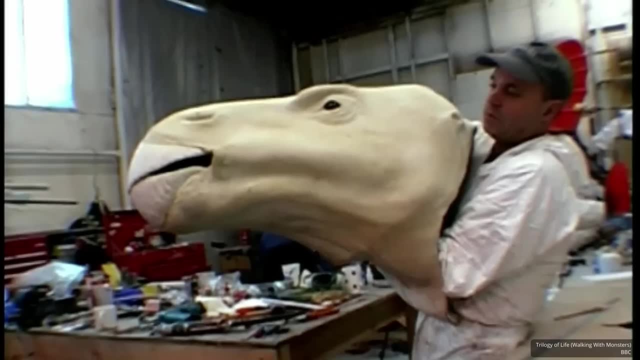 Science and entertainment are both integral to its DNA. So too are fact and speculation. In the words of its primary paleontological consultant, Michael Benton, Science is about hypothesis testing and making an hypothesis is speculation. Artists, animators and puppeteers all contributed to the science as much as they drew from it. 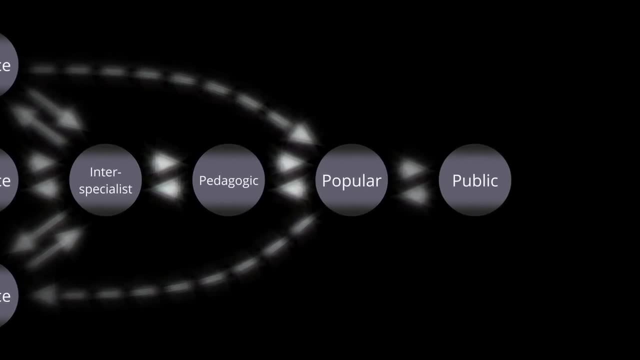 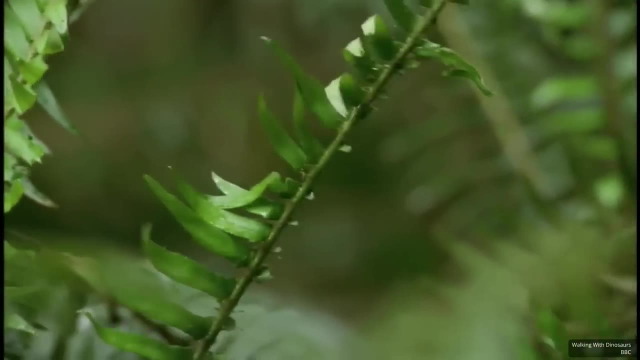 Bringing prehistory to life in a public-centric context demanded they ask new questions and inspire new inquiry. As one example, while operating fake Diplodocus heads, puppeteers discovered they needed to move in an unexpected way to strip leaves, initiating a new scientific 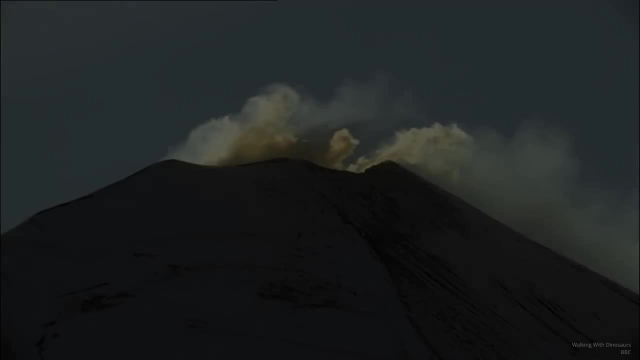 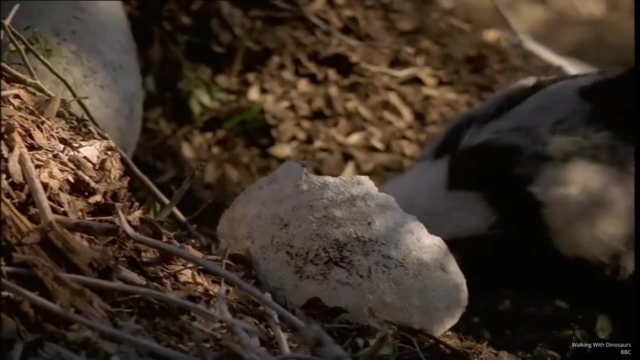 dialogue from the public space. Watching the final episode back, I was surprised to see volcanism so strongly linked to the dinosaurs' decline. Egg-stealing mammals also get a look-in, But it's still the asteroid, the deus ex machina, that gets all the narrative fanfare. 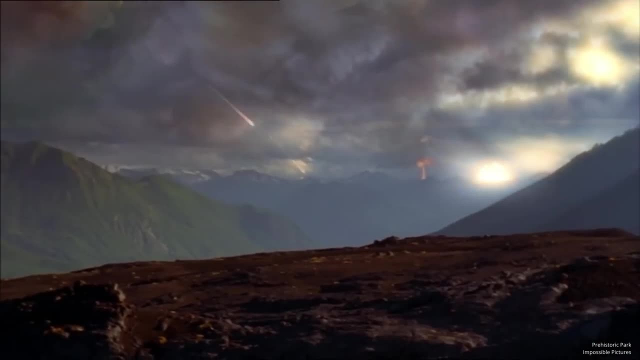 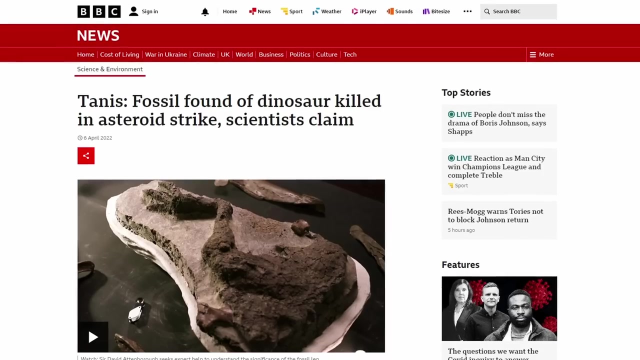 Same old story, the story generations of documentaries have rendered in CGI. Action films are one thing, but if it's on factual TV, there's even more reason to believe it right? Only last year, headlines exploded with the discovery of a fantastically well-preserved 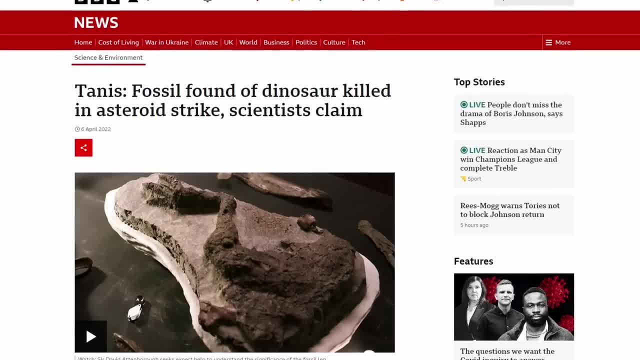 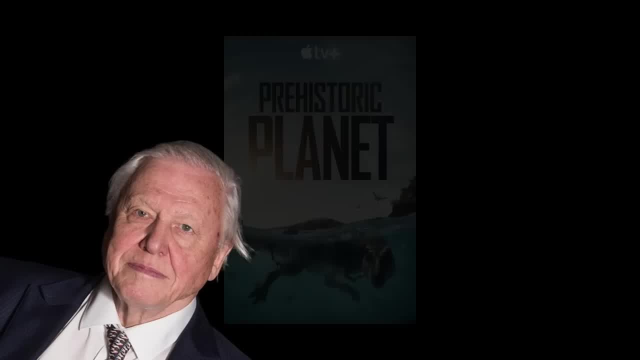 leg from a dinosaur that could have died on the very day of impact. Several lines of evidence suggest it was buried in a tsunami and there's impact ejector nearby. With the help of a David Attenborough Helms documentary- no, the other one, the team pulled. 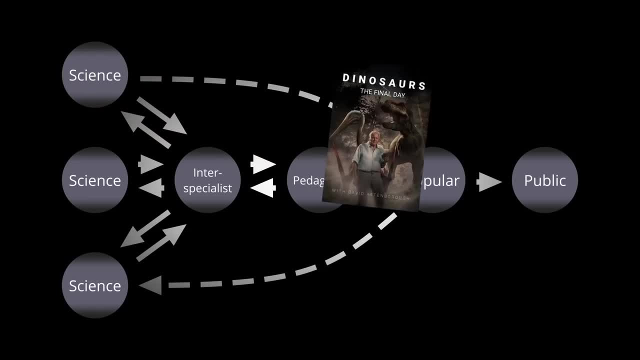 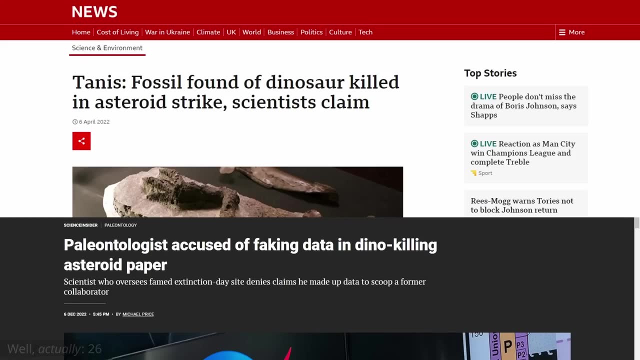 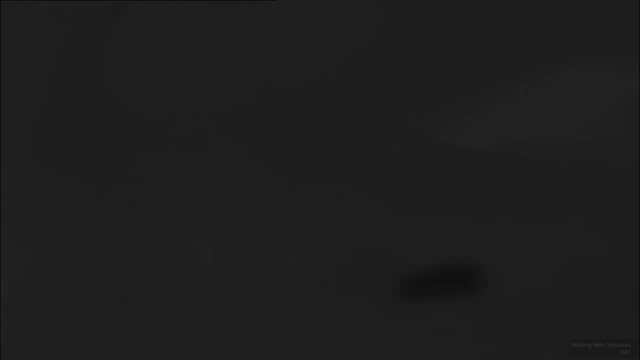 a sneaky on us and put it in our heads before the peer-review process had completed. So, despite its grand claims, this conclusion is so far provisional. The million-dollar question, then, is: do these documentaries reflect modern expert consensus Outside of the contrarian volcanists' continuing struggle for recognition? 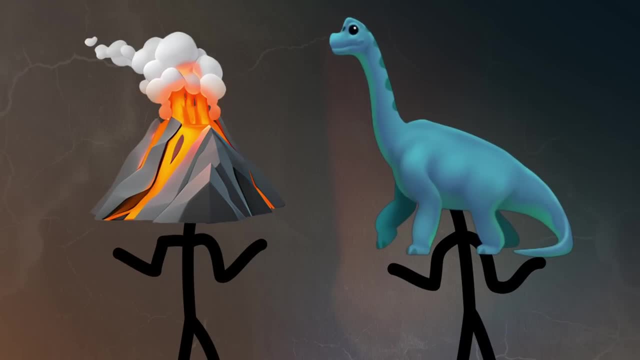 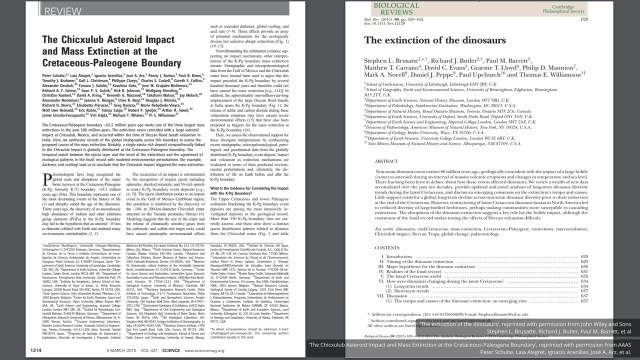 and surprisingly still one or two OG uniformitarians out there. the debate over the KPG extinction in specialist levels has moved on. The fire of the debates may have abated, but the passion of those seeking evidence has not. It's not just the mummified leg. 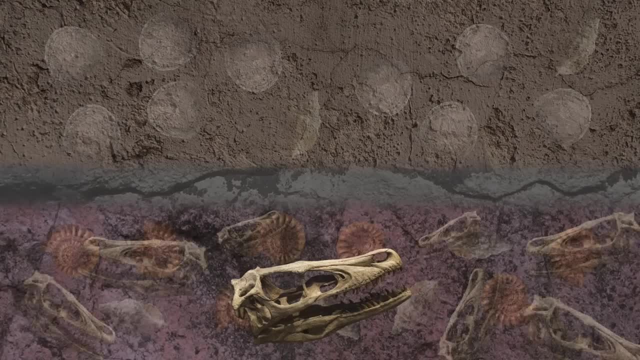 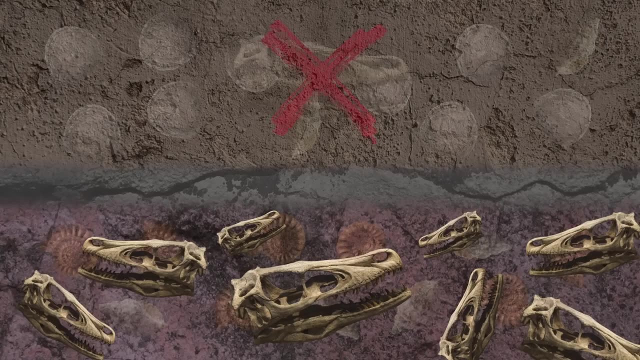 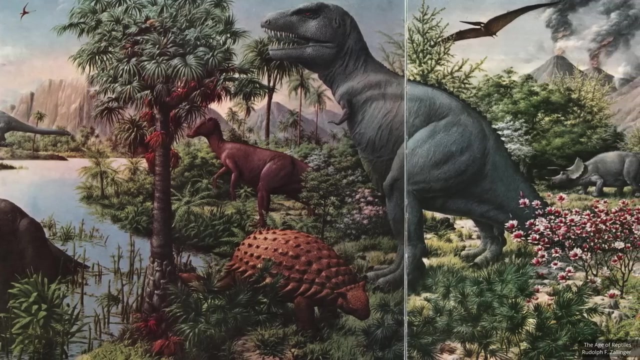 Fossils today are being discovered faster than ever before, filling in gaps and narrowing boundaries, Combined with improved radiometric dating, chemical analysis and modern statistics- all evidence that's widely supported points. the same way, These days the question isn't so much: did an asteroid kill the dinosaurs? 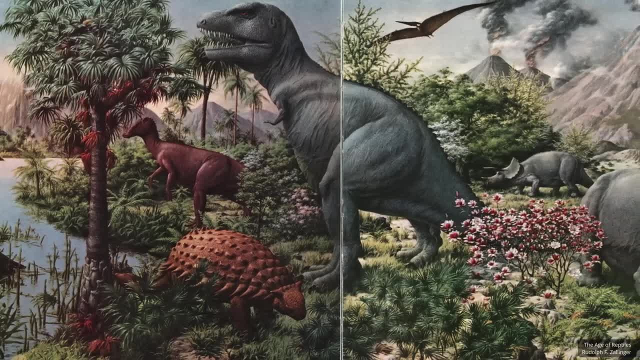 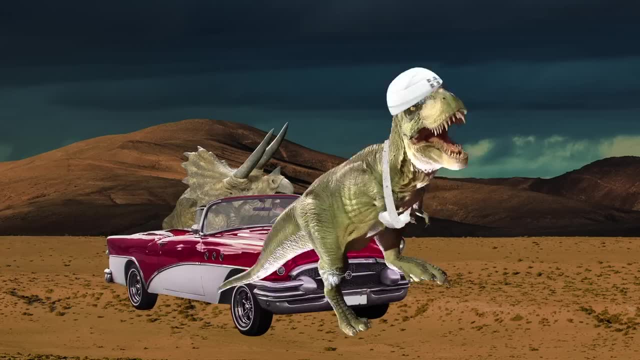 as would dinosaurs have died soon anyway, even without an asteroid, Were they already in decline? Although, let's face it, if you have a long-term ailment but get hit by a car, the coroner's going to put car on the death certificate. 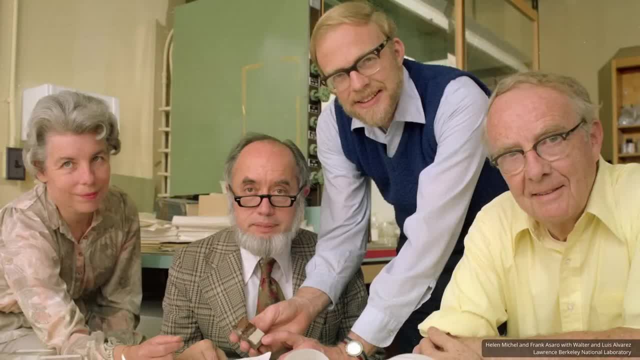 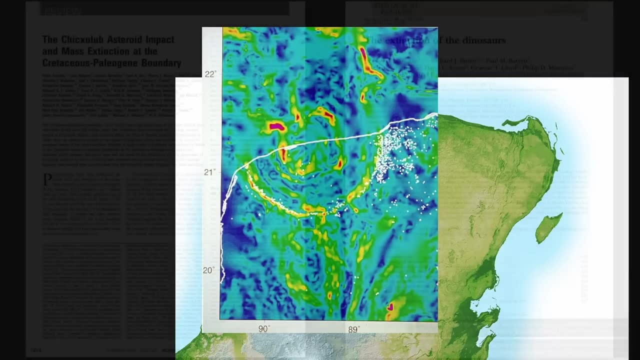 Though they arrived as mavericks amid a media frenzy, Alvarez Alvarez, Asaro and Michael met the chance. The crater silenced all doubts about the physical impact, and multiple reviews of recent years, based on a wealth of evidence, name it as the primary driver of extinction. 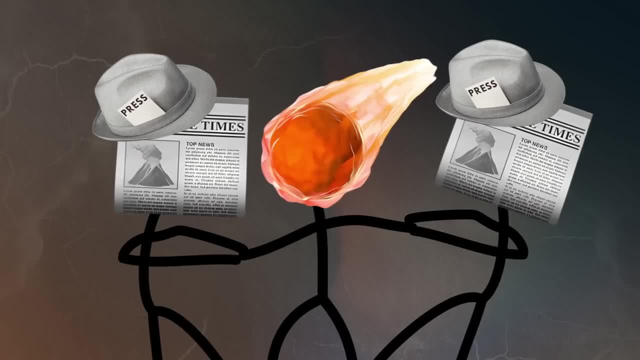 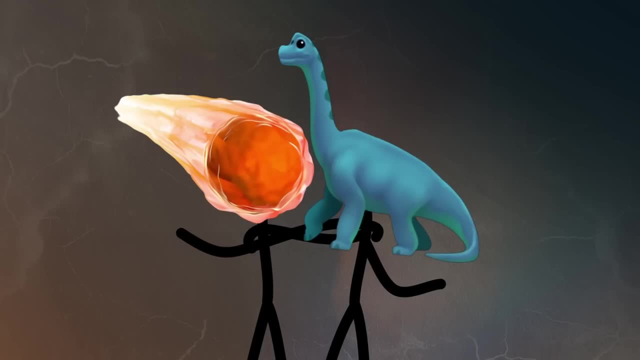 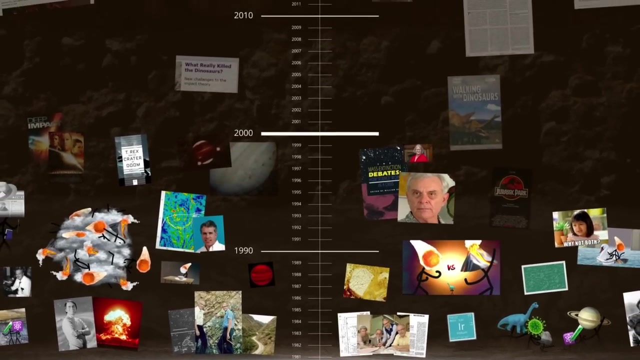 The media monstrosity might be pulling it in all sorts of directions, but international panels of scientists keep arriving at the same conclusion, Even panels of vertebrate paleontologists, those erstwhile impact sceptics. So maybe I should ignore all the noise, all the arguments, all the media spin. 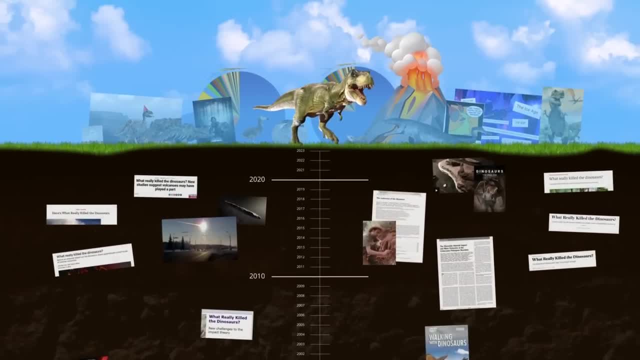 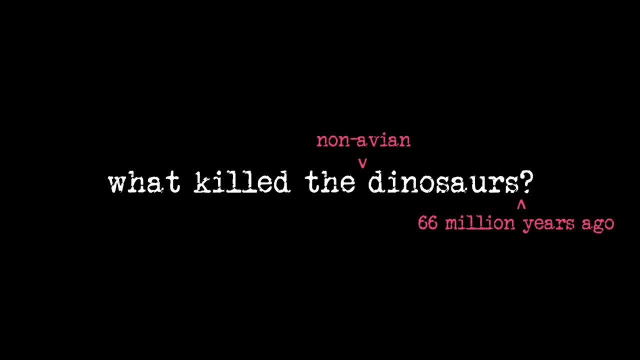 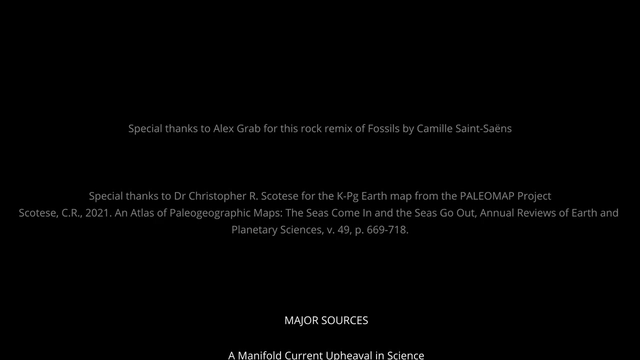 and trust Alvarez. I should, after everything, come to the conclusion that was obvious from the very start of the video. What killed the dinosaurs? An asteroid Hold on hold, on hold on a minute. Just one more thing. I read this popular science paper and I thought it was really interesting. 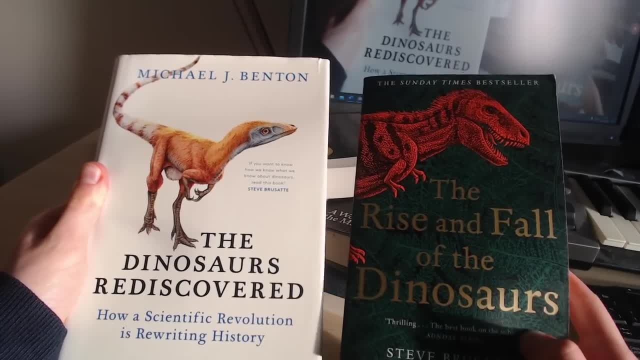 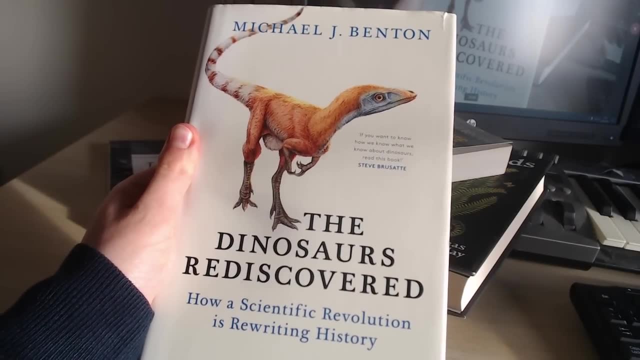 I read this popular science paper and I thought it was really interesting. I said I read this poepular science book and this one states, based on statistical modelling, that the dinosaurs WERE in decline beforehand. and this one states, based on statistical modelling, that they WEREN'T. 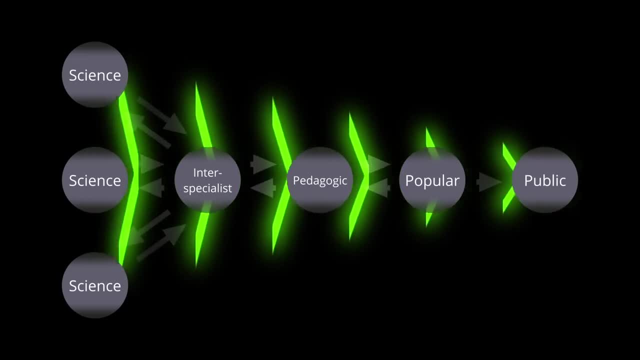 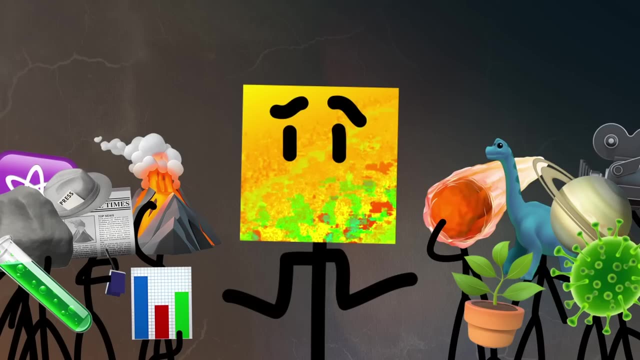 Two highly respected books A YEAR apart. Both sat at the popular end of things, where it's all supposed to be a thing of. Is this all true? If so, then you can't afford to paddle the weight of that. It never will be. 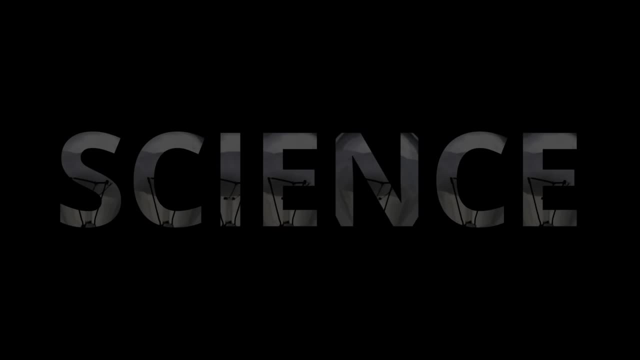 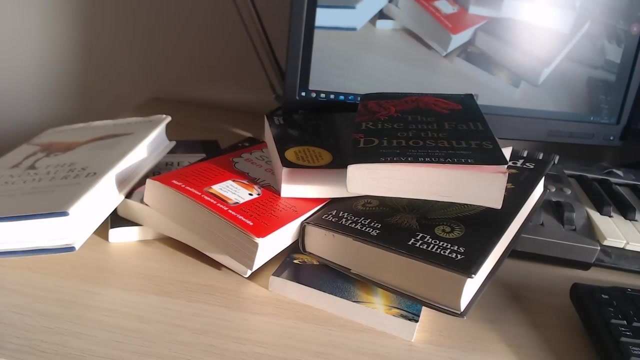 There's not enough gas in there to make the rest whatsoeverival about itㅠㅠ, anything. Are you enjoying this science? You've sent me down a rabbit hole and I've made a stupidly long video and all it's done is crush my confidence in any science I ever read, ever being accurate. 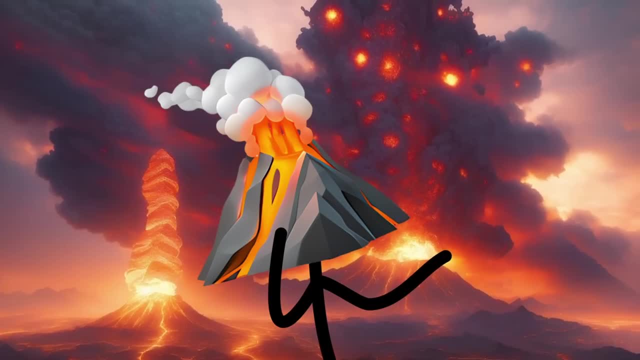 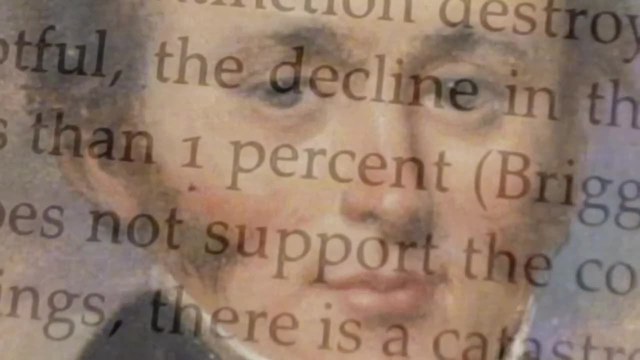 There are still people arguing for volcanoes. Why shouldn't I believe them? I don't know enough to judge their evidence. The media keeps telling me they've got something. Or maybe there was no extinction, It was just 1% of species. Maybe it was the space lasers. What is truth? How could 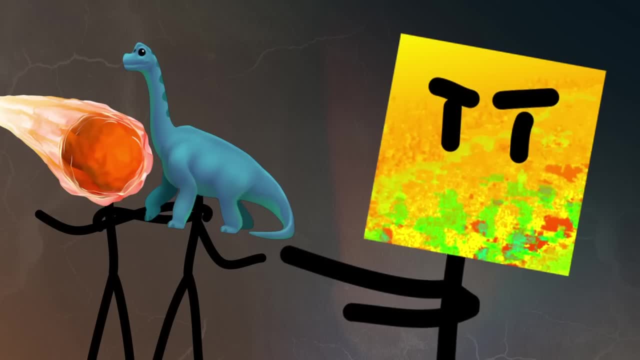 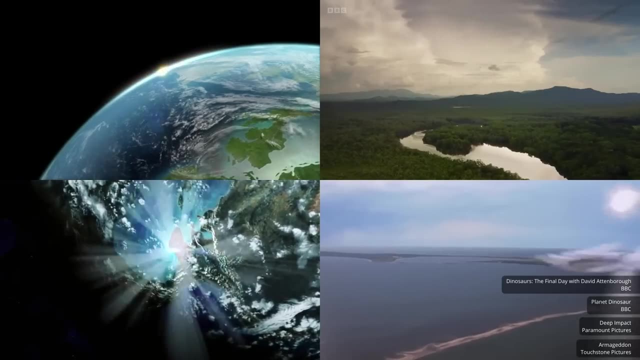 anyone even know anything in this ridiculous system. Oh, I just have to trust this panel. How do I know this panel is trustworthy when there are still doubts out there? I don't have the time or brainpower to understand. Science is a mess and it keeps shouting asteroid at me in a 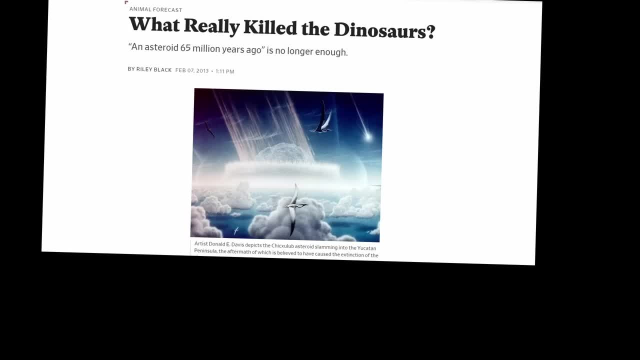 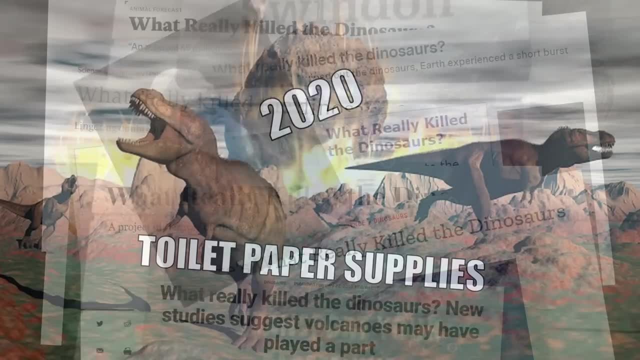 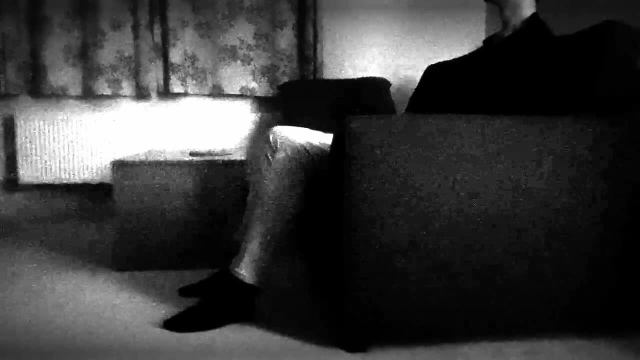 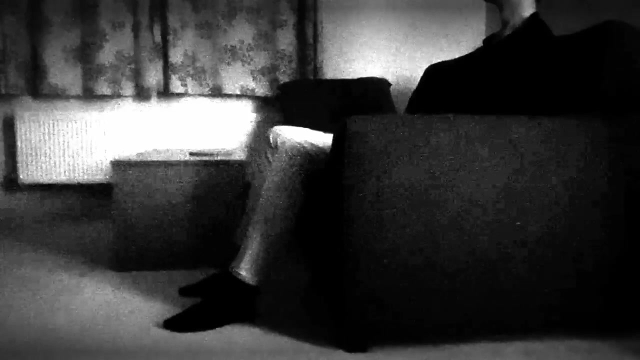 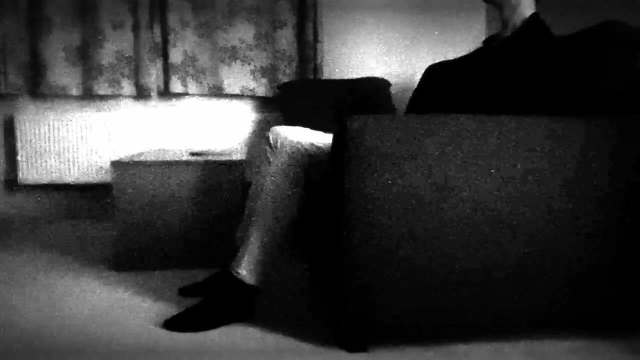 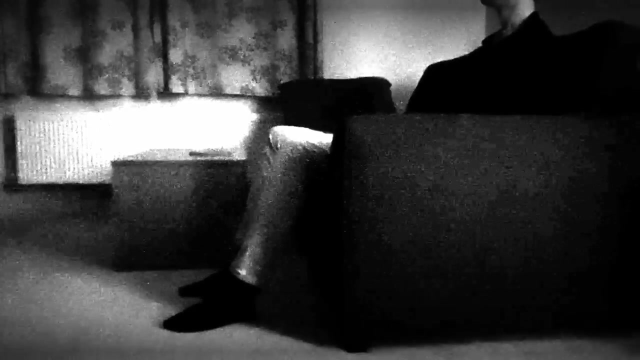 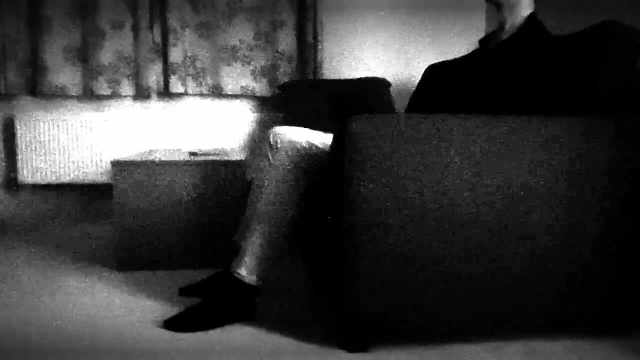 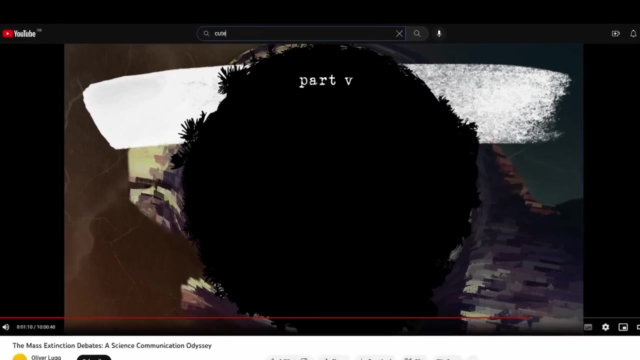 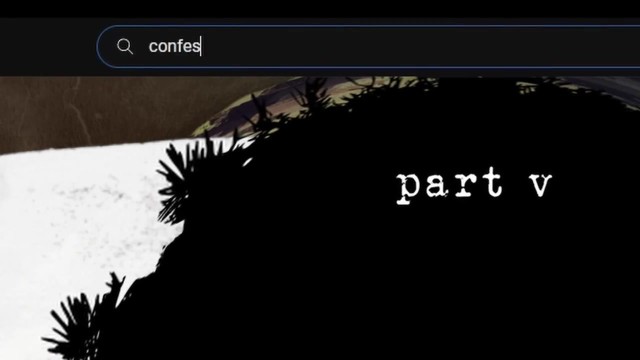 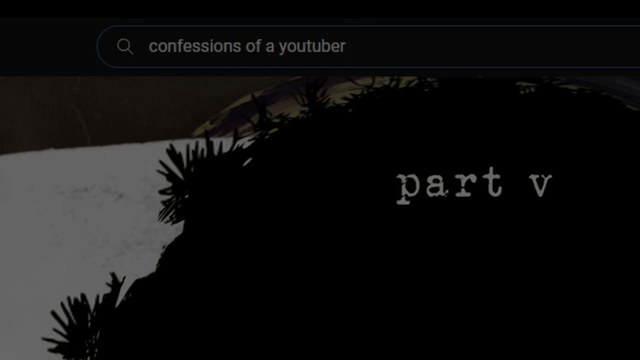 very suspicious manner and I don't know anymore What really killed the dinosaurs. Why am I doing this? No, seriously, why am I doing this? Confessions of a YouTuber As I read the many sources covering the mass extinction debates. 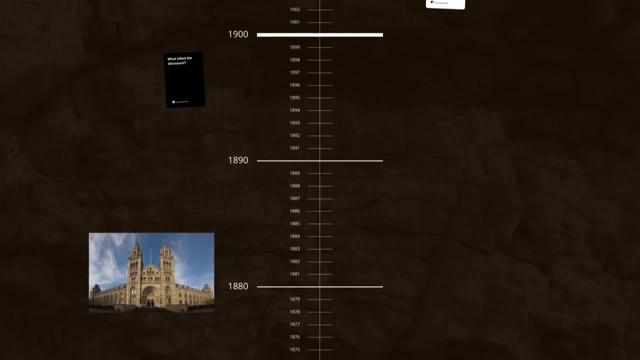 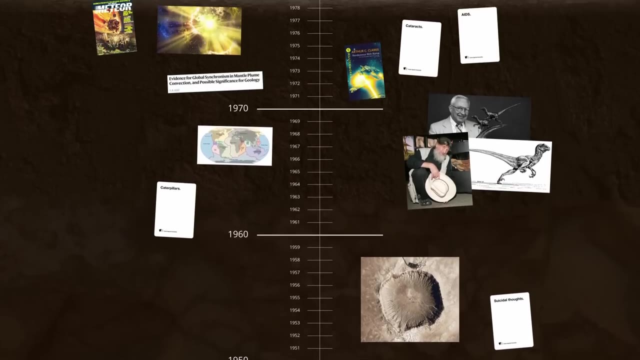 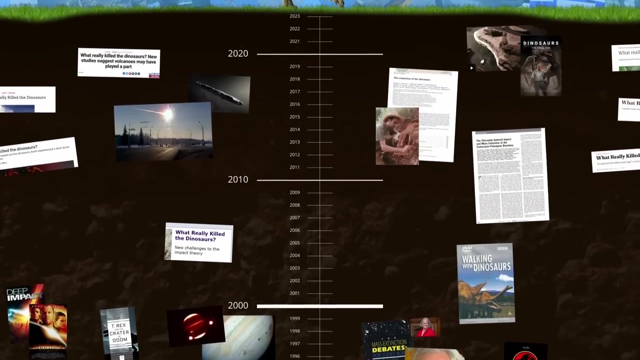 something was nagging in the back of my mind, A sense that many of them had missed something. Then it hit me. Many commentated on the event and denounced the state of science communication, as if the whole thing was separate from their current context. News articles ridiculing the media's involvement ended up looking naive. 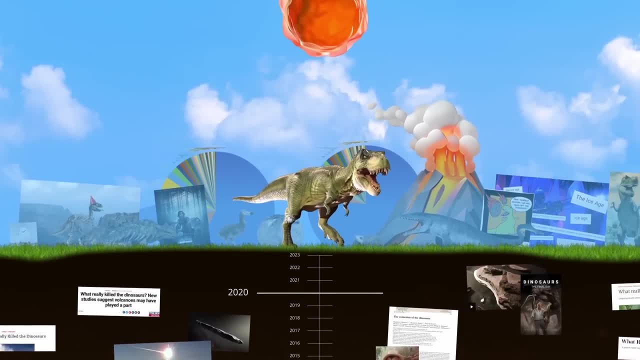 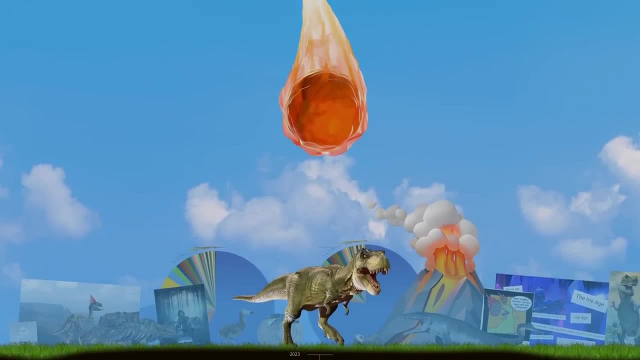 because very few of them acknowledged their own position, pitfalls and potential influence within the science ecosystem they so condemned. I've therefore decided it would be journalistically irresponsible of me to ignore my own place in all this. Why me? Why this video? Where does it fit? 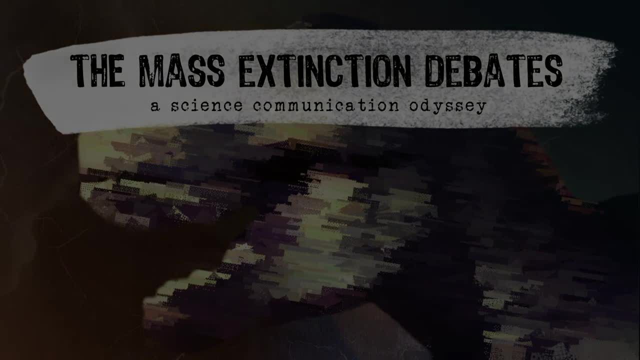 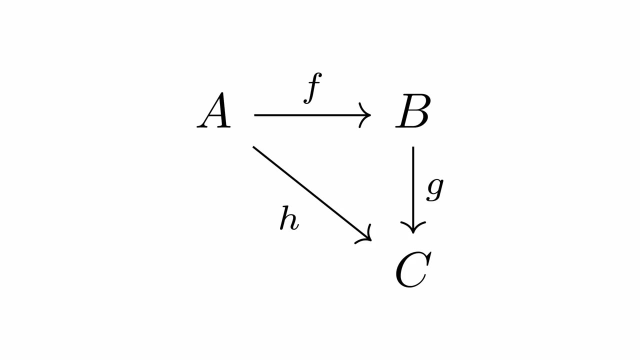 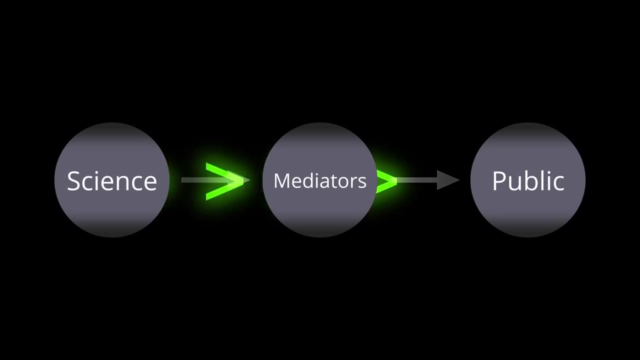 into the whole thing, Hopefully answering these questions, I'll be able to answer them in the future. I have a master's degree in mathematics, No qualifications in geology or paleontology or anything relevant to this video. I've always been fascinated by science communication, though. 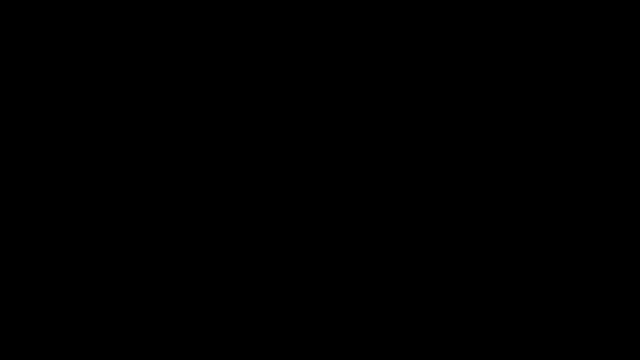 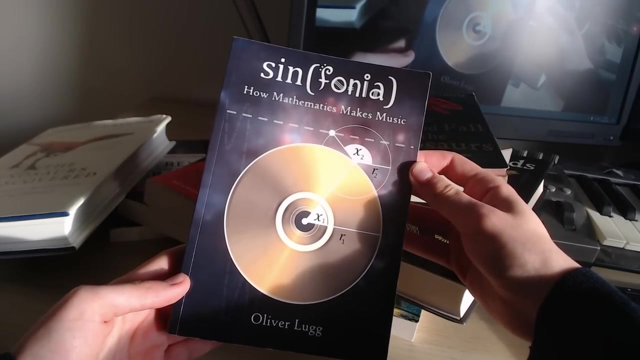 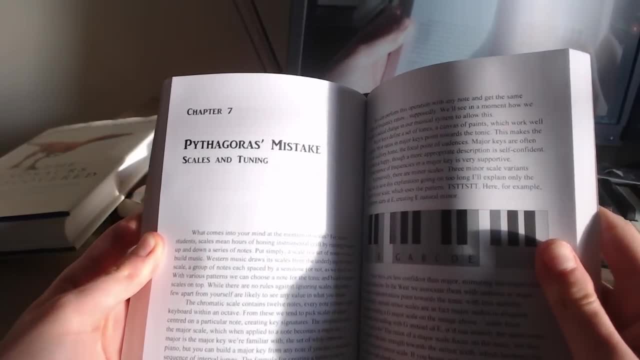 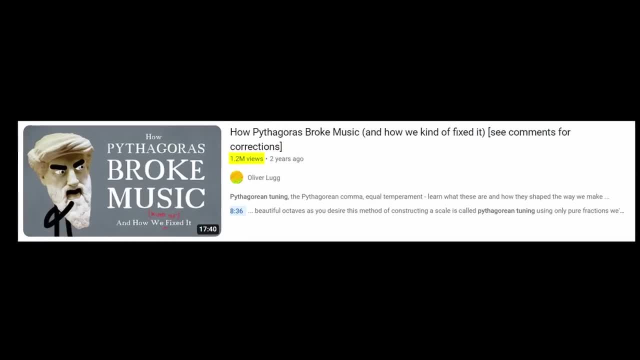 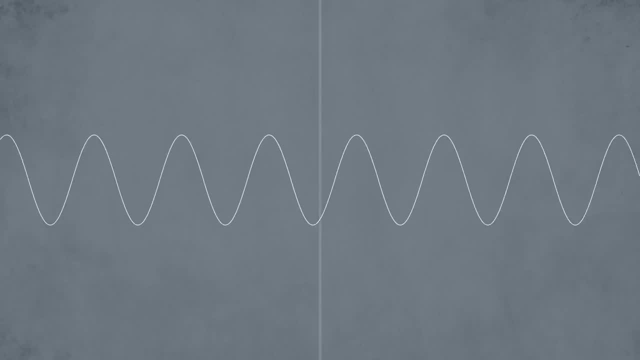 and that YouTube video now has a million views Mad right As a video. I'm still proud of it. Most people really like it. It's well-paced, well-explained and well-animated, except for the gap in the sine wave. Yes, I know, it's there. 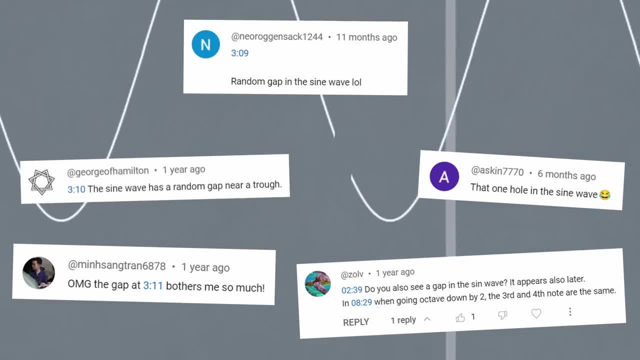 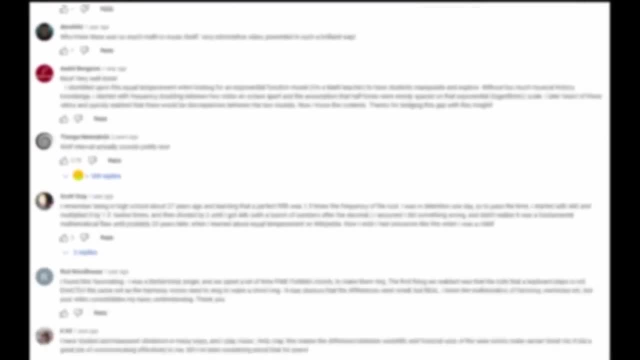 I had to leave it in as I didn't have time to fix it. Please shut up in the comments. If only the complaints in the comments were limited to the animation. For two years now I've been on the receiving end of a non-trivial amount of. 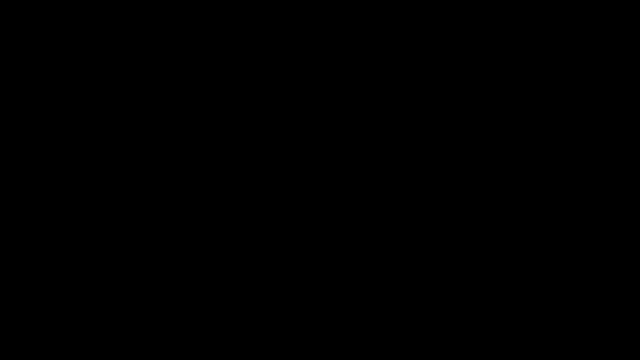 vitriol regarding the video's content, It's a video about the history of the maths, of music, And while the maths- my specialist subject- is A-OK, the music and history… While I maintain there's only one thing I said that's outright, factually wrong. 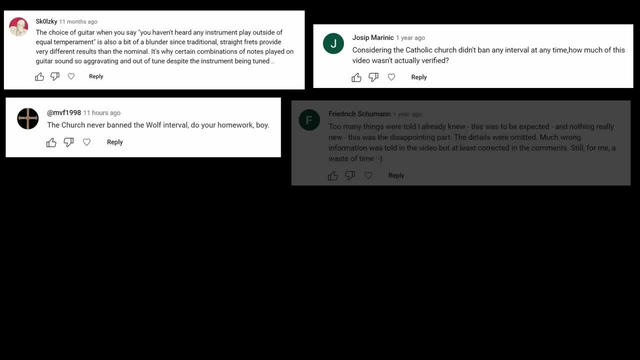 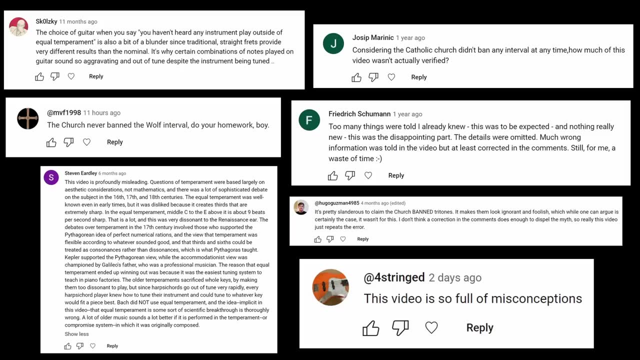 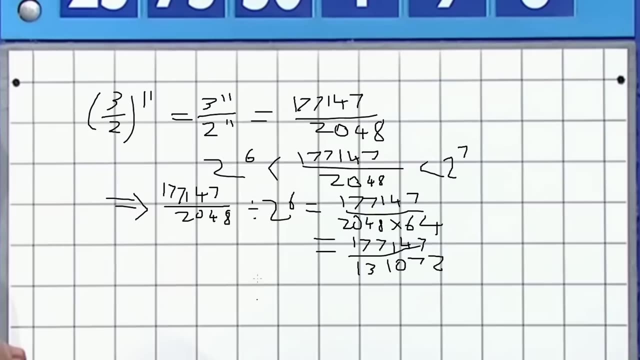 I didn't do myself any favours with misleading phrasing, key omissions and oversimplification. There were plenty of reasonable comments pointing this out, and a few quite hurtful ones, Turns out I had approached the video from the mathematical zeitgeist and relied too heavily on popular representations of the other subjects involved. 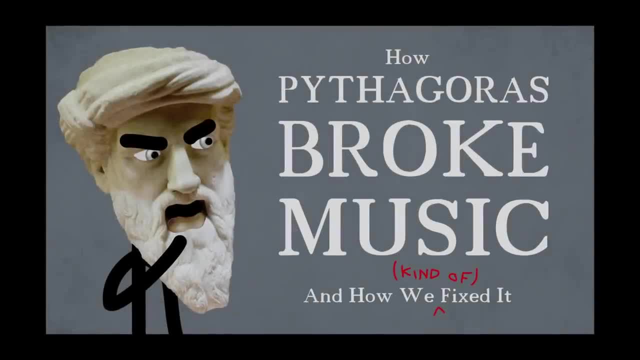 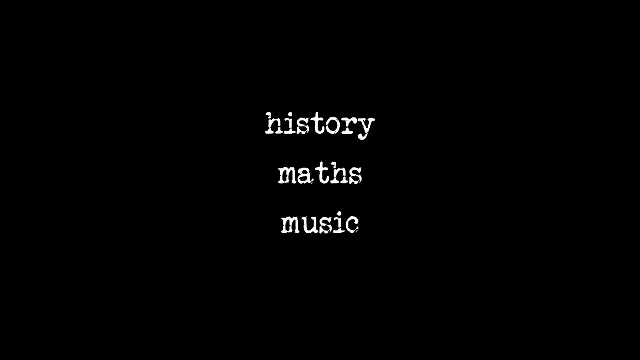 What does that remind you of? Now, I'm not the victim here. My video got too popular. woe is me. No, that's not my point. My point is that a video made by someone without formal grounding, in half the stuff they were. 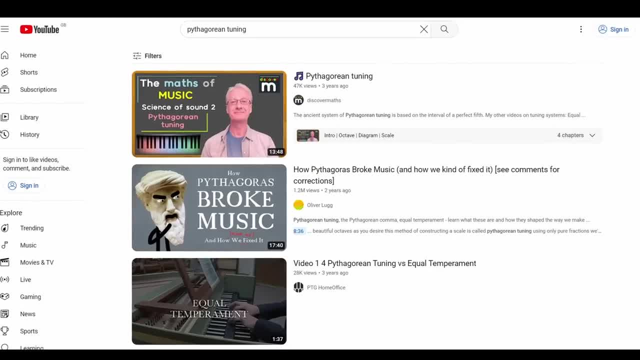 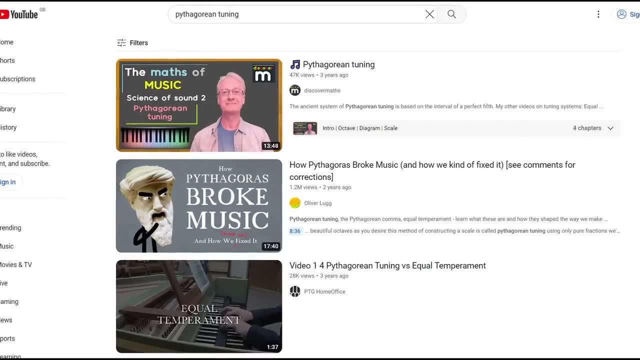 talking about is now many people's go-to reference for this topic. Seriously, I've had several people email me asking if they can cite the video in university projects of their own. There are doubtless many more who did that without contacting me. I did not make this video with the academic. 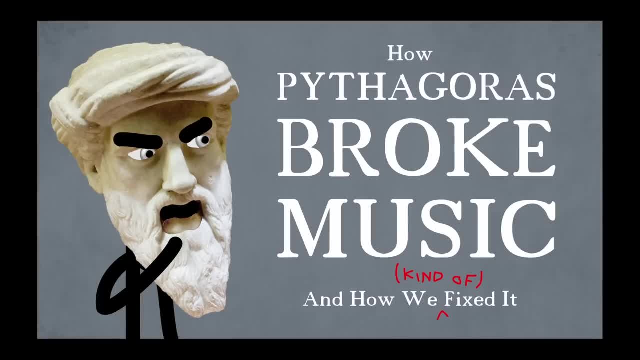 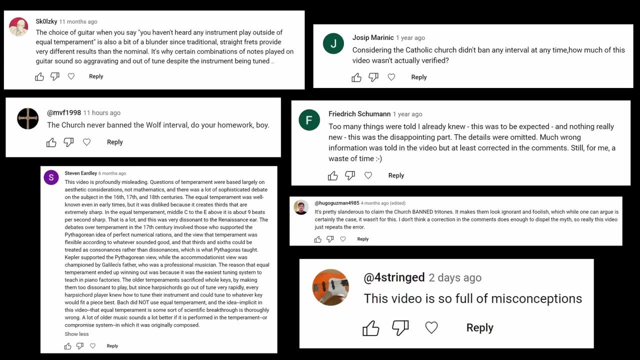 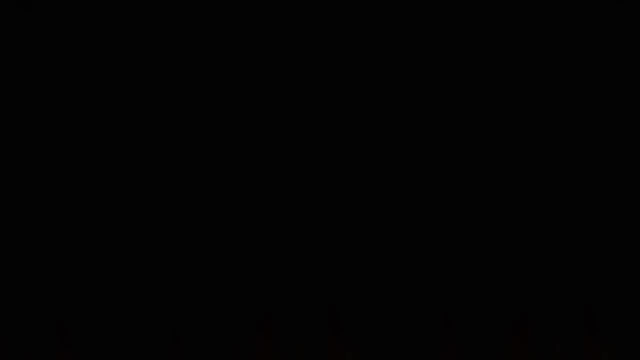 authority that befits something a million people have seen. But the internet doesn't care, Unless you stumble upon a comment from someone who knows better. you're probably going to believe every word I said, And that scares me. It scares me that a single person with mediocre knowledge of a topic 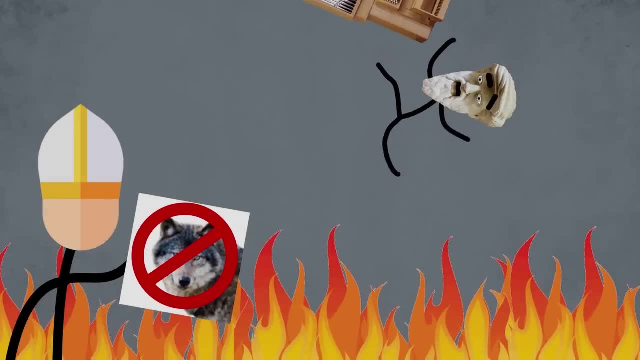 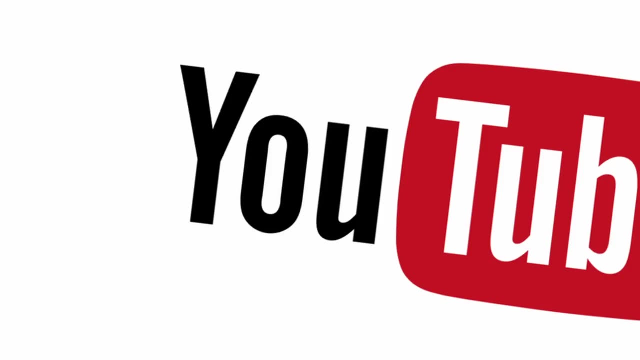 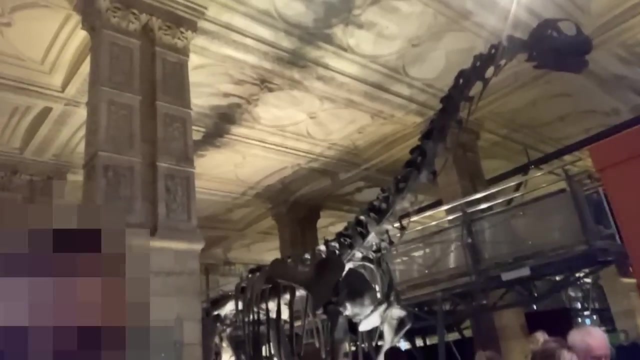 can have such outsized influence on media perception of that topic. I know I'm not an isolated case. It's in the name YouTube. You And you're all scientifically proven to be idiots. Me, though, I'm admitting I'm an idiot. Remember I don't have a face. You shouldn't be trusting me. 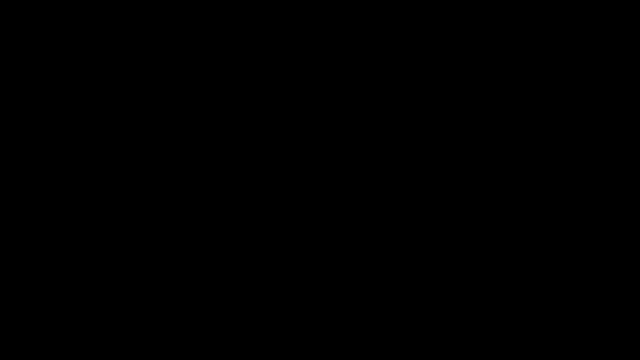 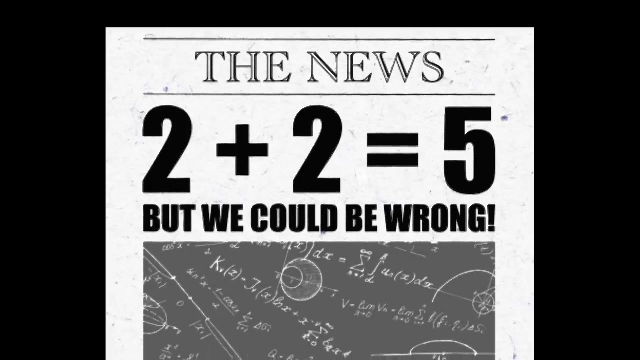 Yet just by saying that, I can make you perceive me as more trustworthy. Sure, admission of uncertainty is necessary for good science, But it's not sufficient. I could have been lying about that, just as I've lied about everything else in the video. 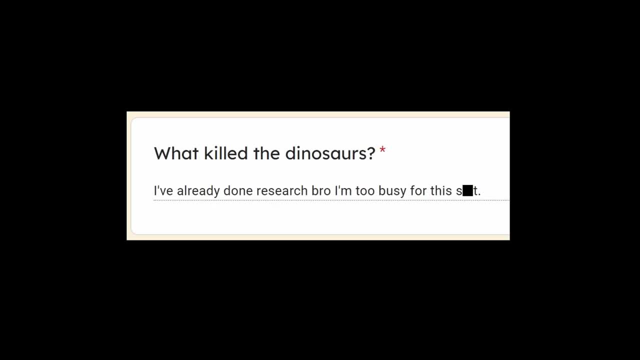 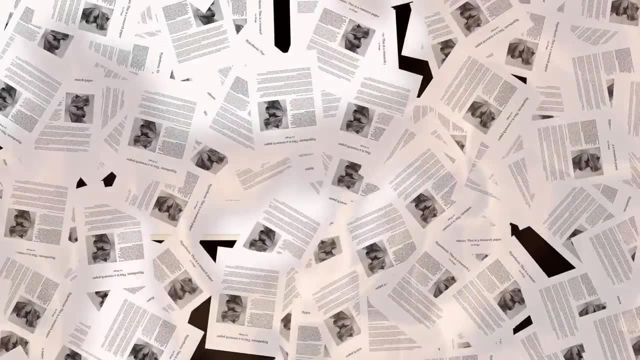 Maybe- How do you know, You're not going to take time out of your busy and multifaceted lives to check all my sources and then check all their sources, and then collate every academic review to know which of those sources run fairly biased, and then read the entire history of science. 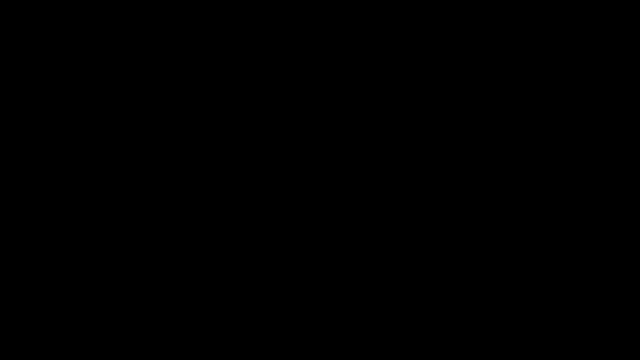 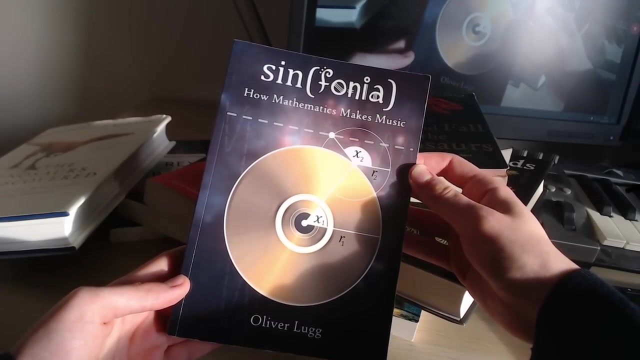 to know whether those reviews are being held hostage by a problematic paradigm In producing the book all those years ago. that would land me in hot Pythagorean water. I drew a lot from 2008's handbook of public communication of science. 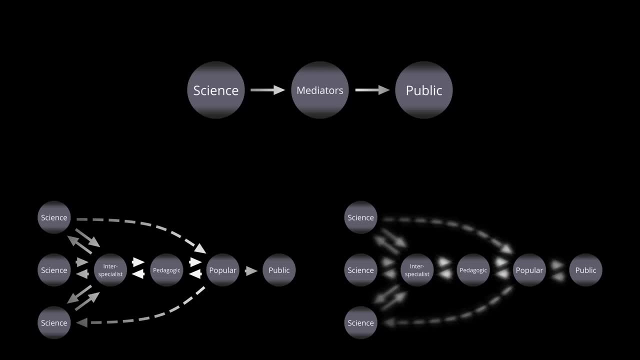 science and technology, which I went back to for this video. I squashed its overview of communication theory into my aside- last chapter, for instance. Very much recommend it's more thorough treatment. if it piqued your interest, We'll come back to the handbook itself, but right. 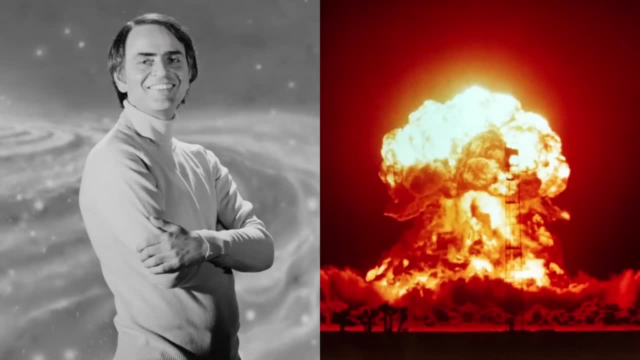 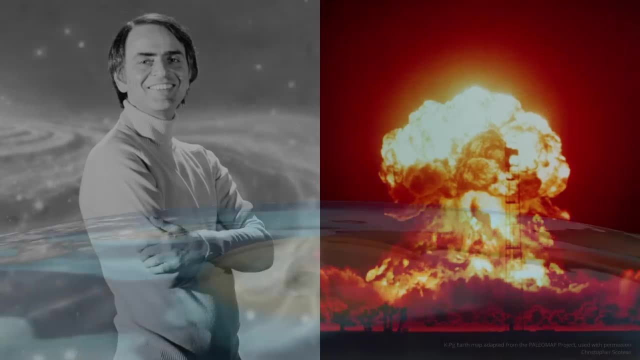 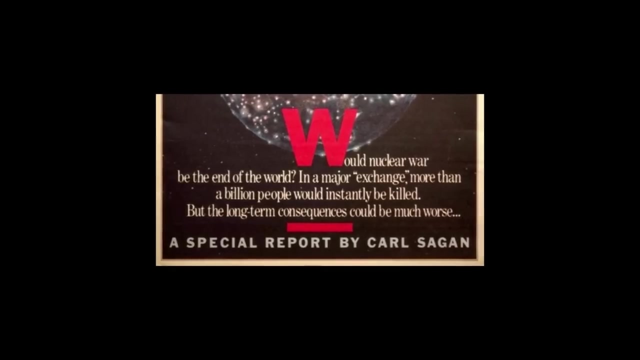 now let's talk about this guy. Carl Sagan, you may remember, spearheaded the push for governments to recognise the threat nuclear winter posed to civilisation, A theory inspired by and arguably instrumental in promoting the Alvarez impact hypothesis. His deviation to the popular level. 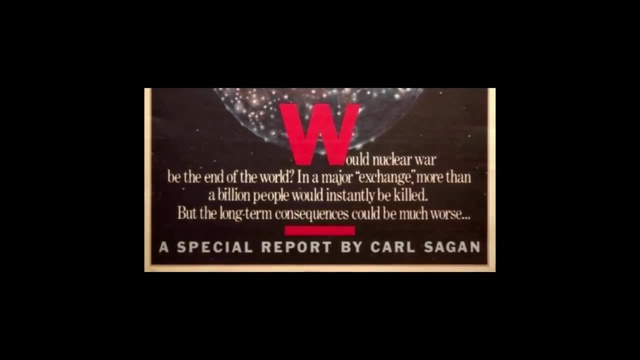 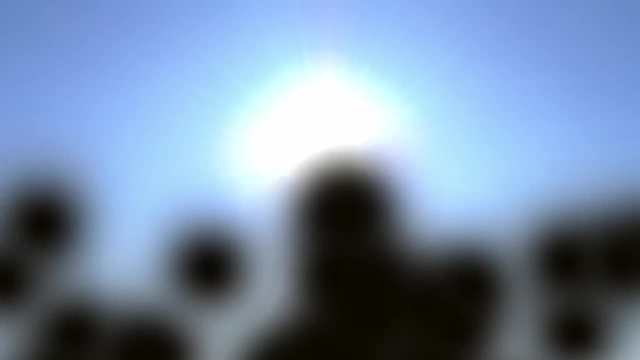 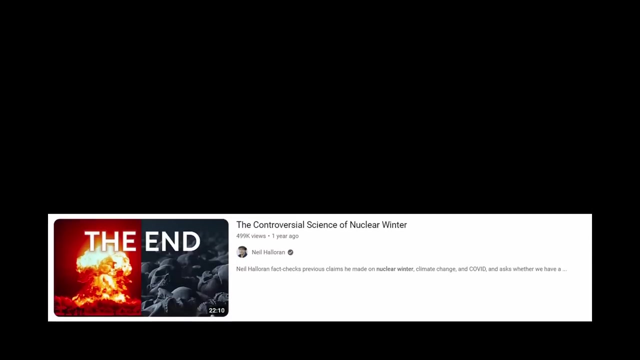 succeeded in instilling the fear of nuclear winter in our minds, but once scientific enquiry reeled it back in, the theory came up short. Many modern experts doubt full-scale nuclear war would throw up enough aerosols to block out the sun. I know this because I watched a YouTube video. 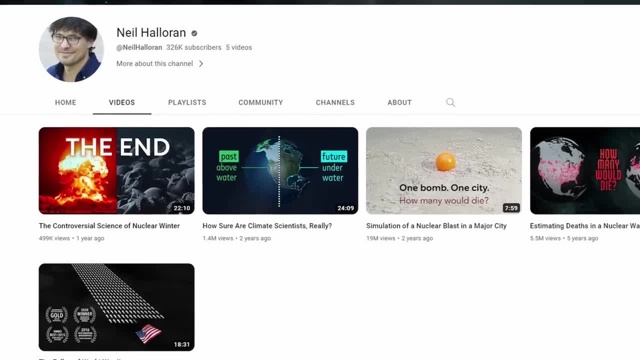 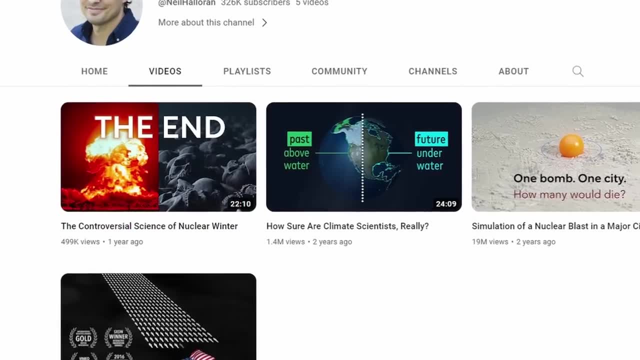 Neil Haloran's videos are some of the finest things you can watch on the platform, and his latest re-examines an earlier claim he made about nuclear winter. The video is part of a broader series looking at how much we can and should trust science. But even here, in a video about 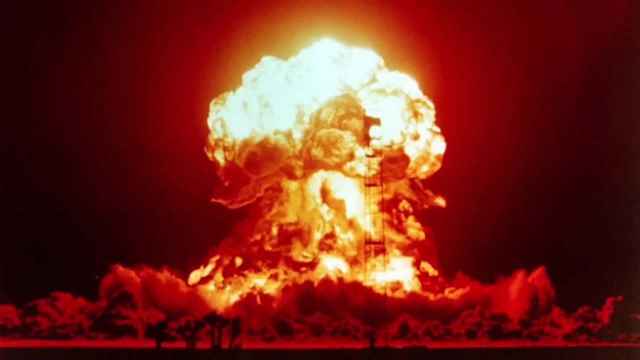 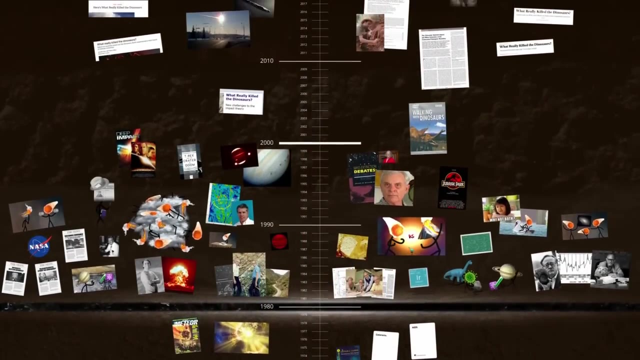 a theory we all take for granted, and the implications of trusting its extreme claims on communication dynamics. Neil does not once mention the extraordinary journey of uncertainty surrounding the impact and impact winter. Instead, it's the comparison point, A solid, well-grounded theory to contrast the one 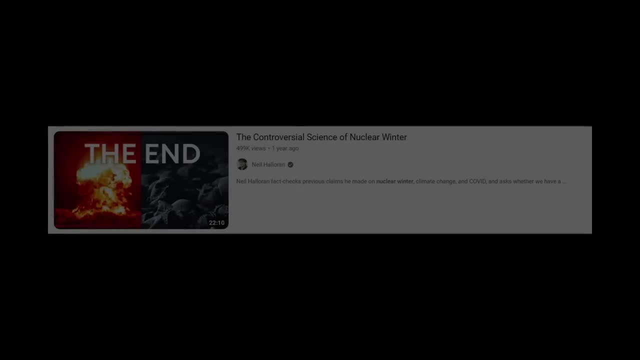 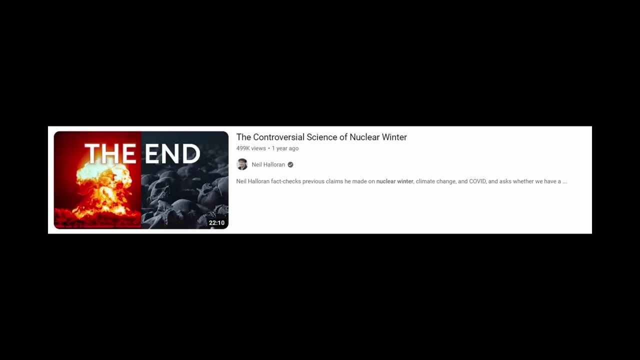 and just structure-bulleted theory to contrast the one being upturned. Neil may well have been aware of the impact debate quagmire but either way reasonably did not get into it. I just found its framing a bit astonishing after. 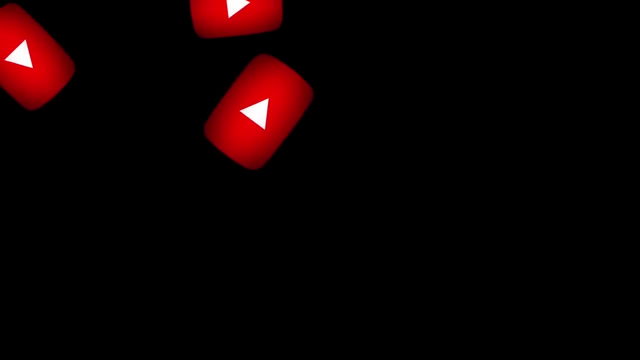 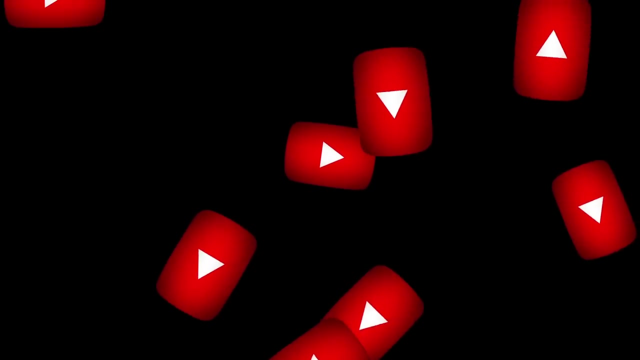 well this If accepted beliefs in a video about questioning beliefs may be uncertain. how much is there being presented as fact on the site, despite intense arguments to the contrary, Not maliciously, not intentionally, merely out of necessity? How much is there being주quis 박 onsite? 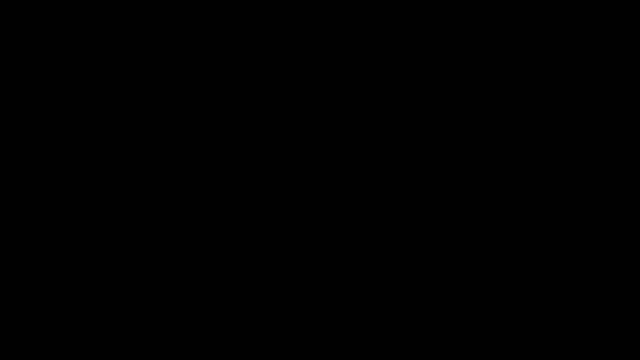 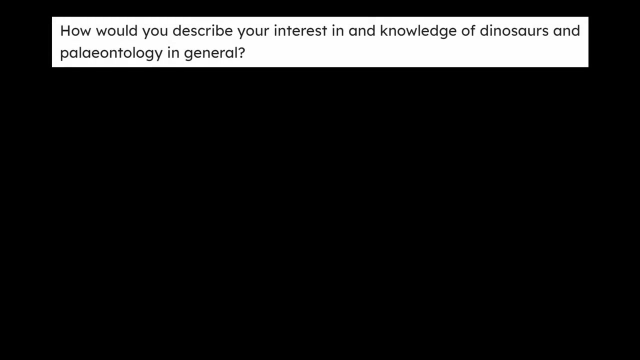 How much have I mindlessly believed? I was further taken aback to discover that, when asked about their interest and expertise in paleontology, many of my survey respondents said more or less nothing, except I binge watch YouTube videos about it. 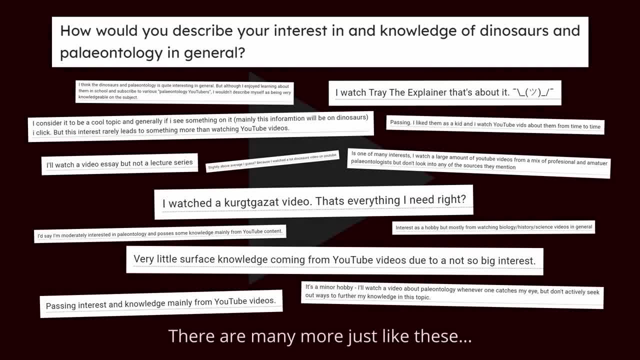 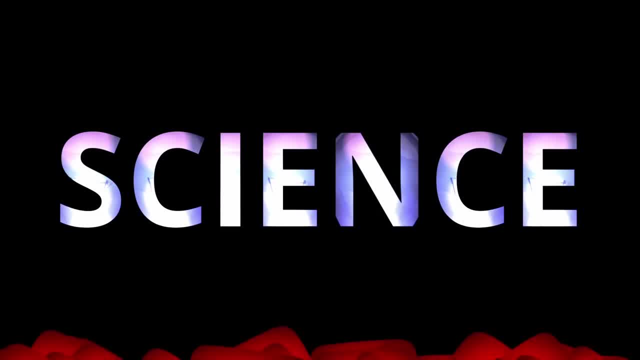 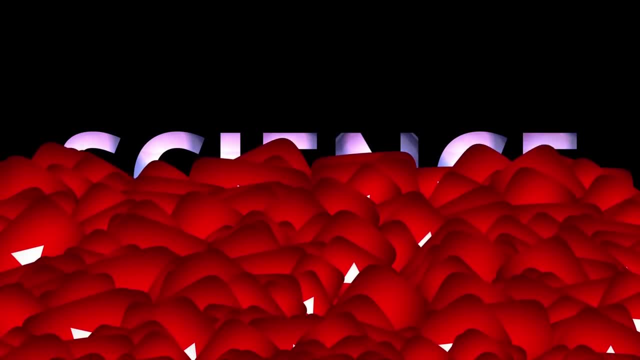 Okay, the sampling bias of distributing the survey to YouTube users is about as extreme as you can get here, but that's not making me feel any better. The participation model has reached a new extreme. Everyone is a science mediator. With the internet's whirlwind of constant information and the lowering barrier to entry. 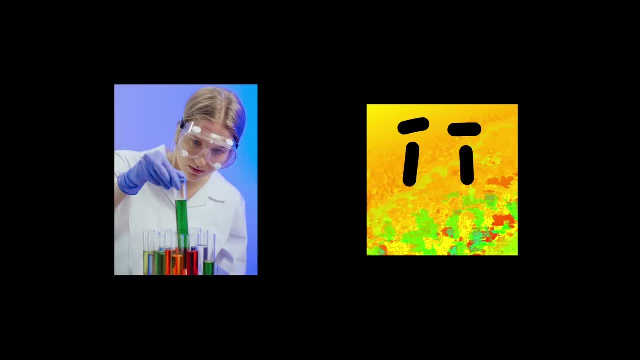 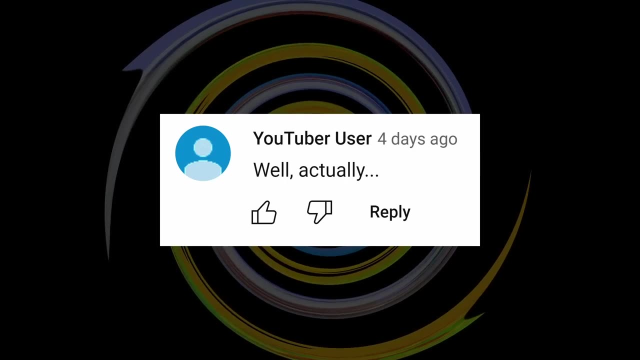 for joining in with a snazzy production. professional and amateur science communication are intermixing without oversight. Only the ethical fortitude of the creator and the threat of a million well-actualies in the comments prevent a video slipping into the dark recesses of misinformation. 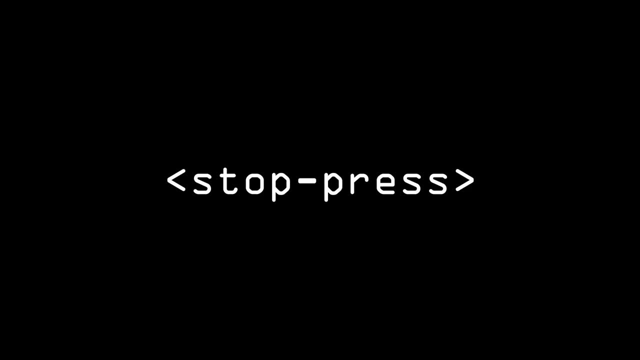 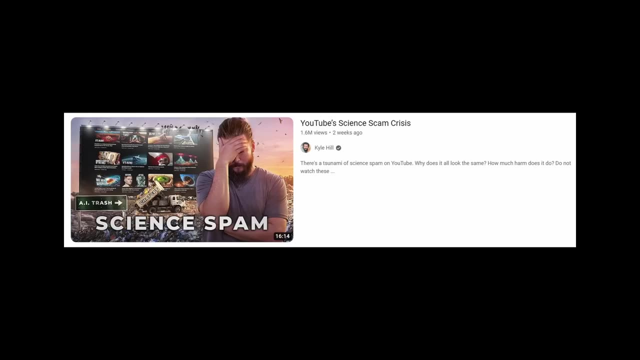 Hello, Er, stop press time, I guess. Shortly before I finished editing this monstrosity, I came across a video by Kyle Hill calling out the influx of trash. AI-generated 100% misinformation science content on YouTube. 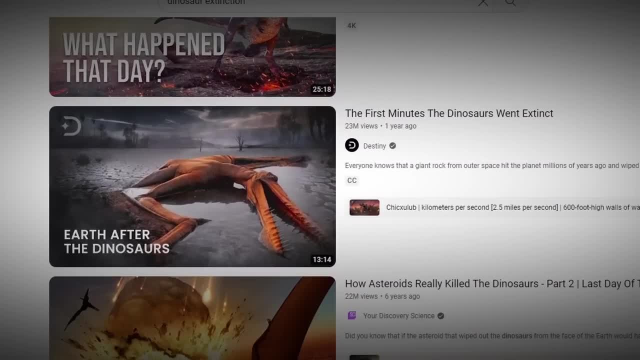 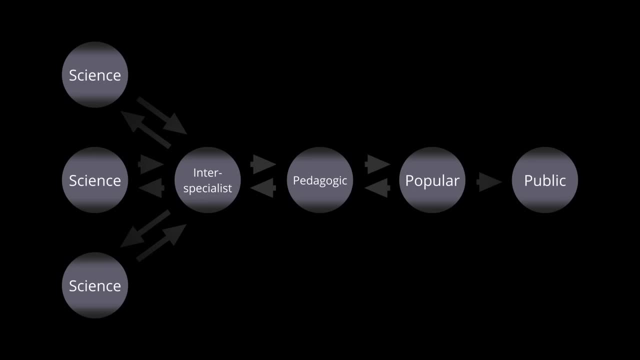 Wonder if it's infiltrated the KPG extinction space? Oh yeah, Coulson has. You know, when everyone's a science communicator, no one is Kind of stealing Oliver at the end of the video's thunder here, but I happen to believe. 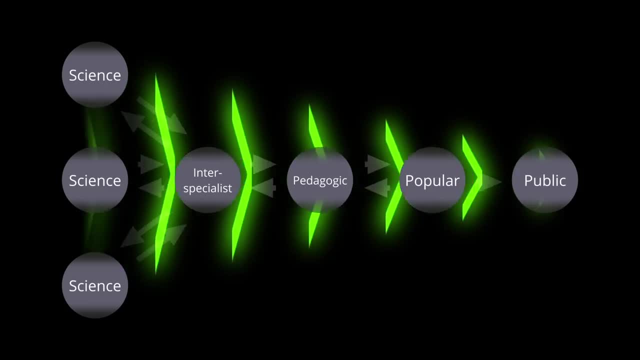 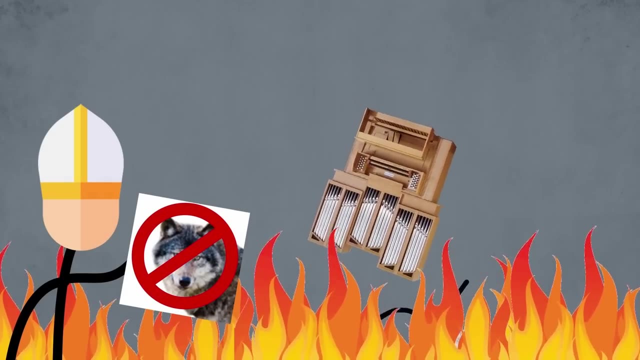 the context of information, delivery is more important than the content. If you're annoyed, this video has been and will continue to be about me as much as a science. that's the point. This was always going to be information refracted through my own eyes, so why not lean into? 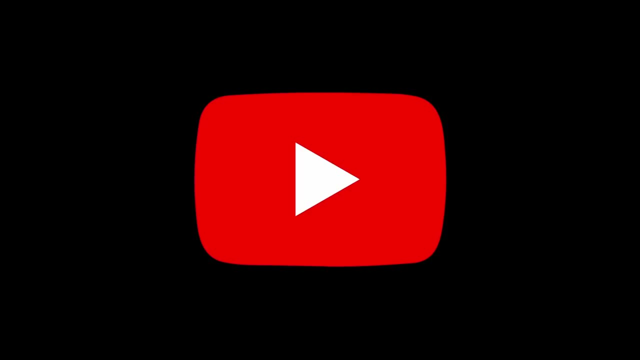 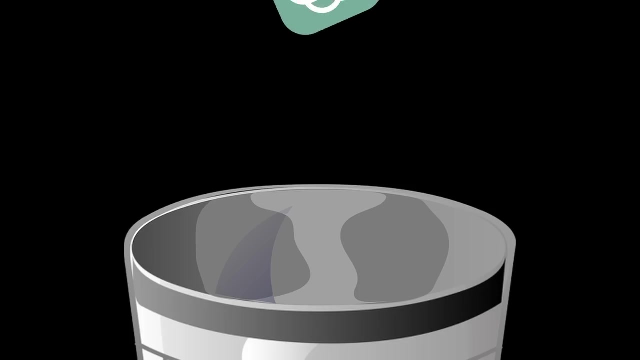 it and make awareness of that the message. Why not hold on to the fading crumbs of personality I can muster for this godforsaken website? Needless to say, I don't believe the correct path forward here consists of tools which, by their very nature, remove all context that's even removed from the content of this video. 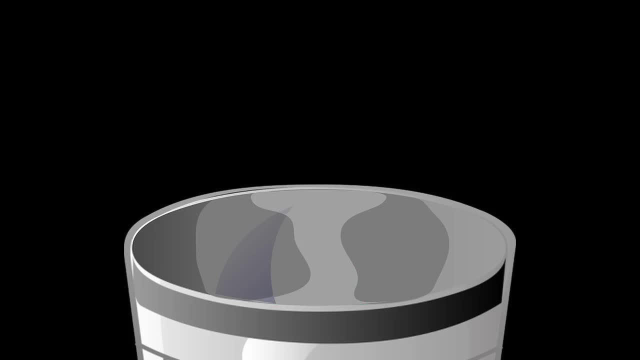 I don't believe the correct path forward here consists of tools which, by their very nature, remove all context. that's even removed from the content. that's even removed from the content I can muster for this video. Watch this video. don't watch these videos. 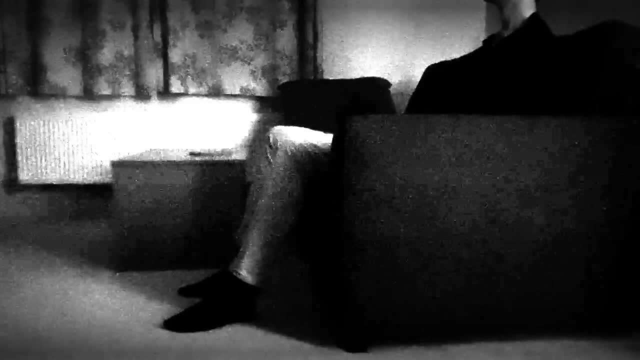 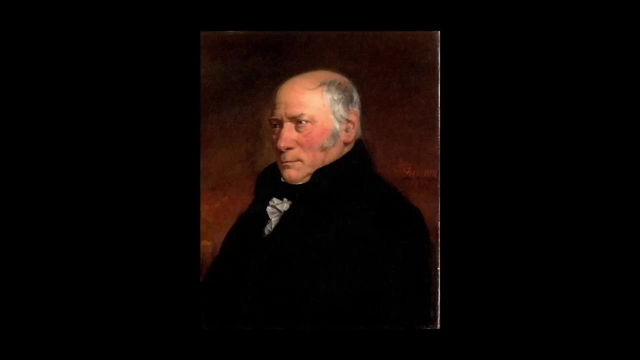 Stare blankly into the gaping abyss of your own insignificance. Have a nice day. Ok, that's enough fun. Is this video Misinformation? It is, first and foremost entertainment. There's a bunch of stupid jokes in it for crying out loud. 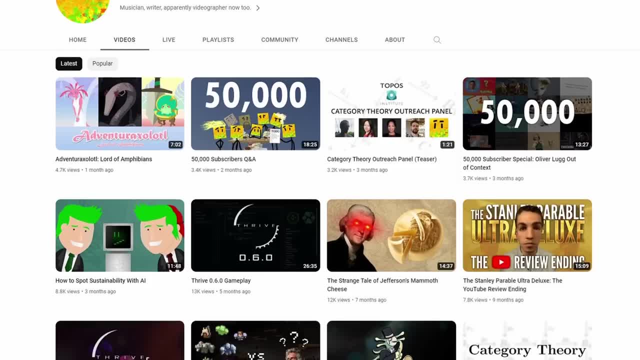 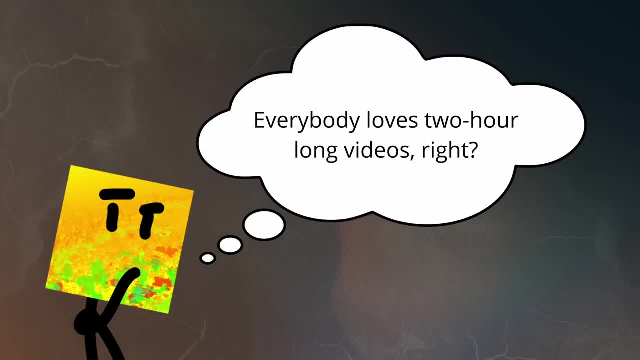 I make videos for my own enjoyment. I am an individual spending my free time spinning an interesting yarn for casual internet viewers. All my narrative choices are made in this video, this context. I simplified and satirised complex issues to save time, to make them more memorable. 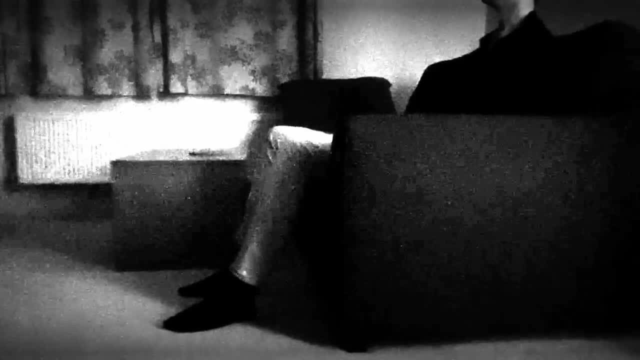 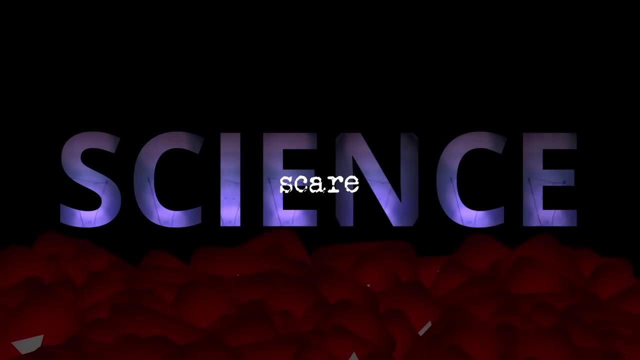 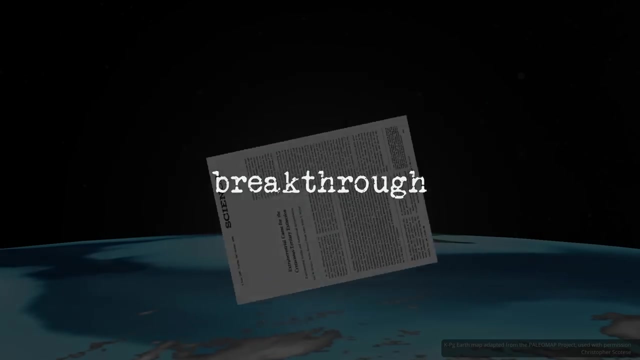 and frankly, because it's fun. Is it fun, Is it? I'm fully aware that I've been indulging in the very communication evils I've denounced. Am I a bad person for doing that, even if I've taken every chance to highlight how I've warped things? That's for you to decide. But in my defence about 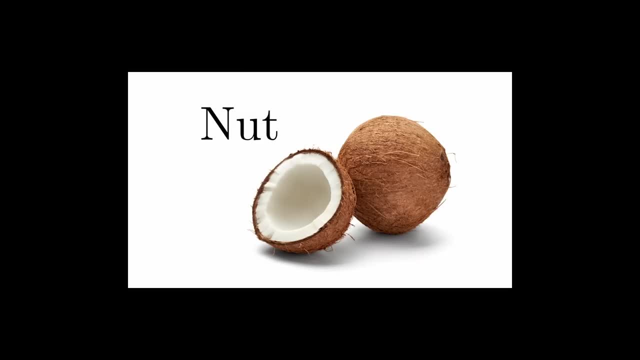 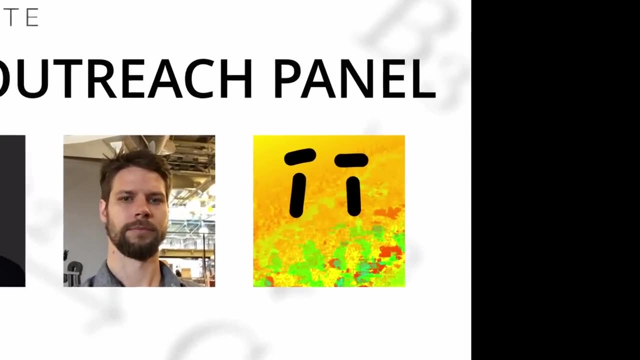 the immense amount of wacky in particular. last time I trivialised a subject this badly, I got invited onto an outreach panel. This website makes no sense Either way. fun shouldn't be an excuse for factual sloppiness. I can't prove it, you can't verify it. 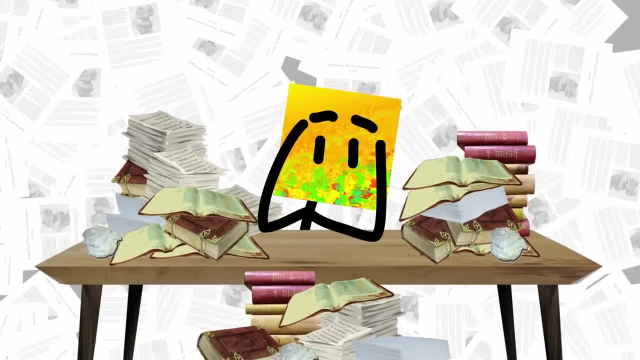 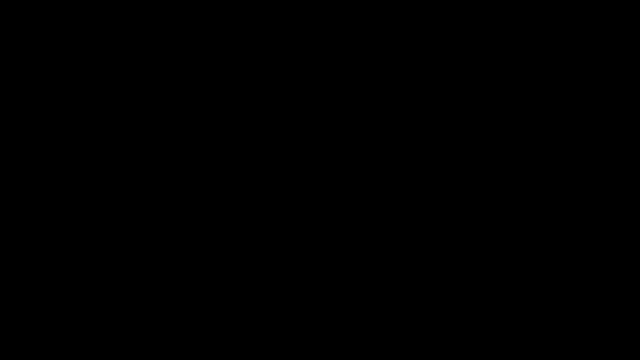 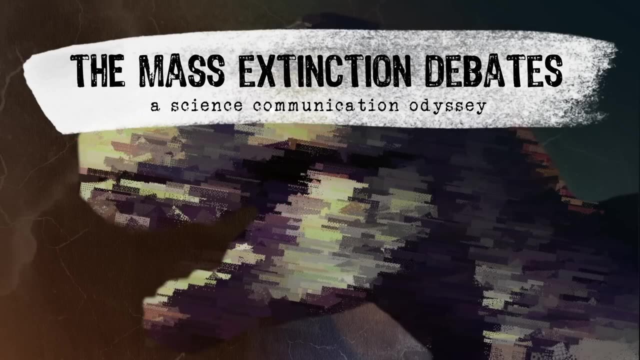 but I promise I tried. I've put as much effort as my free time allows into meeting an acceptable standard of accuracy. That said, I am human. I've probably made mistakes. Please let me know if you find any. But why this video? Why the mass extinction? 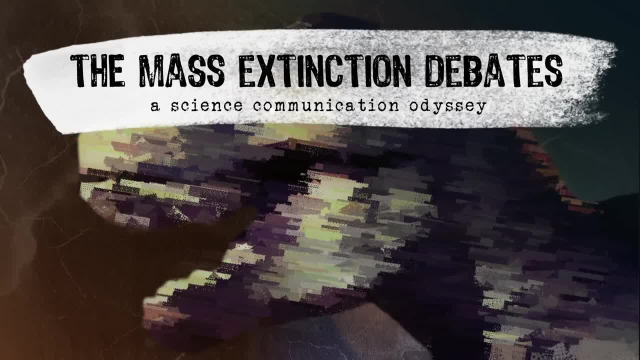 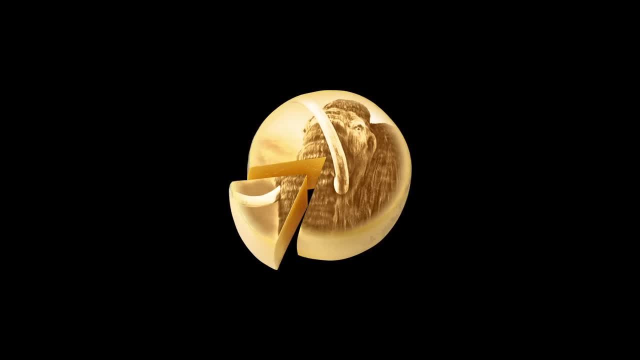 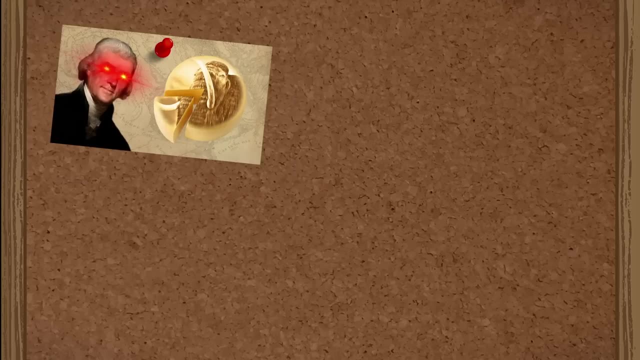 debates as a case study on science communication. in the first place, What point am I even trying to get to anymore? Well, our story begins with mammoth cheese. I made a video about mammoth cheese in September. It went down well for myself and my subscribers, so I thought. 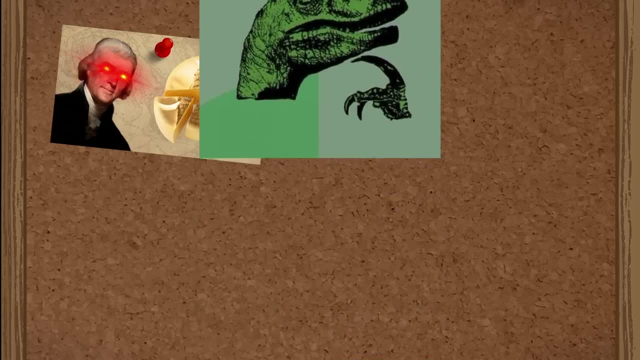 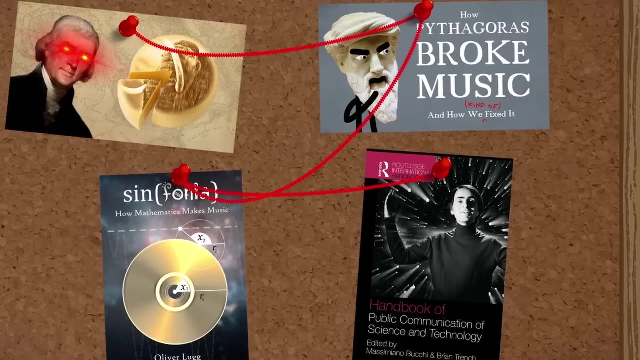 what other obscure paleontological factoids do I know of that could result in a neat video. And I remembered the Pythagoras video and the book it grew from and the book that grew from and I remembered a single line. I'd read in that book six years earlier. 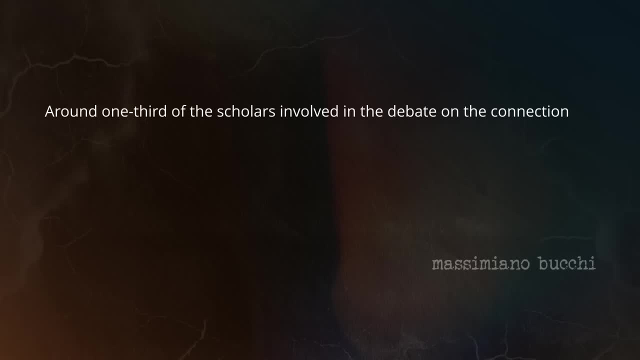 Around one third of the scholars involved in the debate on the connection between mass extinction of dinosaurs and a meteor collision with the earth stated that they had heard of the impact hypothesis from the mass media, And I thought that's a cool and little known statistic. 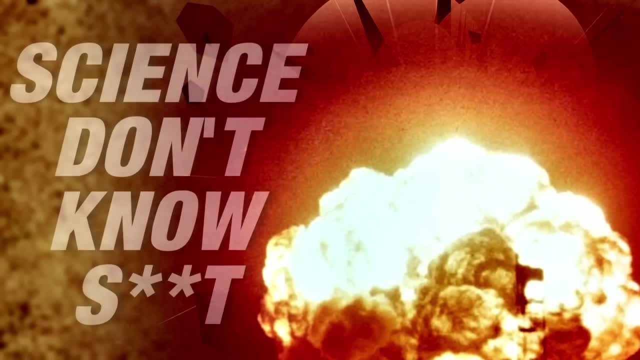 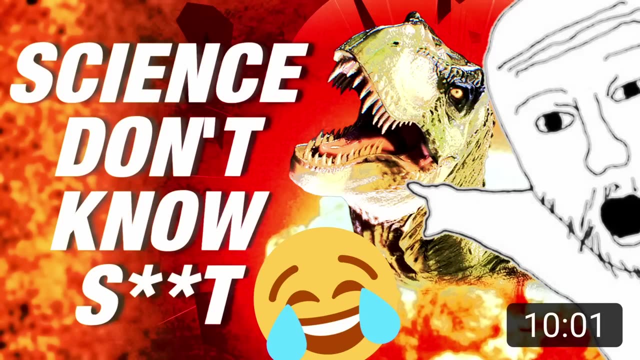 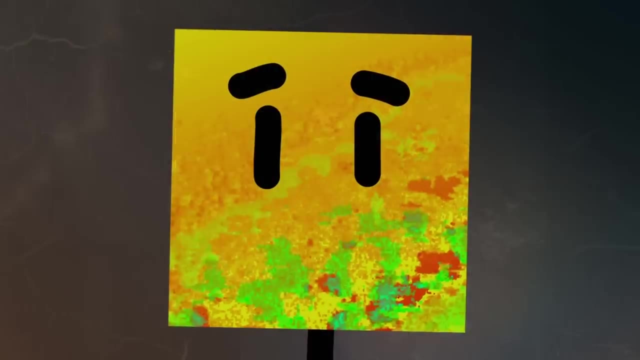 I could make a video about that. say something provocative about how media poses rigidity on science, yet scientists are reliant on it. Add some dinosaurs, bish bash, bosh like a ten minute video, instant hit. Yeah, what kind of colossal hypocrite would you have to be to talk about popular science dynamics? 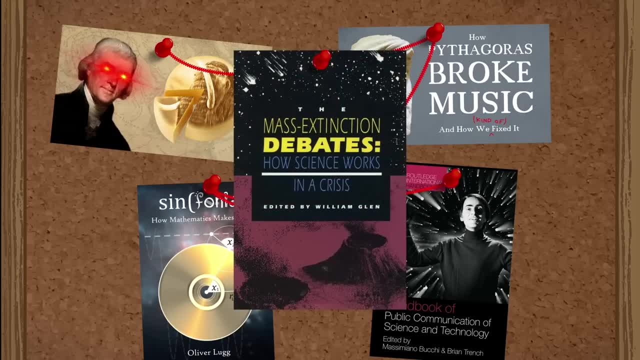 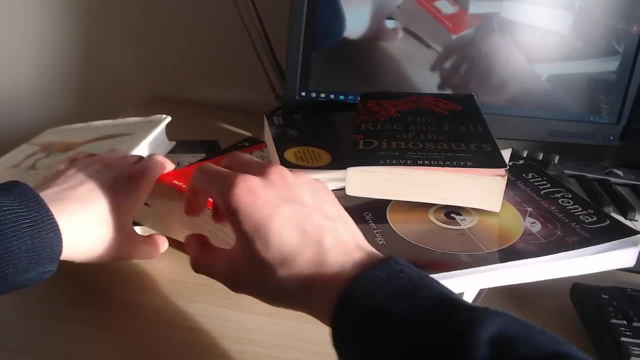 based on a single line of research, So I sought out the source. Mass extinction debates isn't the ultimate origin of the statistic that honour belongs to this article, but it was the item reference to the mass extinction debate And I thought that's a cool and little known statistic. 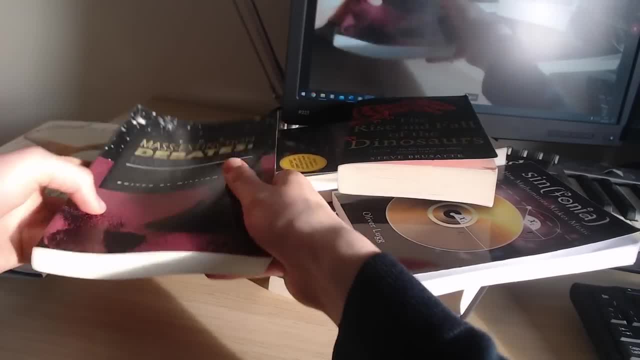 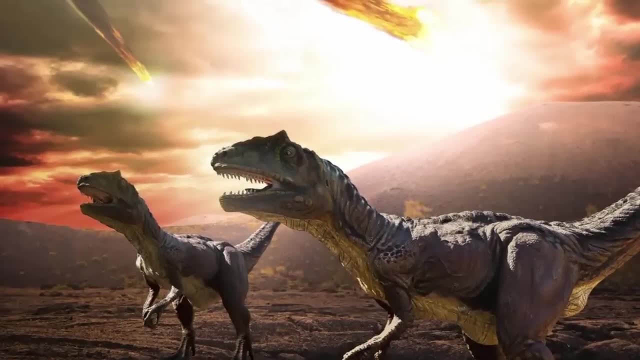 referenced in the handbook, and it opened my eyes to the scale and theatrics of a conflict that had raged years before I'd even been born, A conflict I assumed my whole life was all but settled. The reference led in particular to Elizabeth Clemens' chapter on the debates and 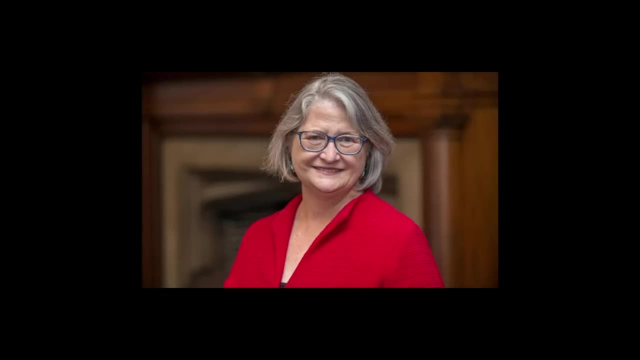 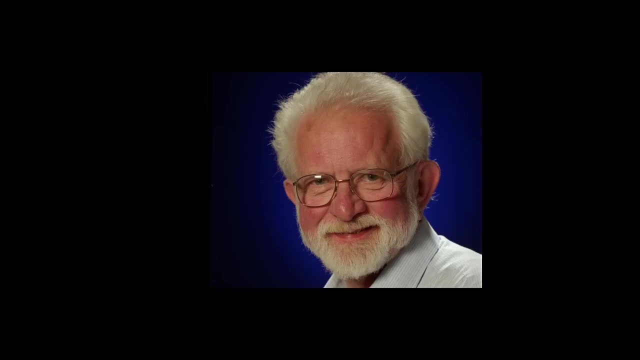 popular science. As noted, Clemens is a political sociologist, but she's also the daughter of William Clemens, vertebrate paleontologist, and one of the Alvarez team's most consistent opponents. She therefore had a unique view and she was a political sociologist, but she was also a political. 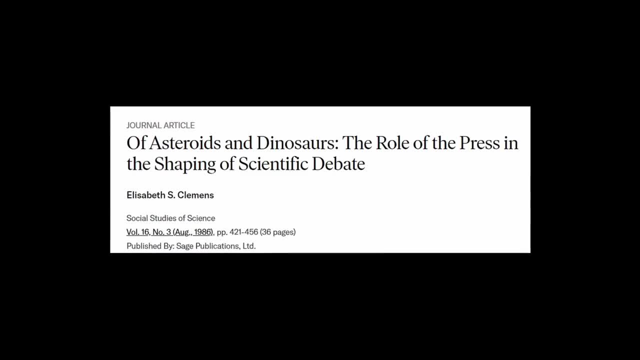 sociologist. She was also a political sociologist, but she was also a political sociologist of the debate's societal components. writing multiple articles on a topic I can only recommend. By the time I got around to reading her chapter in earnest, I was already neck deep in other. 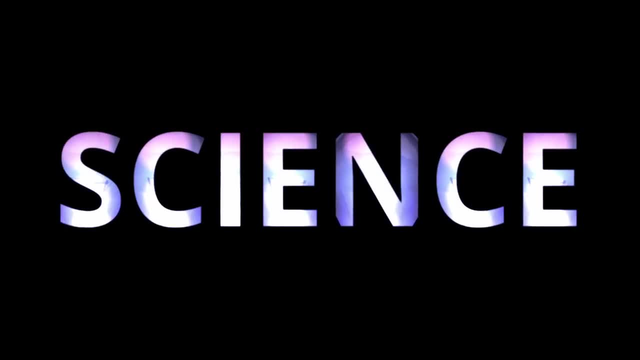 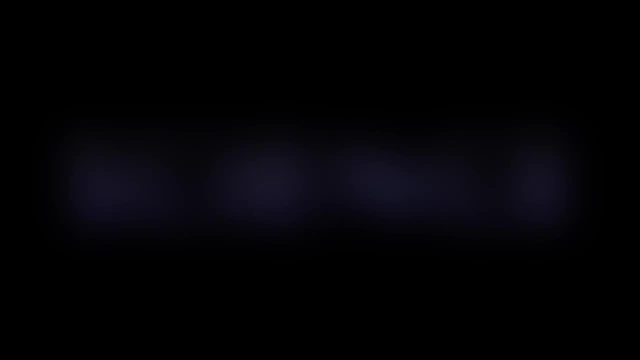 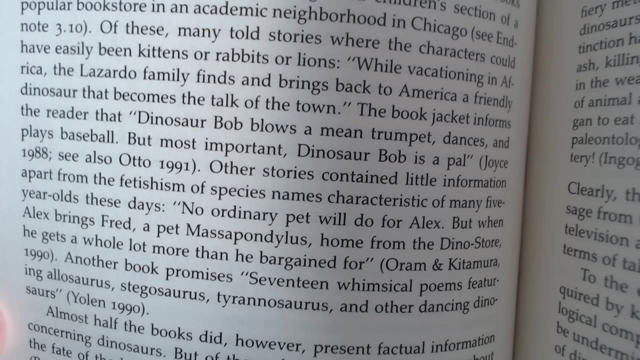 research. The more I learnt, the blurrier science became, The more contradictions and arguments I found that I couldn't resolve, the less I felt I could ever reach a satisfying conclusion. Deep in this mindset, I came to Clemens' account of her perusal of the children's section of a 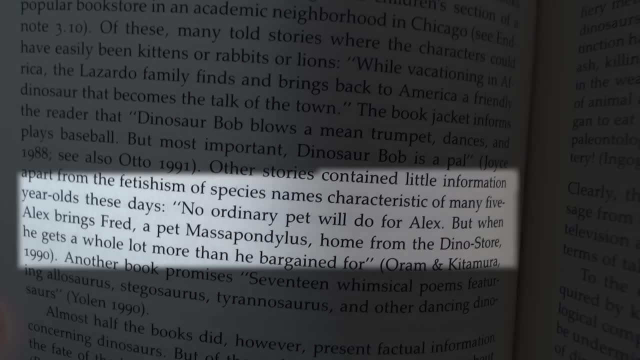 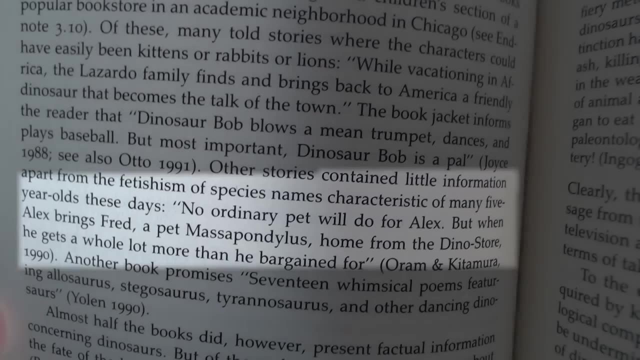 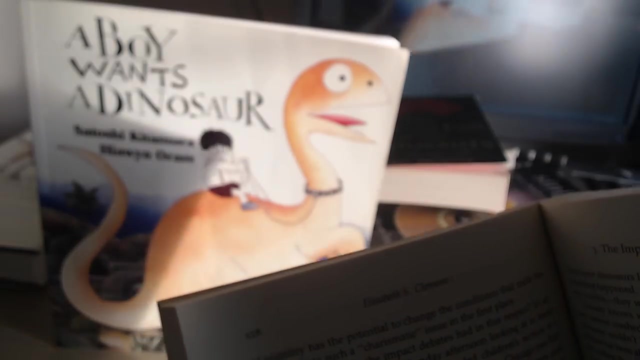 book. It contained little information apart from the fetishism of species names characteristic of many five-year-olds these days. No ordinary pet will do for Alex, but when Alex brings Fred- a pet Massaspondylus- home from the dino store, he gets a whole lot more than he bargained for. 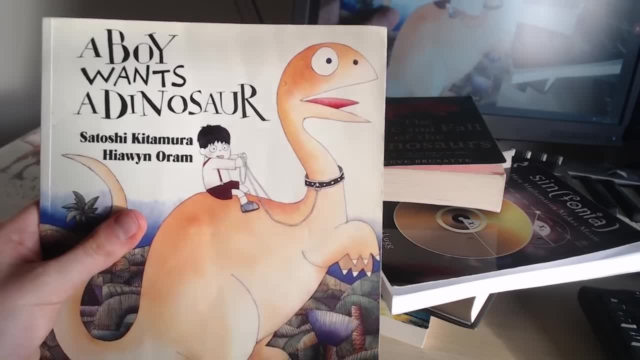 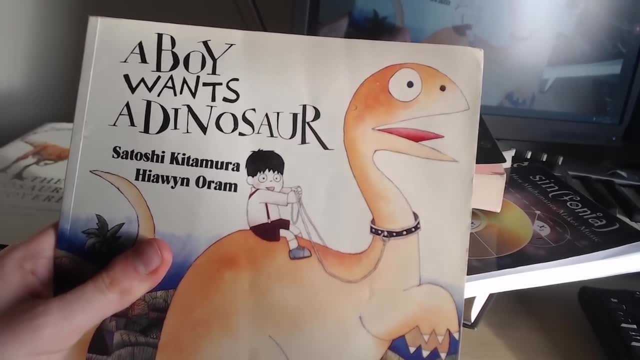 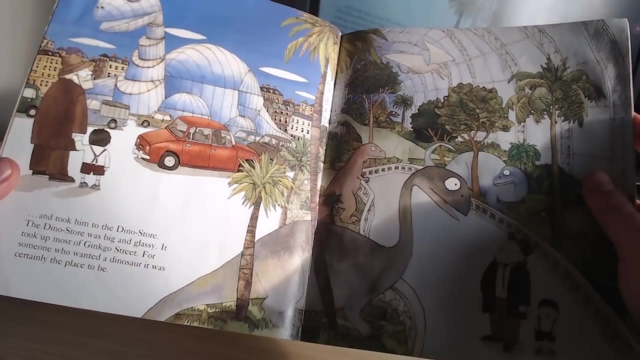 I remember this book. It's one of the first books I ever read. Parents say I forced them to read it to me every night for six months, that I memorised all the words, that I sculpted them if they got the words wrong. And you can't buy dinosaurs at the dino. 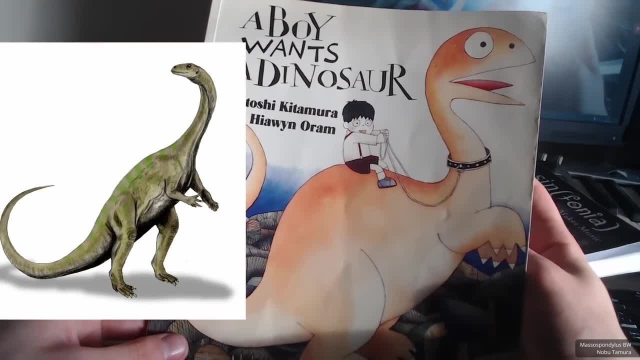 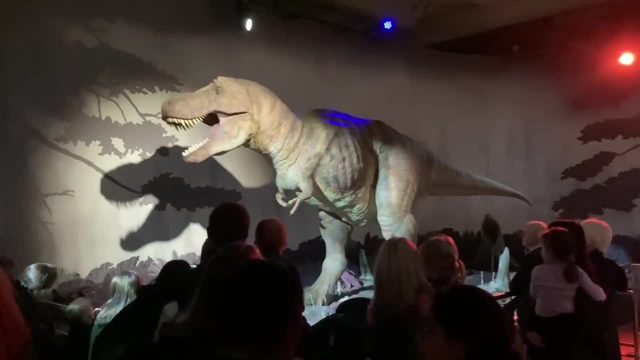 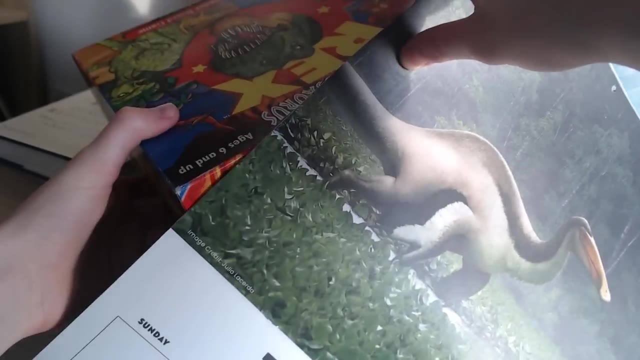 store And that's not what a Massaspondylus looks like, But this is where it began. Dinosaurs- I've always loved dinosaurs. My favourite is the triceratops. Dinosaur books and games and toys and TV shows and friggin' calendars- All my life I've been in now. 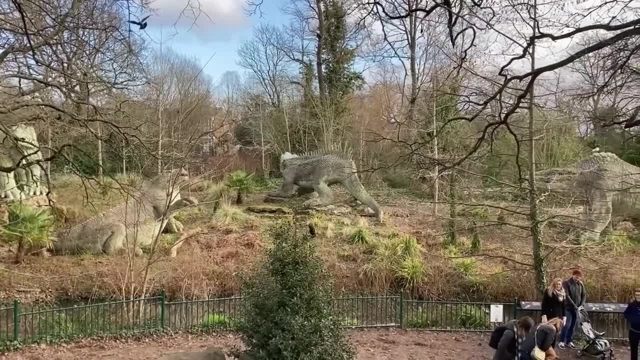 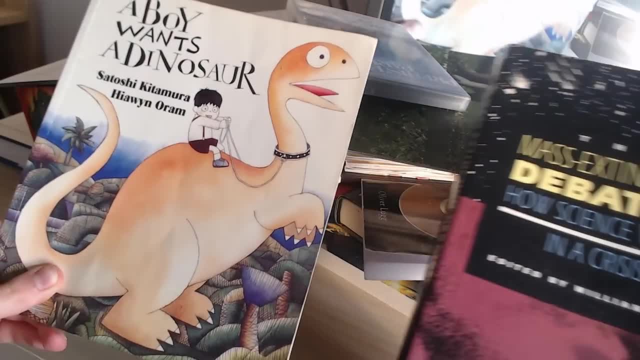 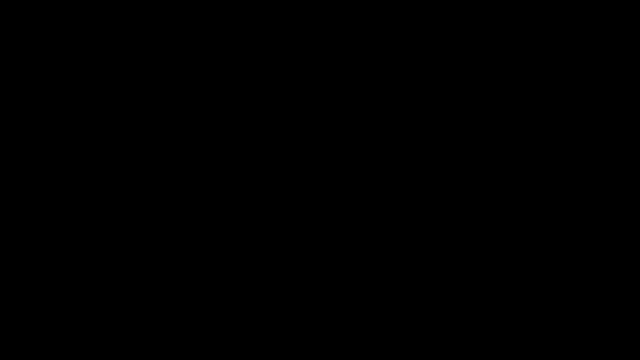 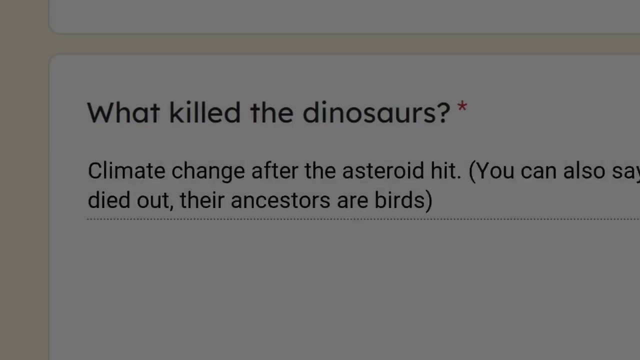 hammered with dinosaurs. I've always been on this dinosaur journey, a constant inspiration, even as so many other passions faded. And I had in my hand at once the beginning and the end And it all became clear. There was, in my opinion, a single answer to my survey that got it right, A single guru. 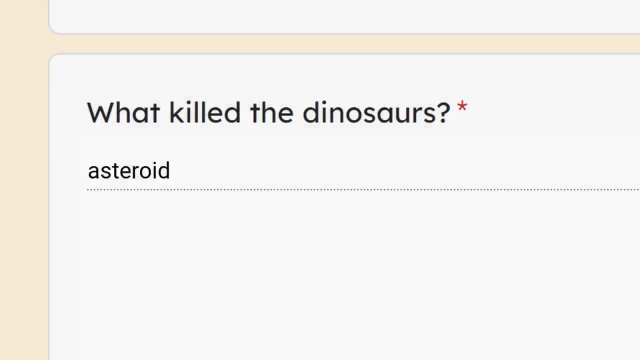 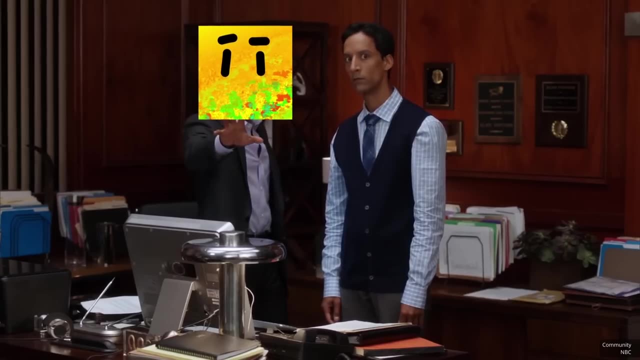 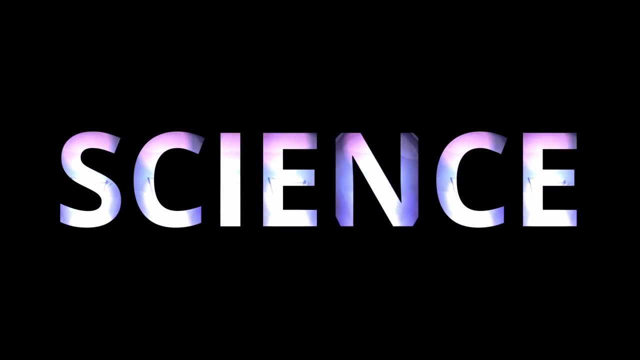 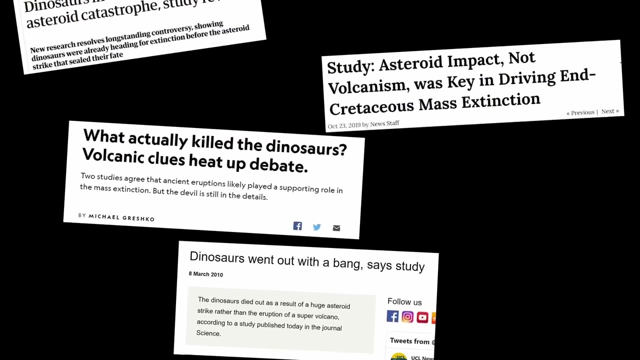 graciously dispensing spiritual truth upon us. What killed the dinosaurs? It doesn't matter, I can explain. Let me explain. What is science. Is it hypothesis testing? Is it a method for reducing uncertainty about the world? Is it groundless, incomprehensible didactic truth statements? The question is hard to answer because 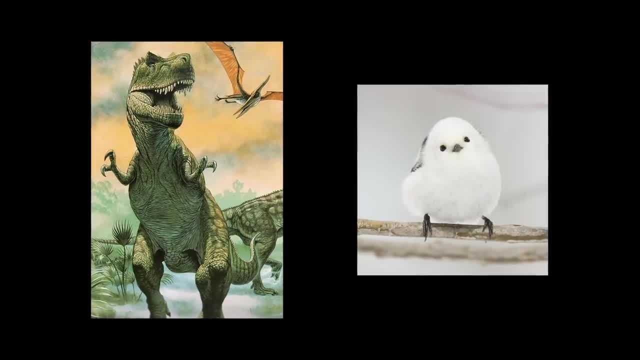 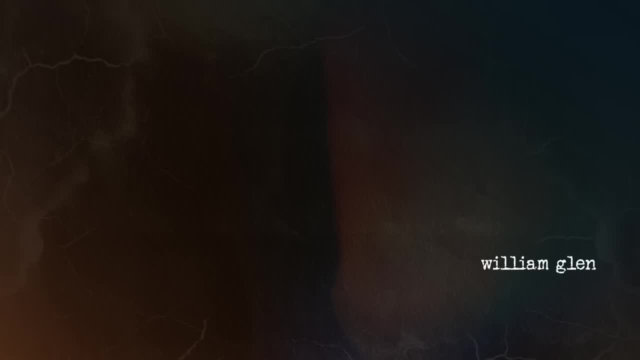 much like dinosaur. it means different things in different contexts. But right down at the metal, in The Philosophical Ideal, I think William Glenn in this 1997 article puts it best: Science is the only self-correcting system of knowledge known to history. 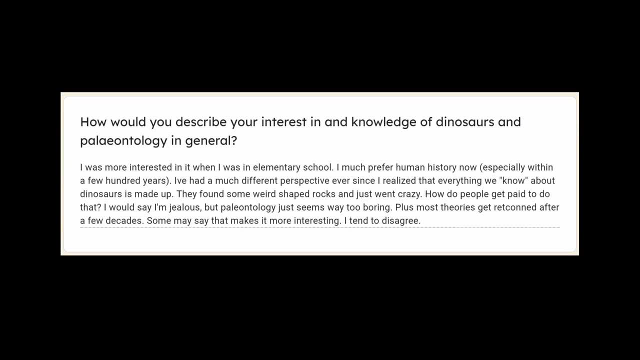 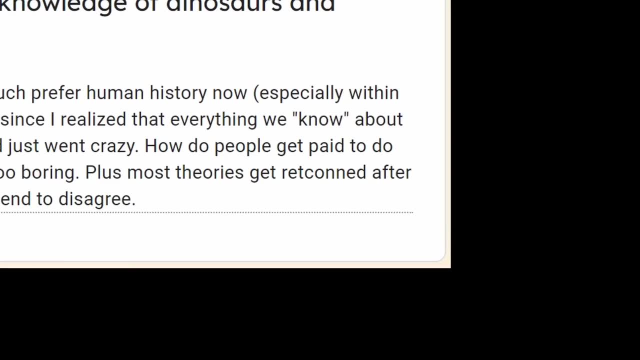 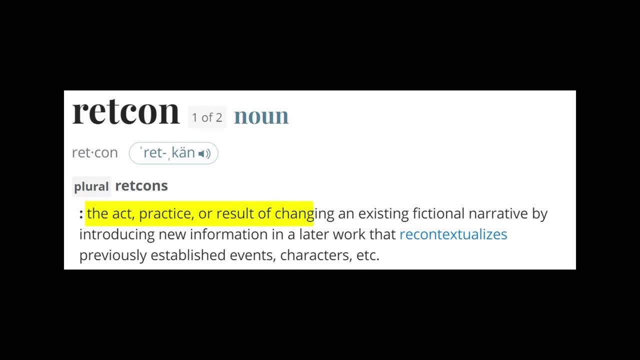 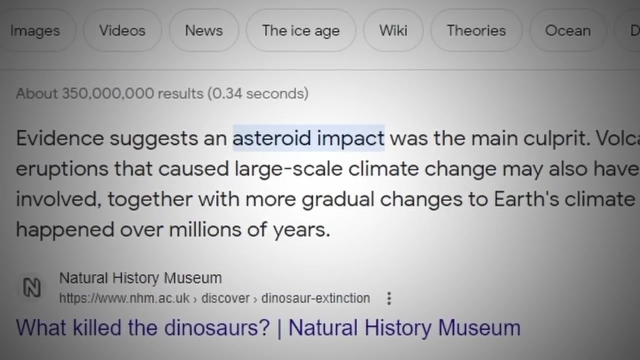 In light of this, let me pull up another response to my survey that stuck in my mind. Someone claimed to dislike paleontology because everything we know about dinosaurs keeps getting, in their words, retconned. Whatever the ideal of science is, it is not a coherent narrative. 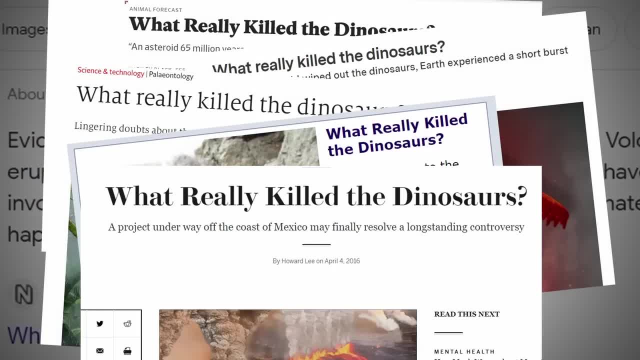 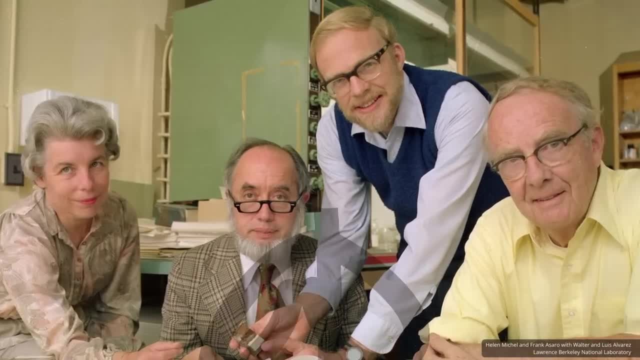 Biases and distortions arise because we, as humans, want it to be one. We want a satisfying story, a simple, memorable idea. We want heroic mavericks and great dogmas to overcome. We want beginnings, We want ends. 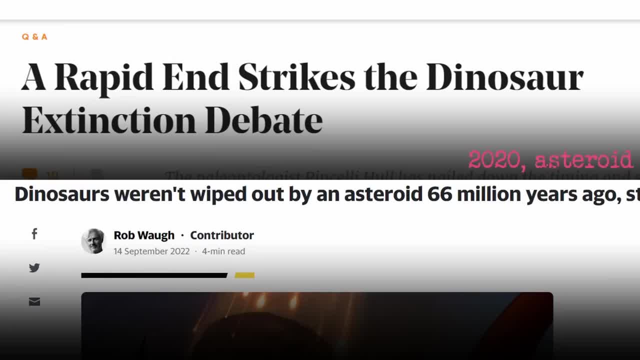 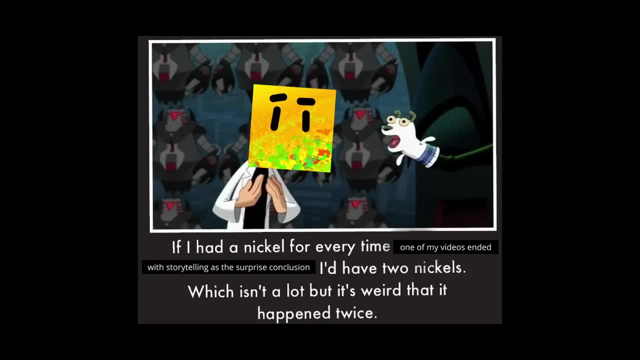 Seriously, everyone seems to want to claim the end, the final word, the great summarising certainty. Even I'm doing it right now. I have the dramatic music for it and everything. Yet science is under no obligation to give us any of those. 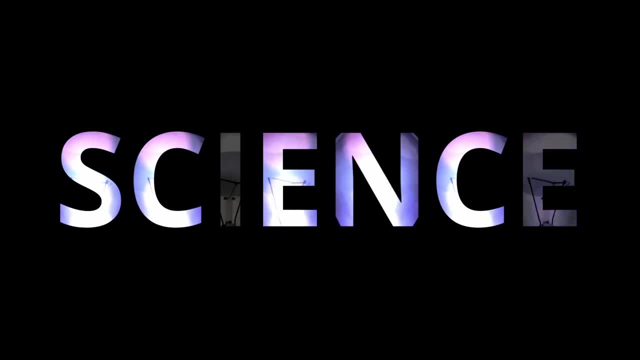 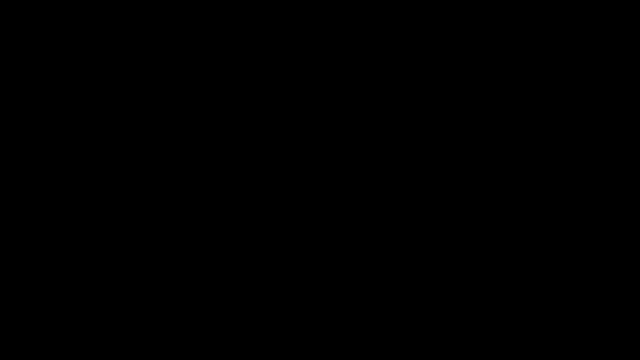 The scientific method is valuable and has transformed the modern world precisely because it is designed to reduce this tendency towards good storytelling. A corollary of science as a self-correcting system is that science will always be wrong, But it's hard for our brains to deal with that. 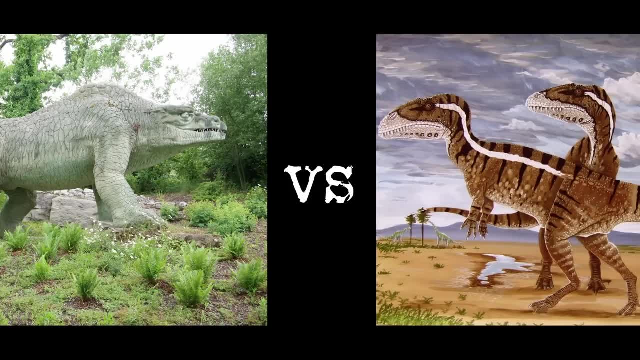 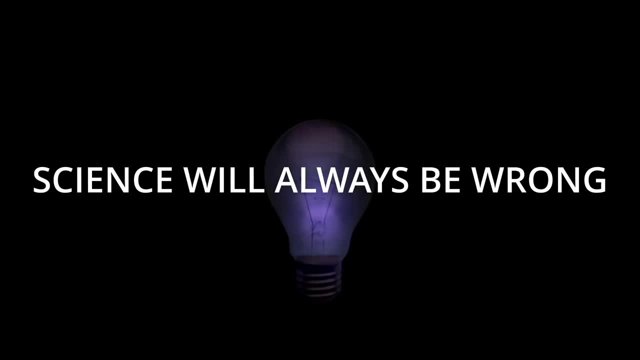 There are some things significant evidence does make us sure. about Others we're still in the dark. Yet science requires us to doubt everything. How can non-scientists assess the correct level of doubt? We can't help but find this contradiction unsettling. 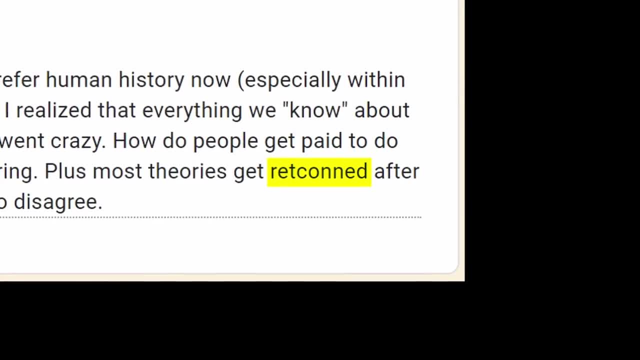 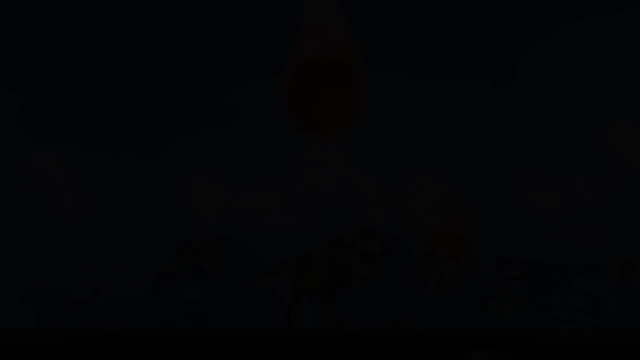 Our communication as a species depends on forming a story: The story of a scientific paper, The story of an eye-catching result, The story of Jessica Alba's sexy hair, The story of Jessica Alba's sexy hips. Some of these are definitely more worthwhile than others. 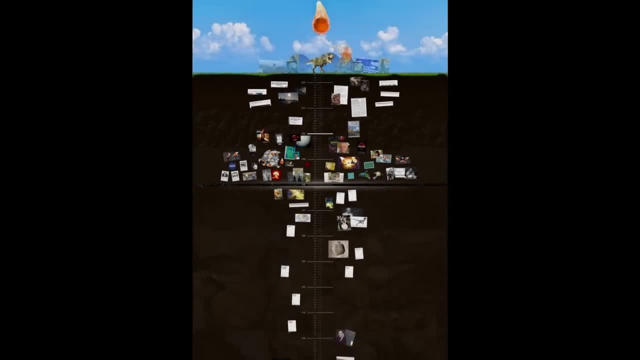 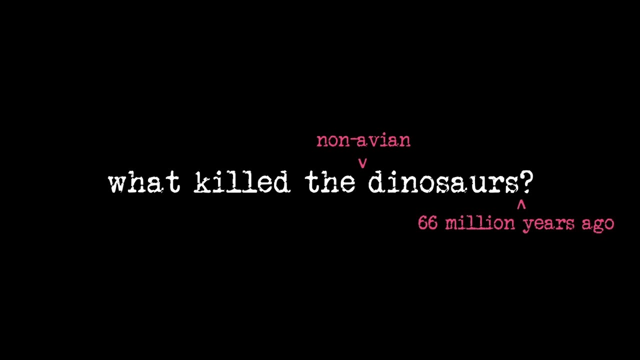 but maybe it can't be avoided. Story with all its disfigurements is the inspiration we as a society rely on. So here's what I think You can dismiss all of what I'm about to say. Again, I have no authority here whatsoever. 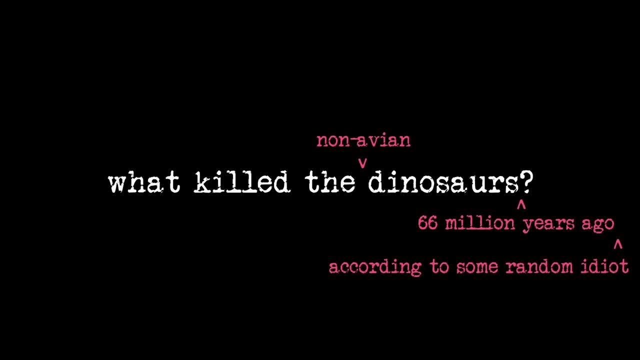 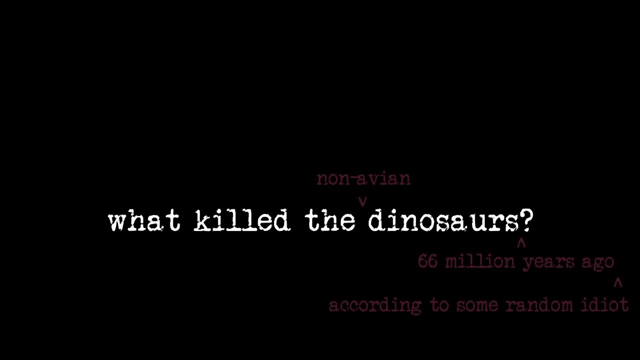 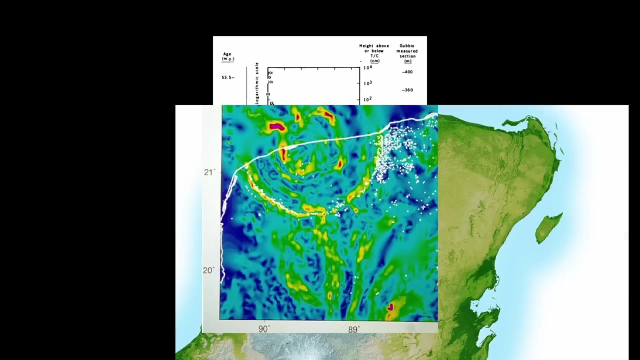 But this is my satisfying conclusion: If we have to tell a story, we shouldn't be telling this one, Because the one that actually matters is: how do we know what killed the dinosaurs? And sure that includes the evidence, the deductions, the results from the majority of specialist papers. 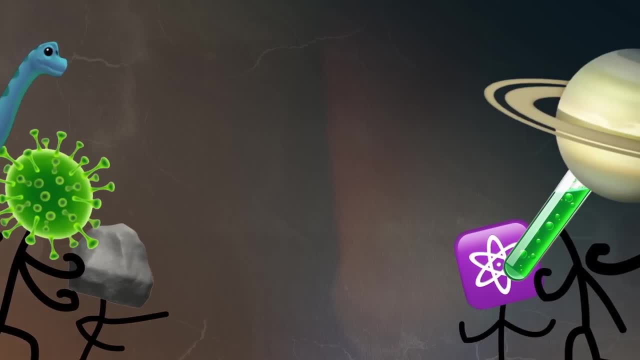 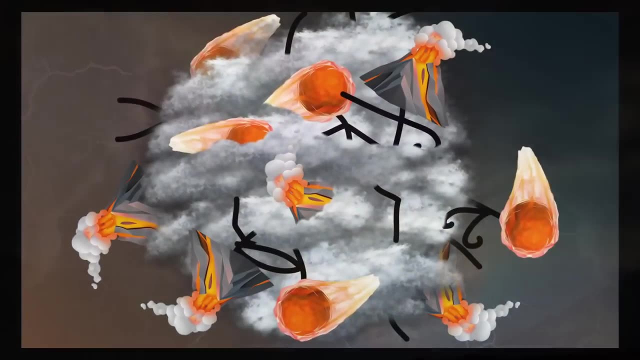 that have supported Asteroid. More than that, though, it's about the communication ecosystem that moulded what you think. you know, The realisation that an obvious fact resulted from innumerable poor judgements could in truth be thrown out at any moment. 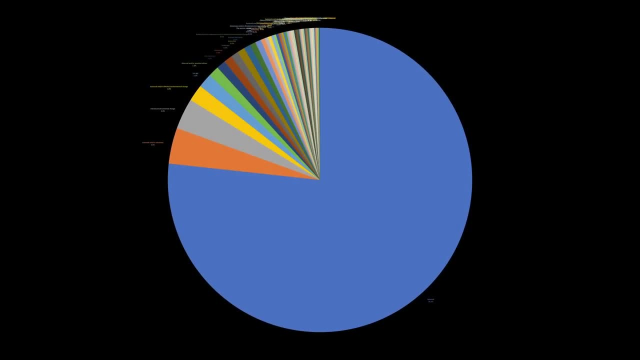 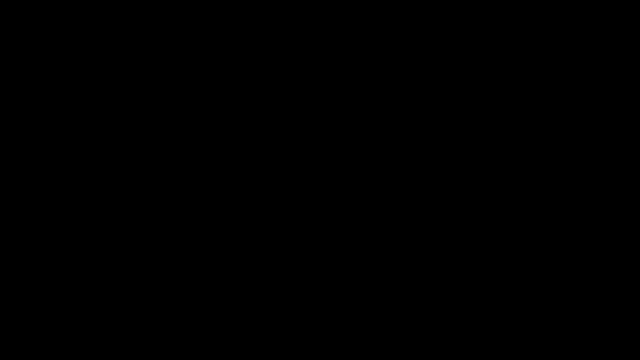 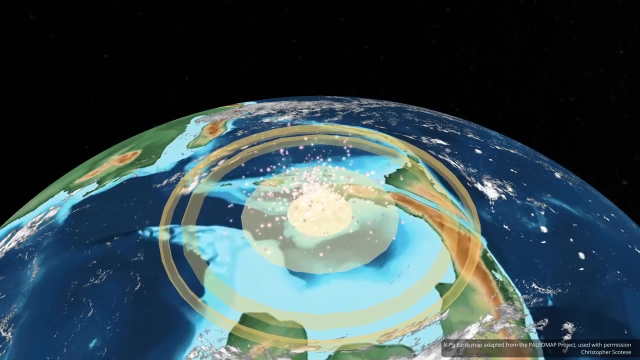 and yet should roughly be accepted by the average person anyway, Because forever everyone who isn't a scientist, the result doesn't matter. Is knowing whether it was an asteroid or volcanoes that killed the dinosaurs going to change anything about your life? I don't think so. 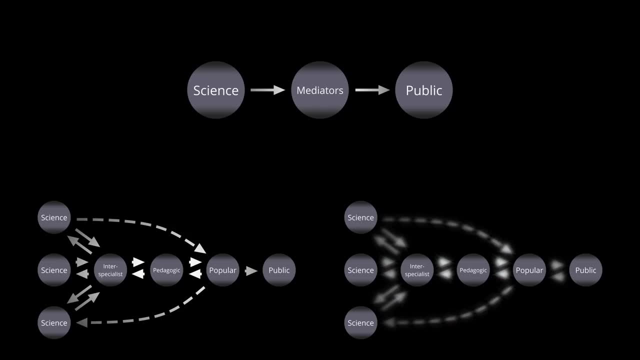 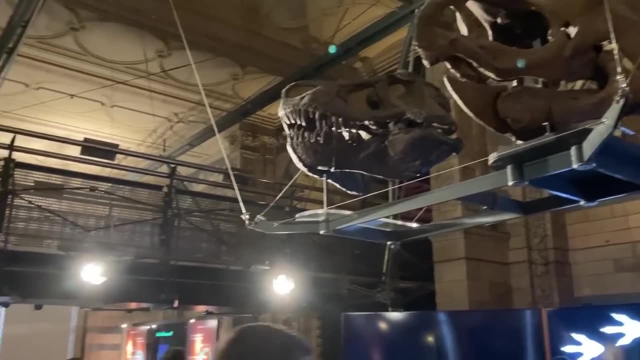 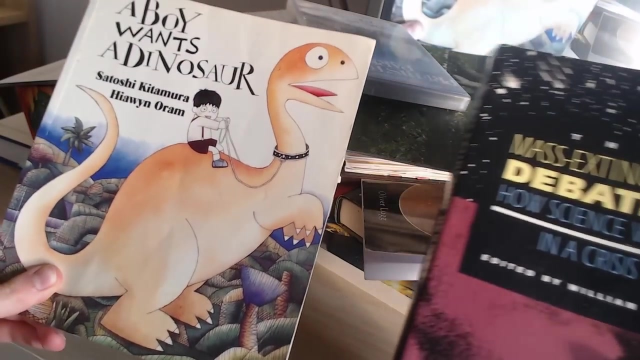 But knowing the intricacies, human inaccuracies and scientific ideals that made you believe it will. Dinosaurs are inherently inspiring And I believe that inspiration should be co-opted to shine a light on the story I've told today. Clemens has a point in her dissatisfaction. 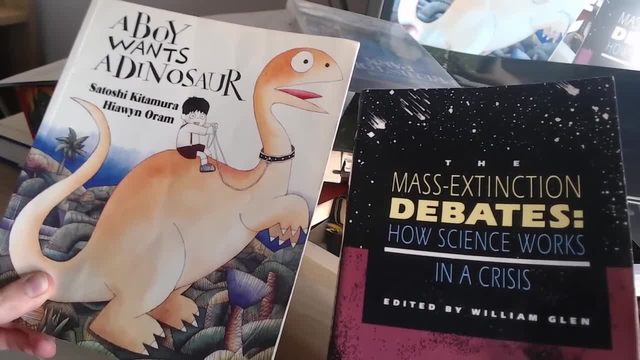 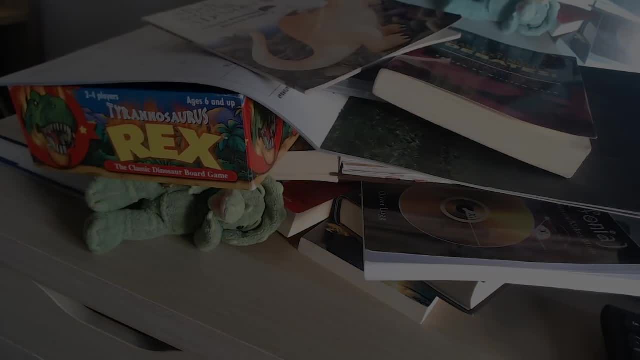 with children's books about dinosaurs. But if it wasn't for them, this video about the nuance and complexity of science wouldn't exist. Maybe it's survivorship bias, but it proves the potential for everyone to reach a fuller understanding. I believe everyone. 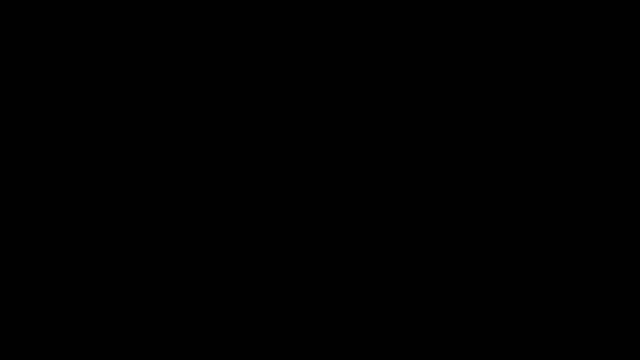 should repeat my journey. Why? Because there are a million more relevant scientific findings embroiled in constant debate that do demand your input. Questions like: How dangerous is the coronavirus? What is causing climate change? The extinction of the dinosaurs may have a controversial history. 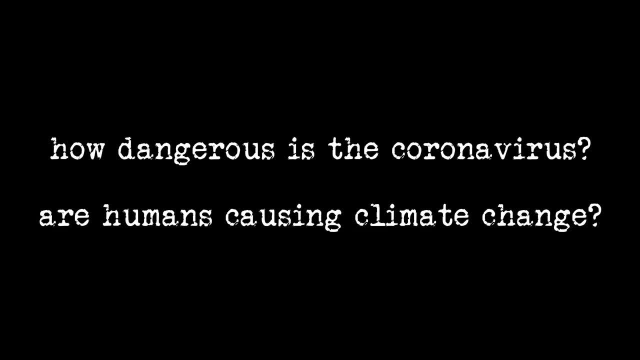 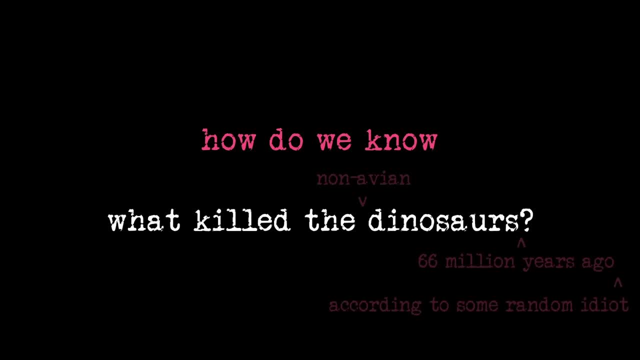 but by societal standards it's nowhere near as fraught with conflicting communication as issues like these. By understanding how science works in a relatively harmless petri dish, one we can all be inspired by on neutral terrain, we are all better equipped for bigger challenges. 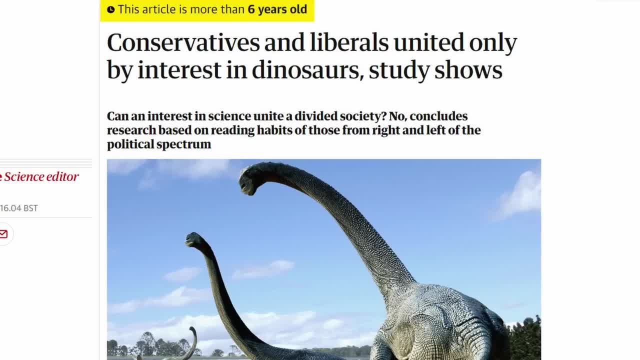 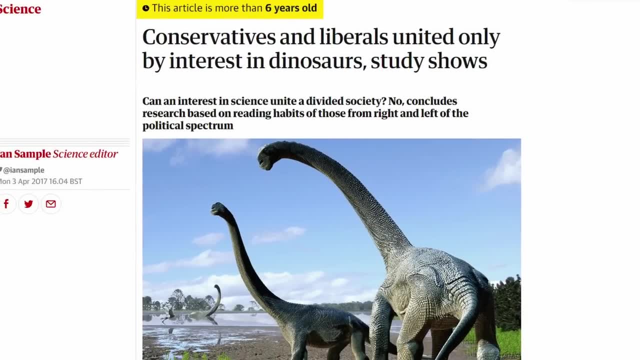 I mean, just listen to this headline. I found Conservatives and liberals united only by interest in dinosaurs. A study claims dinosaurs are our only common ground. The article seems to think that's a bad thing, but I've found a way to make it useful. 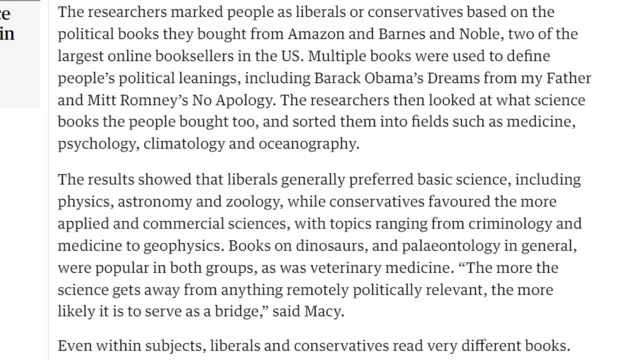 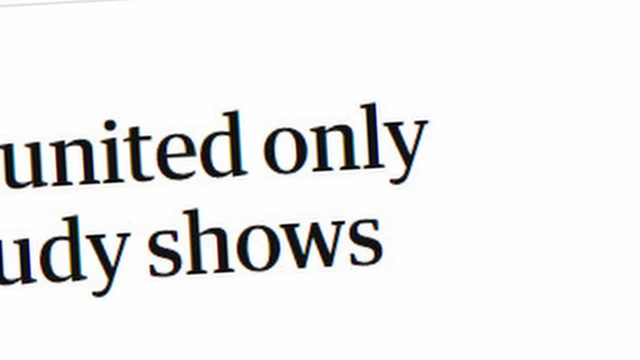 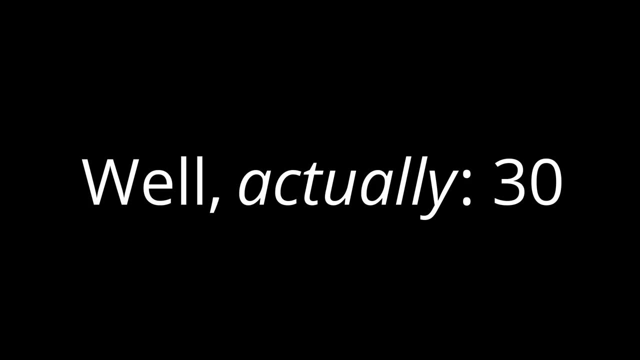 Although the results of the study which correlated book buying habits to judge political affiliation, were that we're united by dinosaurs and veterinary medicine. Only Way to go. I haven't just been keeping this counter for its vast comedic potential, but because I hope it makes a statement. 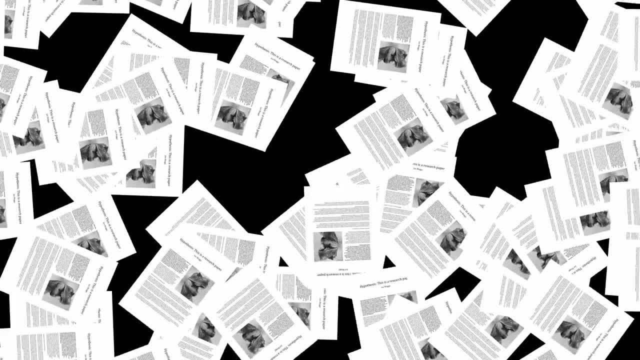 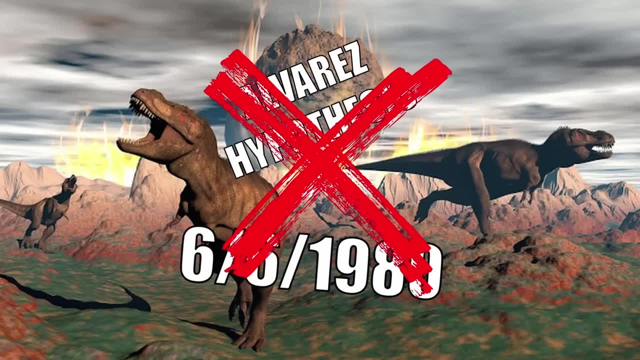 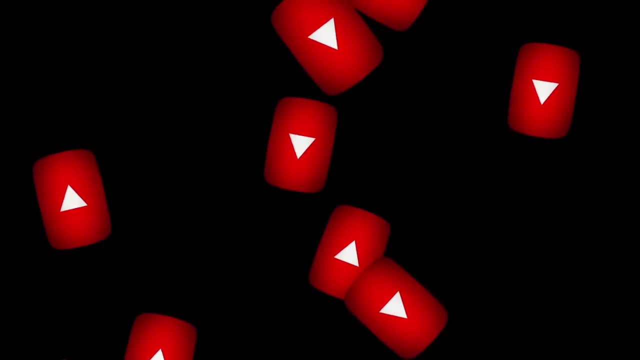 Knowledge is fractal. Well, actuallys, I've had to break my narrative coherency or that of others time and time again to deal with them. It's impossible to make content for my intended context without missing some. The same is true of everything on this site. 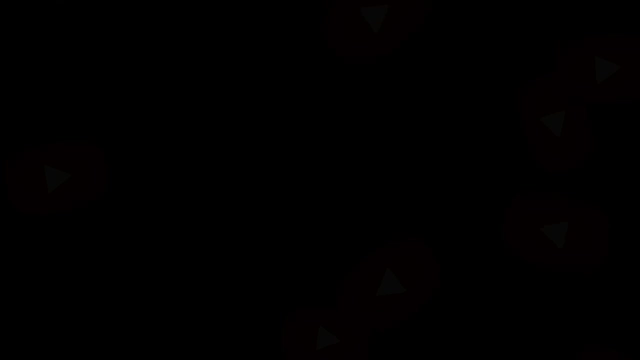 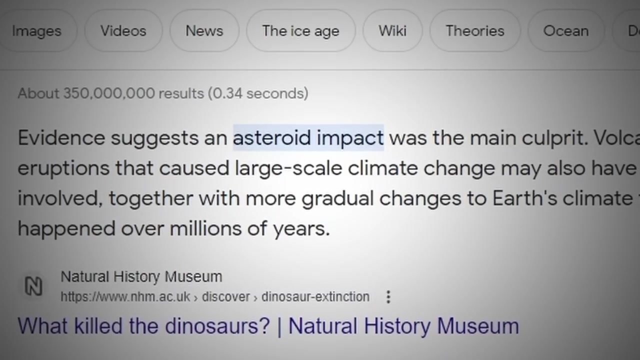 Every piece of science you've ever seen. I hope the takeaway is not the content of these corrections, but that they exist, The awareness that no matter what story someone tells you, no matter the hold of its paradigm over your mind, the fact it is a story. 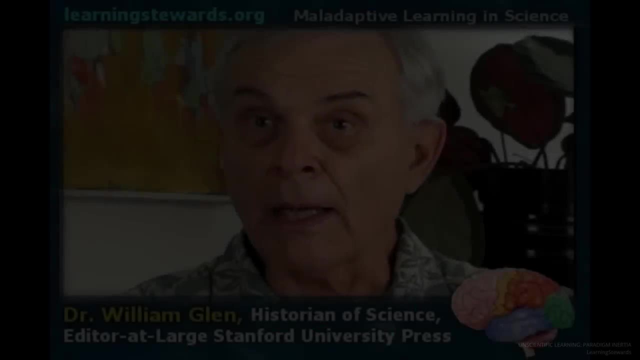 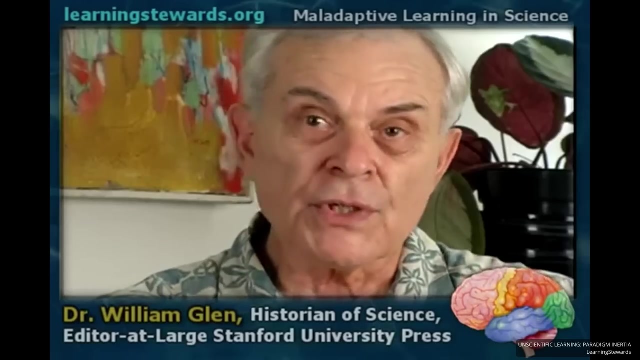 prevents it from being the truth. In the mass extinction debates and in an interview which makes my own points much more eloquently, William Glenn states he believes the purpose of science, history, is to point out the seeds of subjectivity and make us aware of them. 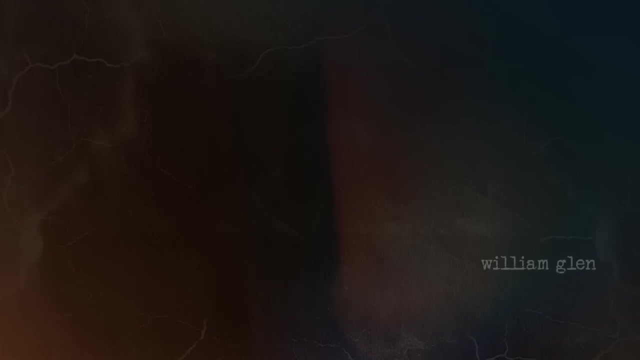 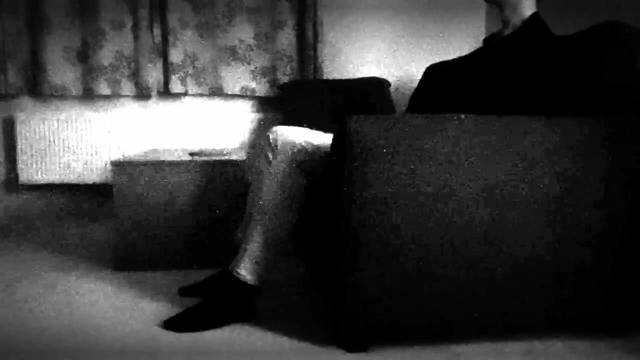 He quotes from Harry Overstreet's The Mature Mind in stating: the single criterion of mental maturity is the ability to hold a suspended judgement. If I might paraphrase, society is not the enemy, It is the ideal we should all strive for, Not in a throwing your hands up. 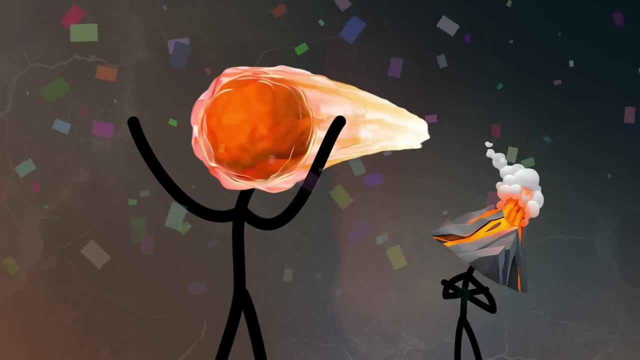 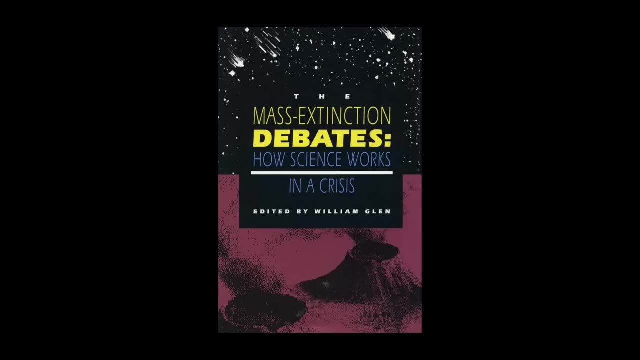 and deciding no one knows anything kind of way, but in an inherent distrust of your own mind's desire for narrative fulfilment. It is extremely hard. I'm not good at it. William Glenn admits he's not good at it. Society as a whole certainly. 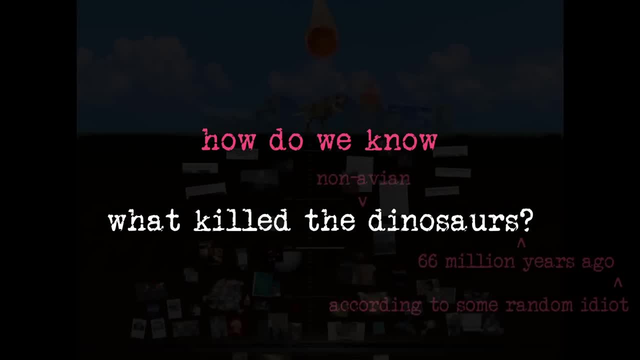 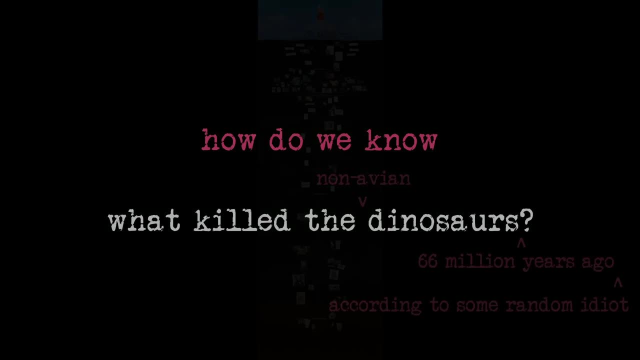 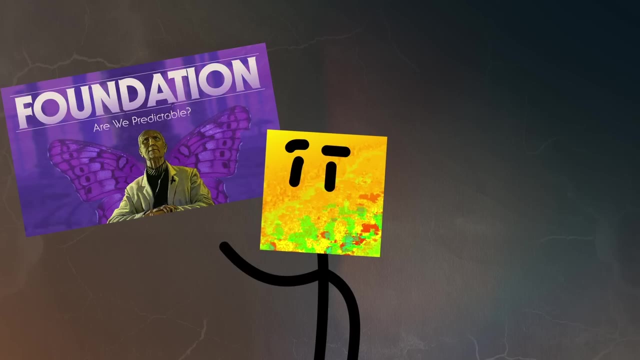 isn't good at it, But we can be better, And if I and a load of dinosaurs can help with that, maybe the story was worth telling after all. You know, last time one of my videos came to the conclusion that uncertainty was worthwhile. 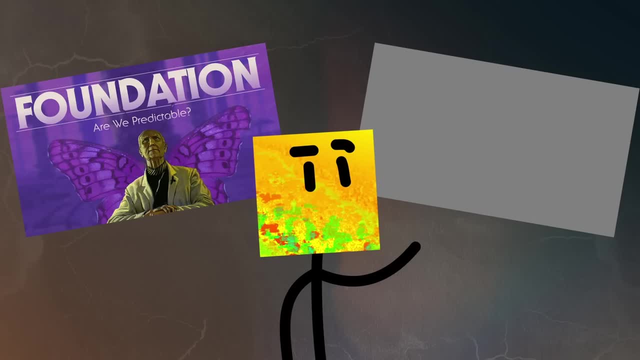 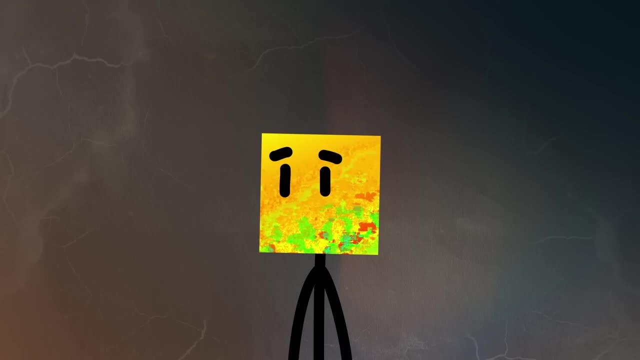 I had my immediate comeuppance at the hands of a projectile from the sky. Good job, there are none of those in this video. Huh, Guess the power of rejecting narratives has broken me free of my own tyranny. Wow, I get to have an actual ending. 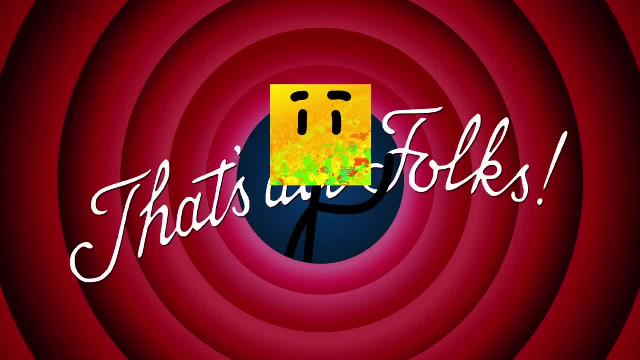 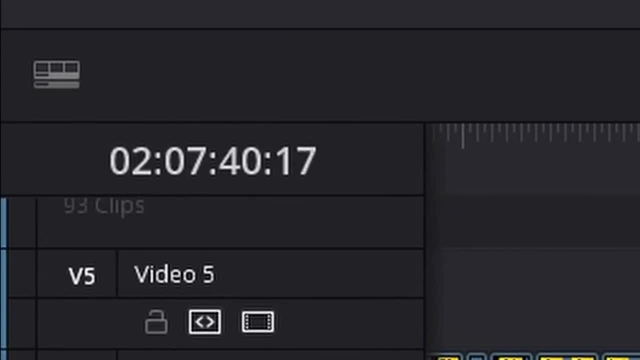 Thank you all so much for watching. Hope you got a lot out of it. It's been a bumpy road to get here. Safe to say, I'm not making a video this extensive again for a long time. Special shoutout, by the way, to those. 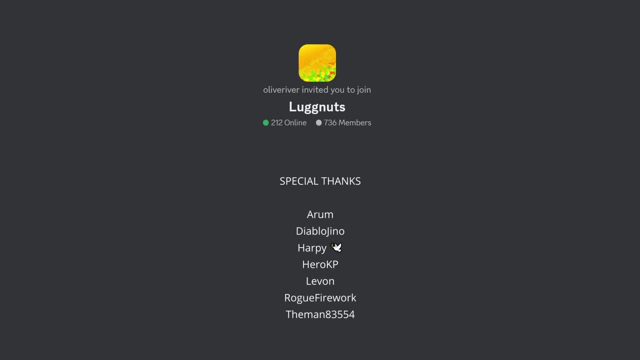 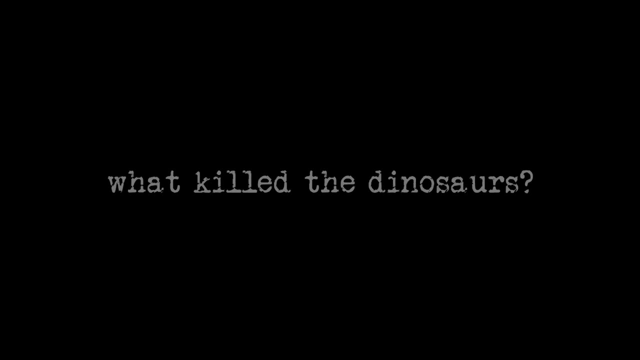 on my Discord, who provided feedback on a draft version of this video and assured me I wasn't going completely mad As a treat for sticking with me so long. let's end with a review of the less conventional answers I received in my survey. What killed the dinosaurs? 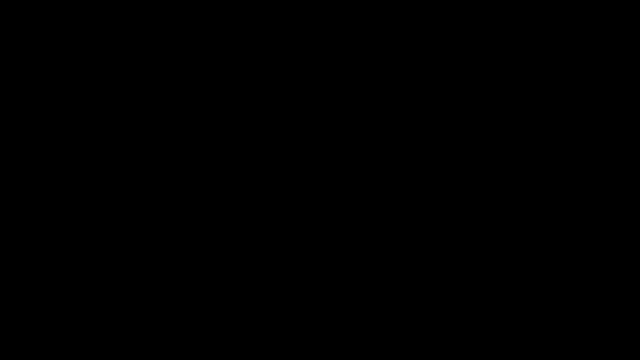 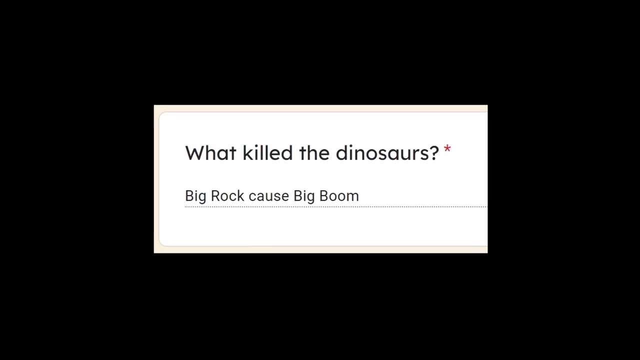 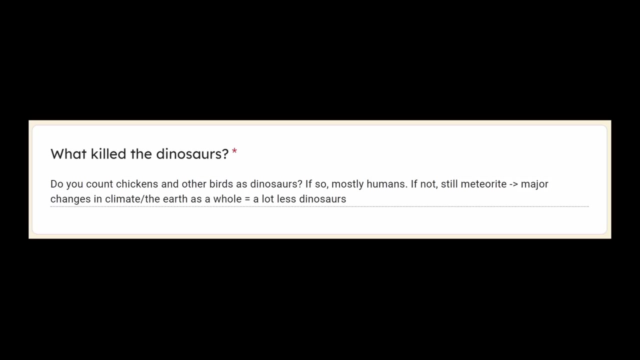 Aliens, duh. The Great Jurassic Eucalyptus Famine, Big Rock caused Big Boom. Do you count chickens and other birds as dinosaurs? If so, mostly humans. Oh my god, that's probably technically correct. 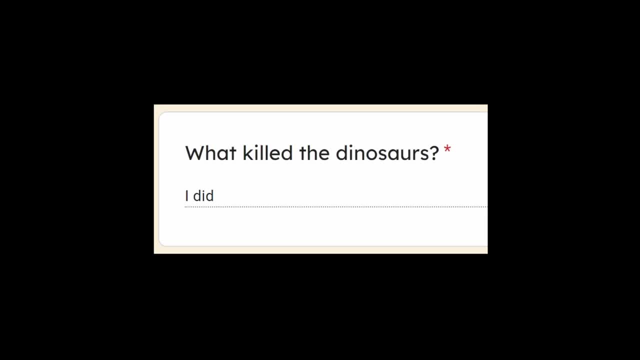 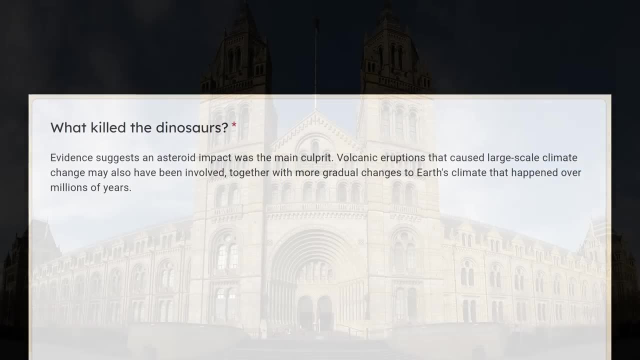 No sun. lol, I did. Society Evidence suggests an asteroid impact was the main culprit. Volcanic eruptions have caused large scale climate change may also have been involved, together with more gradual changes, with climate halved over millions of years. 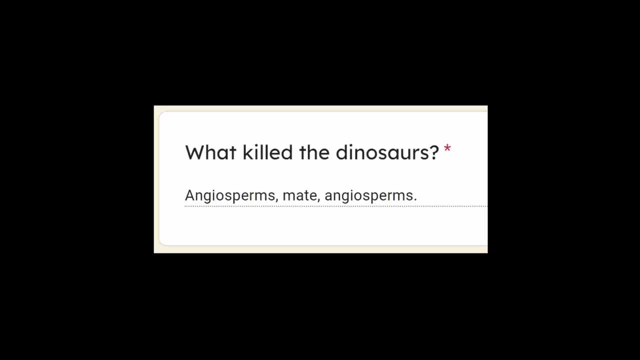 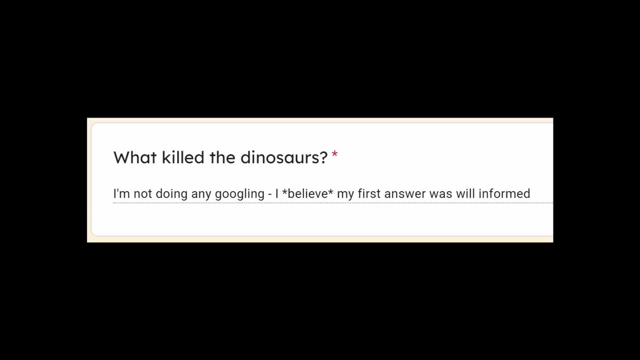 I am not lazy. Angisperms, mate Angisperms, Veronica Sawyer and Jason Dean. Apparently, this one's a reference to the musical Heathers. I'm not doing any Googling. I believe my first answer was well informed. 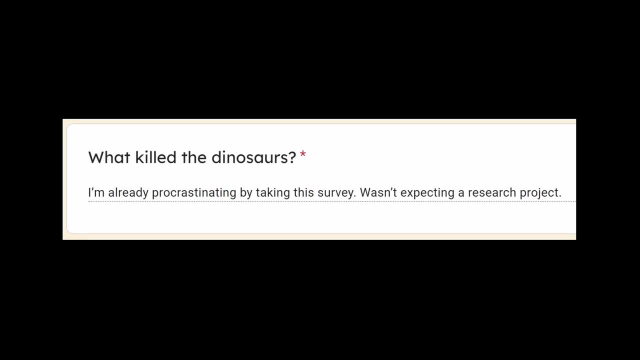 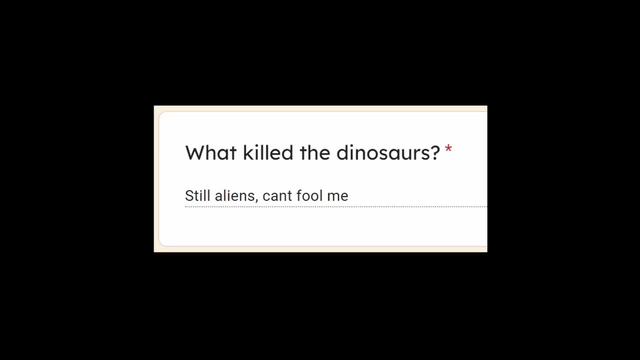 Ho, ho ho. do I have a video for you? I'm already procrastinating by taking this survey. Wasn't expecting a research project. Hubris, EA Games- Still aliens, Can't fool me. Dwayne Johnson Not gonna bother checking much. 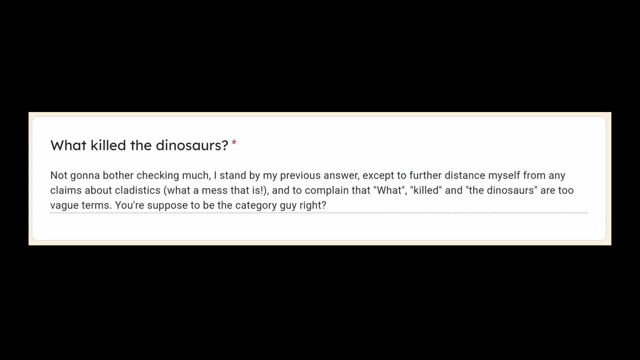 I stand by my previous answer, except to further distance myself from any claims about cladistics- what a mess that is- and to complain that what killed and the dinosaurs are two vague terms. You're supposed to be the category theory guy, right?